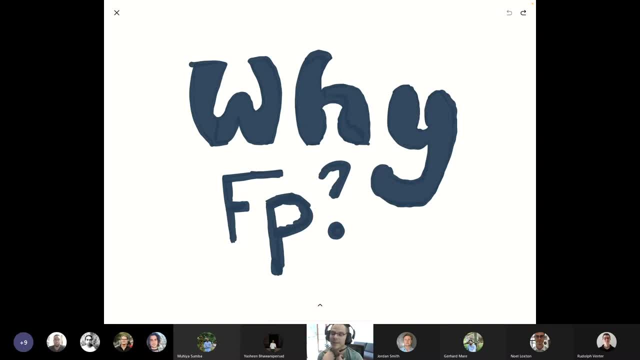 you get imperative languages Which are like it's all about the imperative, And so when I think about the word imperative, it means like steps, It's very much like step driven. It's like do this, then do that right. 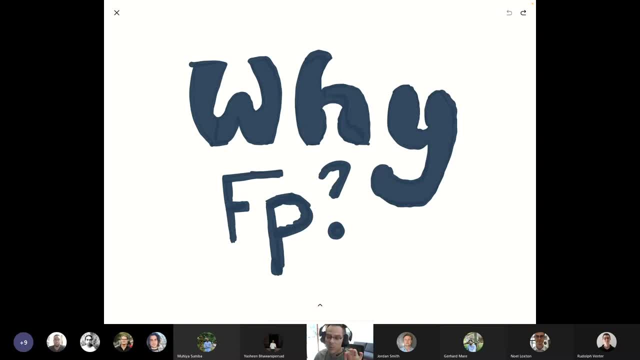 Whereas functional programming often is more about like it's more about the what- What am I trying to do, rather than how am I trying to do it, And then just kind of using it's called like reduction, reduction to solve the problem, And it's very much the same as. 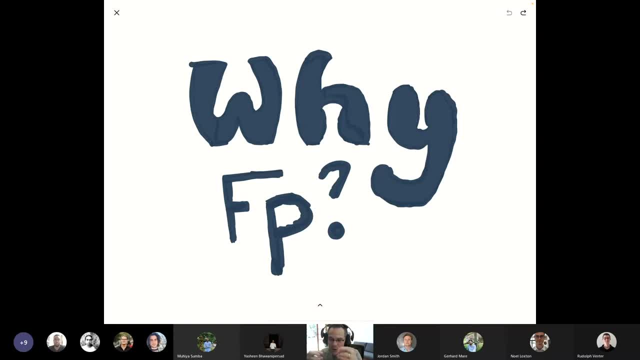 what you would do in maths, So you'd create functions in maths and then you just reduce it to the solution. Do you know what I mean? It's not like there's a like in maths. there's no for loop, There's no like real, like like repeat while do this, while like do these. 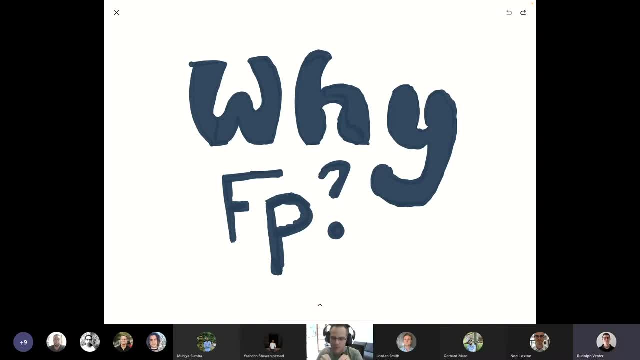 steps in order. Maths is like no. I write out the entire equation and I can reduce it to its answer. It's not like there's steps that need to occur while this thing happens. Do you know what I mean? And so I think, when it's contrasted against imperative programming, 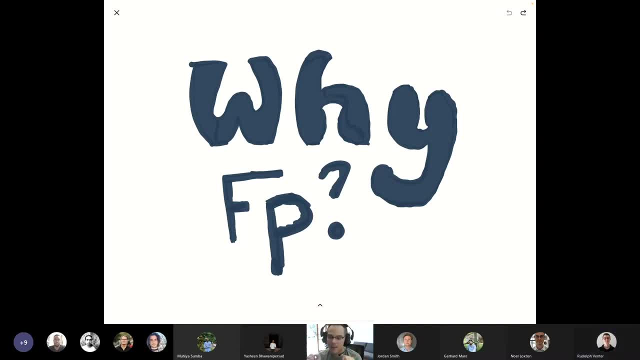 that's kind of like what functional means It's really, and I think your answer of saying it's more about the what, So describing working, describing the problem, rather than describing the solution to the problem, if that makes sense. So I've got a couple of. does anyone else want to say anything? 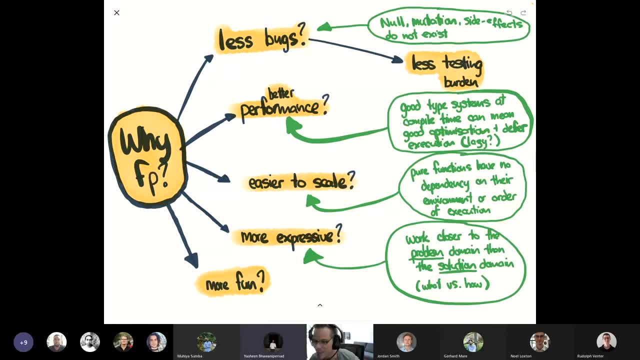 by the way, There was another hand up and then it dropped down. Was it Yashin Tom? like we never learned about it in university, but I remember reading about it on Free Code Camp And it and, like you said, it uses functions, but it's further broken down into two functions. 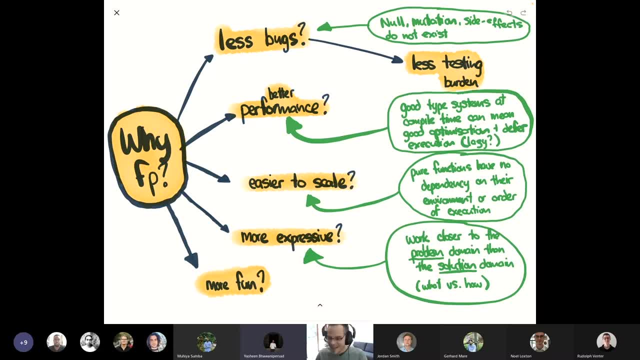 whether the function is a pure function or an impure function. Yes, That's the mathematical concept that you mentioned. Yeah, Like you said in C Sharp or in Java, you know you can use all these loops, but this thing is not focused on the loops. 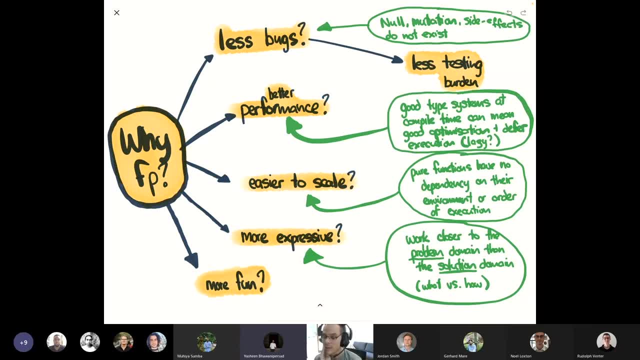 So it comes from the mathematical construct that you spoke about. Yeah, yeah, yeah. So you've hit another perfect point, which is purity in languages. I suppose, And mostly it is around functional languages that have got this thing around purity, So it's how pure a function is. 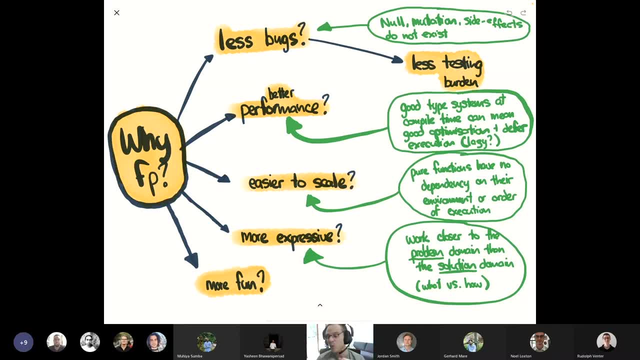 So you get pure functions And you get impure functions, And we'll talk a little bit about purity later. But, like as a summary, a pure function is one where it is the mathematical definition. So, given these inputs, I will always receive these outputs, if that makes sense. 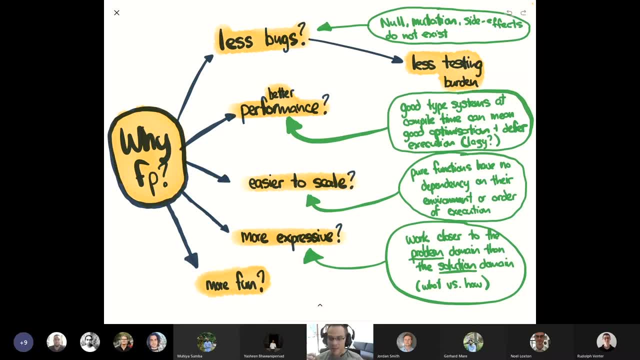 So if I give this function a three, it's going to give me back a four, Like if it's a plus one type function, right, it adds one to its input. That's a pure function because it's dependent on no other state around it. 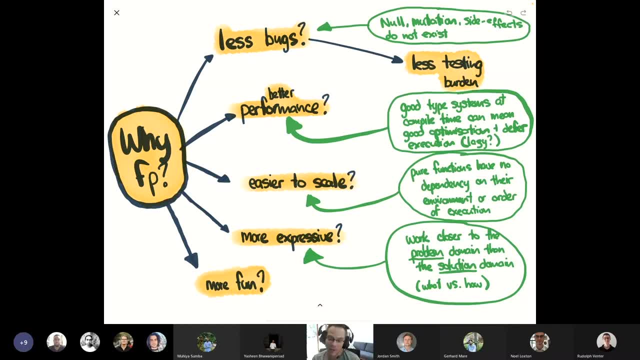 It's absolutely pure. So it doesn't matter what I give it. It doesn't matter what I give it. It doesn't matter what I give it As long as it's an integer, for example, as long as, like, of course, you can constrain your inputs. 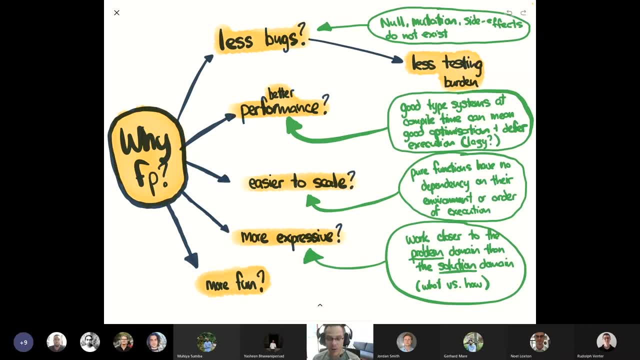 But, given a three, it will always return me a four. It doesn't matter whether the database is down or the file system is dead or the network is disconnected. If you give this function plus one a three, it will give you a four. 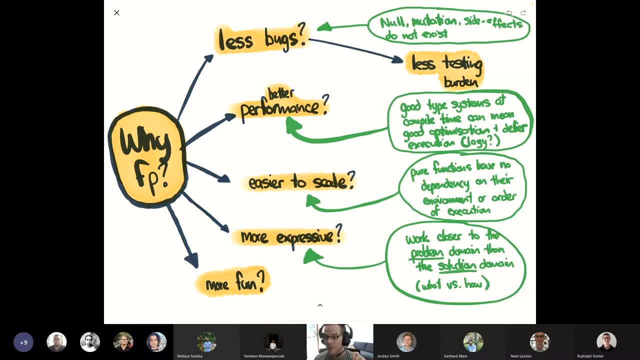 You know what I mean? It's absolutely. it has no dependencies other than its inputs, if that makes sense. And so that's what purity is all about. So a pure function is one where and there's interesting properties. So you might say: well, that's like, who cares whether it's pure or not? 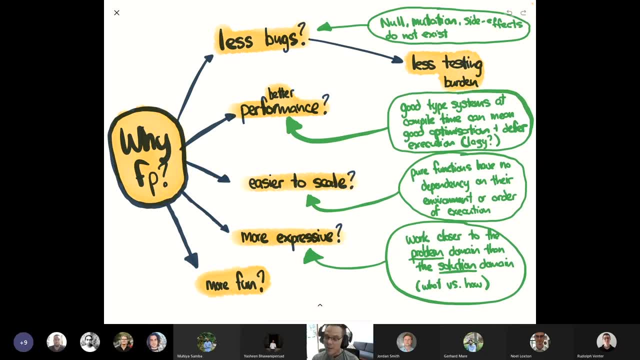 But if you know that a function is pure, you can do certain things with that function in order to optimize it. So if you always know that a three calling this function gives you a four and someone else later calls three with this function, it's like I could have remembered that the answer was four. 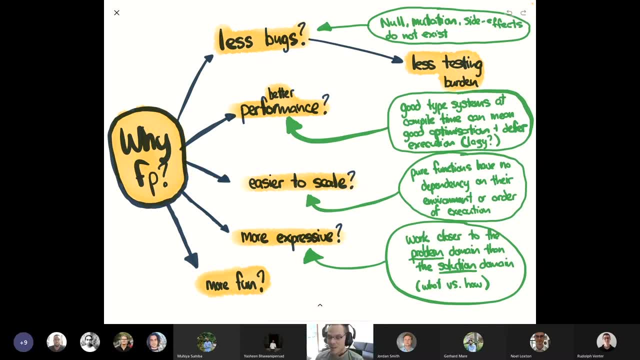 And like you don't even need to invoke the function right, So you can start to do some interesting optimizations around pure functions. Sometimes you also don't even need to call them Right. So something that's impure, it has a dependency. 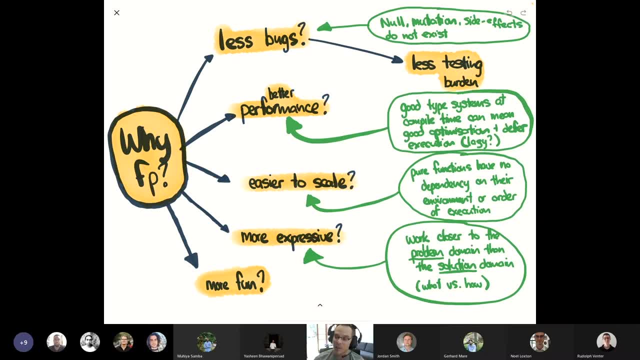 So if I call the function with a three and it looks up how much it needs to add to it from a database and it then figures out that it's a one, it means that next time I call this function that you know it could return a different value. 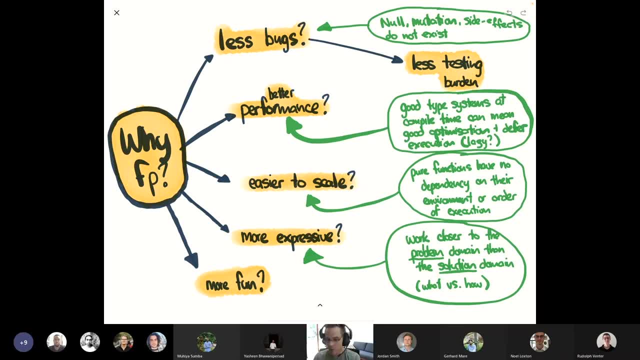 So that's no longer a pure function, if that makes sense. And yes, you can totally separate the world into pure functions and impure functions And good functional language. I shouldn't say good, but I should say like, very strictly functional languages. separate that very, very well. 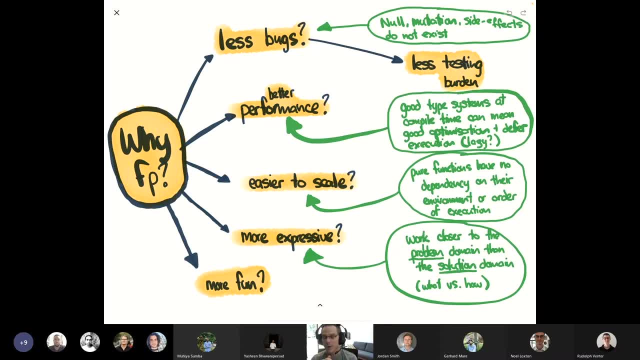 Separate the pure from the impure very well, Whereas more looser functional languages or even looser imperative languages kind of just muddle those things together And they just say: it doesn't matter whether your function is pure or impure, it's just in the way you write it. 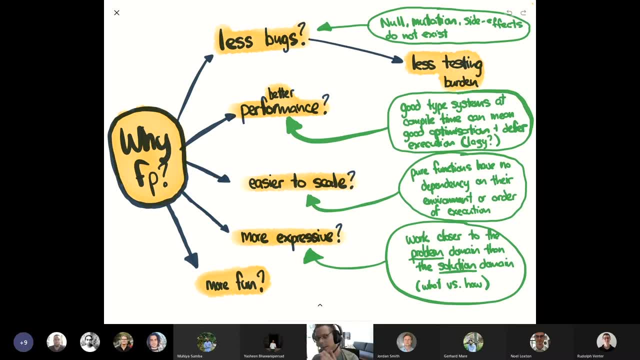 But nobody cares whether it's pure or impure, if that makes sense. So I think we'll talk about purity a little bit later. I think I've got some stuff to like, illustrate it maybe. So these were my reasons for like why FP? 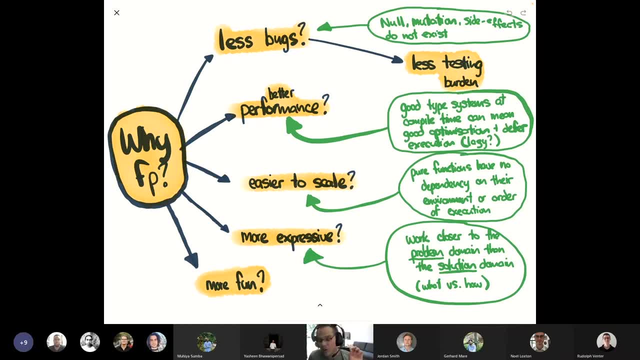 So why would I want to like research or study functionals, Functional programming or use functional programming? And these are some of like the popular opinions as to why. So for sure, less bugs, absolutely, I believe so. So I think writing code in a functional way does tend to have less bugs. 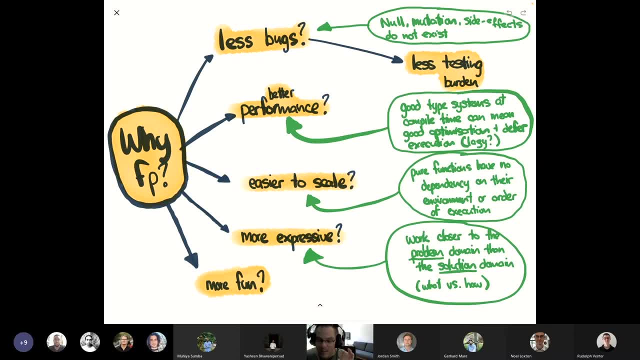 And we'll get into like I think this is an interesting space And this is really like beginner level stuff. So this is where we'll focus. So things like null, the concept of what is null, And mutation and side effects, which is that purity, impurity thing like, do not exist inside pure functional languages. 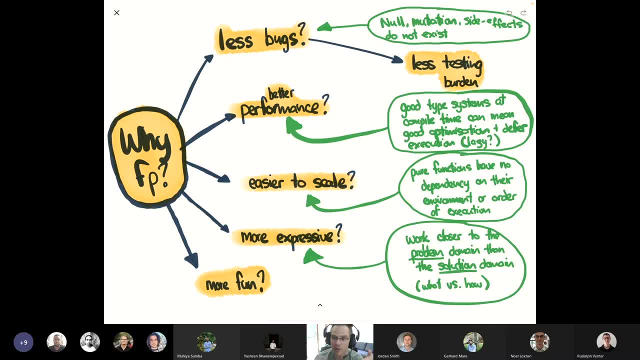 And those things are often, very often, a huge source of bugs. So null mutating stuff and side effects are a big source of bugs. So a very strict functional language may remove those things entirely or they'll put them into a clever little box to help you manage them, manage those side effects. 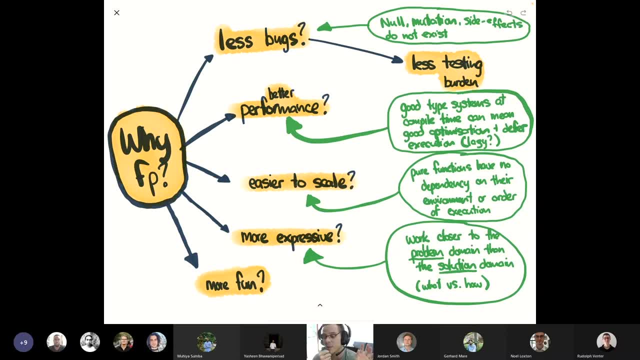 And so, like, less bugs means less, Less testing that kind of stuff. It doesn't necessarily mean that the code is written faster, though. Like, don't connect less bugs with like more code. I'm not sure. 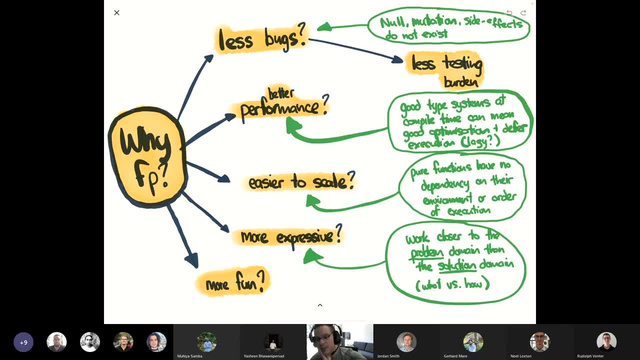 We can talk about that. But another good reason might be better performance, So potentially better performance. So I talked about this a little bit earlier. but, like having a good language which has a stronger type system allows a compiler to potentially optimize code better. 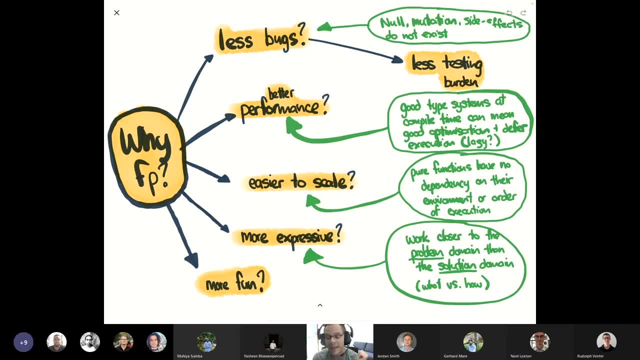 If that makes sense And even do stuff like hey, this guy never calls this function or never calls it with these kinds of inputs. so in fact, like let's never invoke that thing right, And that's called being lazy, potentially. 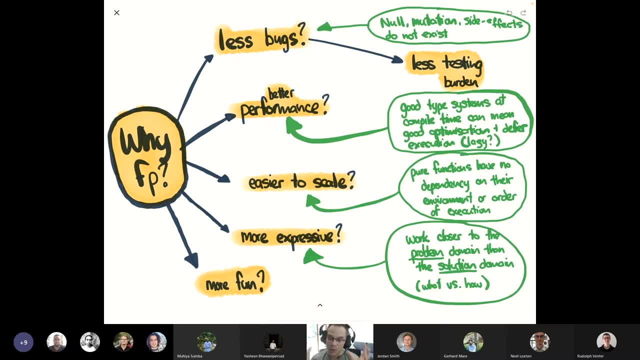 So if your compiler is a reduction one, so it reduces to the answer. things that are not part of that reduction tree, like never get executed, Whereas in an imperative language where you say do this, then do that, then do that, guess what? 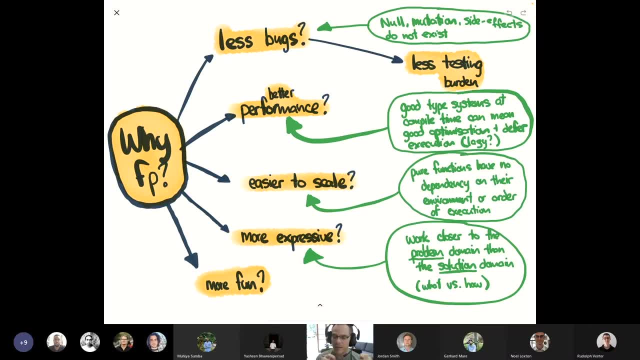 You've done all three of those before you get to the answer. If the answer at the end never needed you to do the second step, like in your imperative world, you still did it like that's. you know that's wasteful right. 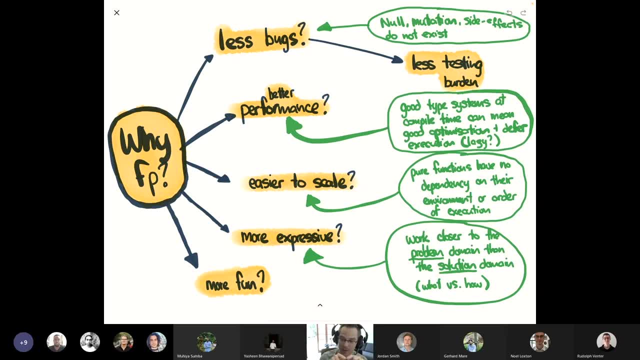 Whereas a functional language jumps right to the solution and it says: okay, I'm going to do this. and in order to do this, I need to do step one and step three and then resolve to the answer. Guess what? It just skipped step number two. 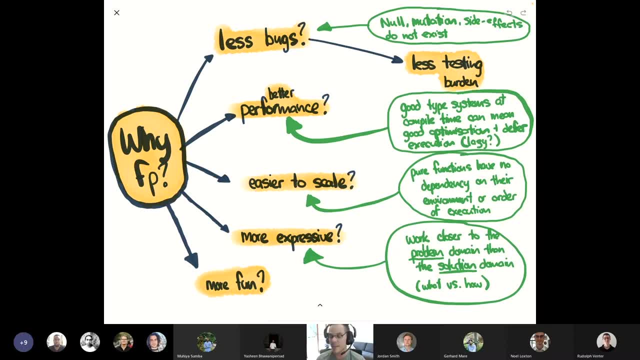 And so the idea of that is like: is this idea of this concept of laziness? So if you write a program that does a whole bunch of stuff And you never print the output, your program may never need to get that, never need to like run that calculation because you never used it. 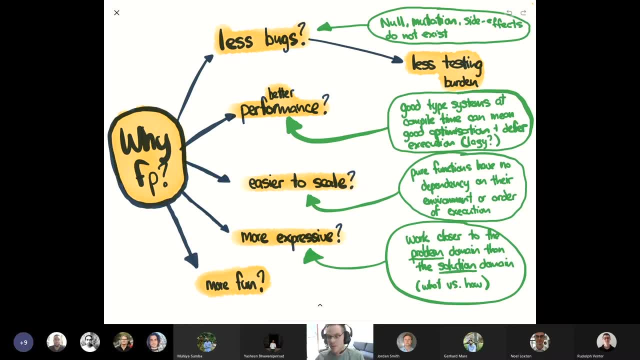 So like, why would it even go and fetch it right Or calculate it? So functional languages or good strong type systems can sometimes be interesting because compilers can leverage them to find areas of optimization, which I think is pretty cool. 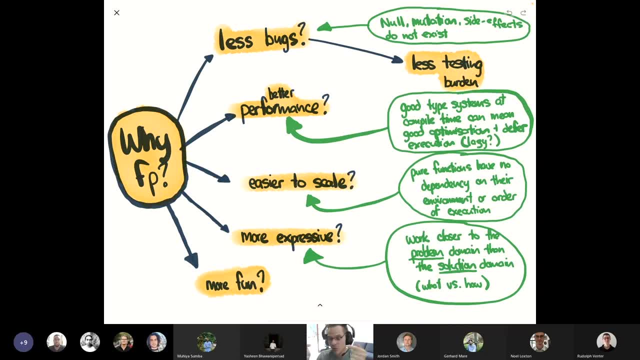 Whereas in imperative language it can't Like. the compiler just goes: cool, I'll do that, do that, then do this. It doesn't really know that the output of this One may not be used in the final result because of the, because of the purity concept. 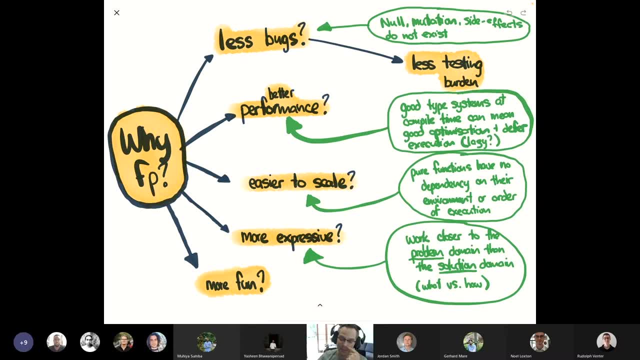 Actually, it doesn't know that calling this function doesn't make some external change somewhere, so it can't skip it because it just doesn't know that this is a pure function, Whereas a pure function you can skip it if you never need to use it, never need to use the result of it. 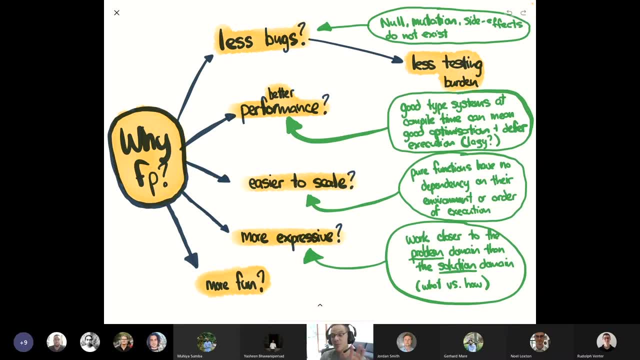 But like it's getting a little bit hand wavy, but but it's interesting and easier to scale potentially. Yes, this and this I have like real experience with, So as As like system architecture is becoming more and more distributed, and this is a big topic. guys like this is something I'm very passionate about is distributed computing. 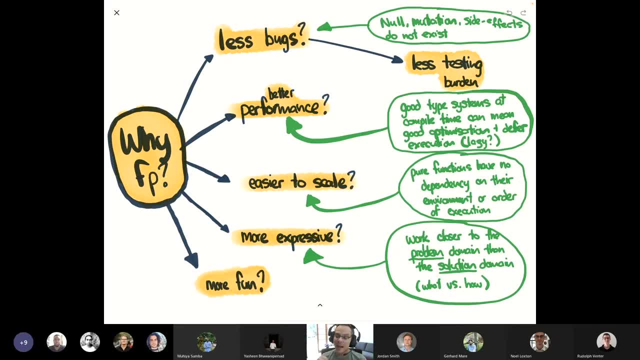 But like the more code that is now being run across many machines at the same time to achieve like a single task, the more you want more of a functional type of approach and I can dive into the detail of why that is, But it really comes down to like state and mutation. 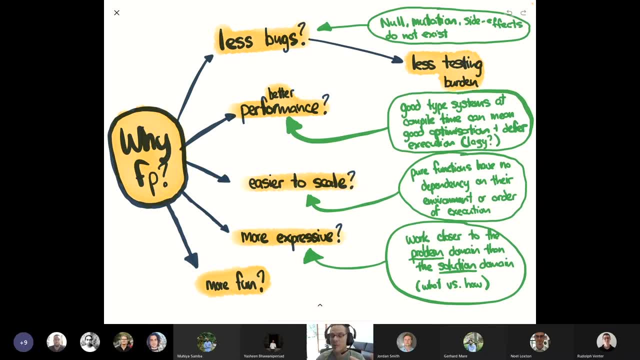 Where does state Live, et cetera. And functional styles are often a nicer style that allows the distributing of computation to more than one node, And so certainly at Synthesis- I mean, you guys know that we do a lot of AWS cloud and we build microservices and we use Kubernetes and and we like that kind of stuff- 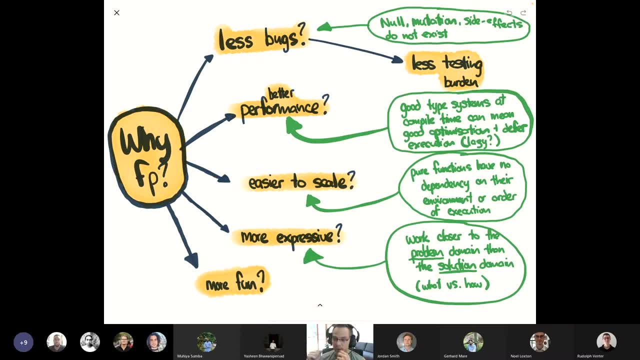 So like, of course, a lot of our architectures are distributed, And so you have to think about how does this code run across potentially many machines in order to solve a problem? And I think that the fourth point is more expressive. so maybe it is more expressive, I don't know, and this was that earlier point, I think, made by Yashin. I hope I'm pronouncing that right, Yashin- that you, working closer to you, are writing code that is closer to the problem domain more than the solution domain and that speaks to the what. so you know, your problem domain is generally a what problem and your solution domain is more of a how, how am I solving this thing? what is the problem and how am I solving it? 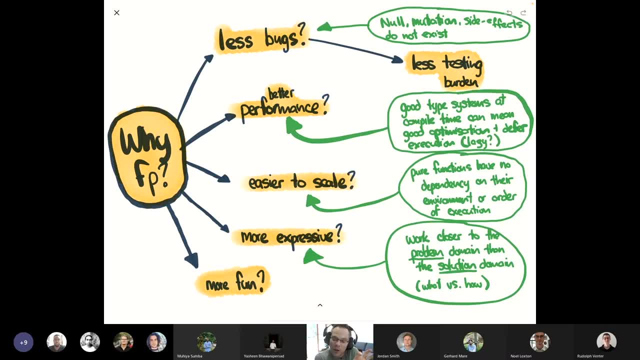 Well, that's a good question. With functional programming, you, you feel like you're closer to that, what so? you're writing code that's more about describing the problem rather than describing how you would solve the problem, if that makes sense. you almost let the language and the compiler solve the problem for you, just through reduction, just reduced to the solution, if that makes sense, like let the compiler figure out the best way to do this, which is interesting, a very broad point, but- and so it's definitely not absolute- but it feels like you're closer to the problem. 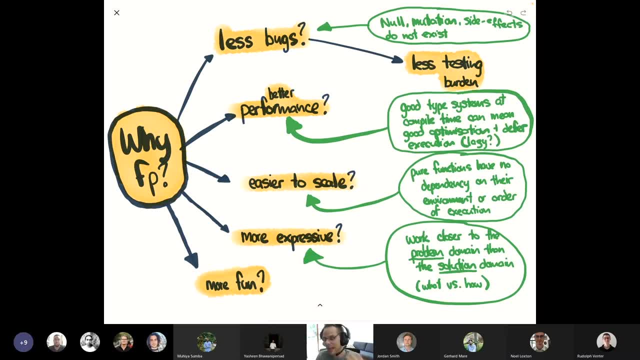 And maybe it's more fun, Like I, I would say I love like, I love the. I love the idea of, of, like, of continuous learning, right. So for me, when I, when I use functional languages, I always feel like geez, like I know nothing. 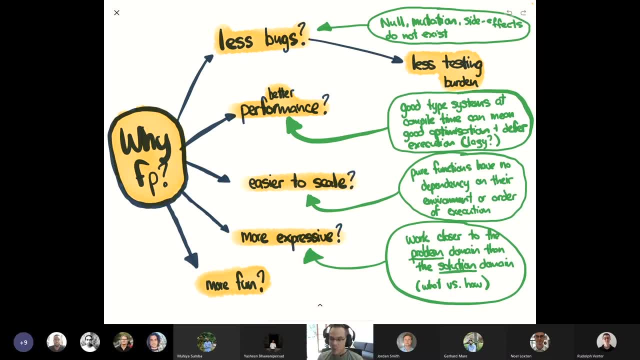 I, like I'm starting, these concepts are like, whereas when I, when I jump into my old, familiar languages like C, C++, C, sharp Java, even JavaScript, Python, where it's like these are simple languages, man, they're easy. 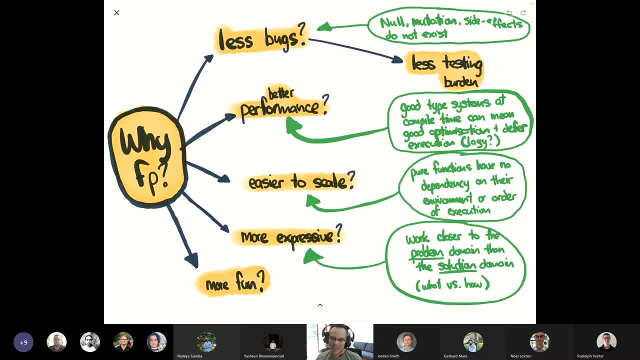 There's like There's not much to it, if that makes sense, whereas functional languages often have got these like interesting wrapped up things around category theory and like there's this whole like interesting academic environment around functional programming, which I always feel like for me is like wow, so awesome, like I'm learning so much as I go through it and for me, like that's important, like I think when you write in code, who would want to get good at the language that they use and then use that for the rest of their lives? like not for me. like for me, I'm always looking at like 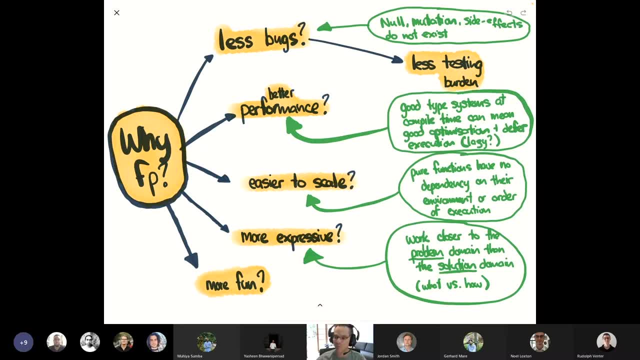 like: how can I improve my skills or know more about this domain or figure out better ways of solving stuff? and sometimes like: don't limit yourself to the constraints of a single language or a single paradigm. right, if that makes sense. 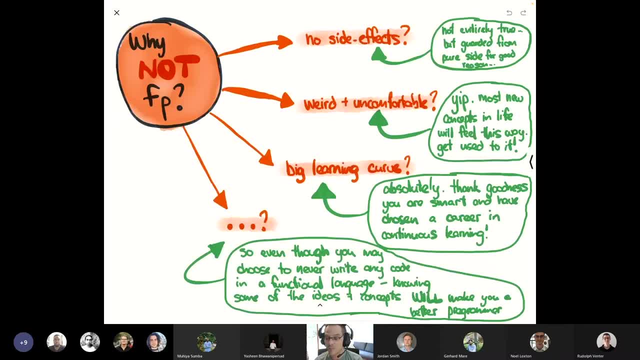 So so these are some of my whys. I also put a why not? because there's absolutely like, why not? functional programming, for sure, and- and these are just some of the ones I could think of- so like no side effects. so like, wow, if we can't write functions that change the state of the world or read the 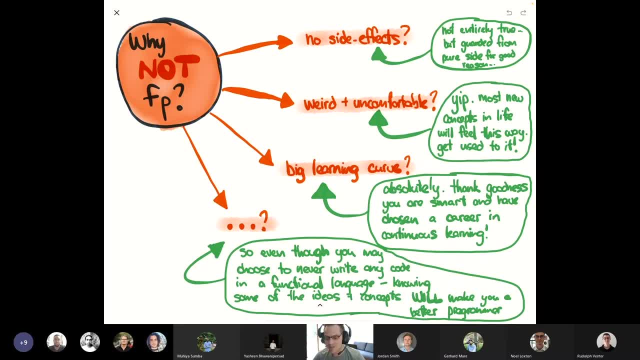 world. like how useless is that? right, I write programs that want to do stuff, right, and if you're telling me I can't write to files or read files or talk to the network or talk to the internet or whatever, like that's pretty useless. that's like very limited to, like, the mathematical proof domain, right. and so, yes, yeah, functional programs, like pure functional programs, don't want side effects. but it's not entirely true, of course they do. they just wrap them into, like into a special holder for those side effects, which makes life more difficult, for sure. 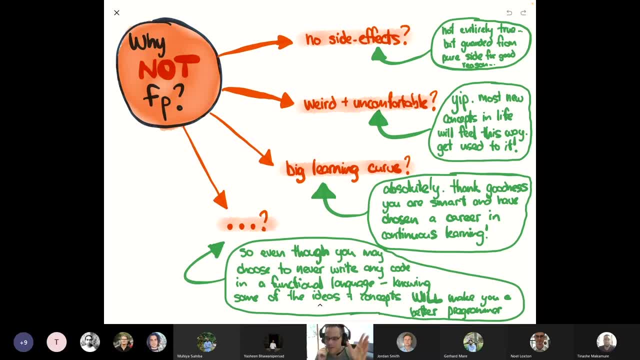 But it isolates you from those changes and we may look at something there like the second point, and this is probably the real reason that why not to use functional programming? and it's like, it's weird and uncomfortable, right? so so we might look at some functional stuff later and you'll go like, geez, that's weird, and and- and hopefully you don't, because maybe you haven't written enough code for your, for your like brain neurons to like harden up too much, and you'll look at it and go like 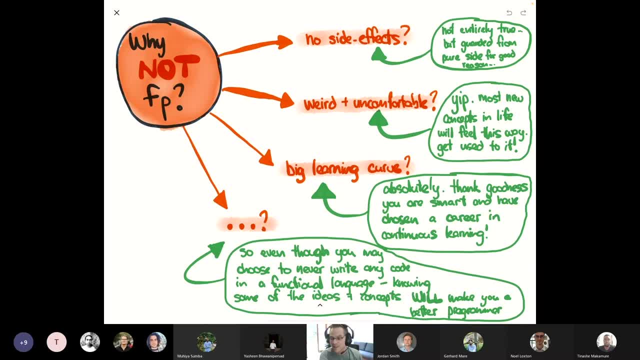 no, actually, like this totally makes sense to me, but I think if you've written it and for me like I'd written 10 years of imperative code by the time I started to go, yeah, this sucks, like I think there's a better world out there. it was weird and uncomfortable in the beginning, for sure. yeah, there's a big learning curve, absolutely, and and sometimes that learning curve is not around the language itself, but sometimes it's those underlying patterns and and constructs that sometimes are in the functional programming world, are like a little bit academic. 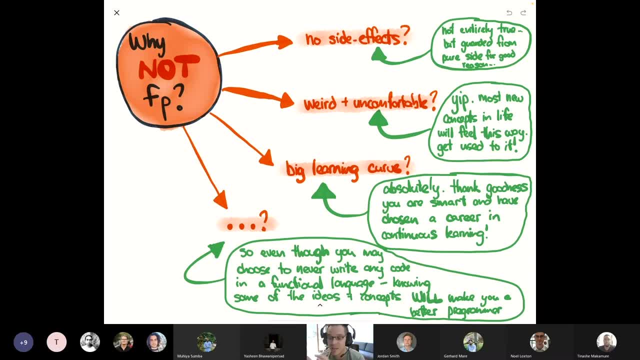 so category theory is, and things like monads and endofunctors and functors even, and monoids and semirings and semigroups like these are words that often are used to build up patterns in functional programming and and it's, and although I think you can be productive without knowing what is a monad, what is a monoid, what is a semiring, these kinds of things, it's like if you, if you want to move into that mastery side, you kind of have to go there. 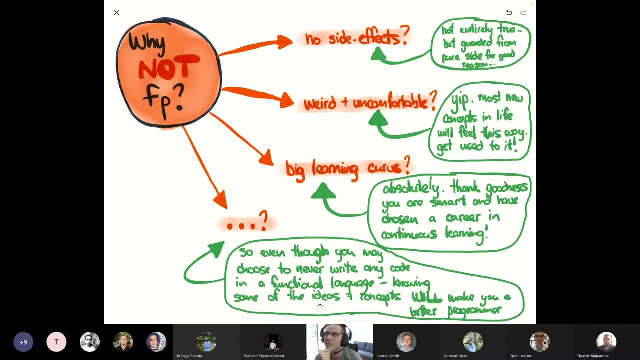 if that makes sense, whereas you- whereas you don't really have these- a sort of similarity in imperative languages. maybe the most similar thing is like design patterns in imperative programming, maybe things like the visitor pattern, and I'm not sure if you guys studied any design patterns at university or or like aware of these things, I don't know, but maybe that's the kind of similar, similar kind of thing in imperative is design patterns. so they're just different. and and so the last point is like many other. 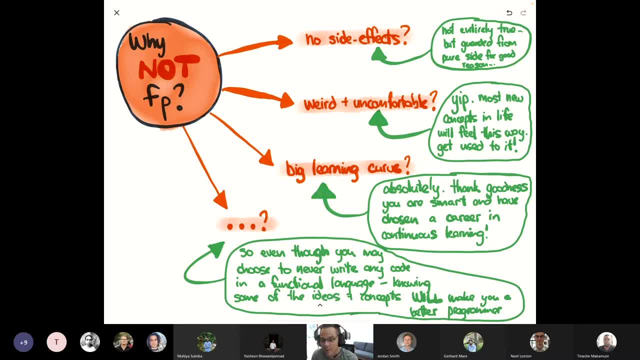 there's like lots of good reasons to not want to use functional programming. one of the big ones is like skills. maybe you know so if you're working on a big project with a bunch of other people and and you wanted to do it in a functional programming language or write it very much in a functional way, or whatever, one of the downsides is like you may not have friends on your team that support that idea, you know, because they they have a particular skill set and they want to be productive, and so there's a learning curve that 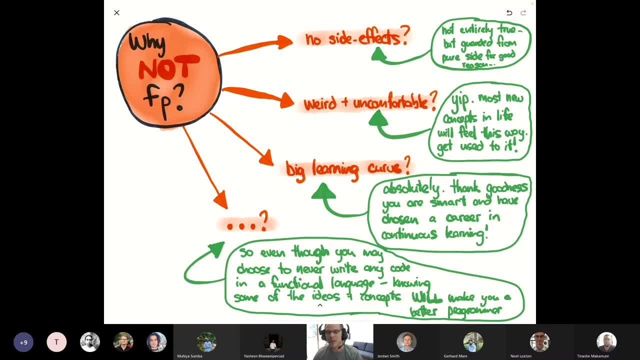 you know the entire team has to go, go through etc. etc. I mean there's many good reasons but in in my view it's not. none of these are good reason to not understand functional programming or under understand some of the benefits that that you can get from understanding functional programming. it's still absolutely worth going and learning and playing and and figuring these things out, because those ideas completely transport themselves into almost every other language and I think I've got like a a. 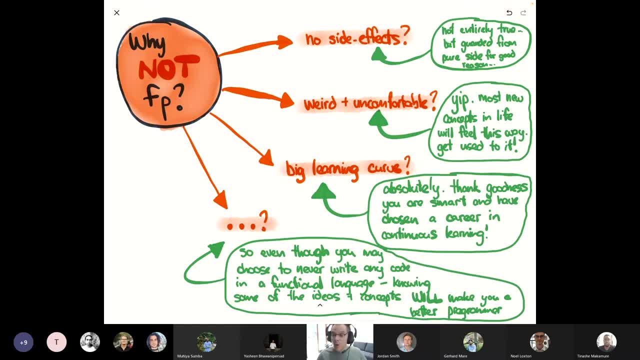 kind of list of languages, and most languages today are becoming more and more functional. you'll totally see this. so it's. it's not a like wasted exercise. you will be a better programmer if you can think about things in a functional way even though you're using an imperative language 100%. and we're all smart people. we're all like, like you know, we've committed ourselves to a career of continuous learning, so, like, brilliant, this is something. this is something. one of those cool topics- oh cool yeah. 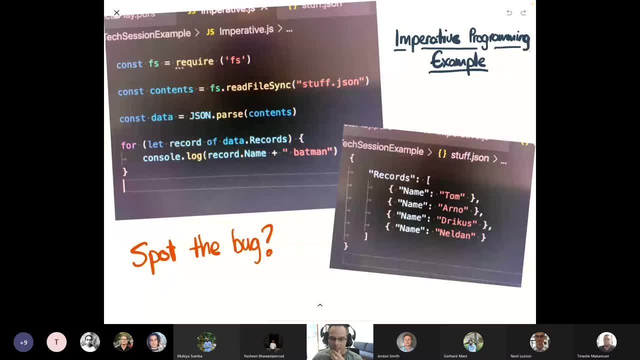 yeah, okay. so here's a cool example of some code and actually like we might live code some of this stuff to make it fixed. but can anyone see? so we've got code there on the left. this is JavaScript and it doesn't really matter whether you know JavaScript or not, I don't really care. it looks like it's pretty simple to understand. and here's that file, stuffjson, so you can see it does like a read file. sync of that file does it? can anyone see a bug here? 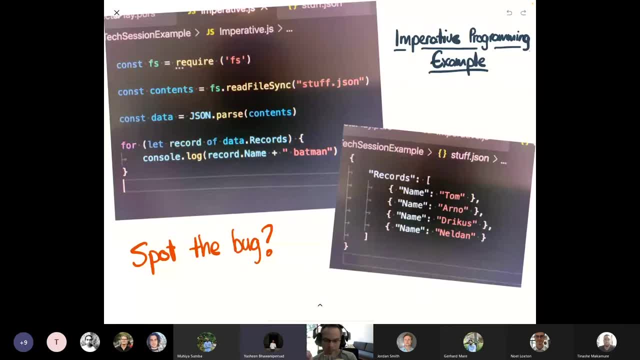 I think the problem is going to be that stuffjson file. yeah, what if that file does not exist? so what am I going to return back to the front like what am I doing with it? I like it, that's. that's a good first bug. any other bugs? 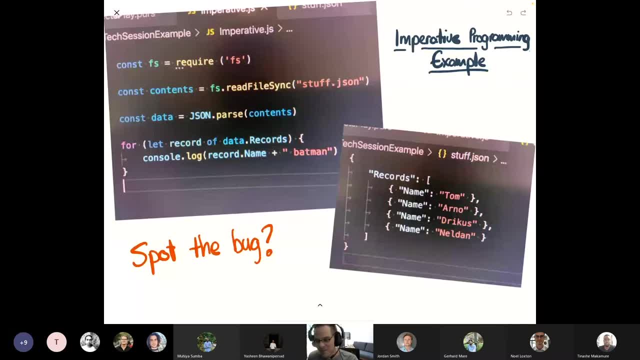 No, I think I've got four bugs. I think I can see four bugs. Yeah, so I can. I can tell you when you run this code. it works. yes, but like Yashin- I think it was you who said what if the file doesn't exist, and that's very good, I would say that's a bug, right? even though it does exist today, how do we know it doesn't exist tomorrow, right? 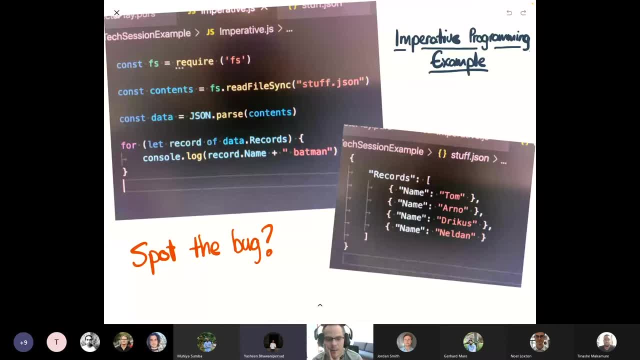 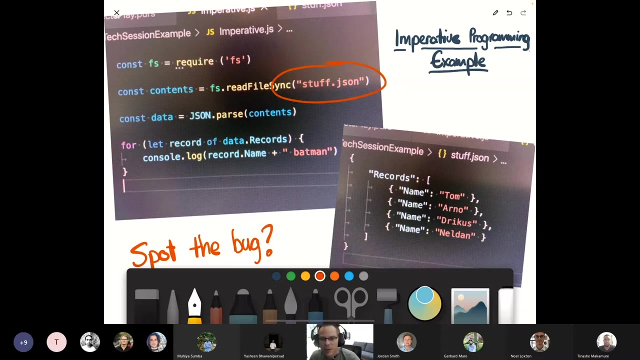 And also that array, the record array inside data. yeah, we don't know, even right onto the attributes, the recordname for each one, for each object in that array. Yeah, yeah, yeah, yeah, exactly like this code is terrible, so it probably works, but there's so many ways it can break, right, because it's like so dependent on this file, right, so we can see. I don't know if I can point. yes, I probably can point, so I can see. like here's the first. oh, I'm using the wrong tool. let me use this, check this. so there's like the first issue: what if that file doesn't exist for sure? the second one is like we're going like 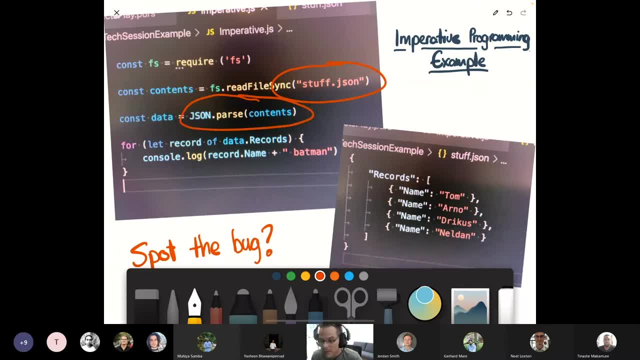 here we're making a big assumption that, like it's JSON, right that it's in a JSON format. what if it's not JSON format? right, and we go JSONparse contents. so like, contents is just a string there, right? so we know that this thing will read like a buffer, a buffer of the contents of the file. it doesn't make any assumptions about. you know what is the format of it's- just like a big string. so in JSONparse we pass it, the string, but we hope that it comes back with like a JavaScript object there, right? and what if it isn't JSON? so that's. 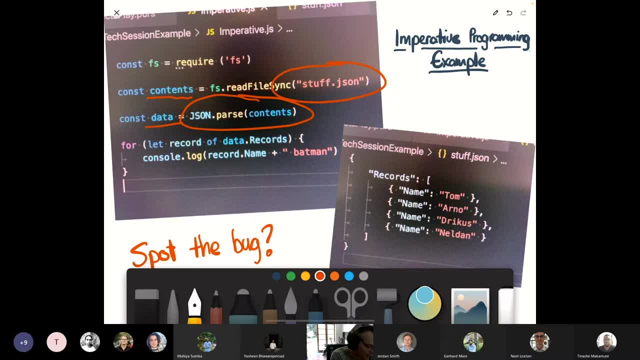 potentially another place it could break. then your, your. your second point was: like we also make a huge assumption that the JSON that so, even though it is JSON, how do we know that it's got an iteratable thing called records that we can for loop over? so that's a third assumption. and then the fourth one is: like we also make for each of those records, we assume that there is a dot name on that thing and we can, and we know. when we look at the file we go, yeah, it's fine, it is fine. but 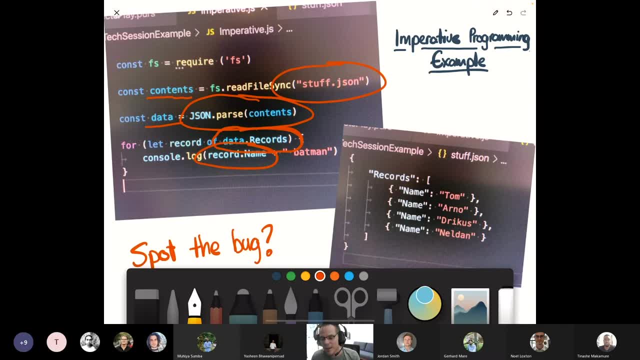 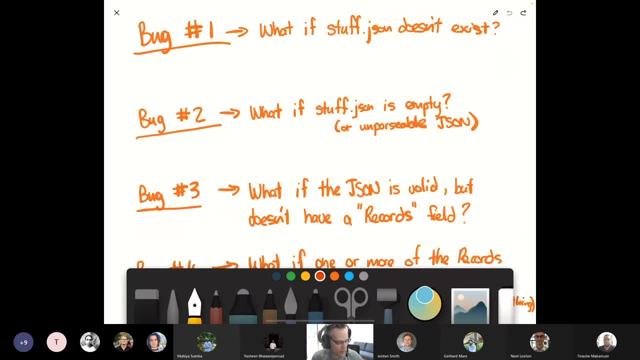 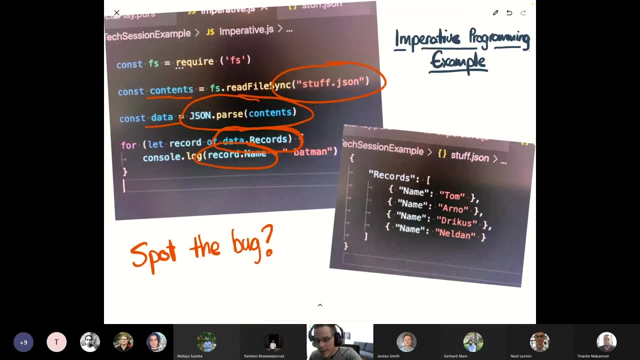 we've. we've made four huge assumptions here, all of which can lead to very interesting bugs, yeah, so I think, yeah, okay, cool. so I made a little list and these are those four, so I'm not going to go through them again. oh yeah, oh yeah, the last point was for bug number four, that last assumption. we may, we? what about the types? so here we're. you know, we're going consolelog of something and we're assuming it's a string, but what if it's an integer? or what if records is actually an object and not an array we can't loop through? 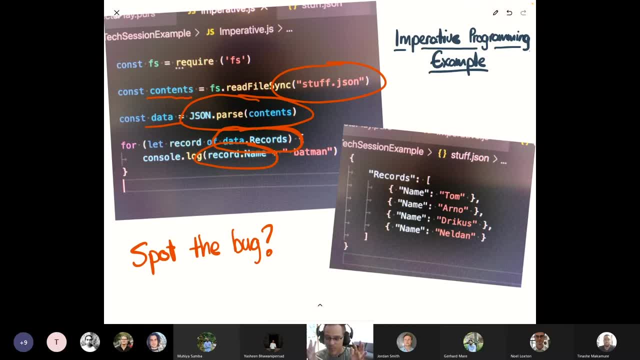 an object or what if records is a string or like it's broken, like everywhere. it's like there's so many bugs and all we've written is like one, two, three, four, five lines of code and in fact we've got more than five bugs in in those things, right. the only like non-buggy part is probably that first line where we say, hey, we're going to use the file system, and probably that could break too, actually, if we haven't got an npm install or I don't know if we have some dependency, who knows? so there's at least four bugs, so I think my next 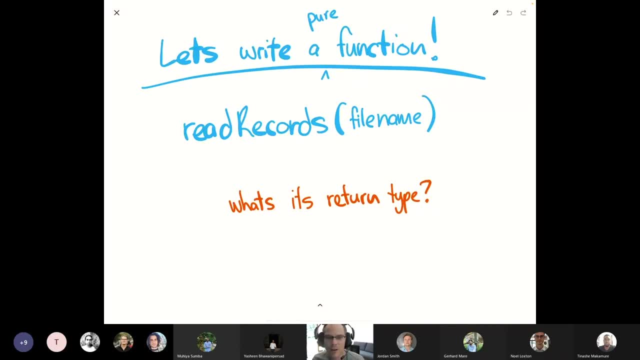 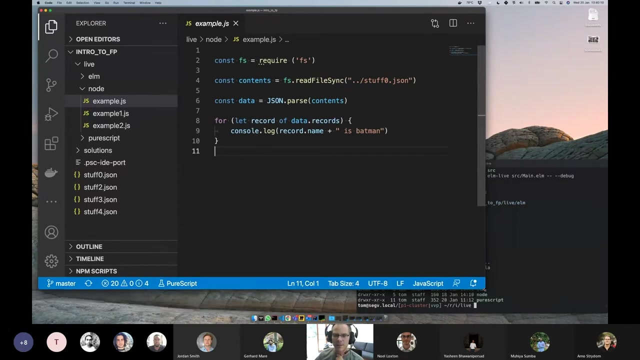 oh yeah, okay. so I'm going to switch now. so let's try and write, let's try and like: fix this code right and I need your help. so what am I going to do? I'm going to take control. I'm going to share my screen from here now, okay, so, okay. so you can see this Visual Studio code thingy here. right, some code here, yes, yes, okay, good, all right, let's see if it actually works. 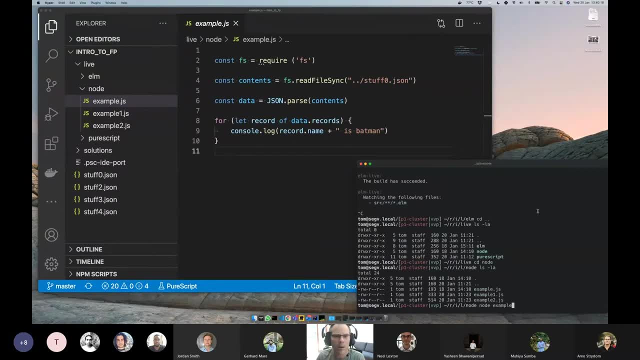 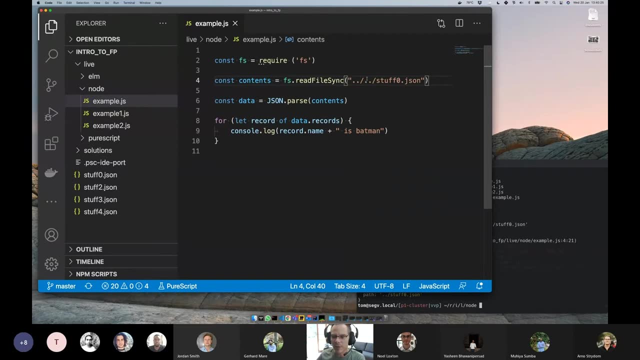 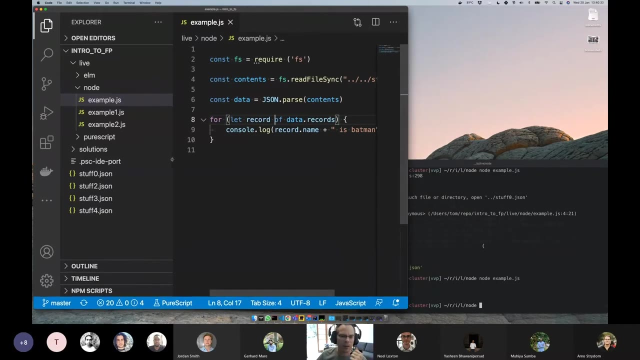 so this is written in JavaScript, and if we go node example- I think it's just called example- it can't open this file. yes, because I moved it. I cleverly broke everything this morning. yeah there, okay, cool, so that works. so. so what we've got is, you know. so here's that original. 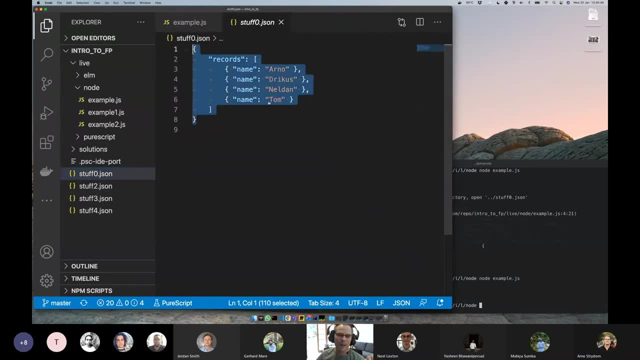 file, right stuff, zero, and- and this was the same as that example we saw- and then I've created. so, first of all, I've created a new file and I've created a new file and I've created a new file. 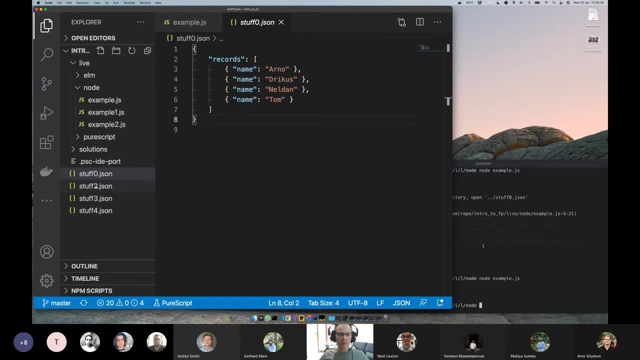 so first of all, stuff one dot JSON doesn't exist, and so that's good, that's a good test. stuff two has got bad JSON in that file. stuff three has like put an exclamation mark there. stuff four has like changed the type, so like. here's a couple of good examples of like broken files. 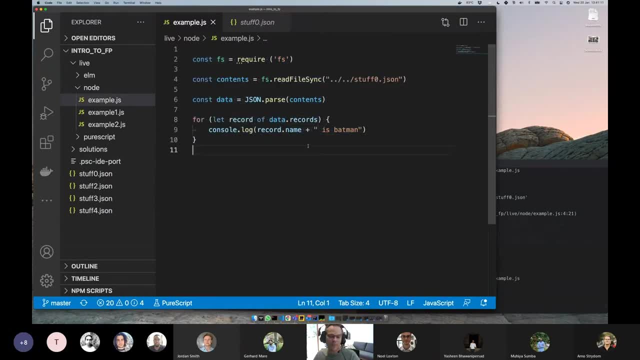 that could. so. so we look at this code and we go, yeah, this is good code, looks fine, seems to work, but there's many ways that we've just talked about that that they can potentially break it. so so, like, how would we like write this more? 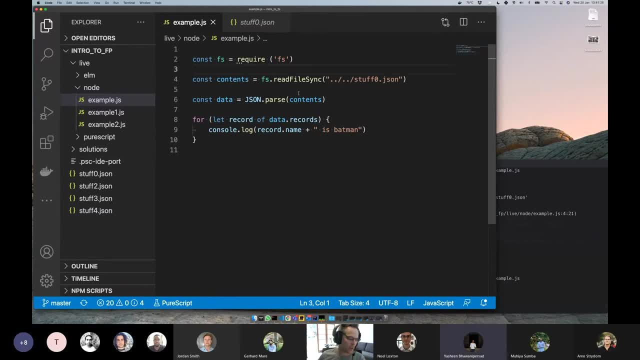 more safe, I suppose, and so so we're in JavaScript, so probably so. so we want to write a function, probably. I mean, this was my idea. it was like maybe we want a function called like read records, right, or something like that, and I suppose we want to write this. 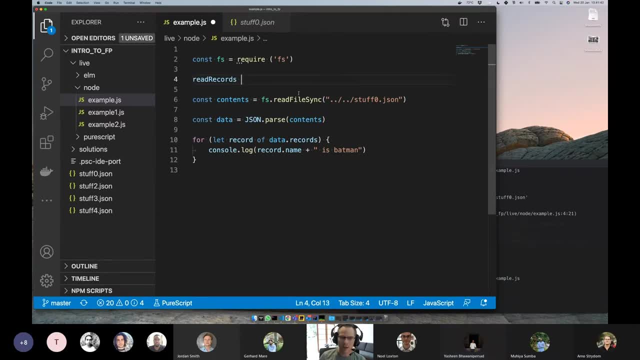 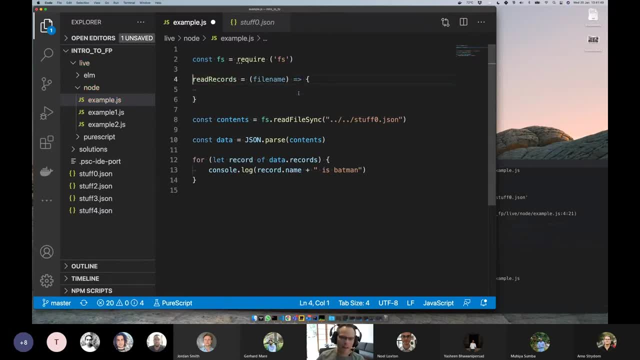 ways of doing it. you could write it like an arrow function like that, and maybe you want to say this is a const, so that's a function called read records, which is a function. but you could also write it like function read records, taking a file name, and maybe that that's probably safer. 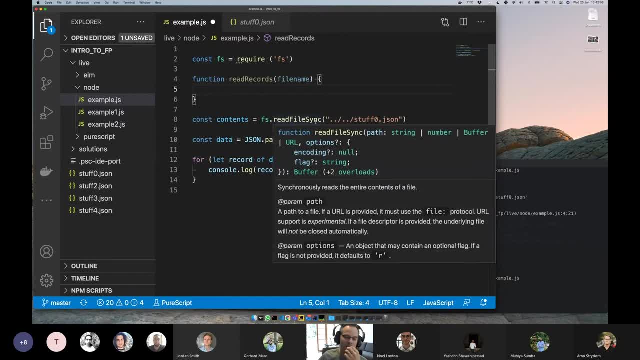 right, so so we'll go with that one. well, it's not safer, it probably just looks looks a bit better, and so probably what we want to do is like, like, let's lift these things up into this. 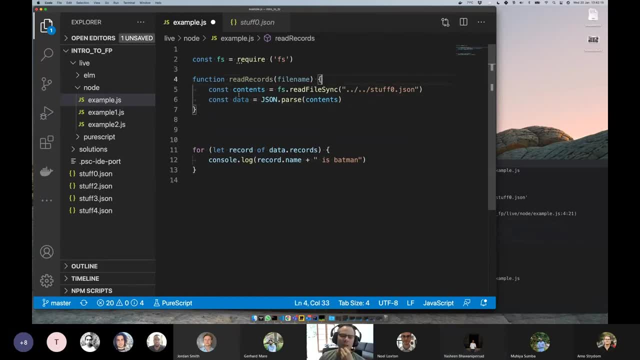 thing. so. so the first question that that I got for you here is if this thing was, was was strongly typed, and and so you know, if you consider that in in C-sharp or Java, you might say this is a function which returns like an. 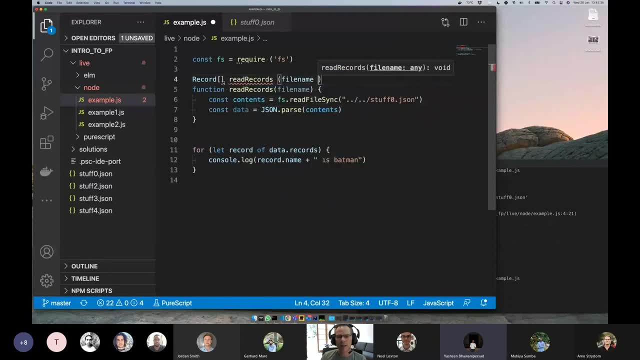 array of record or something: read records, file name, which is a string, right? so I'm trying to think of like, like, what is the signature of this function? read records, right, and and, and. so the answer is what I mean? what? what should read records return? any idea? 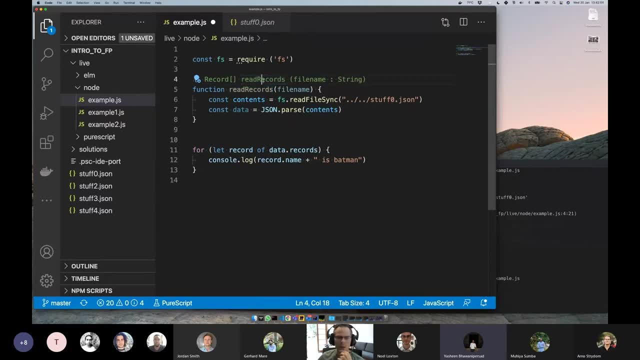 I would say it could return a string array or in any array which you can use to build. you can build a constant every time I plug it inside, or you can just slower, slower, okay. so I'm saying you can return a string array to get all the data inside the JSON file. 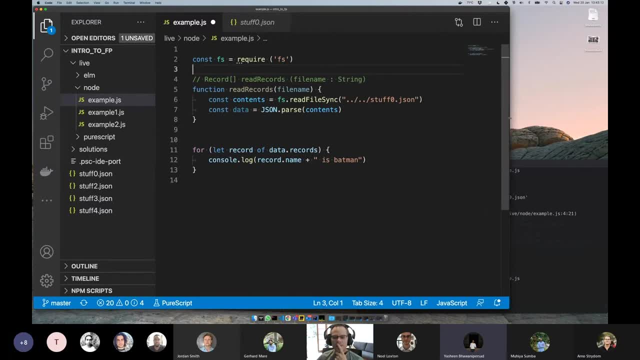 assuming it does exist. yes, I would say in TypeScript I could have done like return a in any array you know and plug that inside. but yeah, Yeah, and, and so I suppose that I mean. 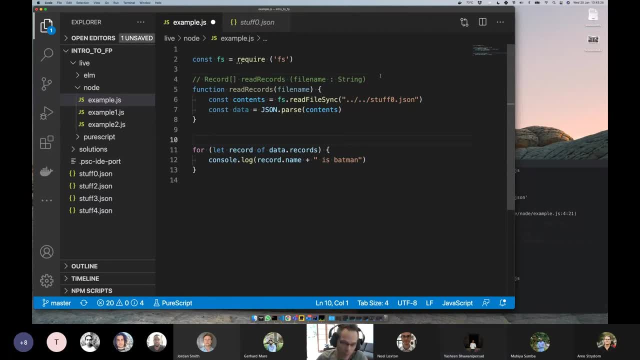 of course we could return whatever we want. right, it's JavaScript, and we could return strings sometimes and ints sometimes, and that's fine. it's all dynamic, but from a caller perspective. so a person making use of read records- right, what is he going to assume that he's? 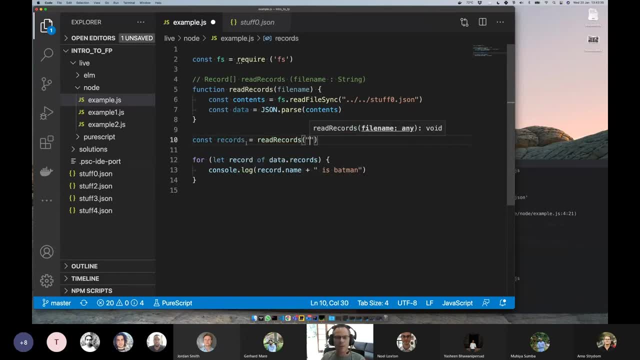 getting He's going to go. const records equals read records from you. know this file or whatever. What do you think when he's reading this code he thinks read records is going to return him. I suppose is the question. 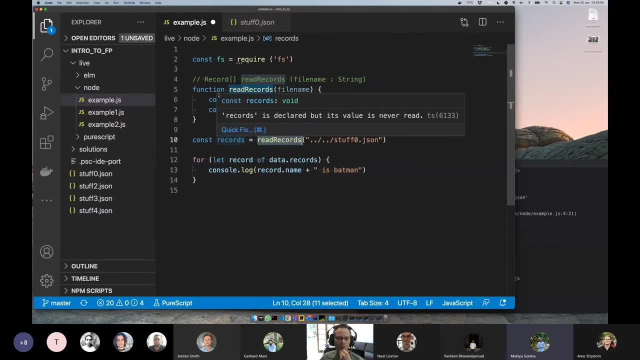 A string array, because you read data: An array of strings, yeah, yeah, so that would make sense. it would be these, these as strings. right, an array of strings. yeah, totally, so I I would say that like that seems fine, so I would go like: yeah, I think it's like a string array. 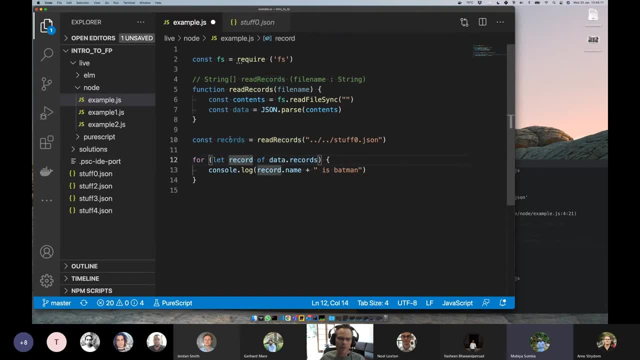 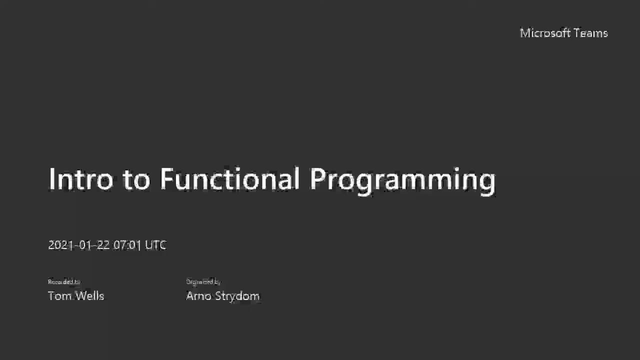 being returned by this thing, and then I'll go that record of records, their log records, something like that, right Set up. so thank you for joining this meeting, obviously. thank you very much, Tom again for. 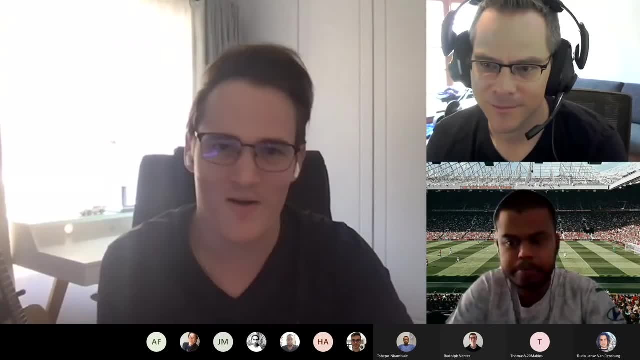 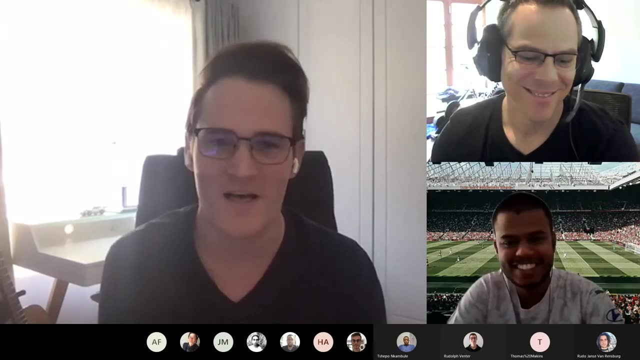 your time. we really appreciate it and look forward to the session. Last time it was interrupted by some load shedding, but I think this session number two is, like I said in the invite, it's said to be a lot more mind-bending. 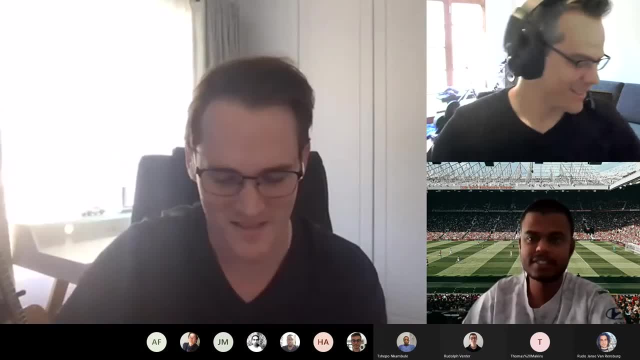 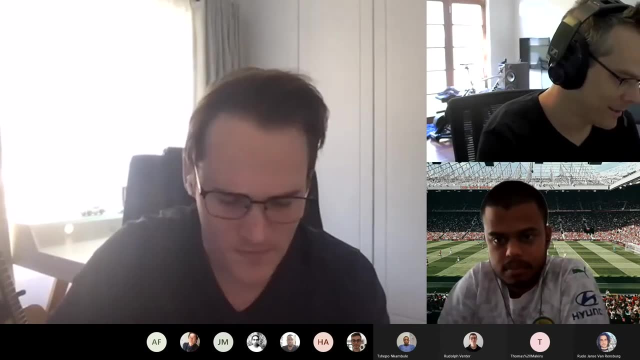 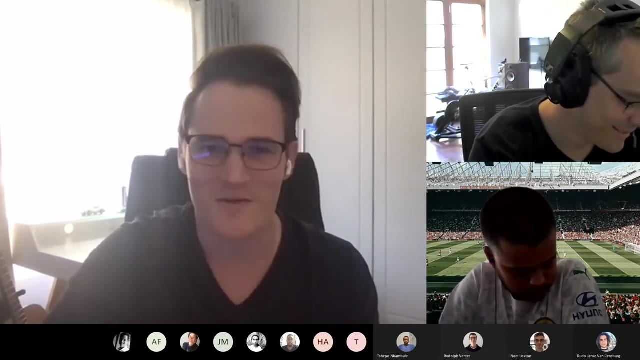 than even the first one was which, which is a tough one but it's. it's going to be very interesting. so just to give everybody a recap on last time, maybe if you went on the call, we discussed essentially just looking at Tom's life story and his 20 years of working as a 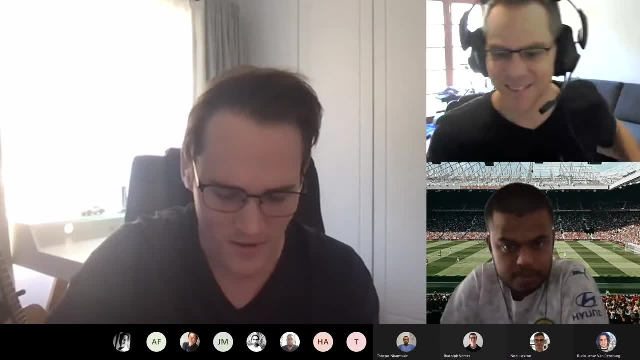 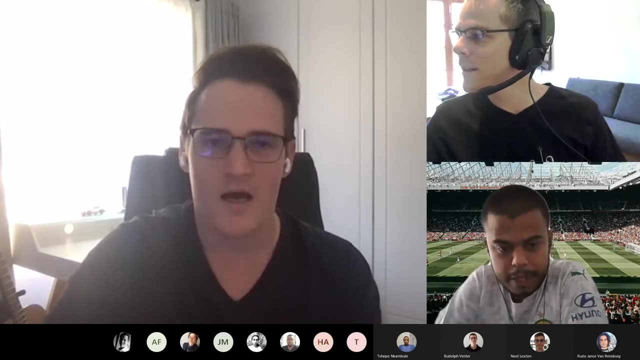 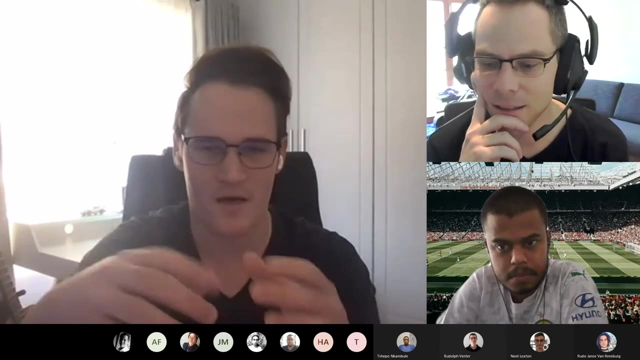 software developer and just gave a bit of insight on some of the stuff that he worked on. and then we started looking at functional programming- just essentially why you would use it or why not, and I did a bit of a comparison on functional versus imperative. and then we started having a test program to have a look at. 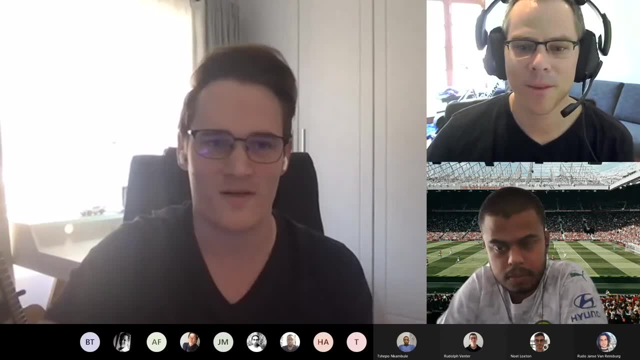 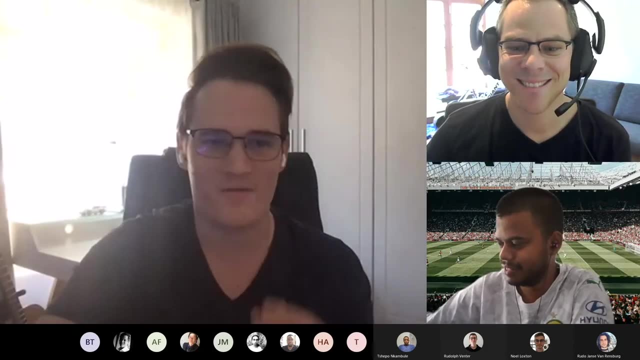 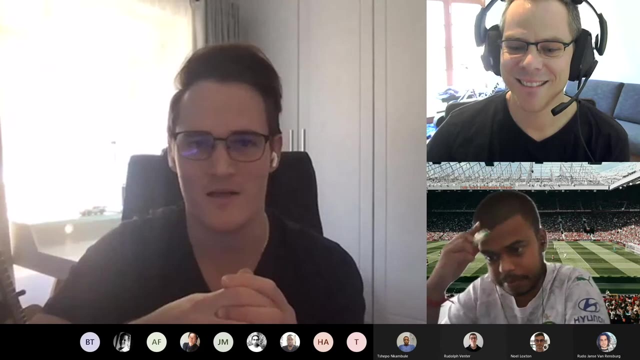 how the functional programming works. so essentially that was a file with four different JSON names where we wanted to add Batman to the end of them and we had sort of a spot mistake to see like four different issues that might occur or bugs that might arise from. actually, 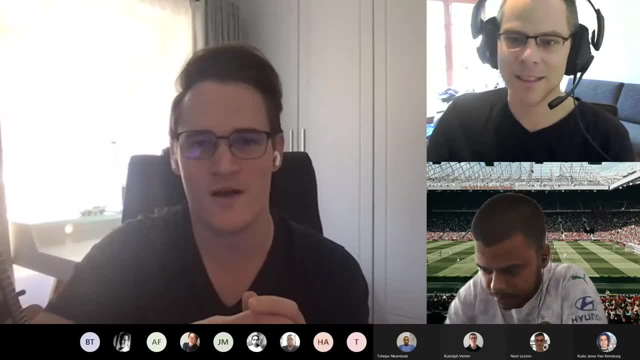 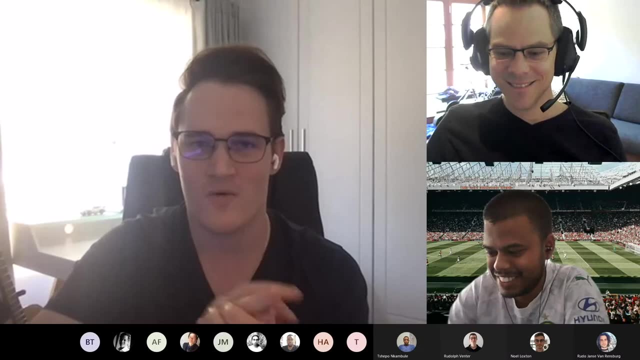 the way that it was currently set up, which was, I think, five lines of code and four, and it was like essentially having the file is not existing either or the data inside it is incorrect. maybe it's JSON, maybe it's XML. some sort of other data structure could have been with. 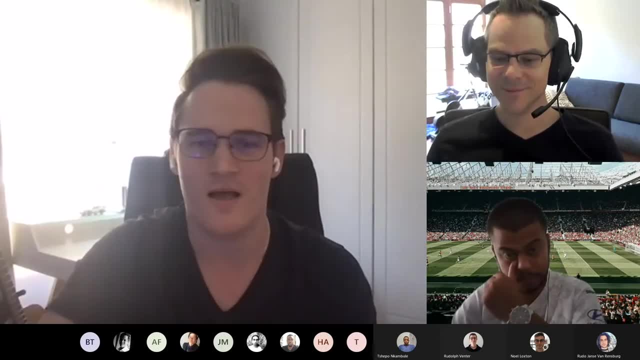 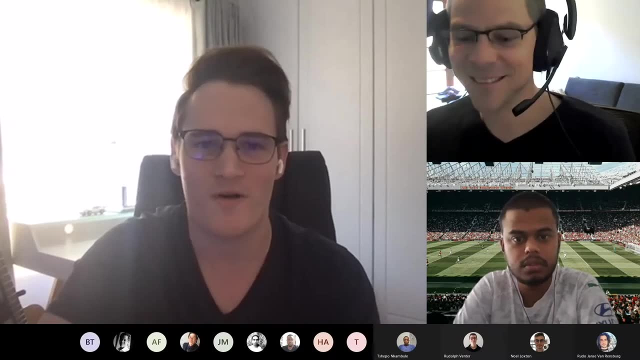 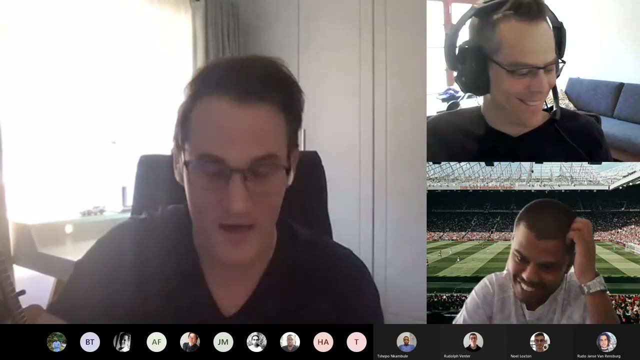 the types. there's a lot of different things, so we essentially talked about that and we were just set to actually make the program better and essentially write it in a more functional way with some pure functions. and then electricity outage hit us and yeah so. 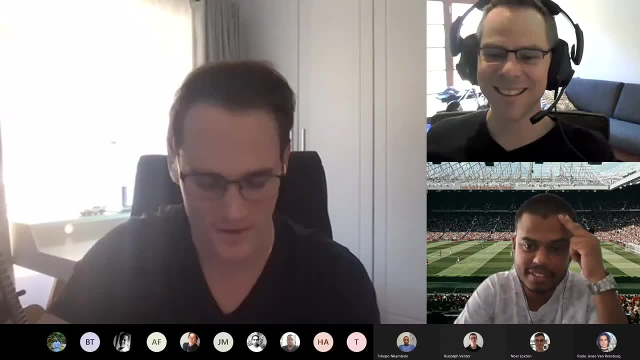 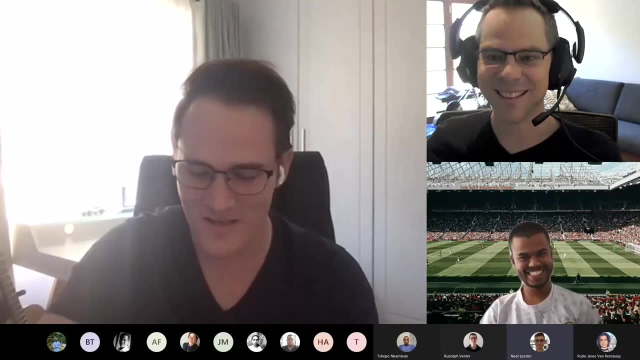 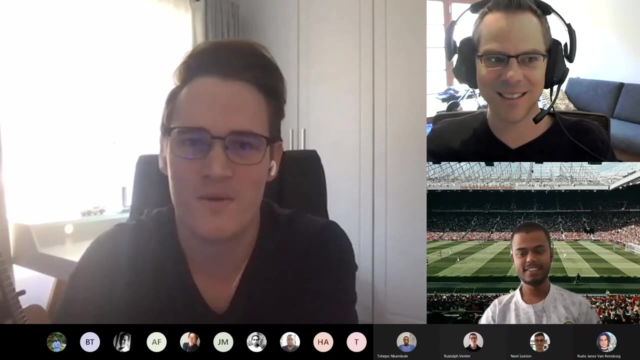 actually the sad part is that it ended up with a very bad dad joke. so thank you for that. we really appreciate it. yeah, so actually, yeah, just to mention that this meeting, this meeting will be recorded. so there's a few people that said they wouldn't be able to attend. 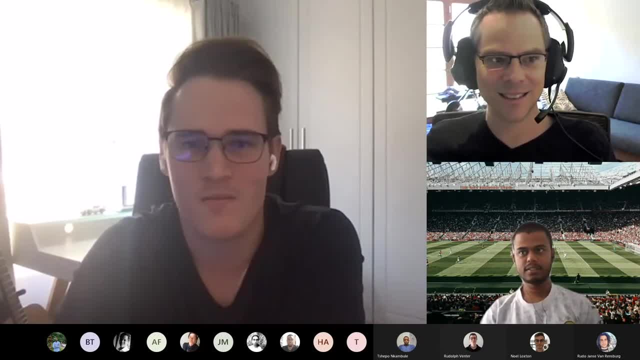 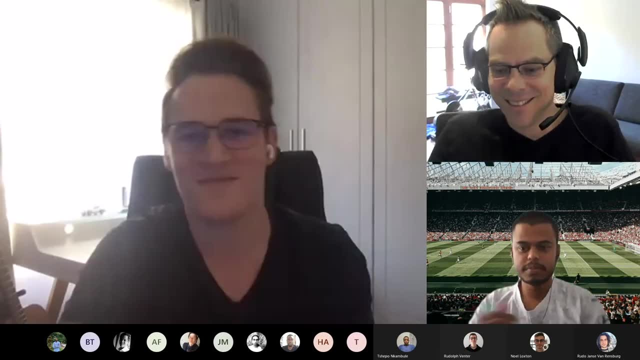 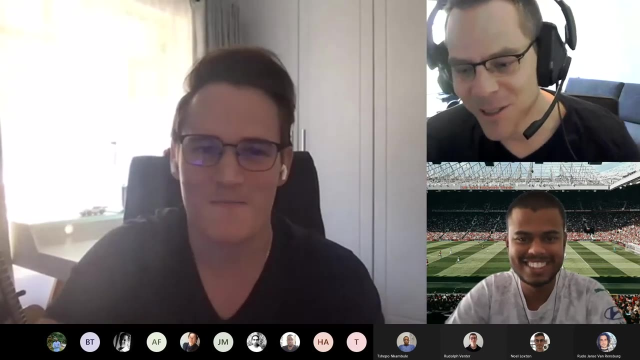 so we're just recording it and we're gonna maybe share it later for them or maybe upload it on the SharePoint or something. yeah, so yeah, without any further ado, Tom, you can take us away. Yeah, that's awesome man. thanks, Ono. I missed the dad joke, unfortunately, because I had no. 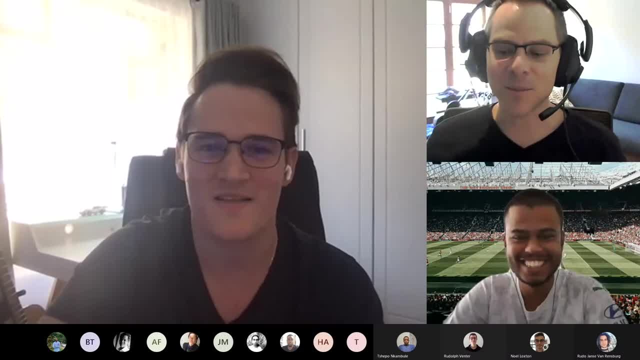 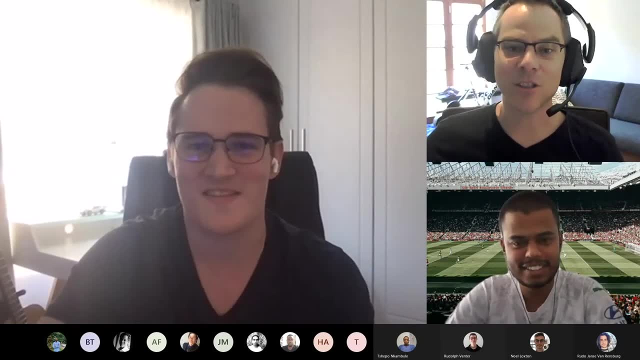 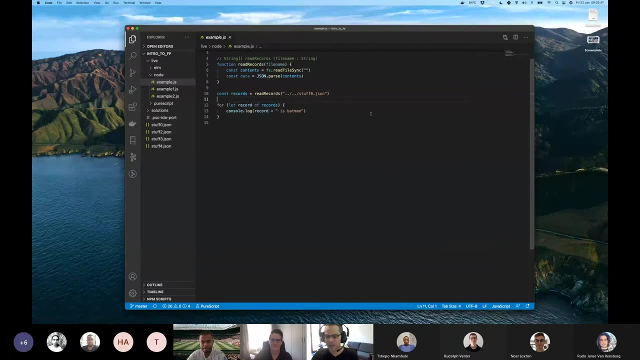 powers back and you said we're gonna make the program better. I think we're gonna make it worse first before we maybe make it better, but let's see how we go. so wait, I've got to share my screen. let's just do that. there we go, and hopefully that is visible. yeah. 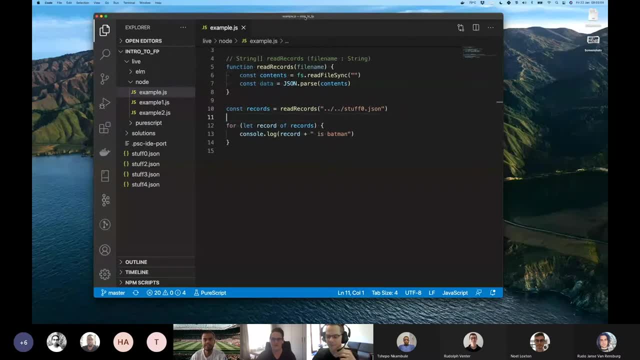 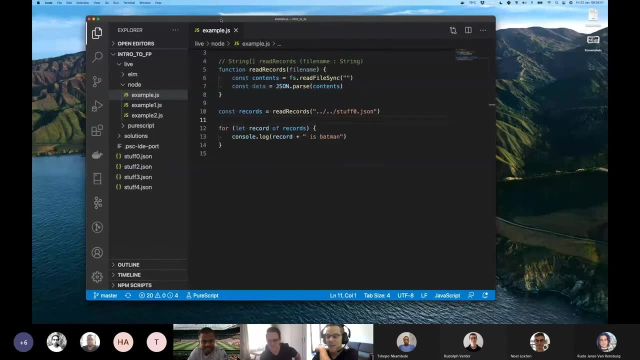 yeah, you can see. yes, oh, yay, okay, good, all right, let's hope for less issues than last time. so I'm just gonna dive right in Ono. great summary. thank you for catching us up. 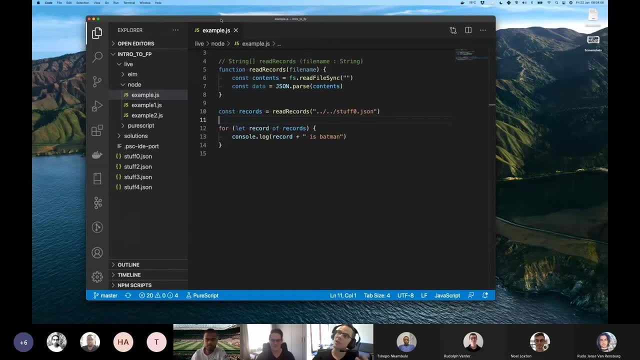 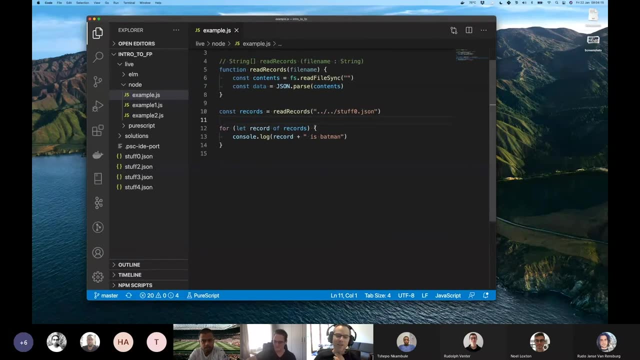 and maybe I thought we could. maybe I've got the first video, the first part of the video, and now we'll make a second part. maybe we'll glue them together anyway. okay, so we were doing this. so we said, cool, we had an earlier version which we now destroyed, so we're gonna. 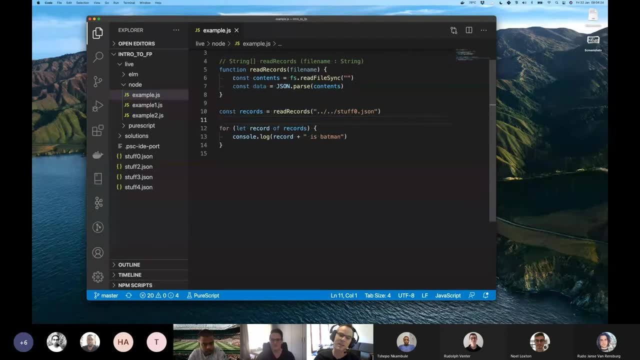 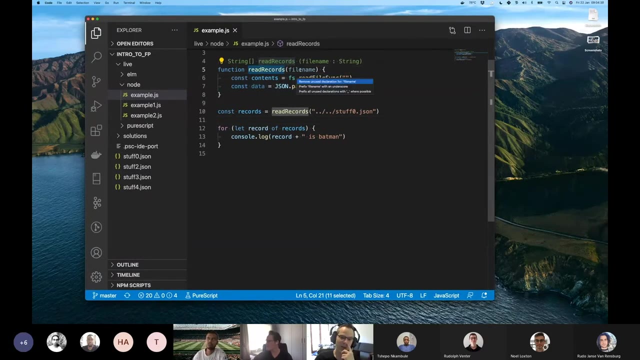 we don't remember what it looks like, but effectively, we are wanting to improve our five lines of codes, of code which was full of bugs, right, and so what we're going to do, I think, is like extract it into like a function called read records. we pass a file. 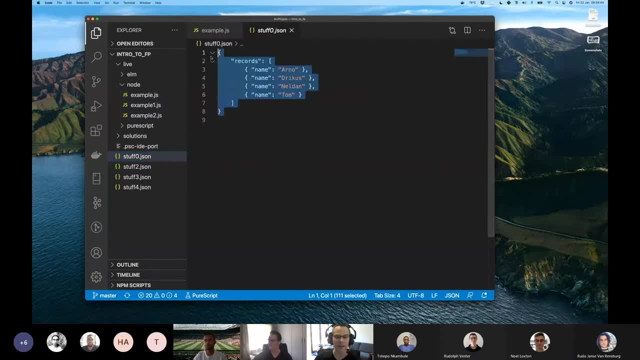 name to that function. it kind of makes sense and we want it to kind of give us back the, the contents of this file, possibly as like an array of strings of people's names, like that. you know, we're going to do that, and then we're going to do that, and then we're going to do that. 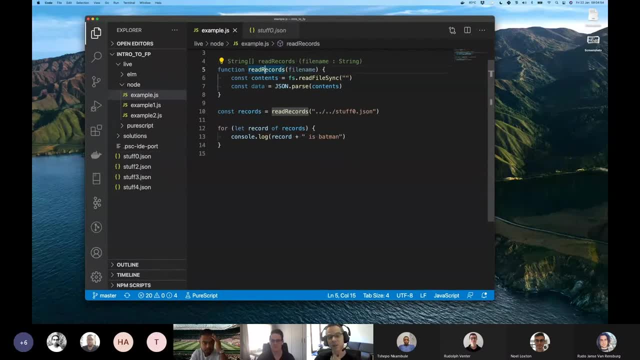 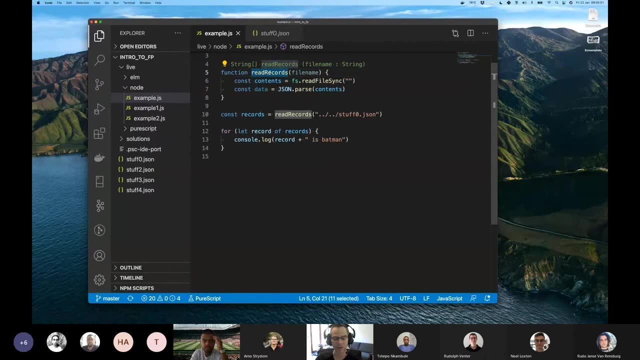 totally makes sense. we said, well, this is JavaScript, let's pretend it isn't, it's still important. it's still a good idea to think about, even when you're writing a function in JavaScript, to think about that. that functions like its signature, like what, what contract does it? 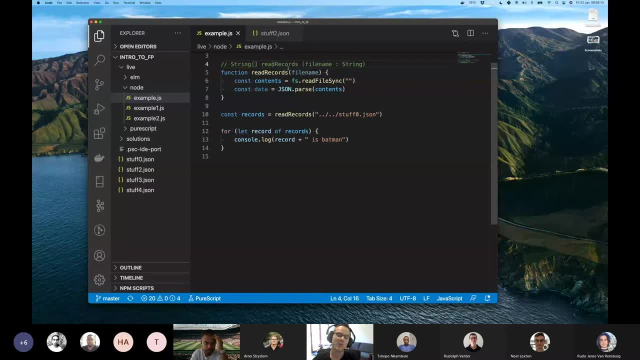 offer, I suppose to, to people using it right. so when, when the you know there's a, there's a huge separation between the stuff happening up here, above, above the you know, the you know. 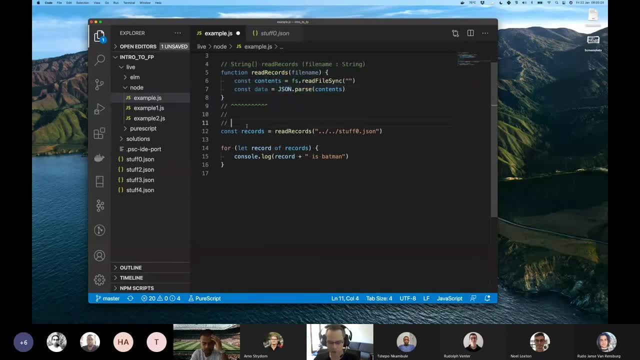 this is kind of like a library code down to here, which is where you know the, the, this is somebody making use of that library, right and? and it could be, although luckily you know we're. 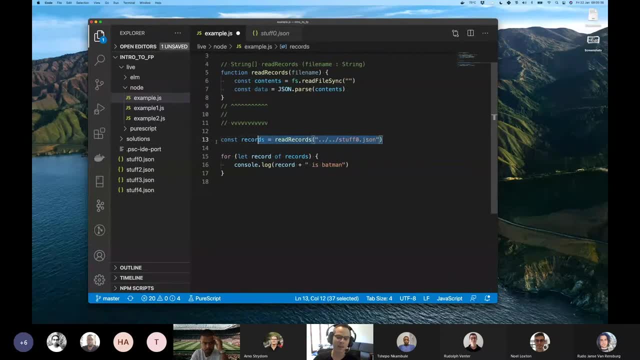 in a single file and I'm kind of one person, but you could imagine that this is a different person doing this to the person who's writing that up there. in fact, it could even be, you know, this could be someone, someone sitting on the other side of the world- you know who speaks a different. 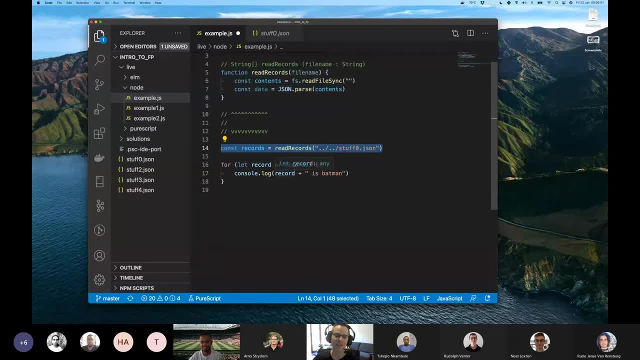 language, speaks German, whereas this is a person sitting in some kind of you know, a you know in South Africa who speaks English and they're making use of it. so it's always it, it's a good. 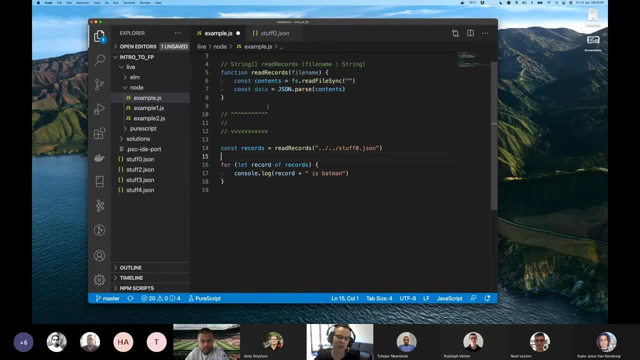 idea in your mind when you're writing functions or generally code is to write it for, for someone else, even though it may be primarily you using it. it just kind of gets you in a good habit of of writing better code, right and and also, like you know, from a from a temporal perspective. 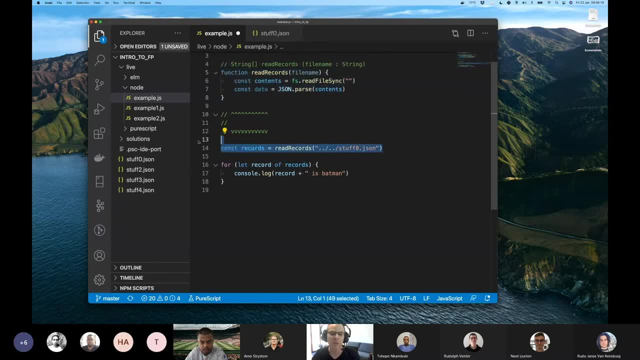 I may write this today and in 10 years, may want to use it right and like. my memory is totally gone and in fact I'm a completely different person, and so so what I was thinking, 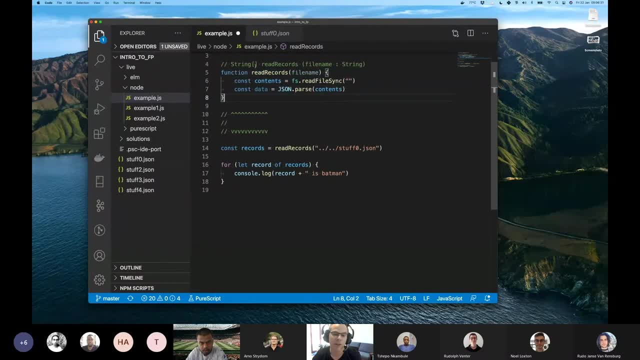 at the time when I wrote this is, you know, potentially completely gone. so it's important to think about functions with their signatures and- and some, you know, strongly typed languages would enforce that JavaScript doesn't, but it's still important, right? okay, so we're saying: 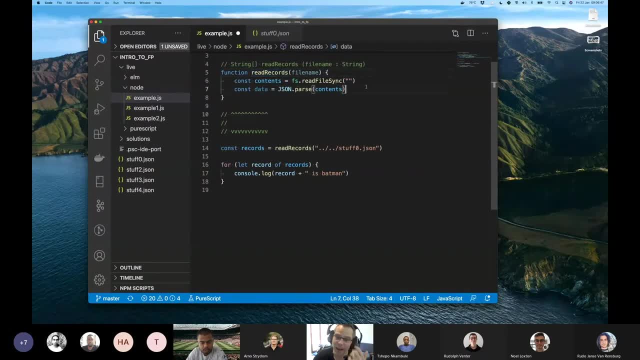 cool, it's going to return a list of strings, so here we go, right. so I suppose we could. you know, let's just lift this up here and I suppose we could just say, or like we're going to write it naively. 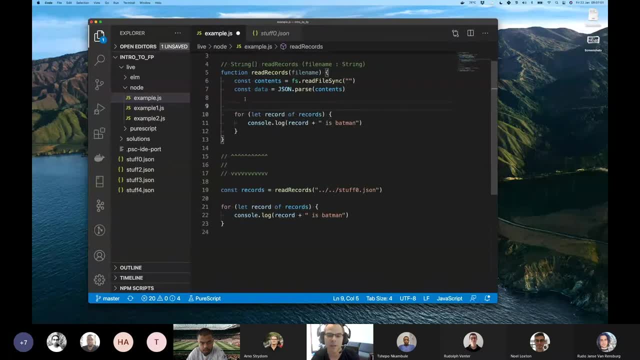 first, and we're going to go something like a var, maybe results. results equals an array, maybe, and then for record of records, I suppose we could go results dot. I think it's push. yeah makes sense. record dot name correct, something like. 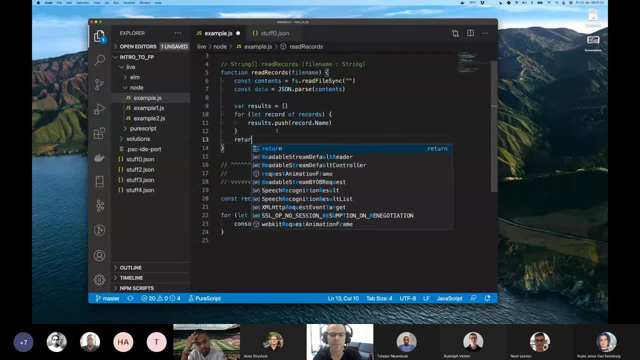 that and then return results. yeah, I, I don't really care. if we- you know, like I, I don't think we're ever going to write this- run it actually to see if it actually works, who really cares? 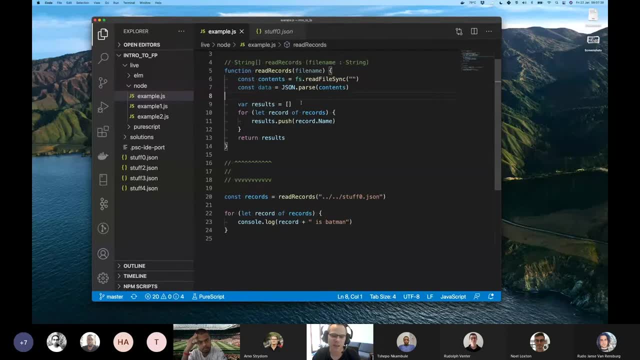 but I- but I think that's probably right- I don't think we've improved anything about like the issues that we had earlier, which was, you know, the file not existing, um it not being JSON, it not having 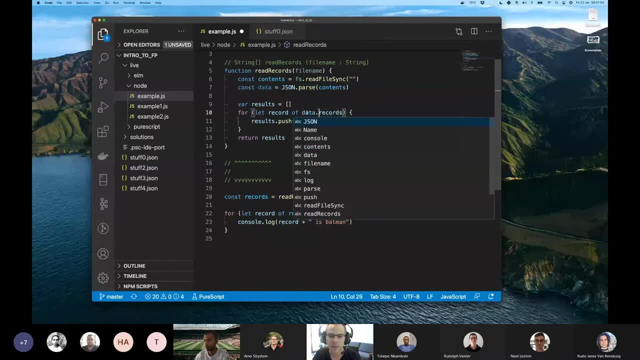 um, oh yeah, this should be like data dot records, right? uh, not having that records thing as a capital- no, it's a lowercase thing. and name also looks like it's a lowercase thing and not having those fields right. so we haven't improved anything. so 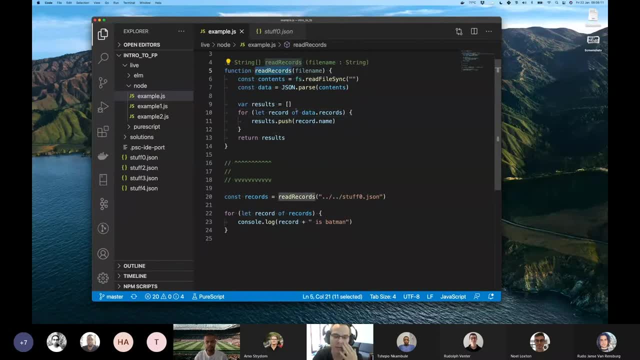 we've just kind of made it, we've just hidden it away in a little function, so so maybe the first thing we want to do is like let's deal with that first one, like the file not existing right, so so let's do that, so we go. 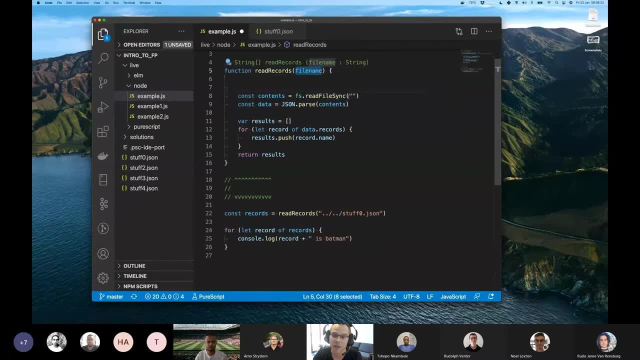 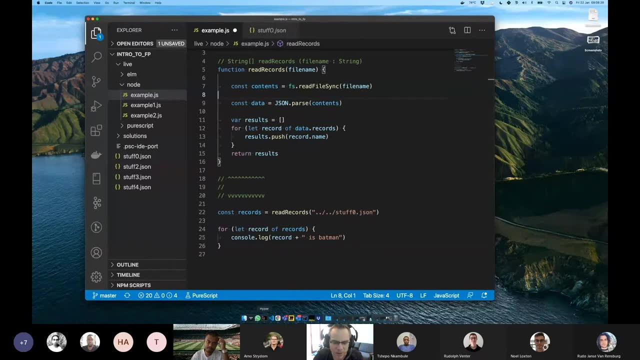 So we know that when the file doesn't exist, there's another issue there. File name should be passed there. Maybe we do want to run it actually, so we can see the exception happening. Let me just open my terminal intro. intro to FP. 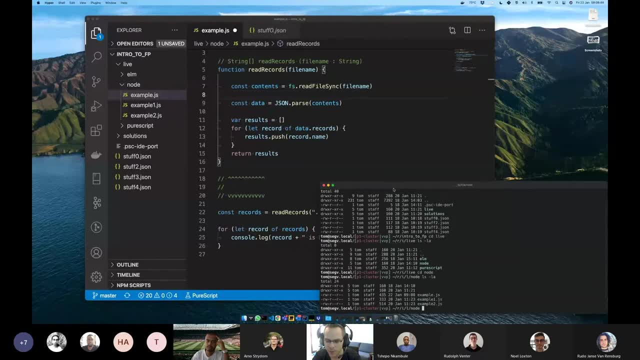 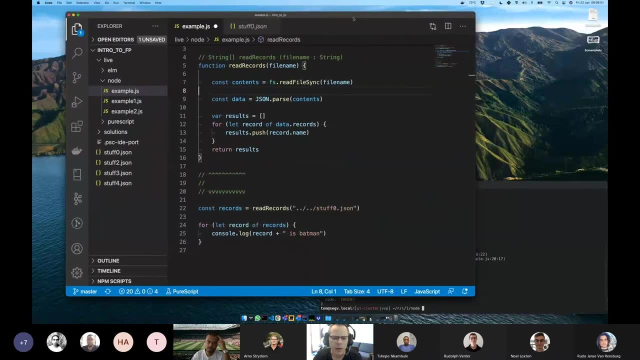 We live node and we go node, example, and it says no such file or directory. I wonder why I don't want this stuff Nought, So that's a good thing. Anyone see our issue here. Stuff is two directories back, I think. 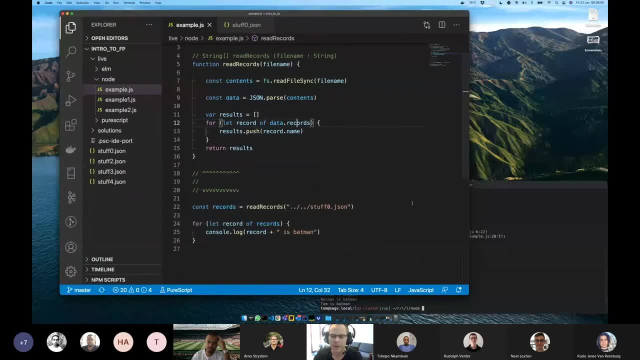 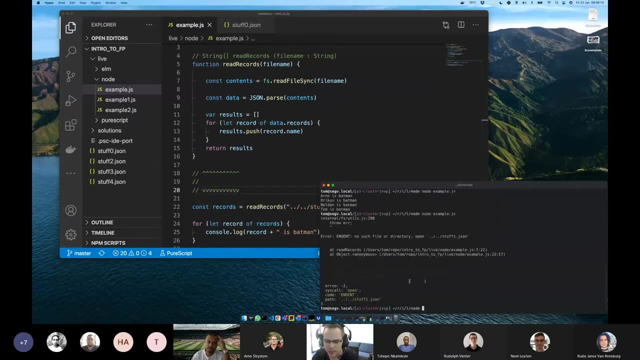 Maybe I didn't save it. Yeah, okay, I didn't save it. So if we made that stuff, one which doesn't exist, as you can see here, we run it. we can see, ah, okay, cool. So it throws some kind of error with some kind of text. 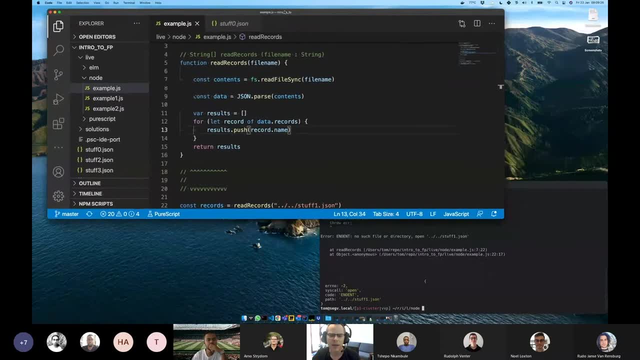 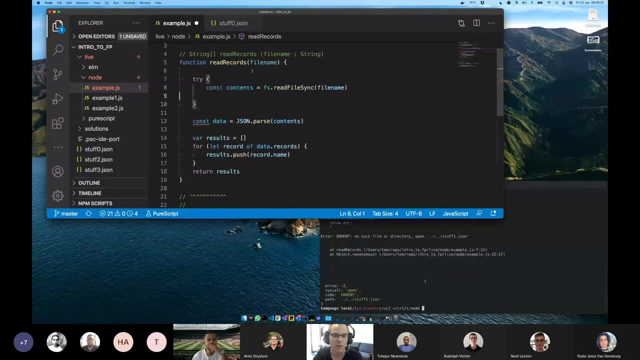 So we've got to be able to sort of handle that right. So how do we do that We catch an exception, right? So not 100% certain how to do this, but let's try. I think it would be. try, probably catch. 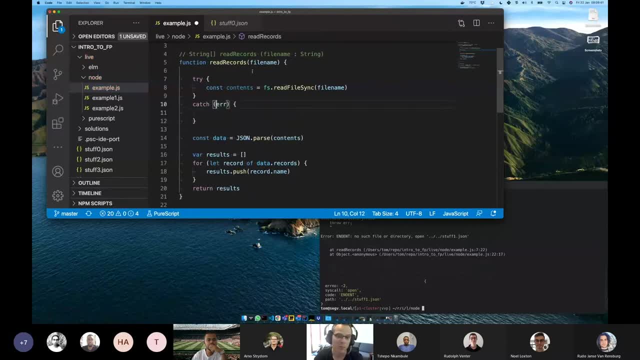 This is probably just catch some kind of error, or maybe we should say exception or ex or something, Because there's no typing here. we just kind of have to catch everything, I suppose. And now the interesting question is like: okay, well, if that happens, what do we do? right, 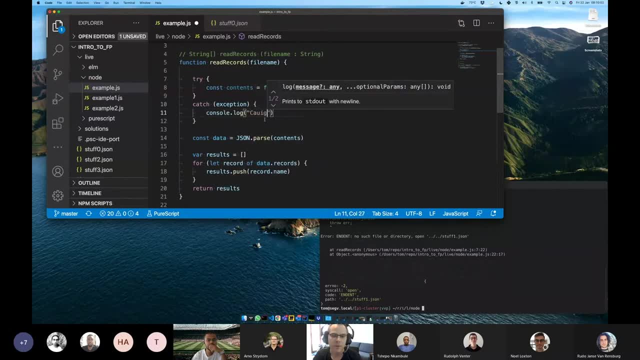 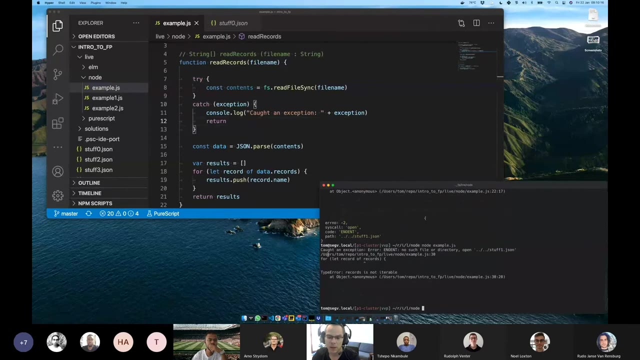 So I suppose we could initially just go just see that it happens, call to an exception and we go plus exception. We just hope that it can print a string and we'll like return if that makes sense. Yeah, okay, cool. 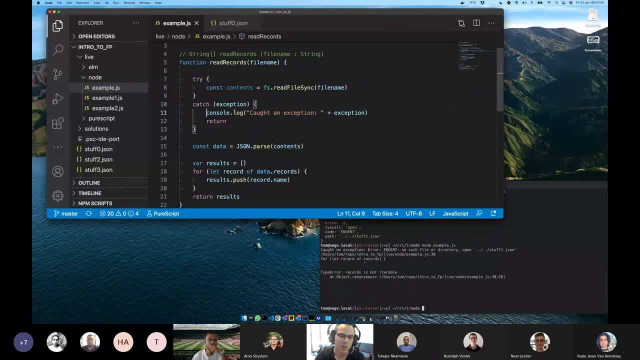 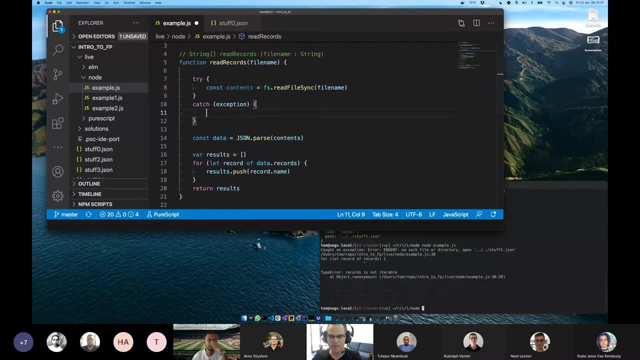 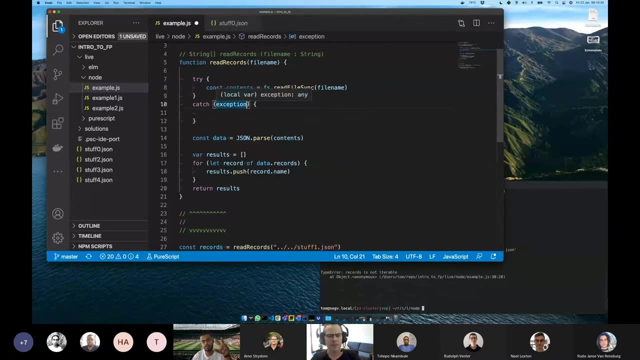 So we are able to caught an exception. that's good, So that's fine. What should we do in this scenario? Does anyone have any ideas? I would have taken out that try and catch block created a new variable of type var. 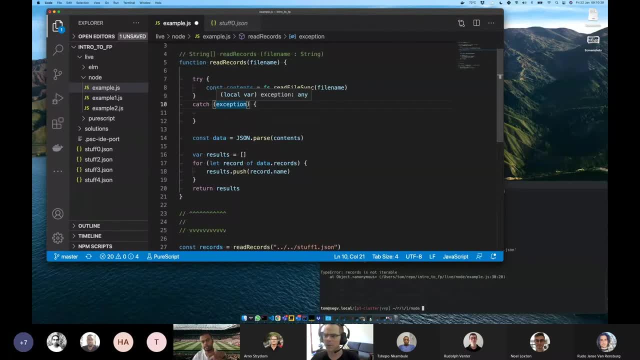 called it, say new file point to that path. So two directions back, stuff, whatever the file name is. And then I'll say: if that file my variable- let's say I said var- my file equals to new file. 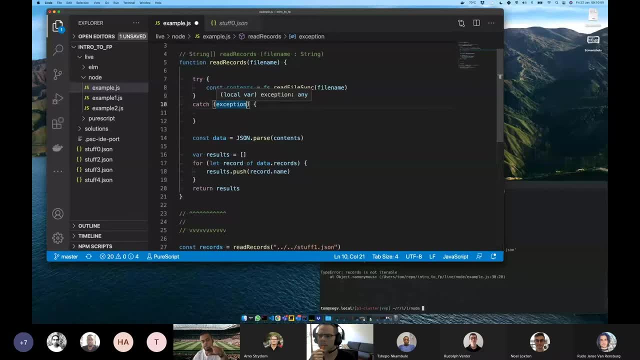 And then I pointed it to some path and then I said: if my fileexists, proceed with the code, else then I can send out an alert front saying file doesn't exist. But haven't we just done that? We know that the file doesn't exist here, right? 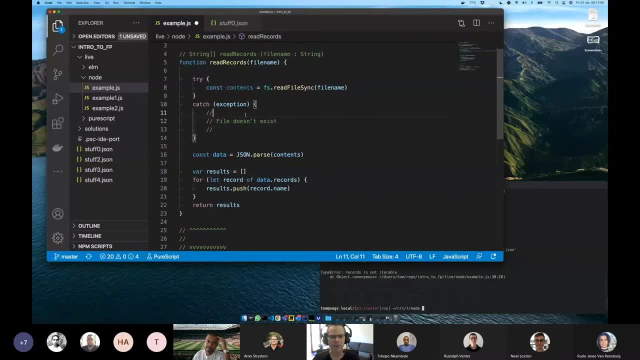 File doesn't exist right. Agree, we're in that place. So what should we do? I mean whether we check that the file exists right, exists beforehand or not. we know now that the file doesn't exist in this piece of code, in this block. 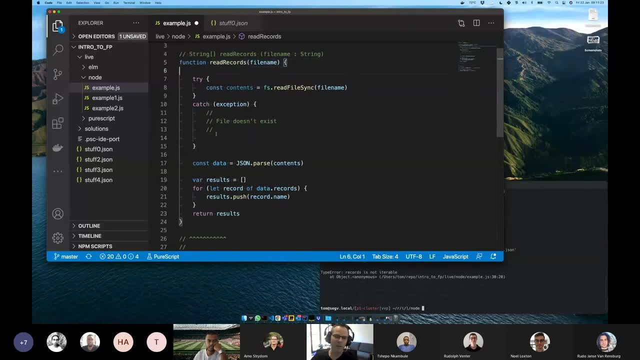 right. so what should we do from a function perspective? what makes sense? um, so, i mean, one of the ideas would be maybe, like we know at this point, like return an empty array- right, maybe that makes sense, because we did promise people that we'd be returning them an array of strings, right? 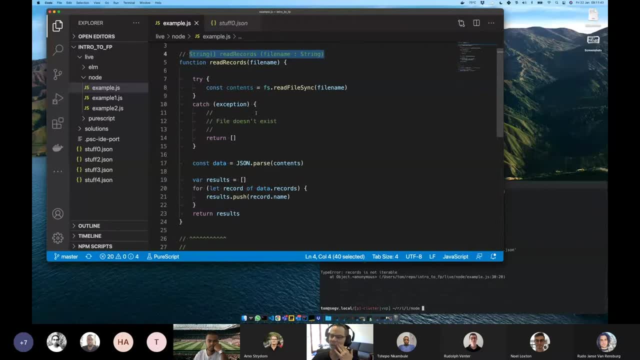 that's kind of what we said. from a function perspective, from a signature perspective, we are promising a set of strings, whereas if we had to say actually like return now maybe another option or we could, we could do something else. i don't know we could raise, i don't know if we can. 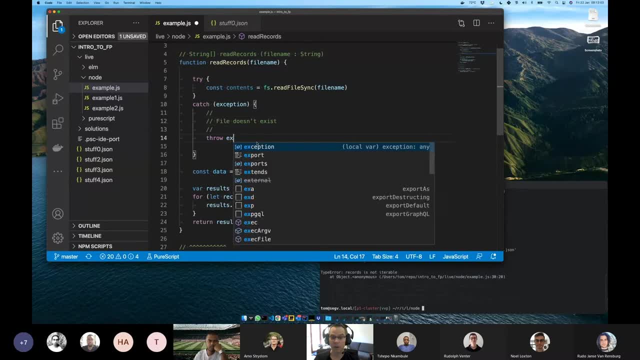 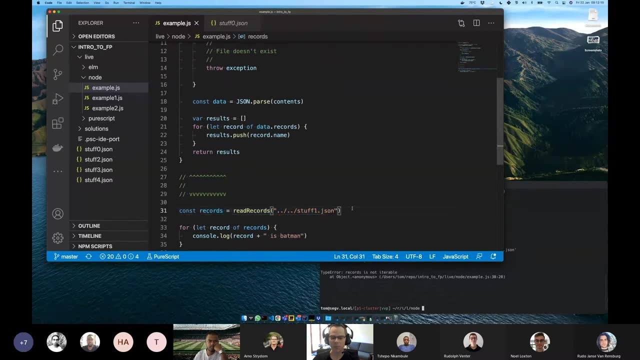 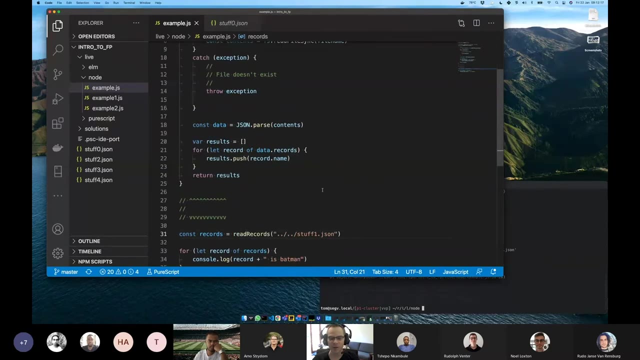 how do we raise, we throw. we could log it and then re-throw it, potentially for the, for the poor guy down here to handle. so so the point is like: what makes the most logical sense to do here and and- and i'm saying that there's, no, there's. there's not necessarily one good answer here, one correct answer, but what? 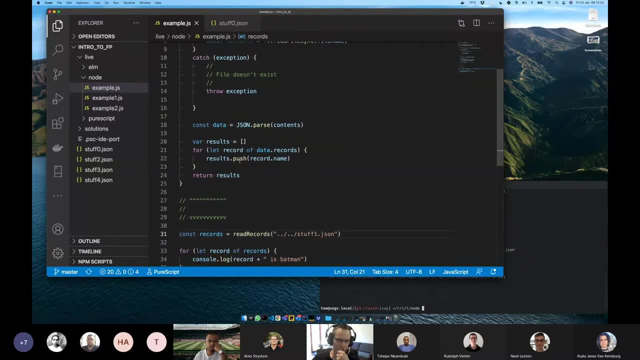 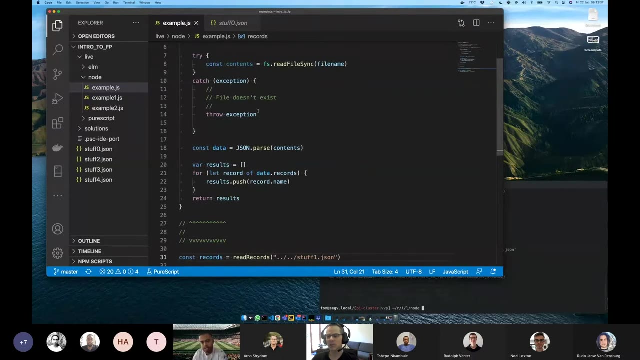 would make the least, what would be the least surprising thing to do here. is it a tough one, or am i? i think, the return of the empty string. i think the return of the empty string because the user on the other end is expecting an array, so even the string already is empty, at least again the same data type. yeah, so that. 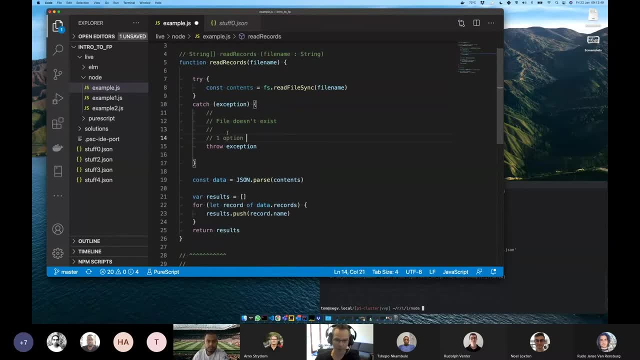 absolutely so that's like one possibility. one option is return empty array, um, which, which which i'm not like. i wouldn't be too unhappy with um, because we are now sticking to our guns. another option absolutely is to say uh. second option is to throw that exception. 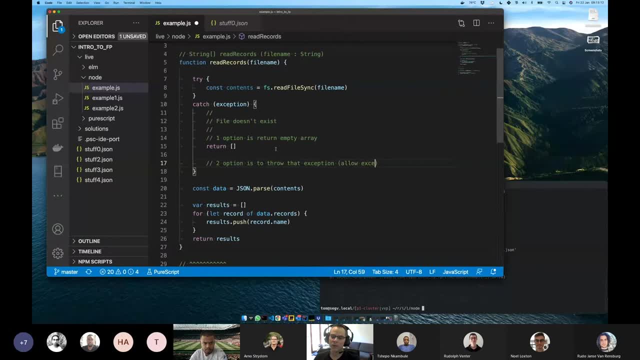 right to allow that exception to like bubble up to the caller because the so, so we can throw up our hands and say: like we don't know what to do, the file does not exist exception. like we don't know how to handle this exception, so let's raise it up and hope that someone further up our call stack knows what to do with it, right. 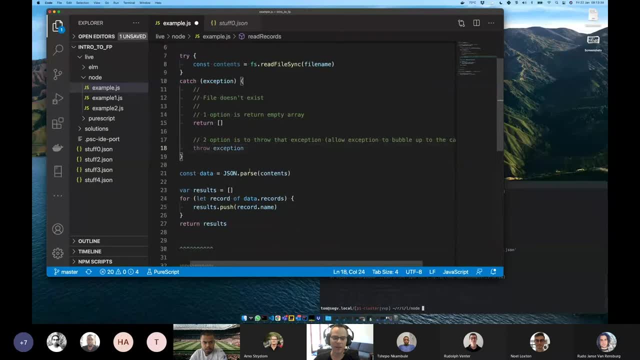 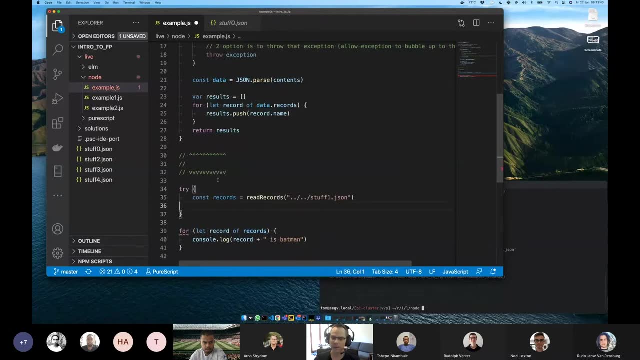 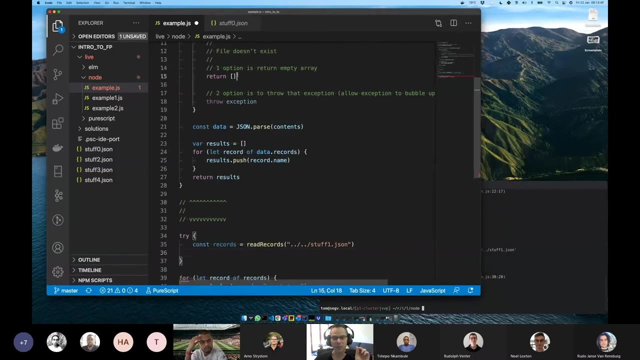 so. so that's certainly another option- is like, just let it raise itself up and put the burden on this poor guy over here to handle that exception, if that makes sense. right, that's a. that's the second. the second option, um, that they have pros and cons to them. you know the the the pro of option one, and i think there's. 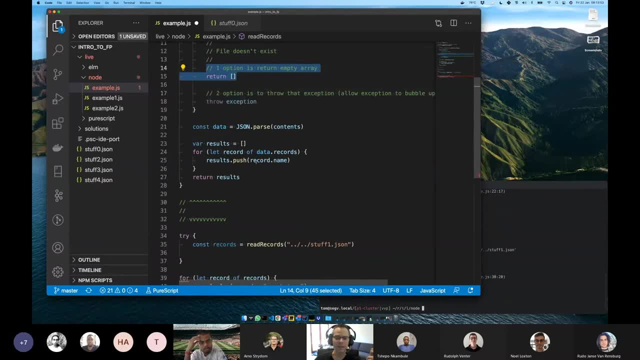 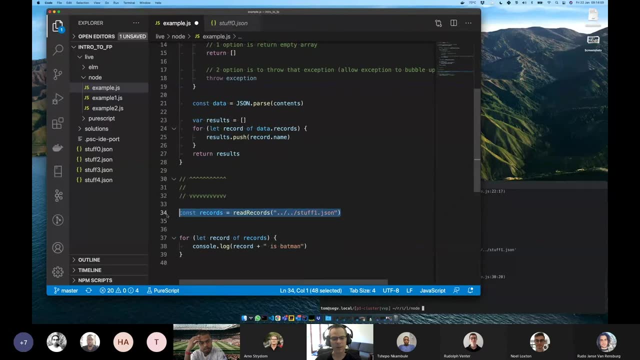 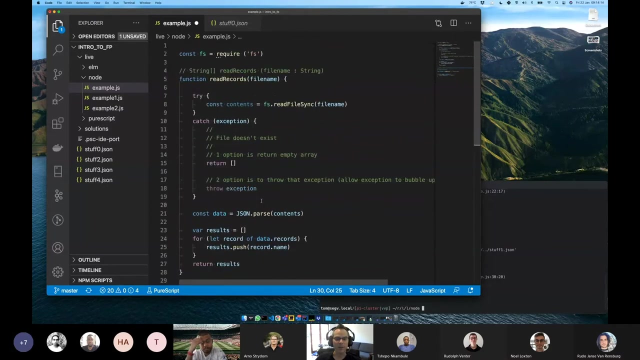 just variations of these two. actually, option one is a nice one, because what it means is that the the burden is not on the caller. so here's your caller, down here, this is your caller and this is like your callee or your library. um, the placing the burden on the caller is not always a good idea, and and the reason why is 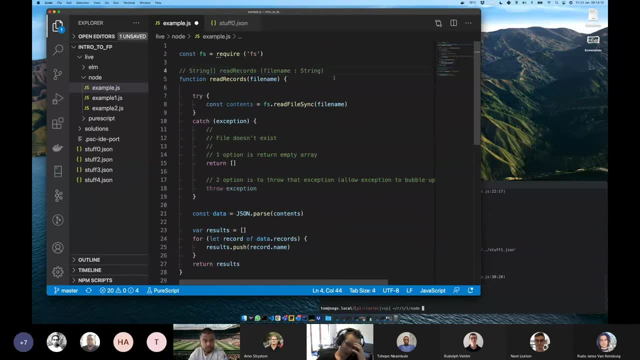 because he kind of just sees this right. so nothing up here tells him clearly that you know there could be something else that happens, right? so when i read this function, read records- given a file name of string, i'm expecting to get back an area of strings, right? nothing here tells me that. oh yeah. 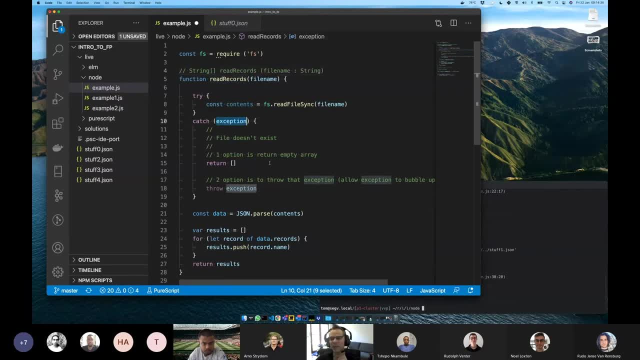 also, you could also get this like nasty exception coming at you that you're not prepared for. you know what i mean. some languages do that so, like java, for example, adds this cool thing here which is throws you know whatever file not found exception. and that's really cool, because when i look at this, 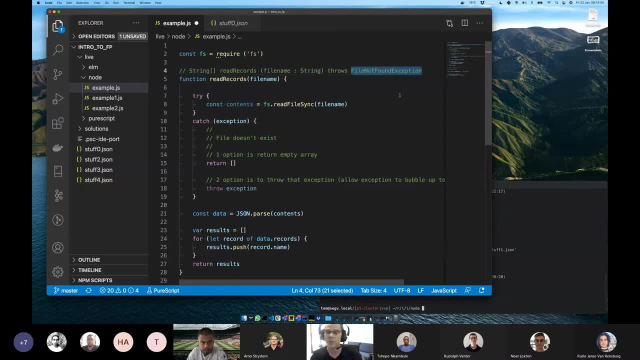 i go, oh yes, okay, so i can get these strings. but i also am aware that you know it could throw this kind of exception and the compiler can even check that you handle this um, which is pretty cool. but most languages don't really do that um, and so exceptions can often come at you from kind of 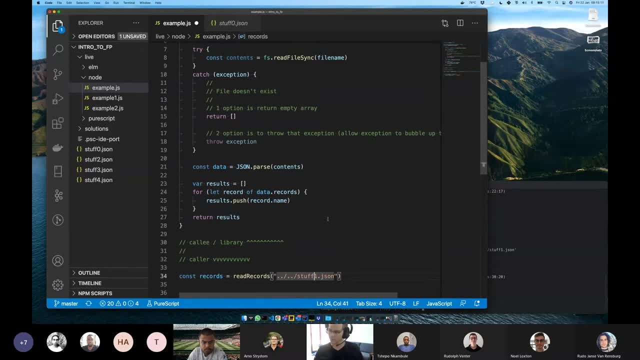 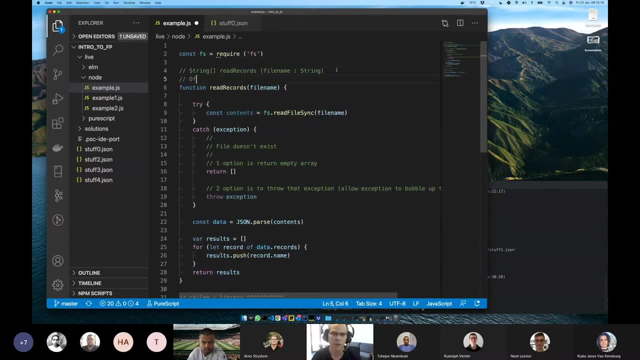 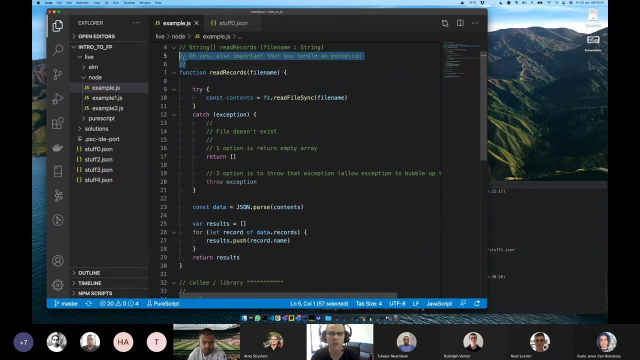 anywhere, and so my view is like: try to minimize that, because i think exceptions are very, are generally very- surprising, unless you write a big thingy up here. oh yes, also important that you handle an exception right, you know, add it into the documentation or something, but, as we all know, like there's probably a smaller percentage of people who will read that, um, okay, so 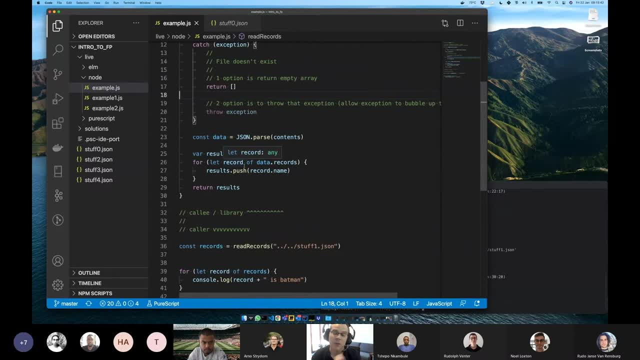 let's return the empty array, um, the, the, so, so from a downside perspective. so so that's a nice thing, because it keeps this clean from a downsize down, a downside perspective, the. the nasty thing about this is that we are we're like throwing away information, right. 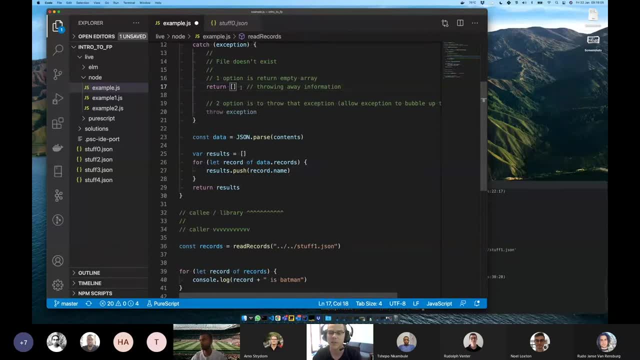 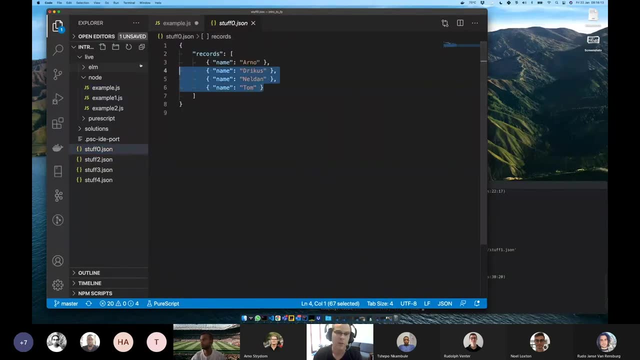 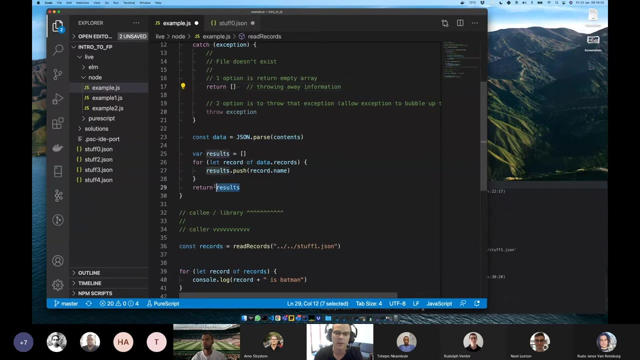 and that information is that actually something went wrong underneath. it's not that it went right and that it was an empty. you know, for example, if i took this and it had no records, if it looked like that, that would also return an empty array down here, right, and so it could be assumed that, oh, look the. 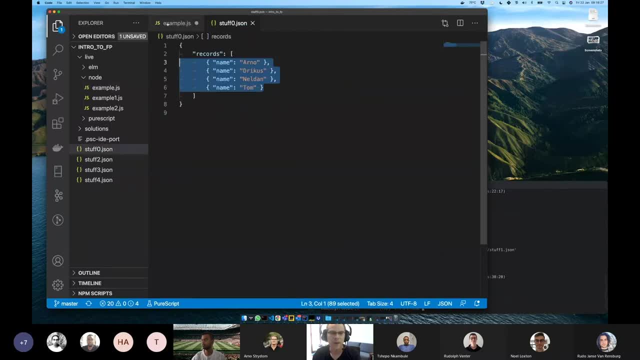 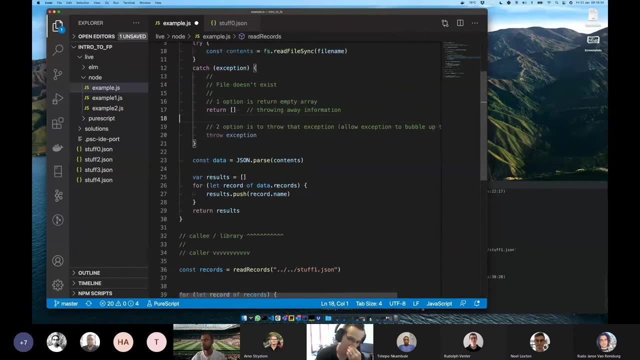 file's just got no records in it, so we're good, um, as opposed to: oh look, the file didn't exist actually, and that's like a bigger problem, um, and so that's the downside, so that's the downside of keeping it clean, right, but but anyway, let's keep going, let's go with that one and we'll solve that. 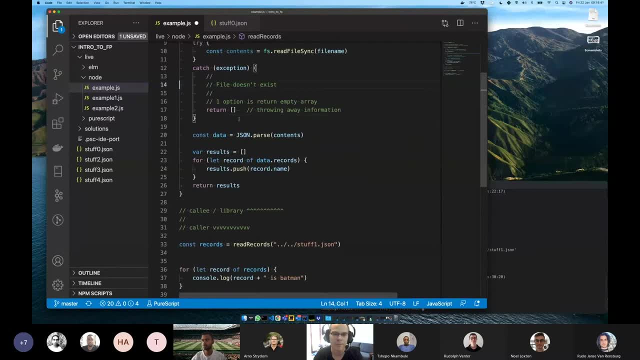 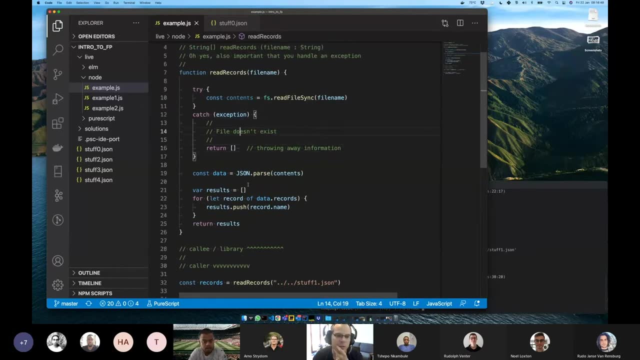 problem, especially in a different way. um, so let's keep that throwing away information. okay, so that looks a bit better. we can now handle the exception, um, and then down here we're gonna pause it. and now already what i'm starting to see is like: oh look, um, i'm not sure if you guys can see the issue here. 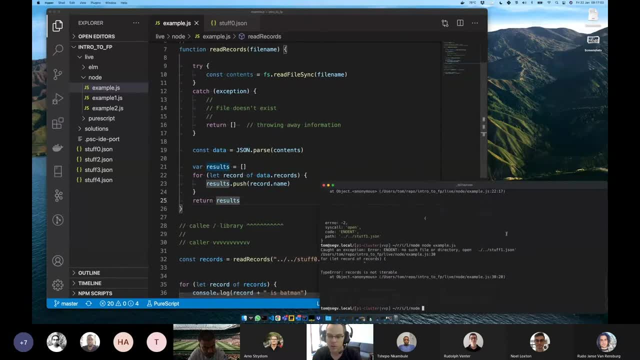 yet, um, but is this code gonna just work? probably not, no, and it's because of that content, right. so so whatう Sunday? you all have mind. you need to know, because today we are back to the future issue here. so it's saying contents is not defined. any ideas why? why that is? 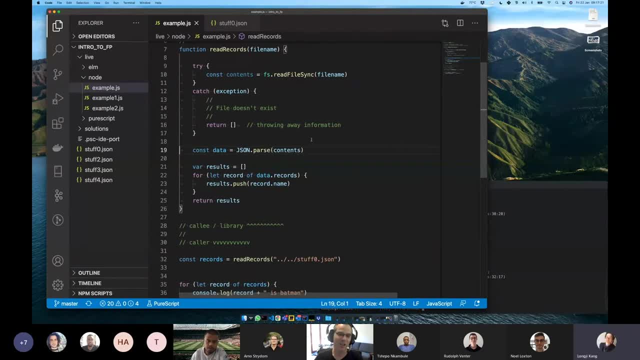 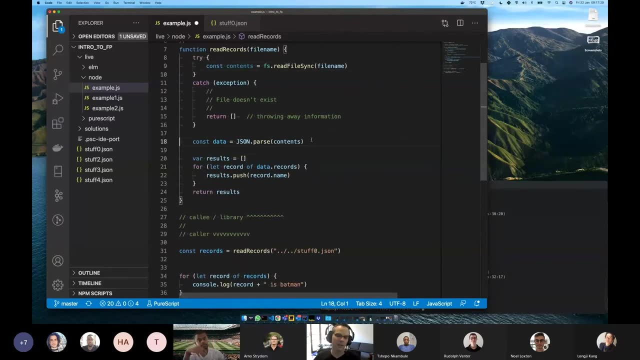 isn't it out of scope? yes, it's out of scope, exactly. so already like, okay, cool. so we we got clever and we said: let's handle this exception. now we're also having to go. oh yeah, so this thing creates some scope. um, so the scope of contents is within this little scope. 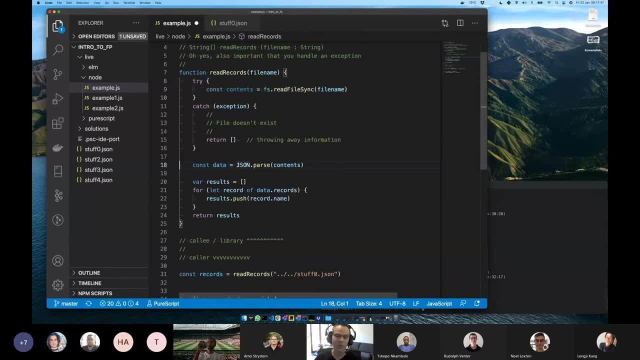 blocky here. so so again we've got like two options right, so we can lift this thing up and we can pop it in there, um, and now we're starting to say, oh look, our exception handling is now like for exceptions of both types, right, because we also know that this could potentially 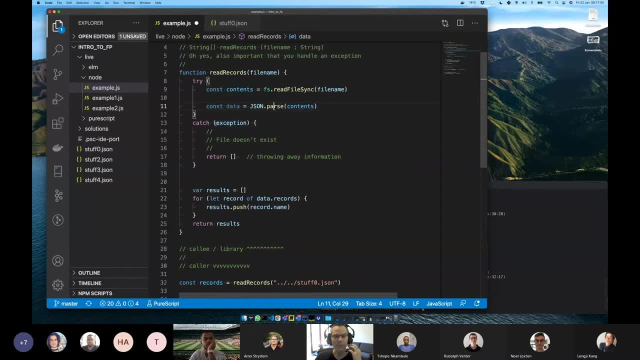 throw an exception and um, and it's going to be caught by the same exception handler, i suppose over here. the other option is to say, well, we, we want to keep them separate. um, and we want to have a second. try catch, block over here. try catch, whatever. 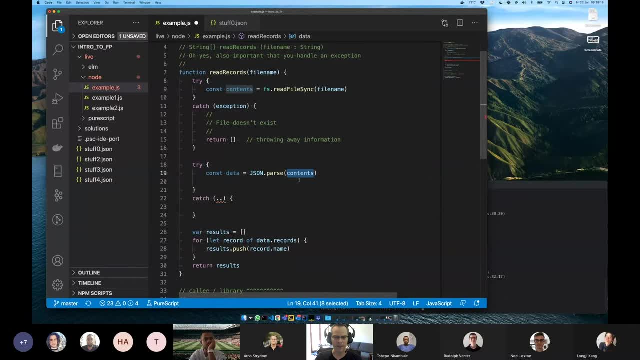 and now we have to deal with the fact that we want to lift that thingy out into a higher level scope. so probably we want it up here: contents equals- i don't know something, um, and make that not a new variable. uh, contents is probably a string, so we want it to be like an empty string. 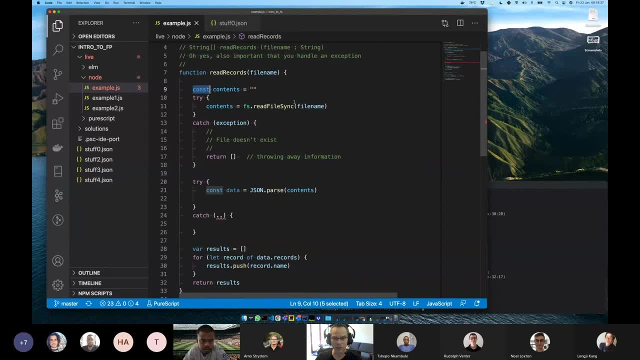 problematic though, because we're like reassigning it here and so it can't be a const anymore. right, it needs to be a variable um, and so, like the reason for having const there was was like quite a nice one, but now we can't have it um exception there, and now maybe we've got. 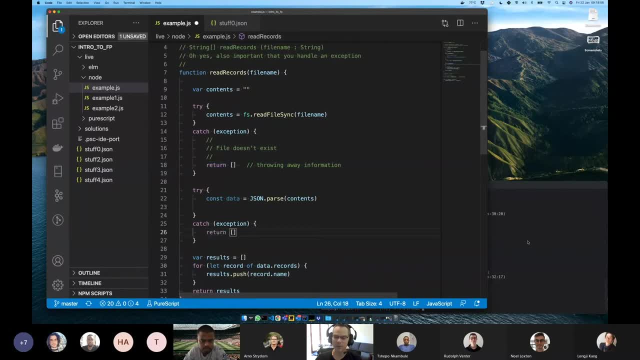 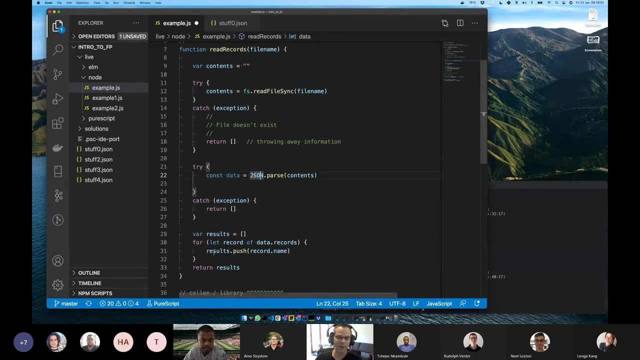 a different way of handling the second type of exception, right, does that kind of make sense? um, and now? yeah, of course. so, like, like, we have that same problem again over here and now, where it's like it wants to run through data. guess what data is in the scope of this thing? 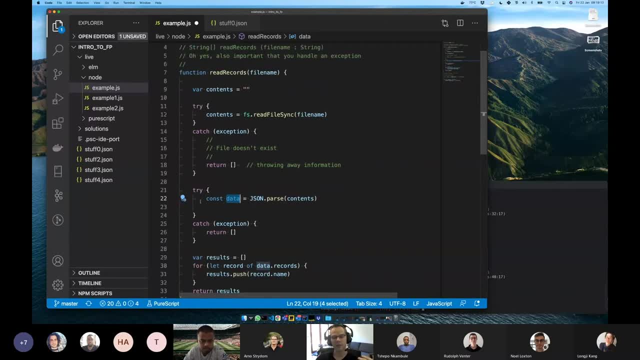 so it's like: okay, ready, we're going. oh yeah, this is like this- lifting into a second try catch block. it's probably going to hurt us because once again it wants var data as something and we're going to reassign it there and it's no longer a const. um. 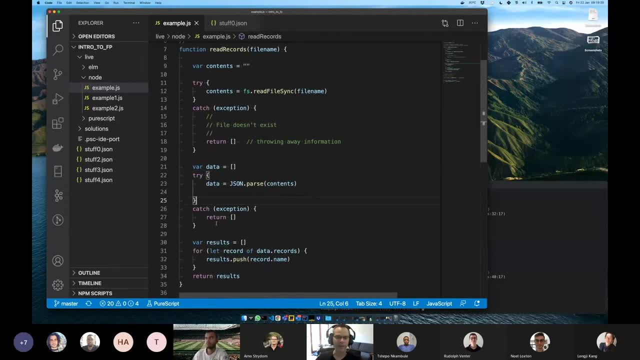 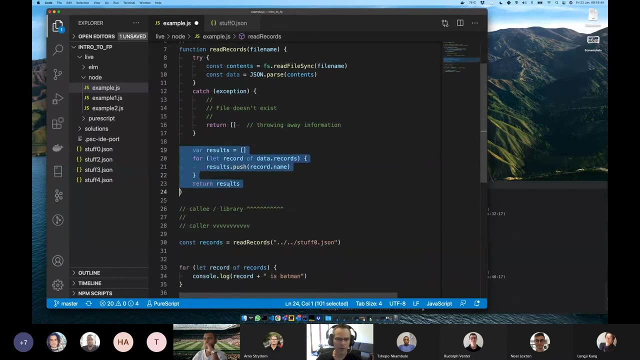 etc. etc, etc. right, so this is probably a bad rabbit hole. so so let's stick with our our first one, which was like cool, let's keep it a const. we were happy with that. this thing can be a const and we can already see that, like we know, this is going to happen again, so we're going to put that. 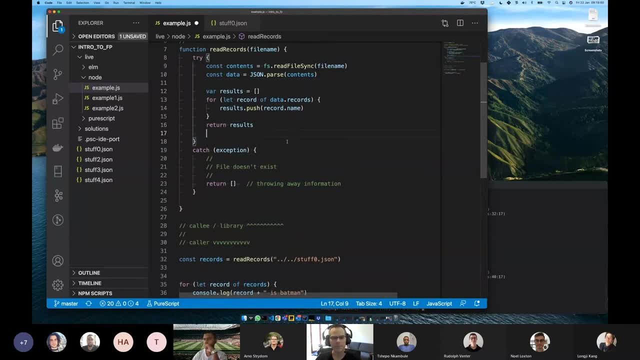 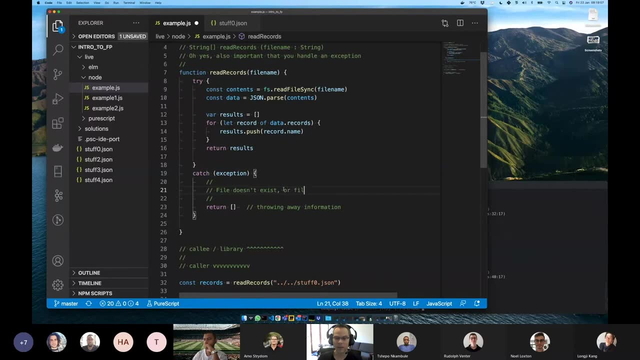 there, um and life, yeah, okay. so, yeah, file doesn't exist, or file isn't json, or records don't exist or doesn't have a dot name attribute, right, so there's many reasons potentially that, uh, this exception could be raised now, right, because that kind of any problem over here could raise. 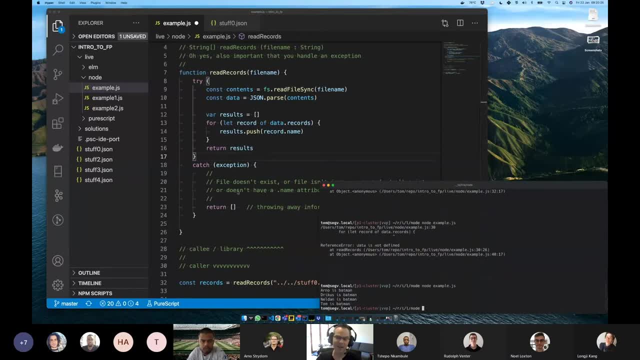 this kind of exception, right, um, but at least our code works again, which is great. um, i suppose we could test it through stuff one, see what happens and it's going to be okay. it's like, oh cool, so stuff one doesn't exist, so it's an empty list there. so nobody's batman, right? 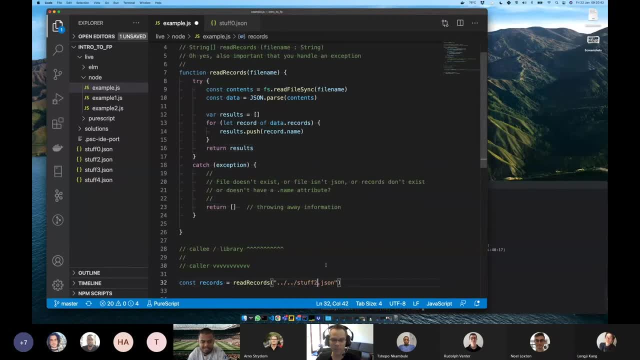 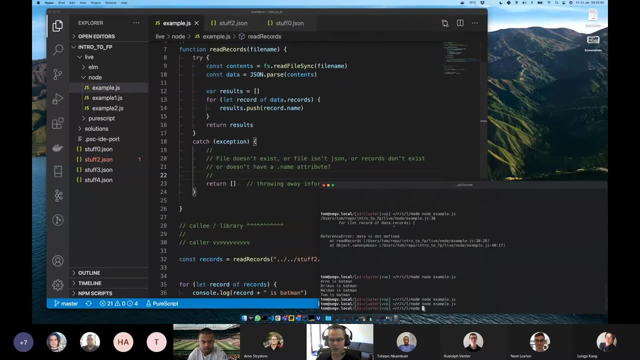 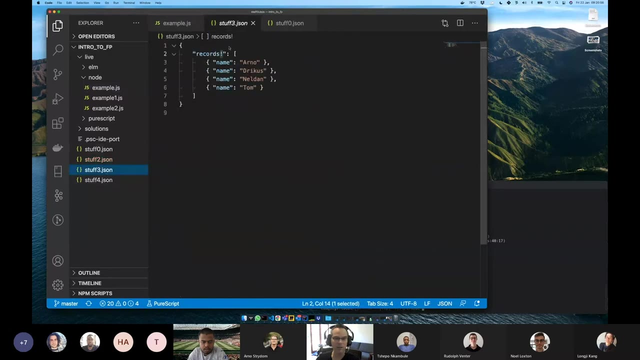 so that's cool, um, well, well, is it cool? i would say probably not that cool, uh, number two: uh was: oh yeah, we broke the json, so also nobody's batman. um, i don't know, you know, they're definitely throwing away information there. three was: we were missing that field there, so again, nobody is batman. 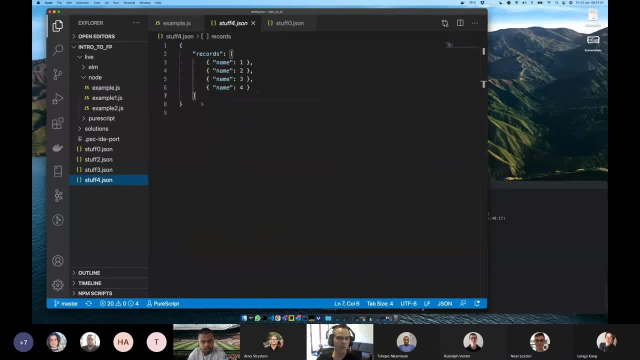 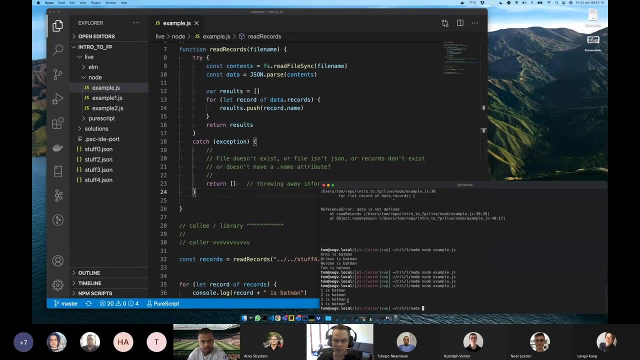 number four: oh, one, two, three, four. oh yeah, so what did we do with four? oh yes, we made them that kind of in, so we like changed their types or whatever. um, i don't know, i mean, like, whether that's, whether that's a good idea is, i'm not sure, um, but but anyway, like what we've. so maybe we've made the. 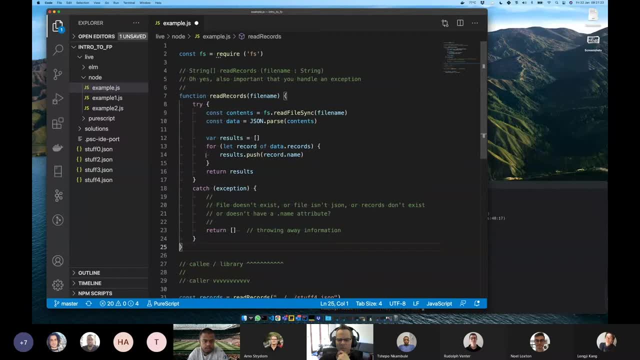 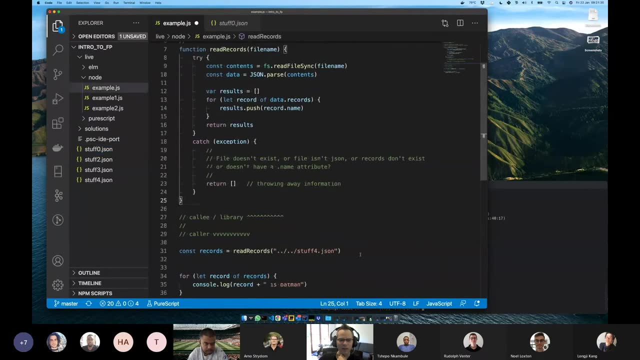 code like less runtime, brittle, but, but i wouldn't say that we've made this much better. what would you guys say? i would say like wouldn't it be nice if the caller down over here knew that something was was broken, right, um and so. so this leads to to saying, well, actually is this, is this type here? 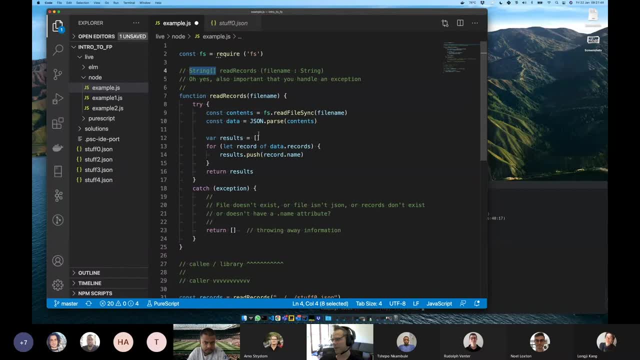 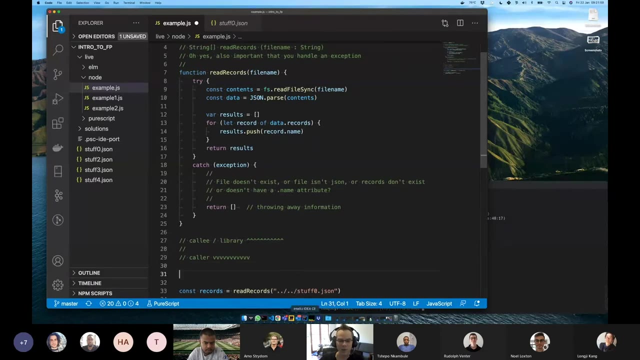 as a return type of string, string array. is that actually appropriate? like do are we allowing um enough space to encode these different kinds of scenarios that could come back? because if you think about it like, actually, maybe what we want is like we've got a few different situations when we call read records. of course, the one is like: yes, we 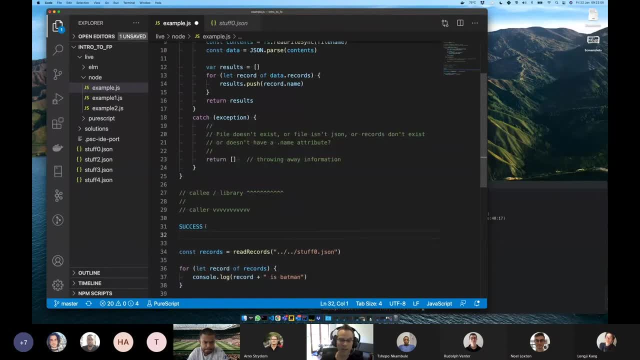 were successful. you know, a second one could be like: actually the file you provided does not exist and it's like actually remember the file you provided because you did provide that file right and so, probably as a caller of this thing, i would like to know if the file i provided. 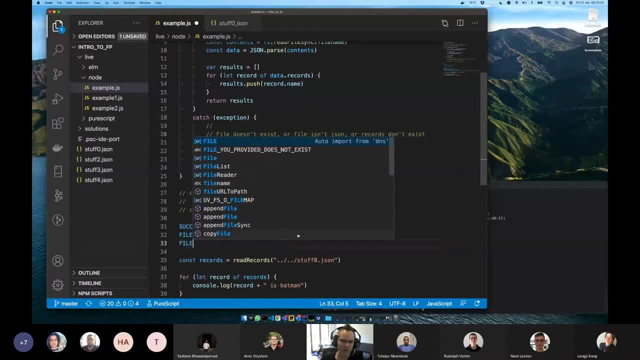 there does not exist right. and then and then there's others, like the file you know isn't json format, you know that's. that's interesting, i think. and the second one was, like you know, maybe there was an empty set of records and actually maybe that's encoded. 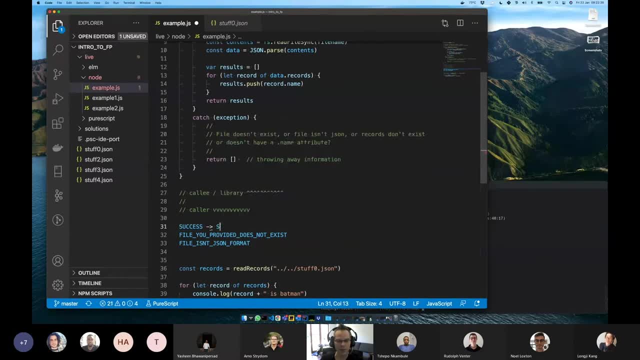 in success, so it's like we want to know that when it's successful i want an array of ints. when the file you provided does not exist, that's actually fine. i don't need any other information included with that error. the file is in json format, probably also. 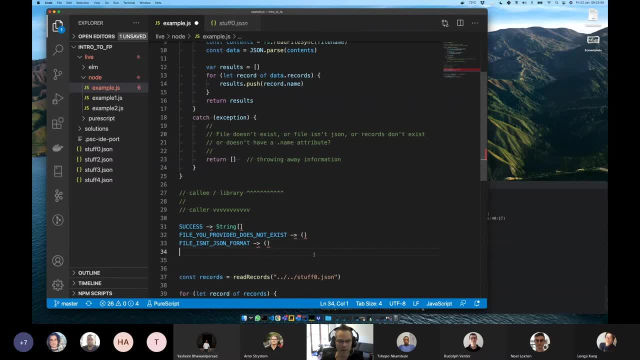 makes sense to not give me any other information. but what about, like the field records? um, did you know, i don't know is broken or like a some kind of pause issue, right, yeah, like a pausing error and actually maybe i do want to know, like i do want to know that um. 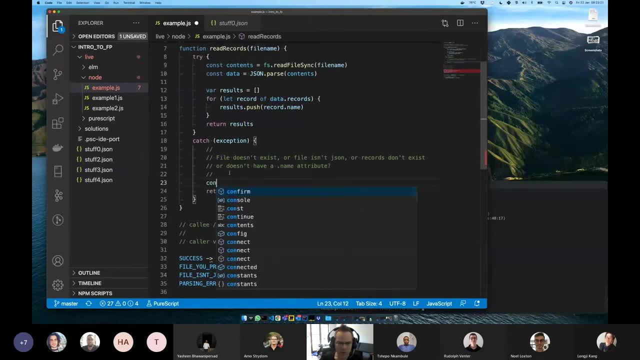 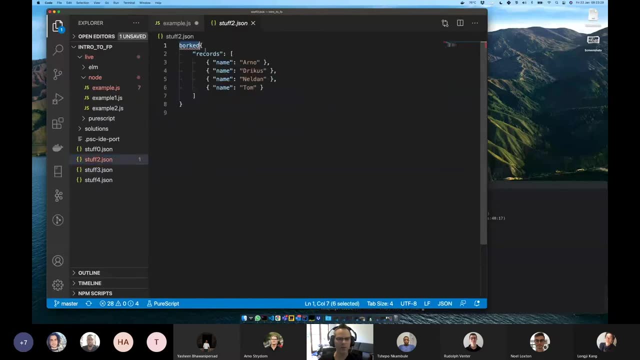 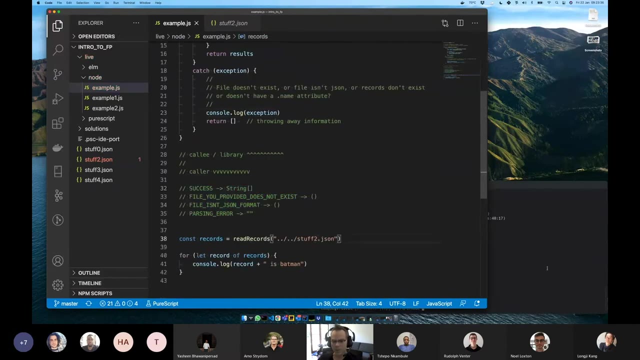 the exception was like let's actually go and have a look. so if we go consolelog exception here and we run this on number two, like let's run it on this balked, on this balked file here, right, which was number one two, i'll just comment that out, number two. i'm sure we're getting some information from the exception. 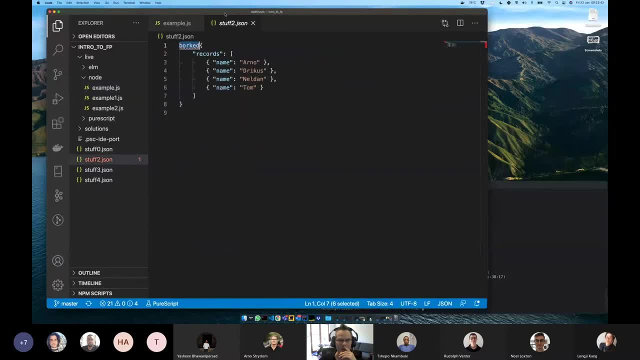 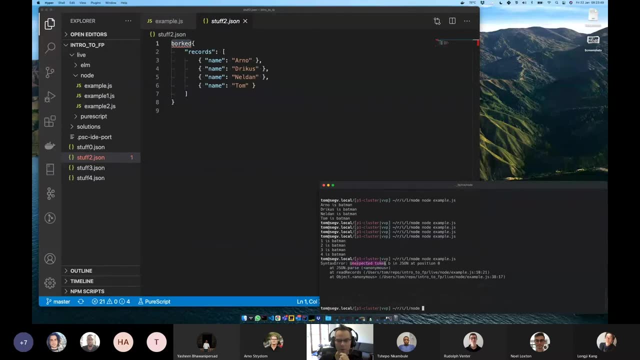 yeah, you can see it here. so when we catch that stuff too, i'll just put it up. when we say: pause that please, as json- actually the exception- does carry a bit of information. it says unexpected token b in json at position naught. so it's saying hey, like i was trying to read json and like b is. 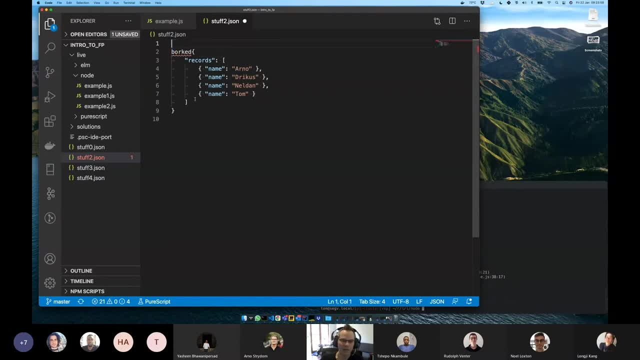 definitely not. the start of a json packet like the adjacent file either starts with a with an open curly bracket, or i think it could start with an open square bracket if it was an array. or it could start with an open quote, because it may be a string or it could be an int, it could be some. 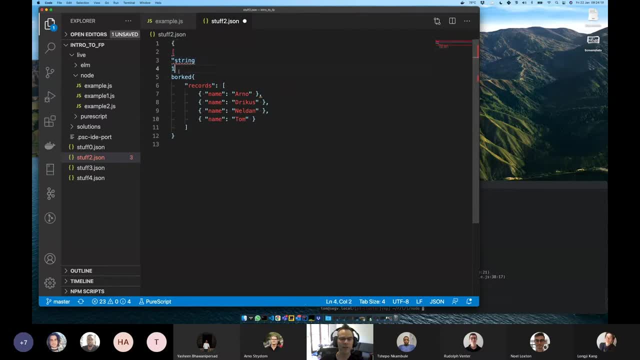 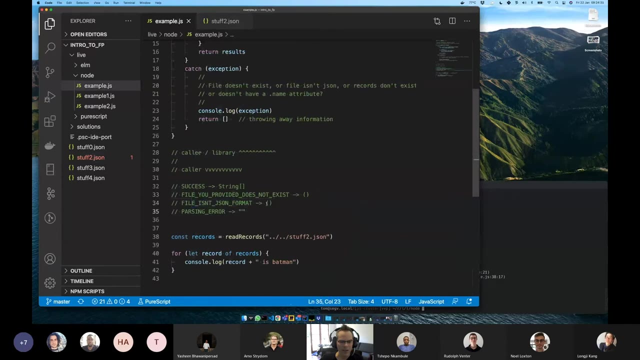 kind of json primitive type, but he certainly is not, is of no type i'm aware of um, so that actually is quite interesting. so when we get some, when we get a pause issue, uh with, isn't json format actually maybe empty's not right? i actually would like to see the particular error right, particular error, because that might be. 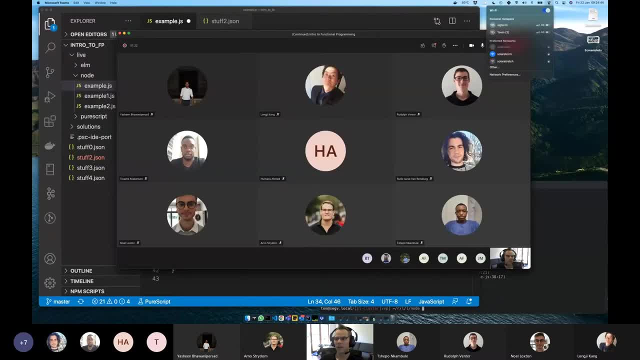 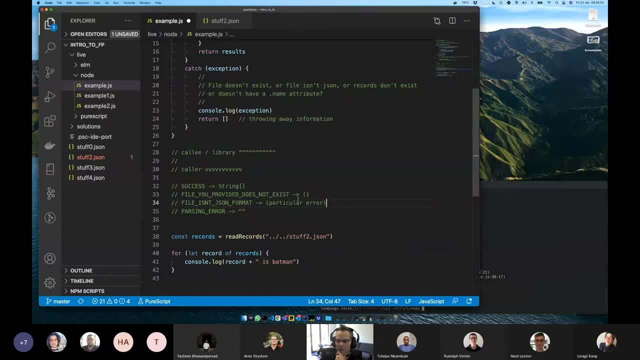 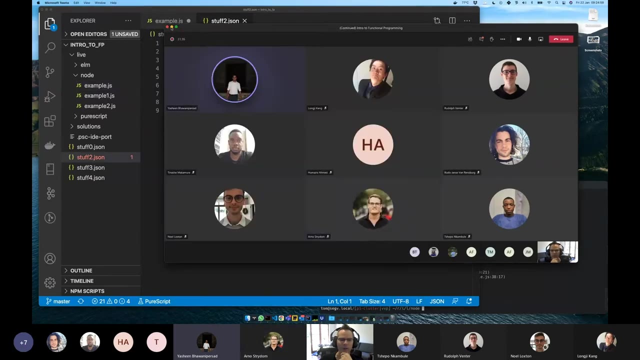 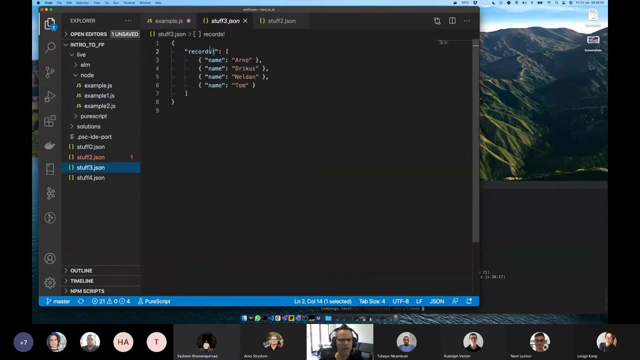 useful. sorry, i think i went on and off for a minute there. um, can you guys still hear me? yes, yes, okay, okay, good, um, okay, cool, uh, does that kind of make sense? so, like we want to maybe carry some additional information, um, i wonder if with like this guy, what we would get. so stuff, three. 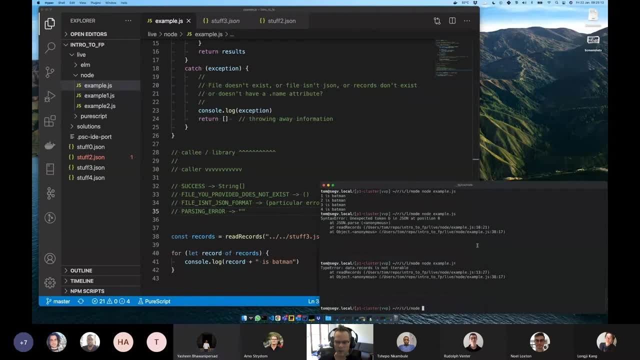 let's try run that and see what the exception looks like. is there one? oh yes, datarecords is not iterable, like that's also very cool. so, um, there's some other kind of issue here, like- uh, i don't know what you'd call it like, like a structure. 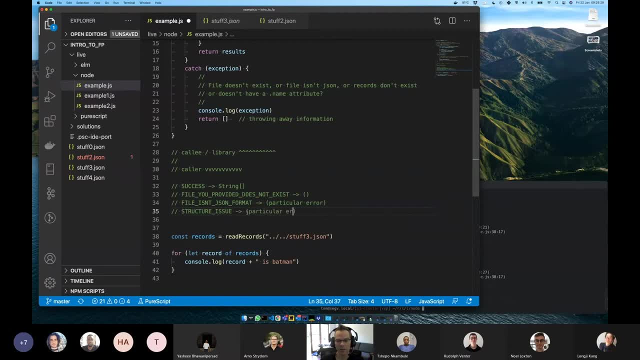 issue right, and on that i would also like to know the particular error. like datarecords is not iterable, does that make sense? so actually, when we think about this function- read records- we've placed a pretty big burden on, a pretty big set of requirements on it. that, yes, in general it should. 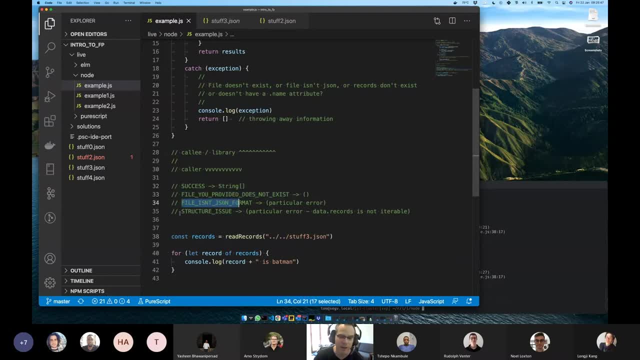 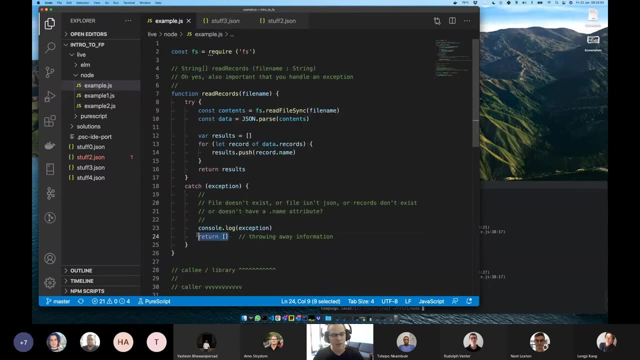 do this, but also sometimes we'd like it to do that and to do this and to have that right. um, there's different and and so string array up here is like it's not, it's not enough. we're throwing away that information here, by the way. so string array is not, it's not enough, we're throwing away. 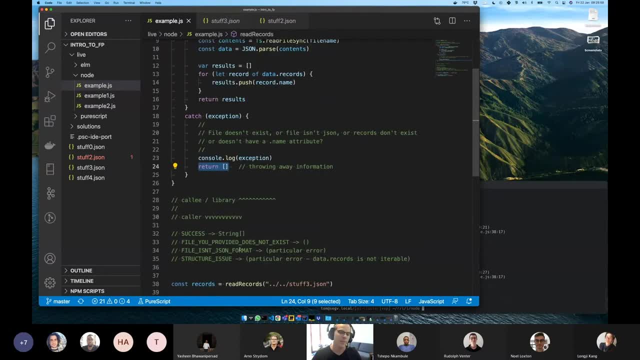 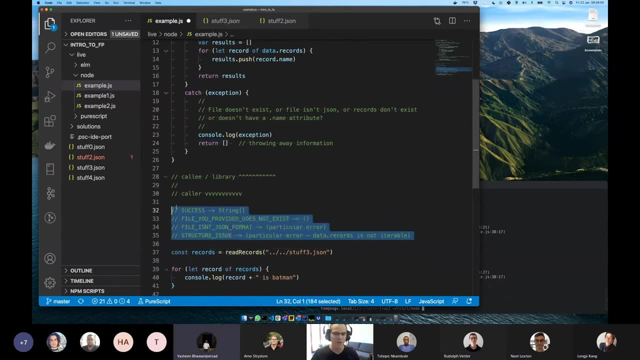 that information here. by the way, string array is not. it's not enough. we're throwing away that information here by just saying returning empty string. so any ideas as to how we could make this function better? given these requirements? i'm i'm not quite sure on what we should return, because 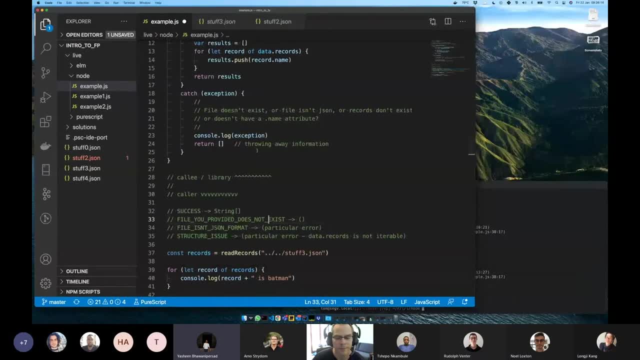 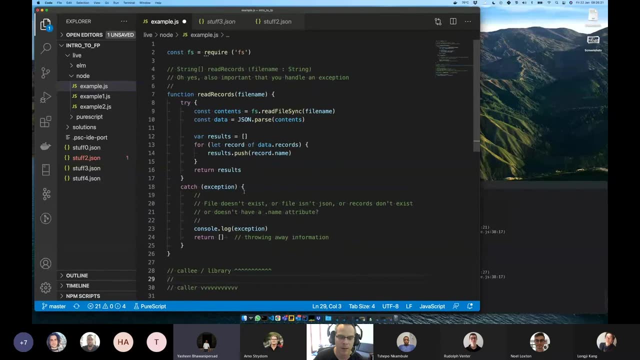 i'm still thinking over there, but i'm thinking the pose that i said with checking the if statement first. if this file exists, and then i can return an inappropriate message to the front. then going on to check, is the first character in the file, uh, in the file, so let's say the sq value of the? 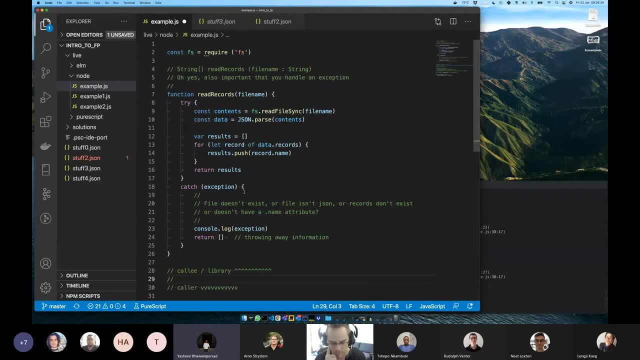 first character, uh. is it a valid one? so, uh, before you mentioned the uh caret, the uh array bracket, the apostrophe and the number, is that valid? uh, and then from from there, i can use the hair's own property to see if this json structure that now we passed the first two if statement, it is a file. 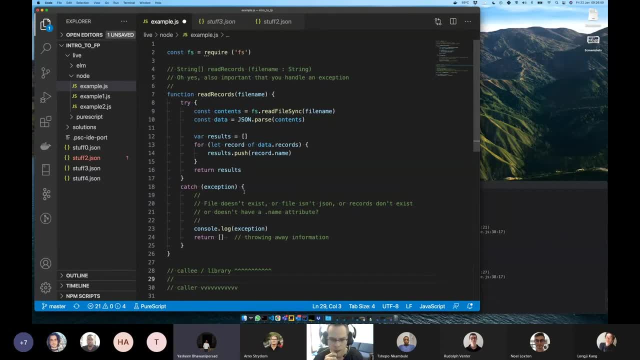 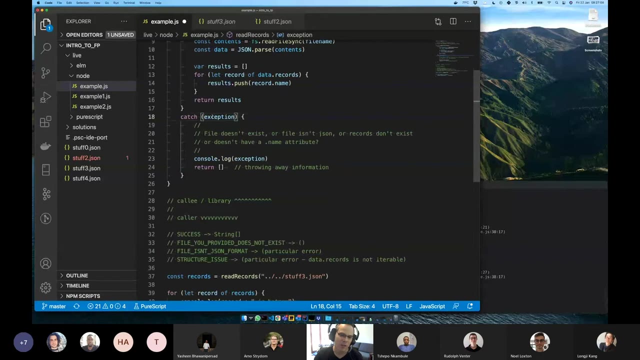 it is a different structure. uh, is there a valid one? this uh structure with the inappropriate prop property, does it have the property of records? and inside the property of records, does it have the property? yeah, no, i, i totally hear you. we can run those checks for sure. um, i'm saying to you like don't bother, you're already, you're already. 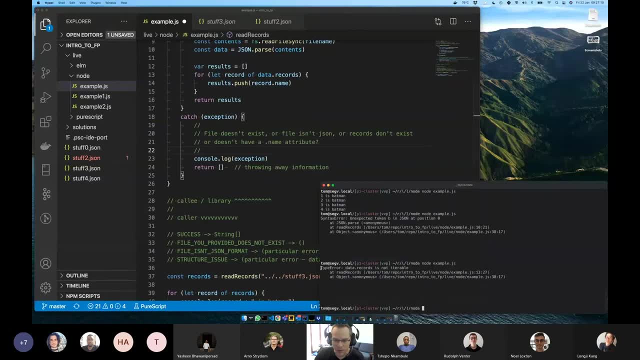 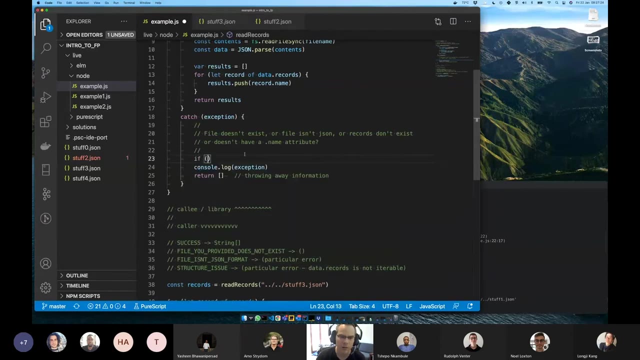 catching an exception here and we could know that, like this particular one is like a type error, right. so we earlier had a syntax error. here i think we get a reference error, here we get an error error. so let's let's separate those two things. so i think you can go. if exception, is it instance of? 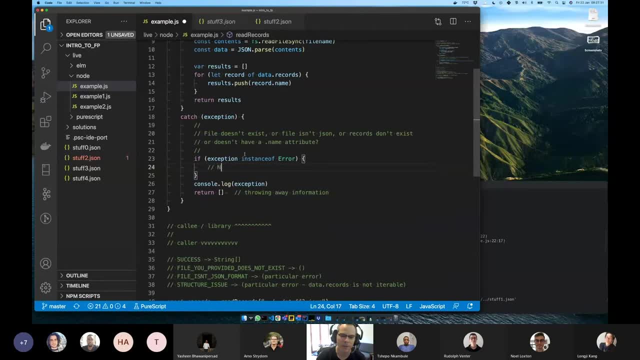 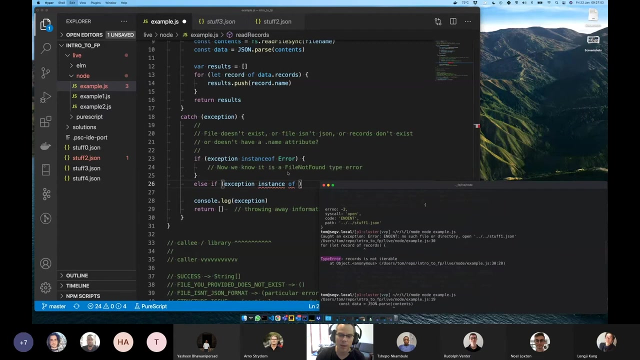 yeah, instance of error. now we know it is a file not found. type error: um versus. i suppose we go else if over there, i don't know, probably here else if exception. instance of um. i'm just i'm just being more lazy than than what you're proposing. um, sorry, instance of type. 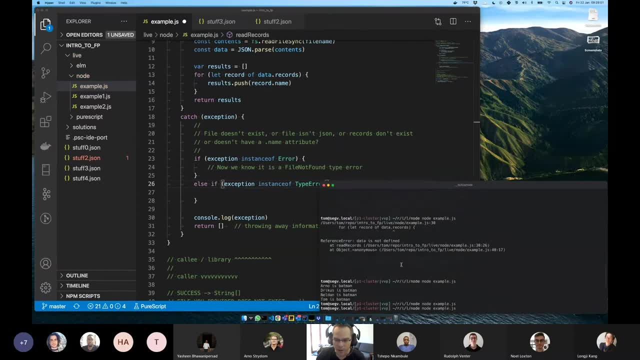 error. so type error tells us: okay, that's that scenario. i wanted to get that parsy one. reference error: no records, not iterable. no, not that guy i mean, which is below it was that balked one, right, yeah, syntax error. which is that one? uh, now we know it is a syntax error. uh, now we know it is a syntax error. 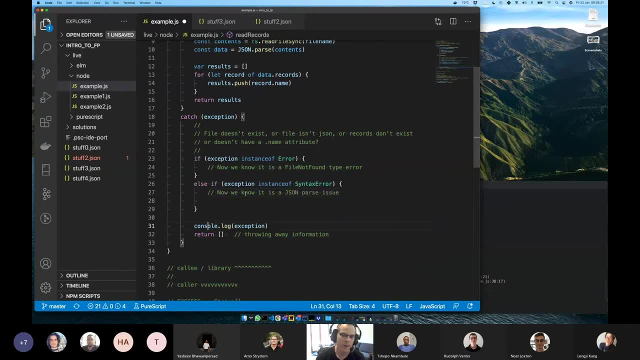 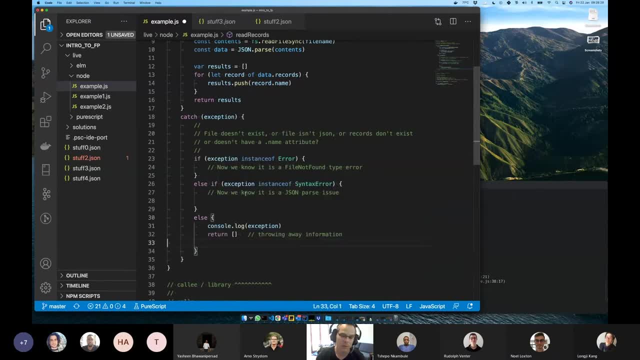 right, um, right, um, and this has got big big else there, and this has got big big else there, and this has got big big else there. so so the question is now so you know so. so the question is now so you know. so. so the question is now so you know, otherwise i don't know something else. um. 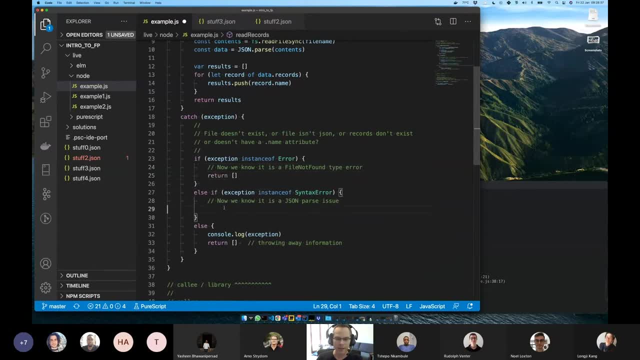 otherwise, i don't know something else. um, otherwise, i don't know something else. um what, what, what are we? are you proposing that we still are? we are you proposing that we still are? we are you proposing that we still return a blanky thing here, or you were? 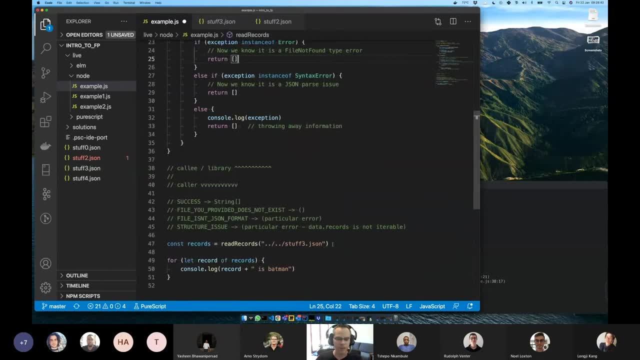 return a blanky thing here. or you were return a blanky thing here, or you were saying: are you saying you wanted to saying? are you saying you wanted to saying? are you saying you wanted to notify this caller somehow of the error? notify this caller somehow of the error? 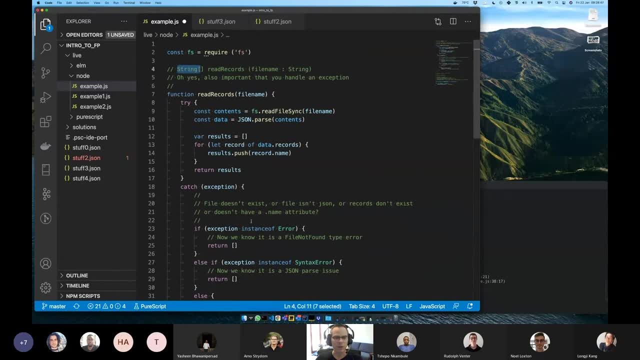 notify this caller somehow of the error, so how do you propose doing that when? so? how do you propose doing that when? so? how do you propose doing that when the only way of notifying him is through? the only way of notifying him is through? the only way of notifying him is through this array of strings? are you saying? 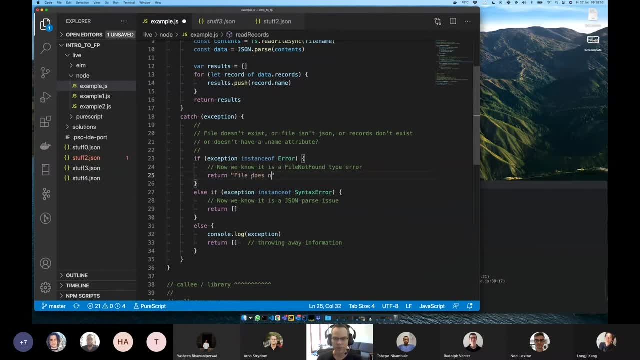 this array of strings? are you saying this array of strings? are you saying return, return, return, file does not file, does not file does not exist, exist, exist, like that, like that. like that. that would be weird if records were set. that would be weird if records were set. 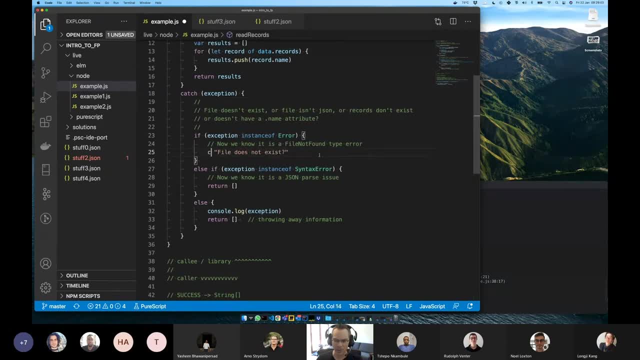 that would be weird if records were set to now a string, to now a string, to now a string, um. or are you saying let's log it and um? or are you saying let's log it and um? or are you saying let's log it and hope he looks at the console? 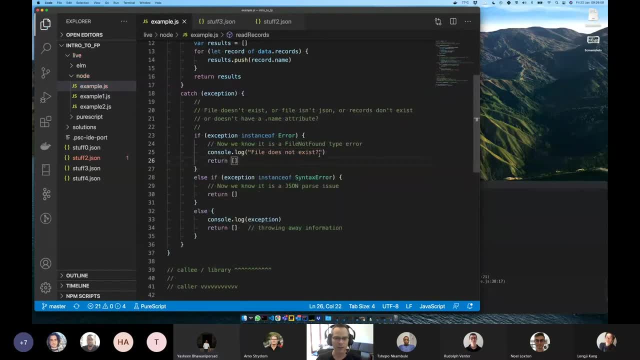 hope he looks at the console, hope he looks at the console. consolelog file does not exist and consolelog file does not exist and consolelog file does not exist and then return, then return, then return thing, or just return nothing here or thing, or just return nothing here or 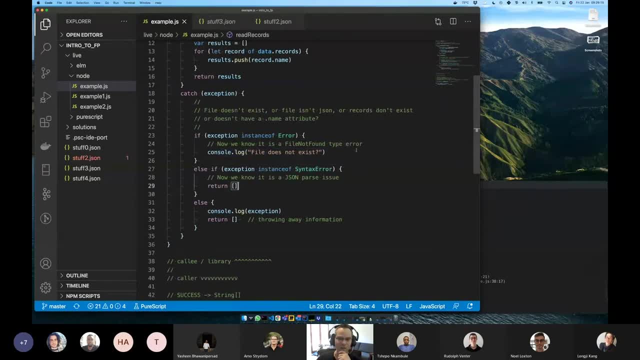 thing, or just return nothing here, or how. how do you propose, how? how do you propose how? how do you propose informing the caller that his file does, informing the caller that his file does, informing the caller that his file does not exist, not exist, not exist. that's kind of what i was asking. not, not. 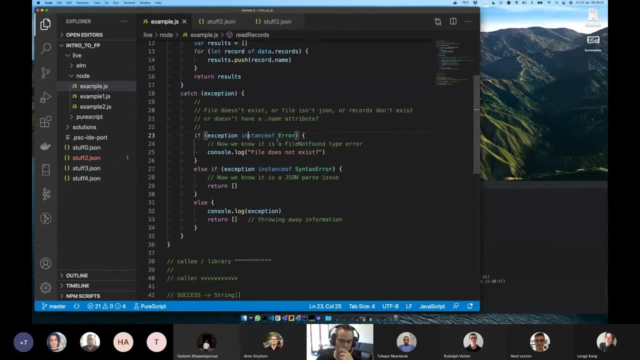 that's kind of what i was asking, not. not that's kind of what i was asking, not not how to handle it. i i think we there's how to handle it. i i think we there's how to handle it. i i think we there's many ways of how to detect if the file 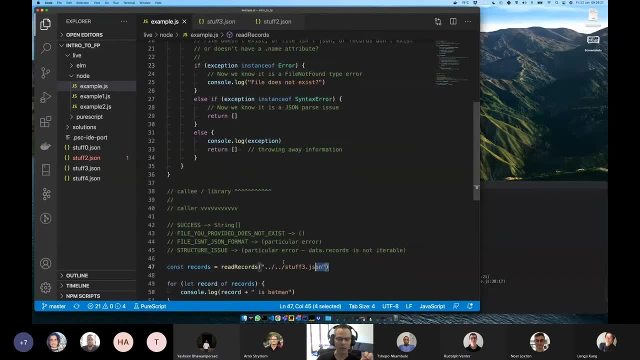 many ways of how to detect if the file. many ways of how to detect if the file doesn't exist. that's totally fine. how do doesn't exist? that's totally fine. how do doesn't exist? that's totally fine. how do we tell the caller down here that his 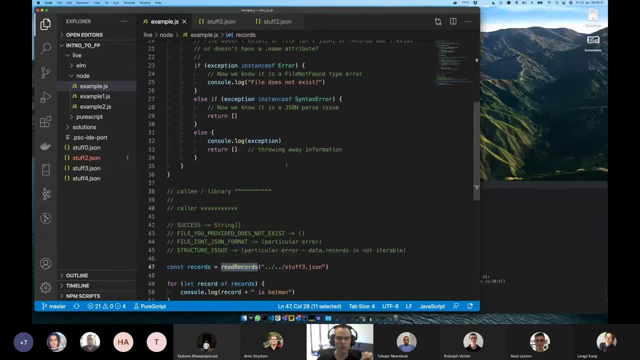 we tell the caller down here that his, we tell the caller down here that his file does not exist. file does not exist. file does not exist. given that all the only way we can, given that all the only way we can, given that all the only way we can communicate with him is through. 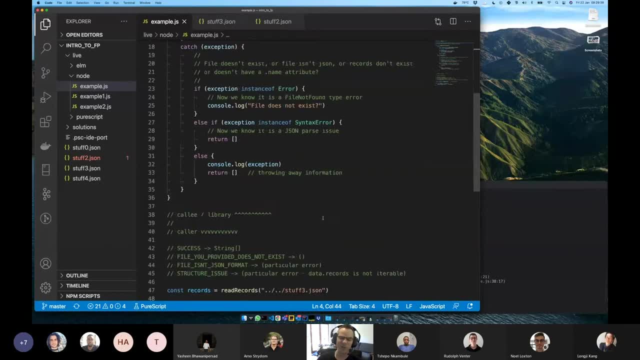 communicate with him is through. communicate with him is through the return value, or all raising an the return value, or all raising an the return value, or all raising an exception to him, which i think we're exception to him, which i think we're exception to him, which i think we're we're saying like let's forget that, that. 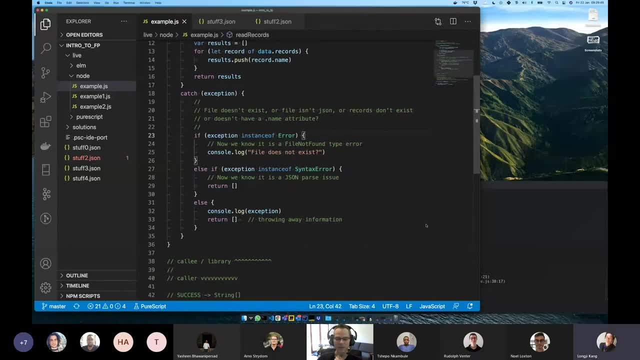 we're saying like, let's forget that. that we're saying like, let's forget that, that that particular one, yes, someone else, um, can we not maybe write the error? um. can we not maybe write the error? um. can we not maybe write the error message into the first item of the array? 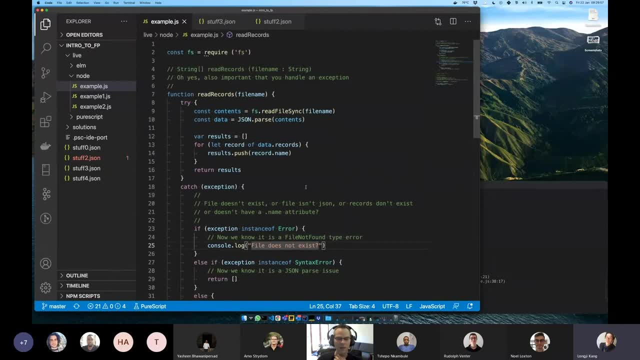 message into the first item of the array, message into the first item of the array, and then just maybe prefix it with, and then just maybe prefix it with, and then just maybe prefix it with error or something. yes, yes, yes, okay, so that's definitely. yes, yes, yes, okay, so that's definitely. 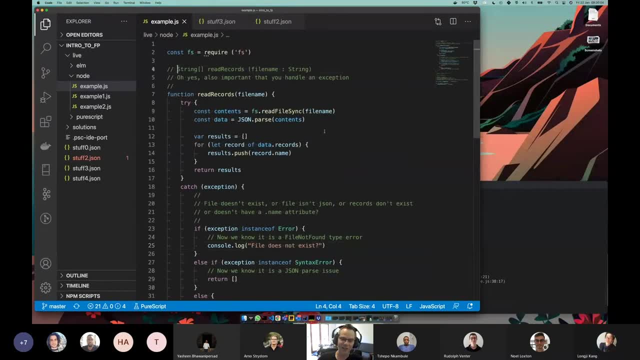 yes, yes, yes, okay, so that's definitely one one, one interesting direction that you're going interesting direction that you're going interesting direction that you're going so. so i quite like that actually, so, so, so i quite like that actually, so, so, so i quite like that actually. so, potentially, what you're saying is: 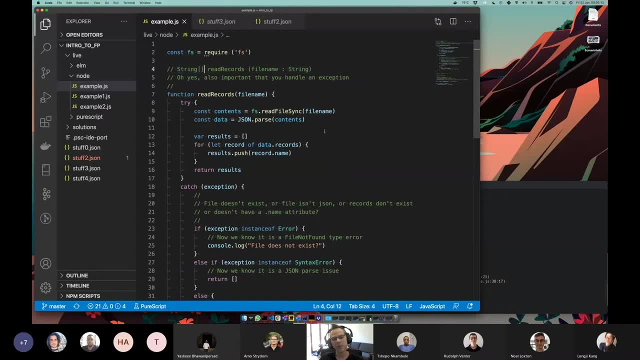 potentially what you're saying is. potentially what you're saying is like when we return this: okay. when like like when we return this: okay. when like like when we return this: okay. when like: whatever we return on this side, whatever we return on this side, whatever we return on this side. maybe there's like an error part as well. 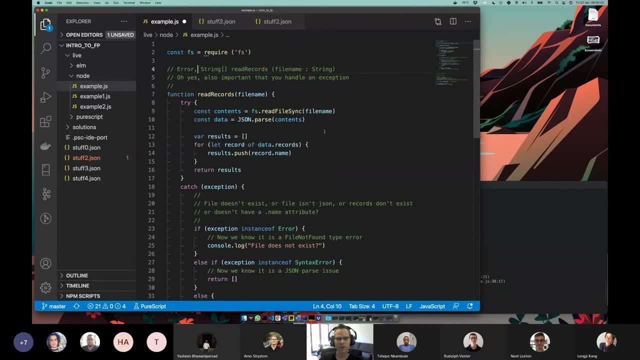 maybe there's like an error part as well, maybe there's like an error part as well, as like a success part, as like a success part, as like a success part. right, and he can check for this right and he can check for this right and he can check for this error part. 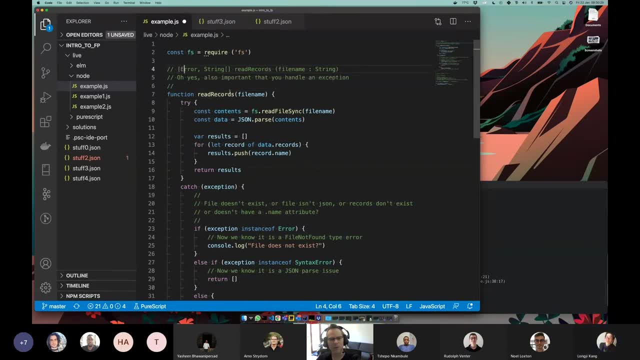 error part. error part kind of first, if that kind of makes kind of first, if that kind of makes kind of first, if that kind of makes sense, so, sense, so, sense, so, and probably the way with javascript to and probably the way with javascript to and probably the way with javascript to do that is like you make that. 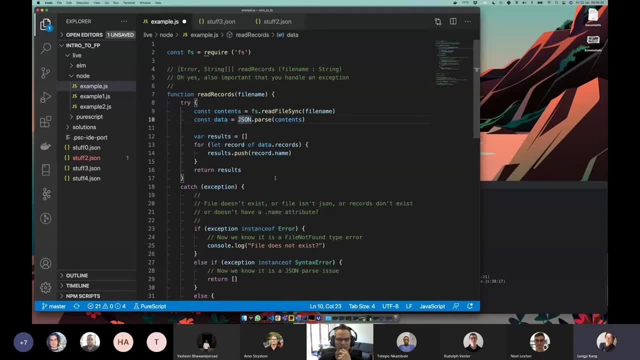 do. that is like you make that do. that is like you make that whole thing an array right, whole thing, an array right, whole thing, an array right. yeah, i think that's sort of what you're. yeah, i think that's sort of what you're. yeah, i think that's sort of what you're saying. so, 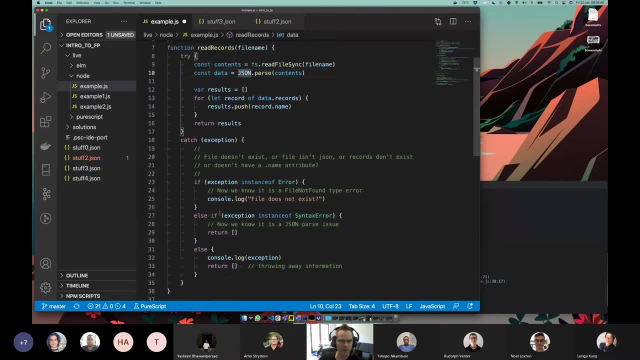 saying so, saying so: okay, well, so i i don't think that's a bad, okay, well, so i i don't think that's a bad, okay, well, so i i don't think that's a bad, uh, start. so. so let's uh start. so so let's. 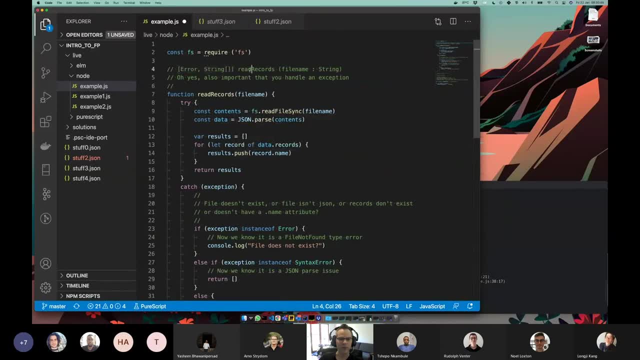 uh, start, so so let's, let's go there. um so, given now this, let's go there. um so, given now this, let's go there. um so, given now this, signature, signature, signature. read records now can return an error. an. read records now can return an error: an. 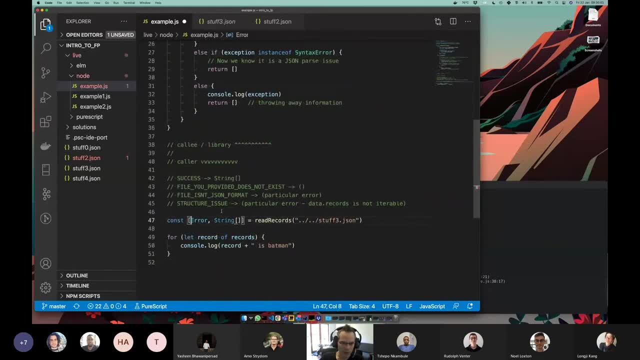 read records now can return an error. an error and a thingy. let's just paste that error and a thingy. let's just paste that error and a thingy. let's just paste that down here. so we know that down here. so we know that down here. so we know that this would be our. i don't know if. 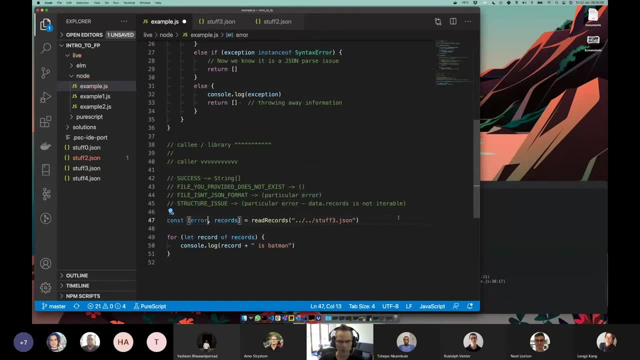 this would be our. i don't know if this would be our. i don't know if javascript will destructure like this. javascript will destructure like this. javascript will destructure like this. maybe it would, maybe it would, maybe it would. uh, error equals something like that. i. 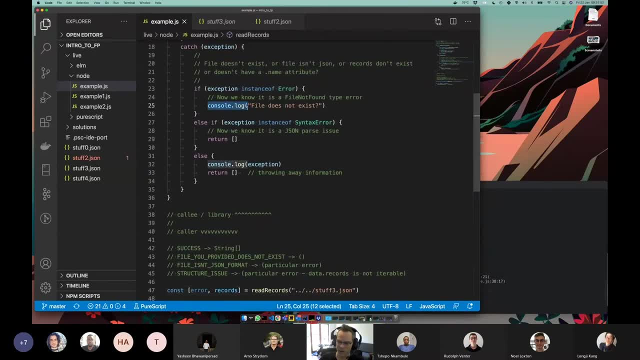 uh error equals something like that. i uh error equals something like that. i think it would think it would think it would. so we can now say like oh yes, so. so we can now say like oh yes, so. so we can now say like: oh yes, so on, in this scenario, hey, dude your file. 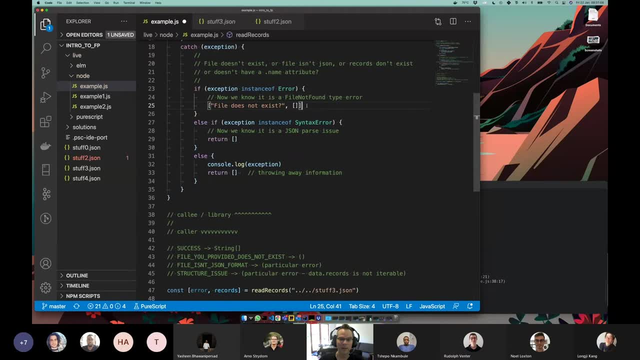 on in this scenario: hey, dude, your file on in this scenario. hey, dude, your file does not exist, does not exist, does not exist, and, and actually i'm going to give you and, and actually i'm going to give you and, and actually i'm going to give you back an empty. 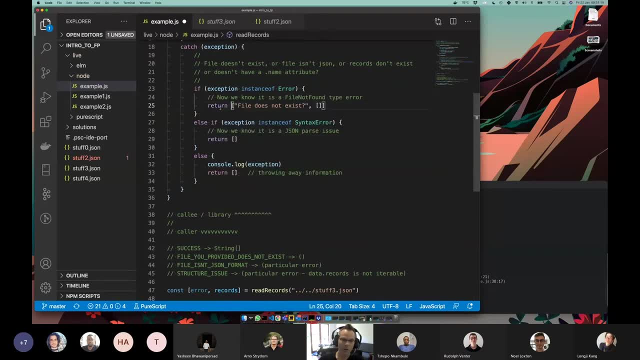 back an empty back, an empty list of things, right? sorry, that should list of things, right. sorry that should list of things, right. sorry that should say return, say, return, say, return, um and the same. here, this is like uh. um and the same here, this is like uh. 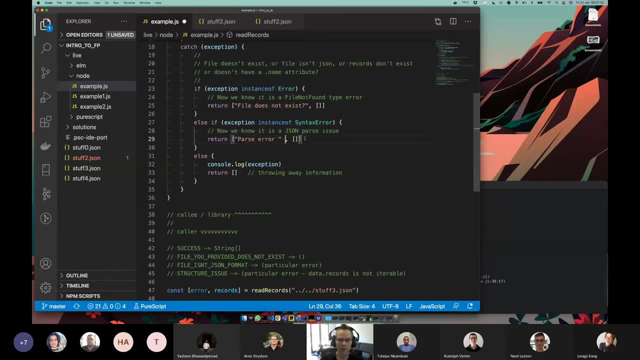 um, and the same here. this is like: uh, pause, pause, pause, error or something, and maybe let's be error or something. and maybe let's be error or something and maybe let's be cool, cool, cool by giving him the exception text over, by giving him the exception text over. 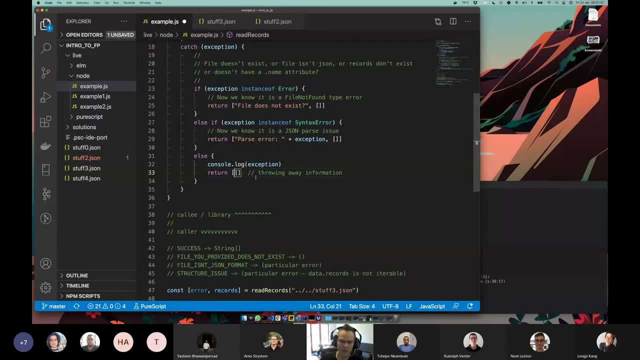 by giving him the exception text over there: right pause error. everything else there, right pause error. everything else there, right pause error. everything else is like um. unknown is like um. unknown is like um unknown. error for now, uh, we're not sure. but error for now? uh, we're not sure. but 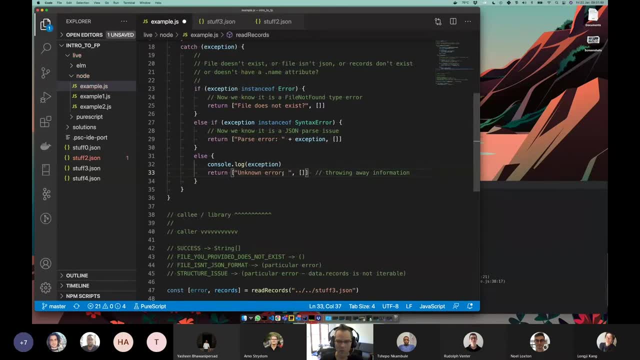 error for now. uh, we're not sure, but there could be other kinds of errors, for there could be other kinds of errors, for there could be other kinds of errors for now, right now, right now, right, so maybe we should go plus. so, maybe we should go plus. 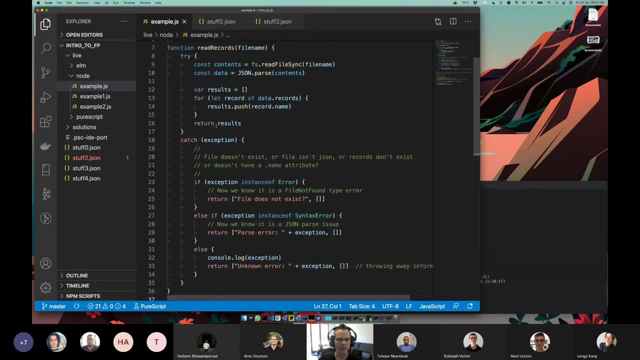 so maybe we should go plus exception, right so that way, and okay so exception, right so that way, and okay so, exception, right so that way, and okay. so then in our successful then, in our successful then, in our successful case, we want to return like null there case. we want to return like null there. 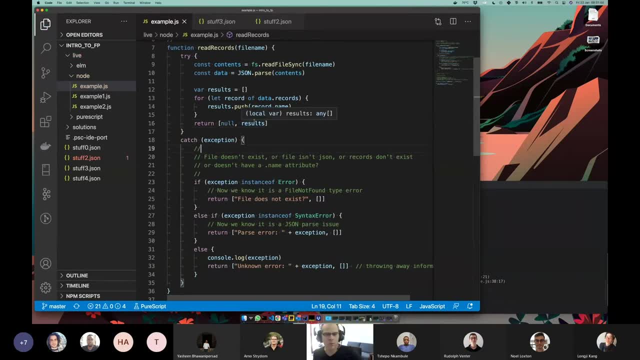 case, we want to return like null: there was no error, was no error, was no error. and here's your list of your list of: and here's your list of your list of, and here's your list of your list of results: results, results. happy with that? i think that that's not. 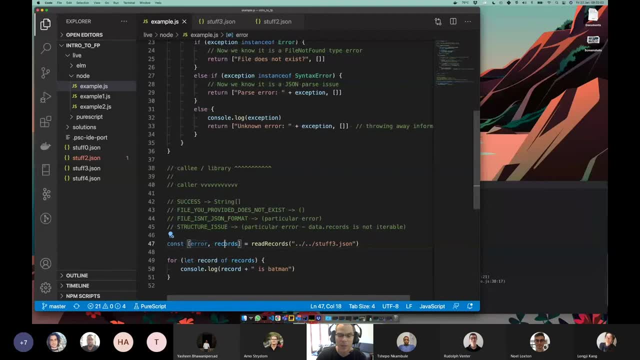 happy with that? i think that that's not happy with that. i think that that's not a bad. a bad, a bad first stab actually, because now, now we first stab actually, because now, now we first stab actually, because now, now we are, now we are kind of saying to the 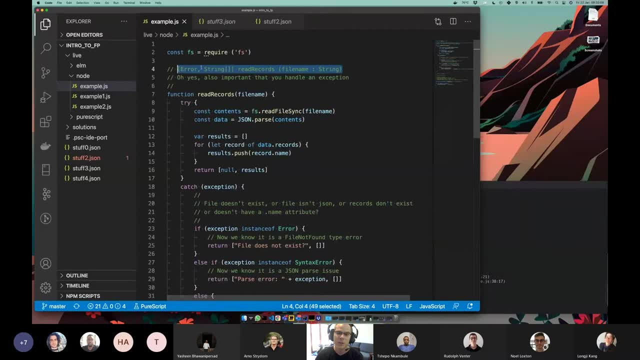 are. now we are kind of saying to the are. now we are kind of saying to the dude like: oh, check there could be errors. dude like: oh, check there could be errors. dude like: oh, check there could be errors. so when he reads his signature, he goes. so when he reads his signature, he goes. 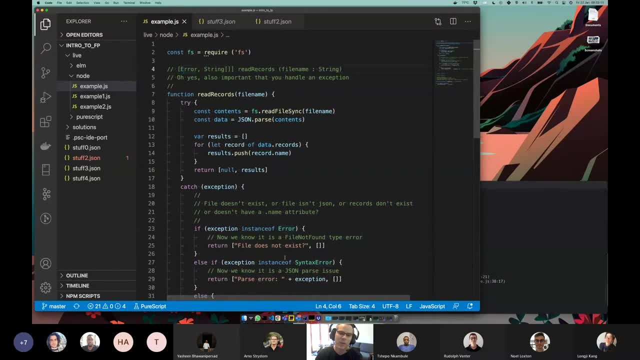 so when he reads his signature, he goes: yeah, i can get my string of thingies. yeah, i can get my string of thingies. yeah, i can get my string of thingies here, um, but also i should be careful of here, um, but also i should be careful of. 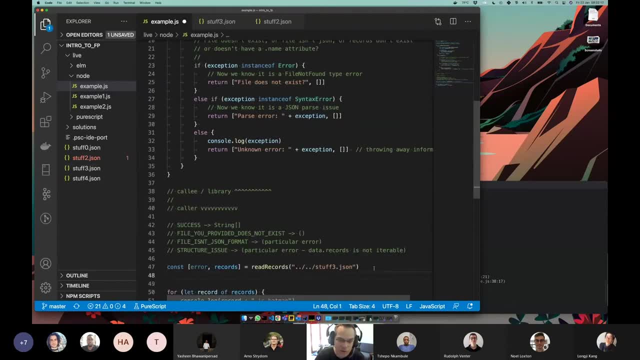 here, um, but also i should be careful of errors there, errors there, errors there, um, and then he is kind of forced, so i um, and then he is kind of forced, so i um, and then he is kind of forced. so i suppose he could still just do this. 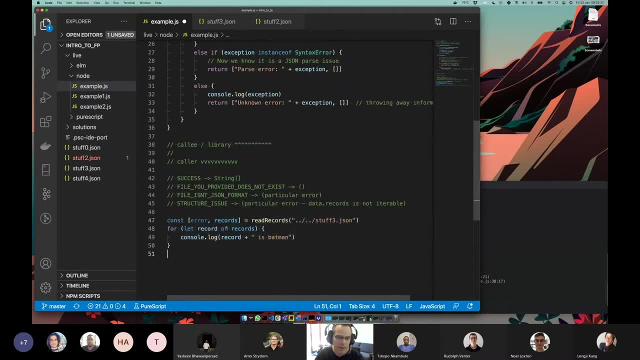 suppose he could still just do this. suppose he could still just do this right. he could just do this um run his right. he could just do this um run his right. he could just do this um run his code, and stuff may break, or he may code and stuff may break, or he may. 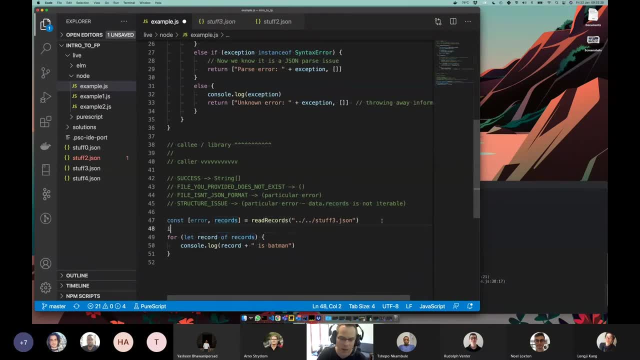 code and stuff may break. or he may assume that you know that it's empty. assume that you know that it's empty. assume that you know that it's empty- batman's, but at least he could check batman's, but at least he could check batman's. but at least he could check. like, if error, you know, then whatever you. 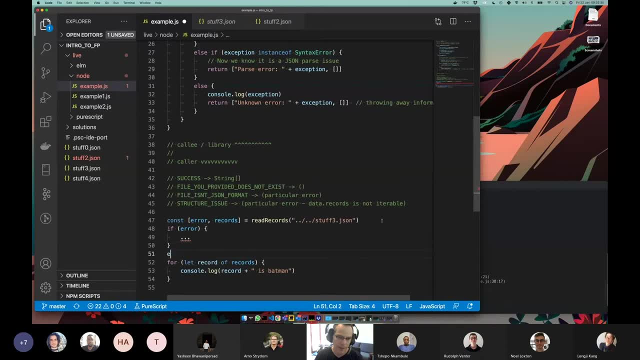 like: if error you know, then whatever you like, if error you know, then whatever you know, do stuff with that error know. do stuff with that error know. do stuff with that error um else. printers like everything was um else. printers like everything was um else. printers like everything was good. 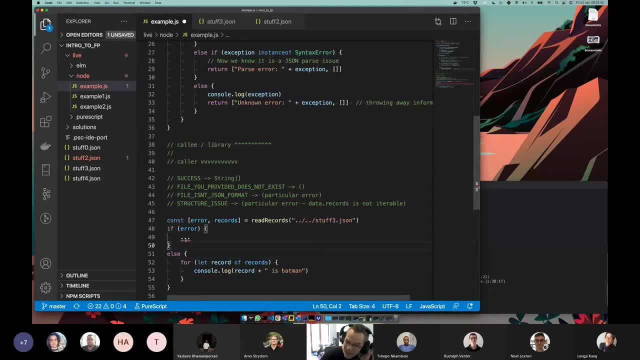 good, good, and print my batman's right does that, and print my batman's right does that and print my batman's right. does that kind of make sense? i'm not sure whether kind of make sense. i'm not sure whether kind of make sense. i'm not sure whether this will actually work. and do we even? 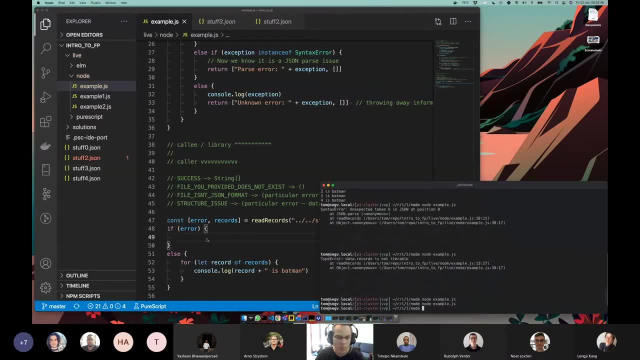 this will actually work, and do we even this will actually work? and do we even care if it works? care if it works, care if it works. um, we're just trying to illustrate the um. we're just trying to illustrate the um. we're just trying to illustrate the kind of the point. um, maybe it actually 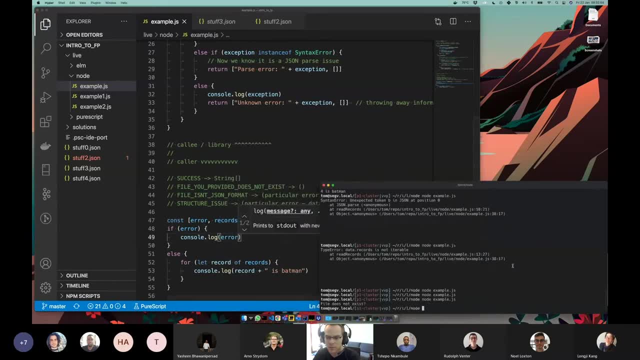 kind of the point: um, maybe it actually kind of the point, um, maybe it actually does work, does work, does work. uh, let's go consolelog error, right. uh, let's go consolelog error, right. uh, let's go consolelog error, right. yeah, file does not exist, so so that's. 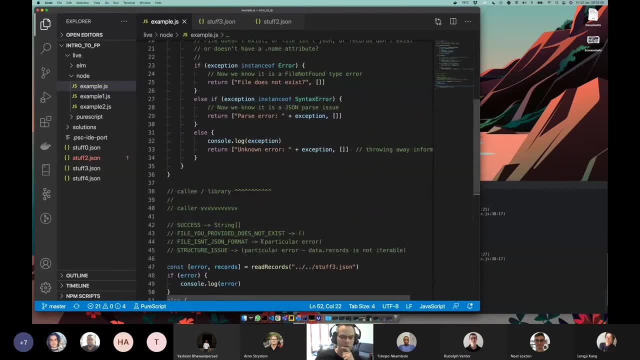 yeah, file does not exist, so so that's. yeah, file does not exist, so so that's pretty cool, pretty cool, pretty cool. check. we wrote good code- yeah, um. so so i check. we wrote good code- yeah, um, so so i check. we wrote good code- yeah, um, so. so i think that this is certainly improved. 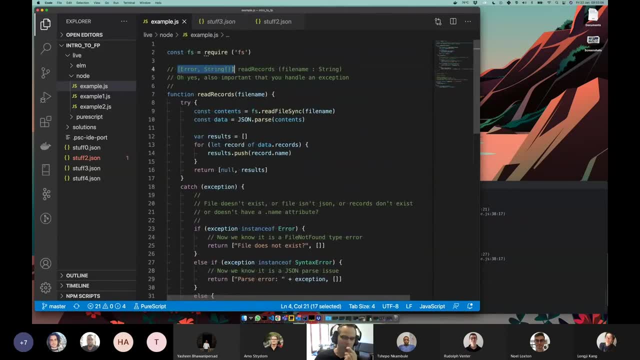 think that this is certainly improved, think that this is certainly improved stuff. i'm not sure if this kind of idea stuff. i'm not sure if this kind of idea stuff. i'm not sure if this kind of idea does this, does this, does this? any javascript programmers out there this? 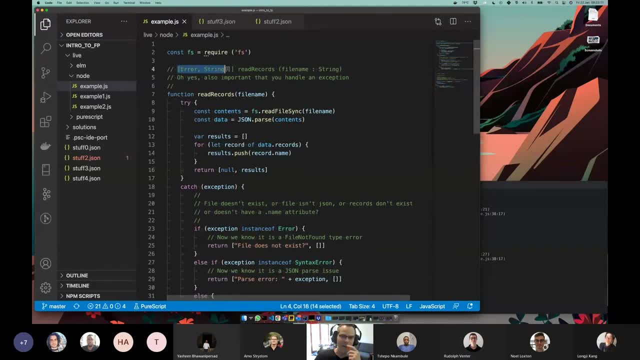 any javascript programmers out there, this, any javascript programmers out there, this, this kind of pattern, may, this kind of pattern, may this kind of pattern may look recognizable, um, look recognizable, um. look recognizable, um. in other places, so often in javascript, in other places, so often in javascript, in other places, so often in javascript, there's this concept of 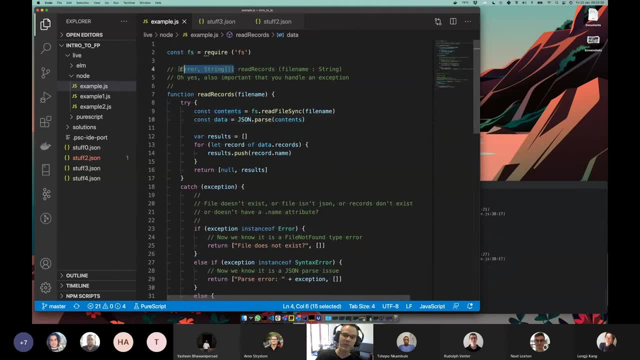 there's this concept of, there's this concept of callbacks right um to provide you data, callbacks right um to provide you data, callbacks right um to provide you data, and often callbacks have this kind of, and often callbacks have this kind of, and often callbacks have this kind of signature, where the first 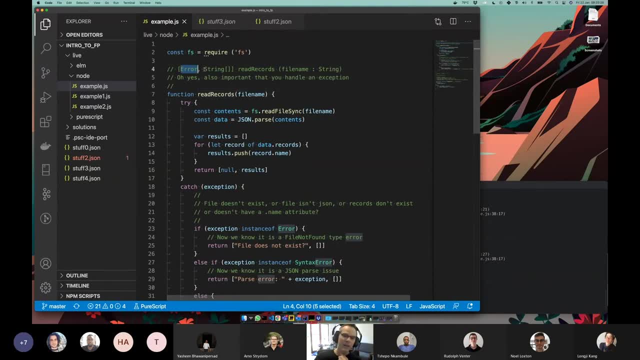 signature, where the first signature, where the first parameter to the callback is like a parameter to the callback, is like a parameter to the callback, is like a potential error, potential error, potential error and the other, and and then subsequent and the other, and and then subsequent and the other and and then subsequent parameters are like the successful cases. 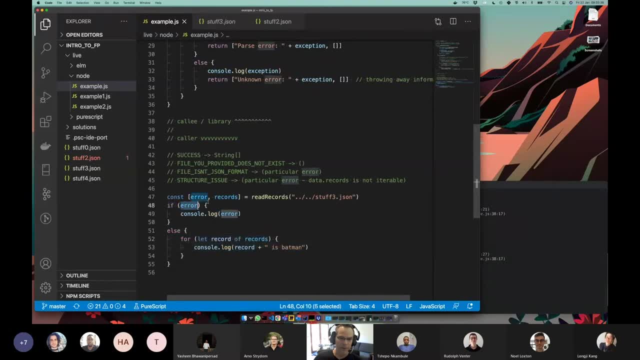 parameters are like the successful cases. parameters are like the successful cases and it leads to a whole lot of code that and it leads to a whole lot of code that, and it leads to a whole lot of code that looks like this, looks like this, looks like this. um, you know, checking, checking the error. 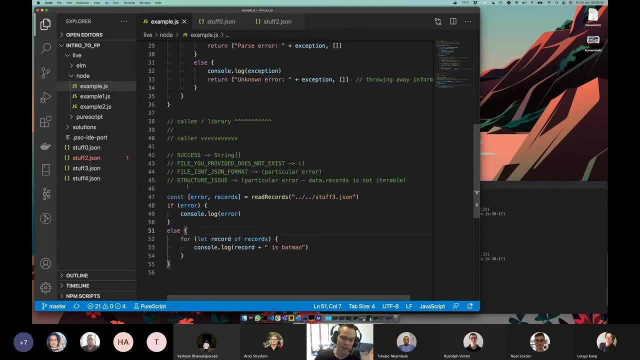 um, you know, checking, checking the error, um, you know, checking, checking the error, um, if that kind of makes sense, um, if that kind of makes sense, um, if that kind of makes sense, so anyway, like like this is certainly one. so anyway, like like this is certainly one. 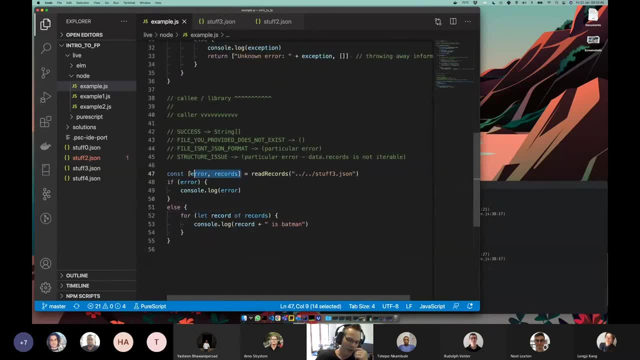 so anyway, like, like this is certainly one one good one, one good idea, the the one good one, one good idea, the the one good one, one good idea, the the kind of problem i would point out here, kind of problem i would point out here, kind of problem i would point out here, or whether it's a, um, an object, because or whether it's a? um an object because, or whether it's a? um an object because you could also say hey, like, why don't we? you could also say hey like, why don't we? you could also say hey like, why don't we make this an object? 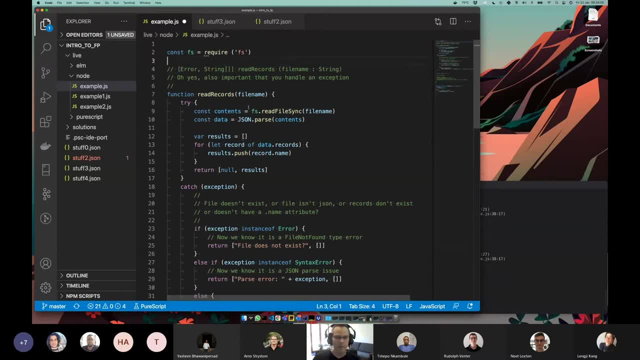 make this an object. make this an object could make it maybe more explicit. we could make it maybe more explicit. we could make it maybe more explicit. we could return, could return, could return potentially- uh well, it's actually just potentially. uh well, it's actually just potentially. uh well, it's actually just right. it's like: 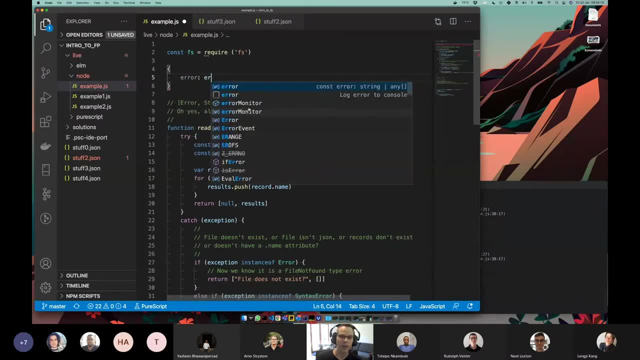 right, it's like right, it's like. this is maybe what it looks like, but it's. this is maybe what it looks like, but it's. this is maybe what it looks like, but it's like error with an error, like error with an error, like error with an error. you know the actual string, or it could be. 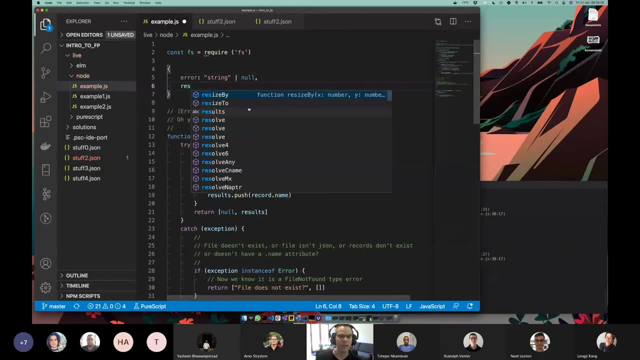 you know the actual string or it could be. you know the actual string or it could be null right. so if we think about its null right, so if we think about its null right, so if we think about its types, types, types, um, otherwise, the results which could be 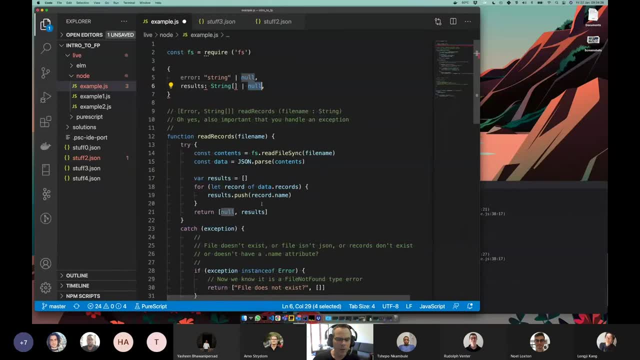 um, otherwise the results which could be, um, otherwise the results which could be: you know a string array, or potentially you know a string array, or potentially you know a string array, or potentially null. actually, if null, actually, if null, actually, if there is an error, because maybe when 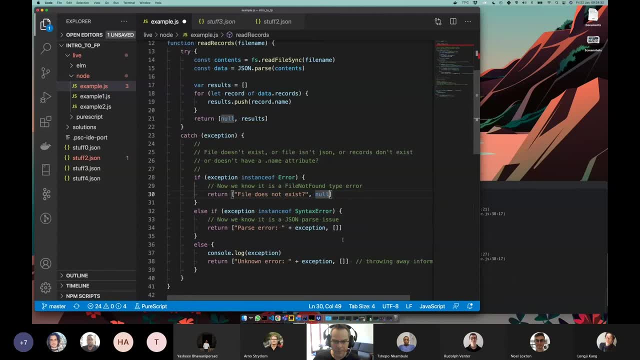 there is an error, because maybe when there is an error, because maybe when things are successful, maybe we'd choose things are successful, maybe we'd choose things are successful, maybe we'd choose to go null there, i don't know. to go null there, i don't know. 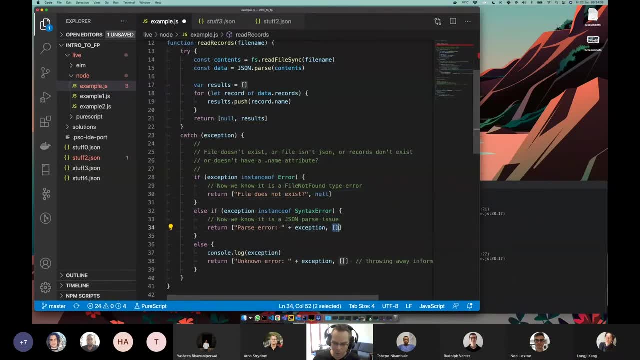 to go null there, i don't know. and that way at least we would hurt the, and that way at least we would hurt the, and that way at least we would hurt the person, person, person calling it um. if he just tried to calling it um, if he just tried to. 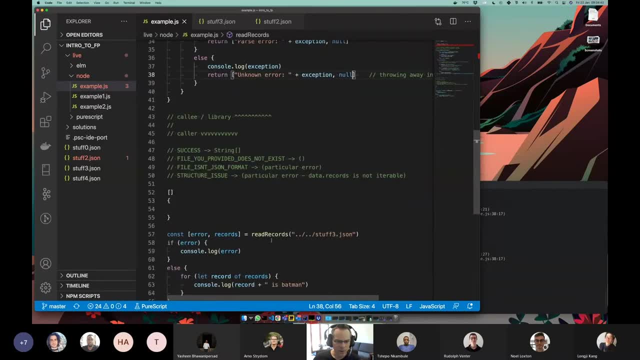 calling it. um, if he just tried to iterate over it, iterate over it, iterate over it, right, so if he just went, if he called right, so, if he just went, if he called right, so, if he just went, if he called this thing and this thing was null. 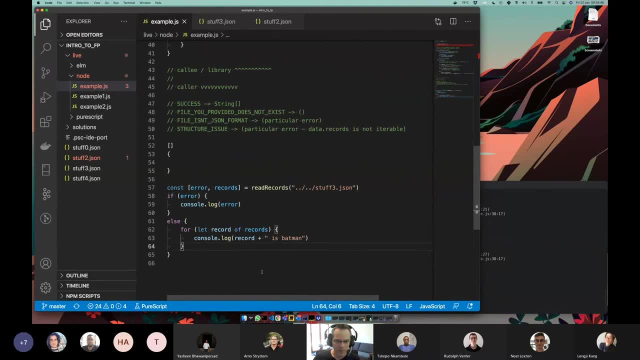 this thing and this thing was null. this thing and this thing was null. he is kind of forced to check for the. he is kind of forced to check for the. he is kind of forced to check for the error before he just iterates through error, before he just iterates through. 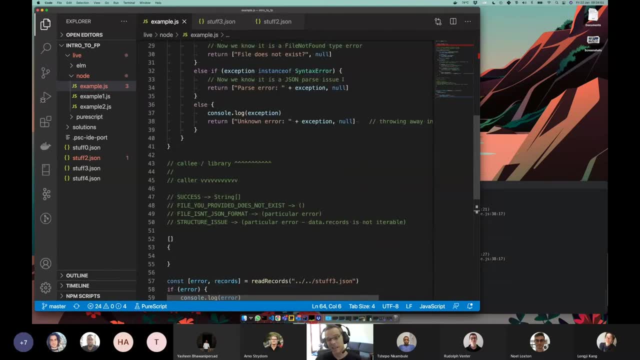 error before he just iterates through them and assumes that they're that them, and assumes that they're that them, and assumes that they're that they're okay, and and i would say, yeah, i, they're okay. and and i would say, yeah, i, they're okay. and and i would say, yeah, i don't know if that, if, i'm happy with. 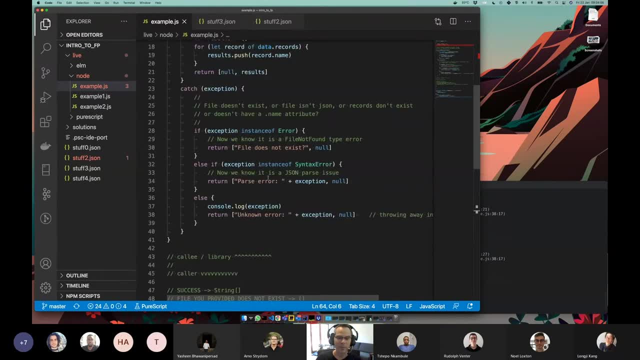 don't know if that, if i'm happy with. don't know if that, if i'm happy with that. prefer not to hurt, hurt the callers that. prefer not to hurt. hurt the callers that prefer not to hurt. hurt the callers, um, i prefer to make you know, force them. 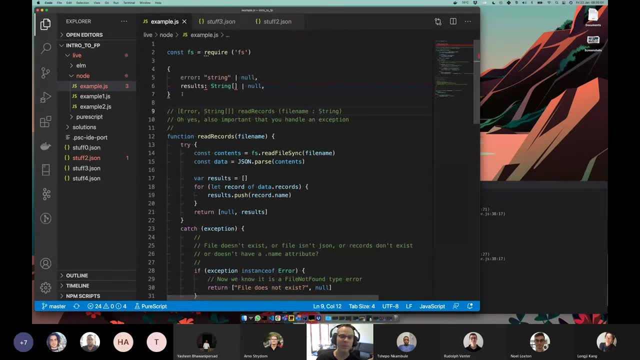 um, i prefer to make you know, force them. um, i prefer to make you know, force them to handle it, handle errors anyway. um, but to handle it, handle errors anyway. um, but to handle it, handle errors anyway. um, but if you think about the types, if you think about the types, 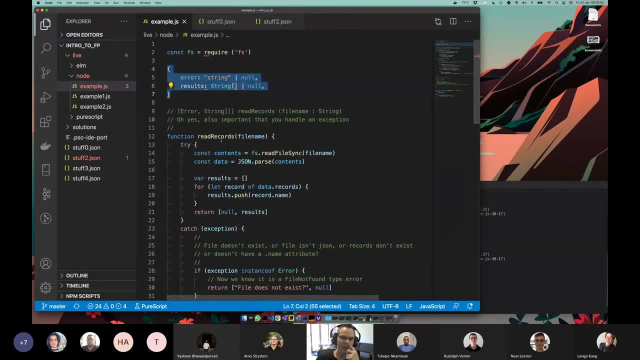 if you think about the types: um, it's kind of this, right, so we're. um, it's kind of this, right so we're. um, it's kind of this, right so we're building the. the return type to this building, the. the return type to this building, the. the return type to this function is, like this object, which can: 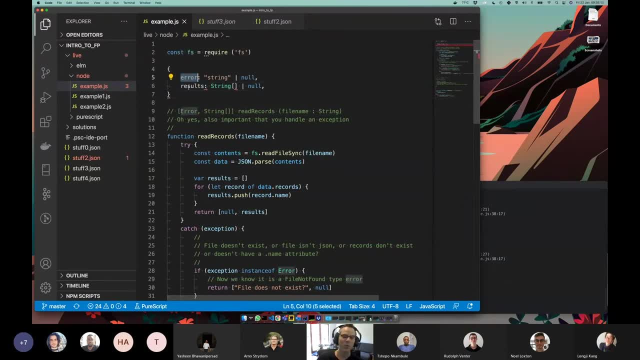 function is like this object which can function, is like this object which can have kind of two different states: either have kind of two different states, either have kind of two different states. either this error type state or this like this error type state, or this like this error type state, or this like successful. 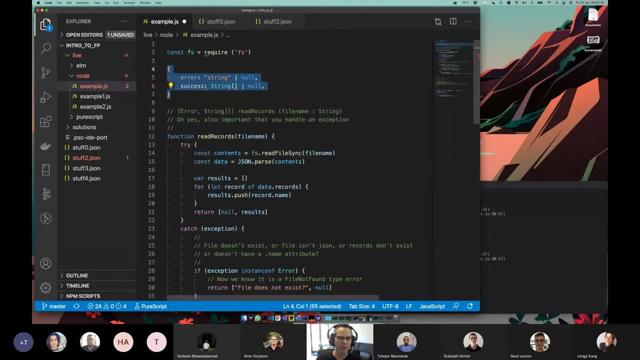 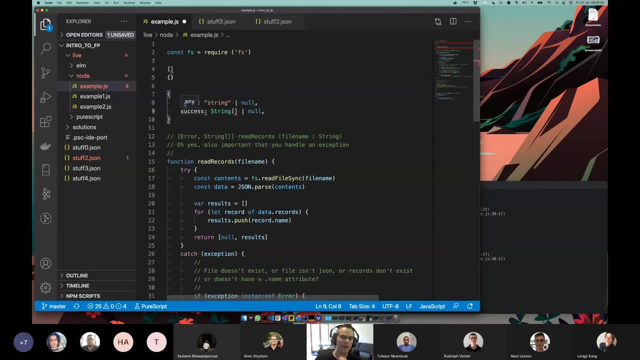 successful, successful type state right and unfortunately, with type state right. and unfortunately with type state right and unfortunately with the. the data structures we have in the. the data structures we have in the. the data structures we have in javascript: either an array javascript, either an array javascript, either an array or a or an object. 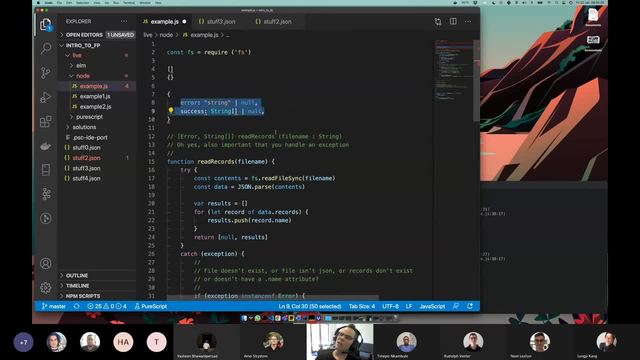 or a or an object, or a or an object. it's always both of them. does that make it's always both of them? does that make it's always both of them? does that make sense? there's no. there's no real sense. there's no, there's no real. 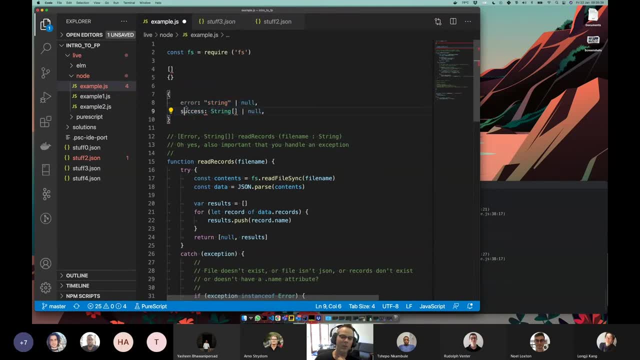 sense. there's no, there's no real primitive way of saying this is an, or primitive way of saying this is an or primitive way of saying this is an or type relationship. does that make sense? type relationship- does that make sense? type relationship- does that make sense like i want an error or i want a success? 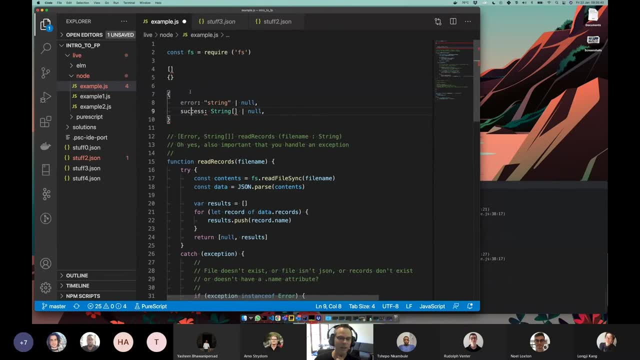 like i want an error or i want a success. like i want an error or i want a success, i don't want both and i don't want none. i don't want both and i don't want none. i don't want both and i don't want none. you know what i mean, because if i think, 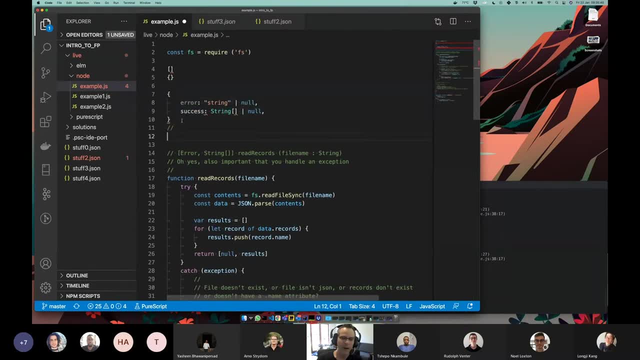 you know what i mean, because, if i think. you know what i mean, because if i think about like, about, like, about, like what. what is acceptable here, um i. what is acceptable here, um i. what is acceptable here, um i? i? would be okay, that error is set to null. 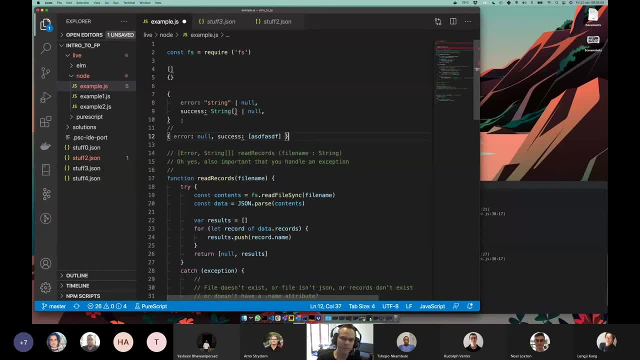 i would be okay that error is set to null. i would be okay that error is set to null and success is set to some array of, and success is set to some array of, and success is set to some array of stuff right, stuff, right, stuff, right. that one is okay, um. 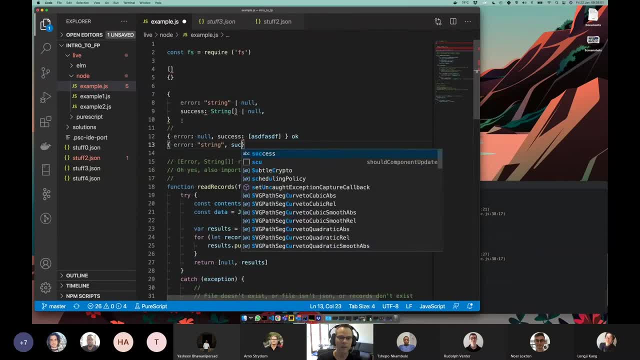 that one is okay. um, that one is okay. um, error being set to something, some string error being set to something, some string error being set to something, some string and success being null, or, and success being null or and success being null or empty, like that's also okay and that's. 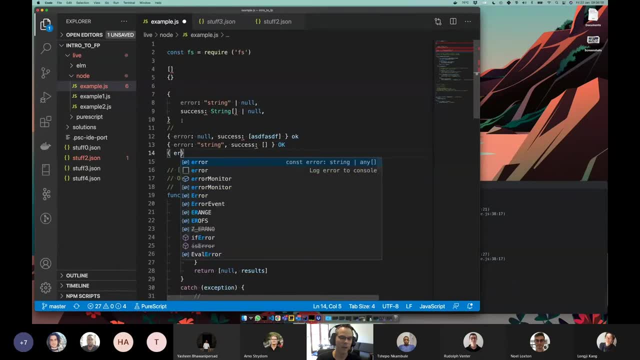 empty, like that's also okay, and that's empty, like that's also okay and that's expected, expected, expected. however, there's a situation here which, however, there's a situation here which, however, there's a situation here which is like a weird one, which would be, is like a weird one, which would be okay with that, and i'm not, and and i. 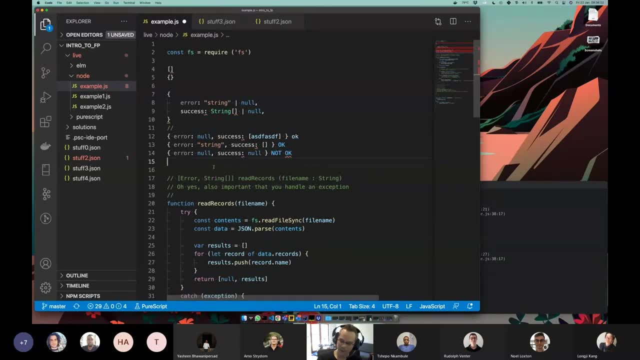 okay with that, and i'm not, and and i okay with that, and i'm not, and and i don't want my caller don't want my caller don't want my caller to have to deal with this situation, um to have to deal with this situation um. 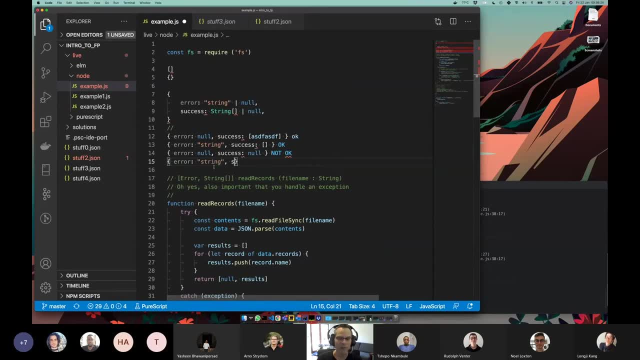 to have to deal with this situation. um, the other one is like where error is. the other one is like where error is. the other one is like where error is something and something and something and success is something, success is something, success is something. success has got stuff in it. this is also. 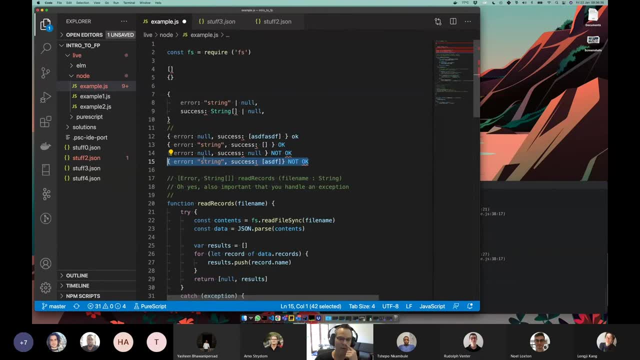 success has got stuff in it. this is also success has got stuff in it. this is also not okay, right, not okay, right, not okay right. this is a scenario that i don't want to. this is a scenario that i don't want to. this is a scenario that i don't want to support, but yet i am, so when i write. 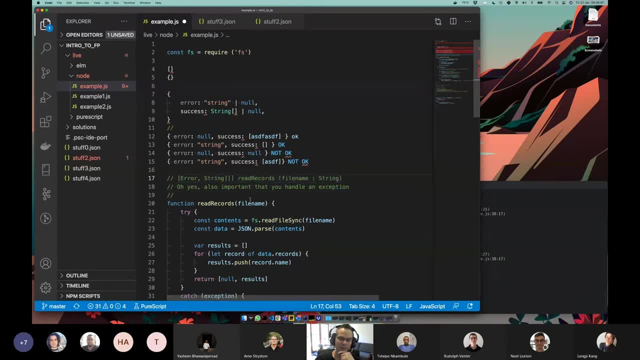 support, but yet i am so when i write support. but yet i am so when i write this, this, this, um, this sort of function signature, um, this sort of function signature, um, this sort of function signature. i'm. i can't encode that into. i'm. i can't encode that into. 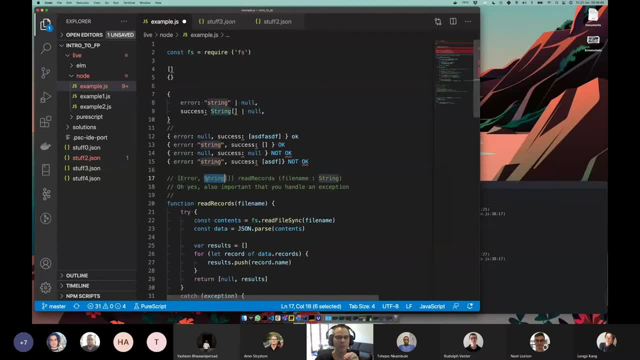 i'm. i can't encode that into. into this to say yeah, it's an error. or into this to say yeah, it's an error. or into this to say yeah, it's an error or it's a string. does that make sense? it's, it's a string. does that make sense? it's. 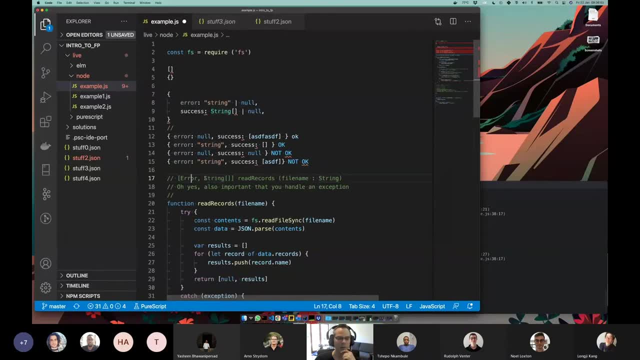 it's a string. does that make sense? it's always both. so what we have here is we always both. so what we have here is we always both. so what we have here is we have an and relationship. does that make have an and relationship, does that make? 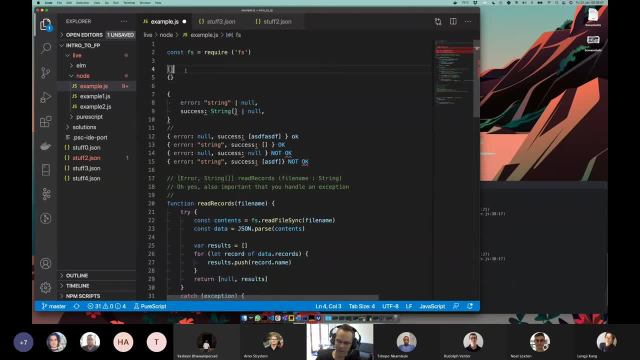 have an and relationship. does that make sense? so objects and arrays certainly sense. so objects and arrays certainly sense. so objects and arrays certainly are both, are both, are both and type things it's and type things it's and type things it's. it's. all the elements right and so. 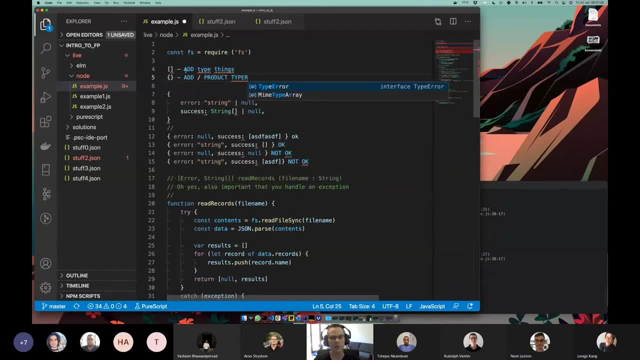 it's all the elements right. and so it's all the elements right. and so often this is called a product, often this is called a product, often this is called a product type. so it's a product type which means type. so it's a product type which means. 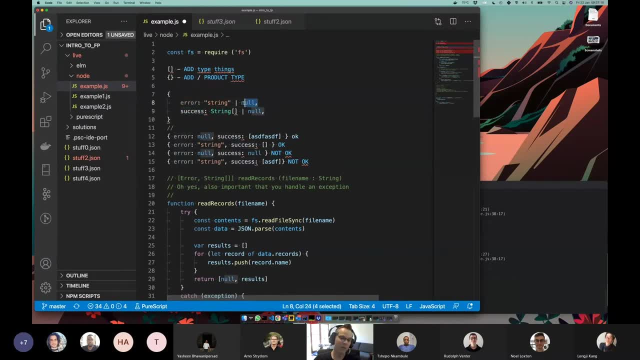 type. so it's a product type, which means it has to have both. it has an error and it has to have both. it has an error and it has to have both. it has an error and it has a success. of course we can set it. it has a success. of course we can set it. 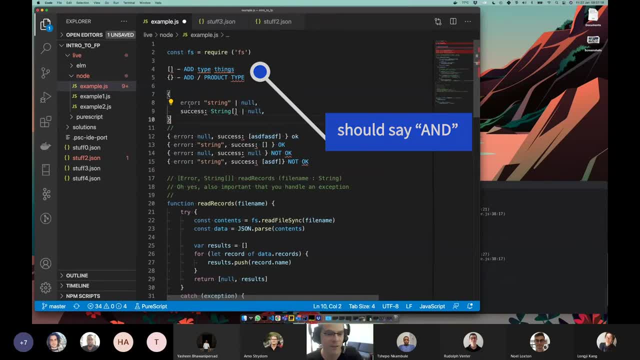 it has a success. of course, we can set it to null, but it's still there. and null to null, but it's still there and null is an absolutely first class value. right is an absolutely first class value. right is an absolutely first class value. right for error. um, this is getting a little. 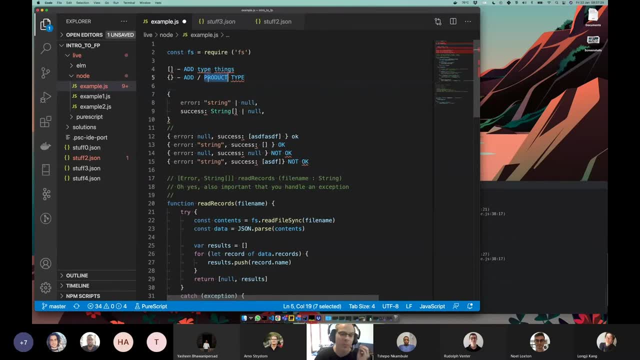 for error. um, this is getting a little for error. um, this is getting a little bit theoretical, but um bit theoretical but um bit theoretical, but, um, but i think it's good to know so knowing, but i think it's good to know so knowing, but i think it's good to know so knowing about product types or 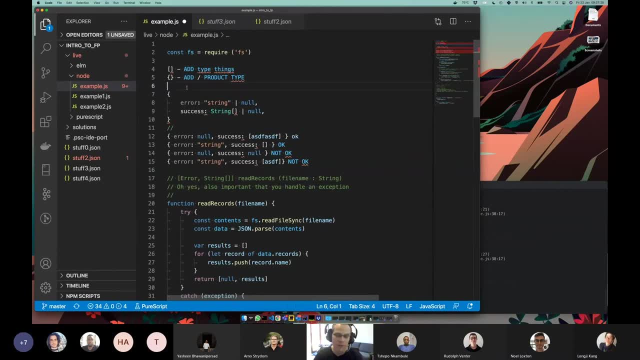 about product types, or about product types or and types. um, this is what most languages and types. um, this is what most languages and types. um, this is what most languages like c- sharp java, like c- sharp java, like c- sharp java, javascript, c and c, plus, plus, etc. 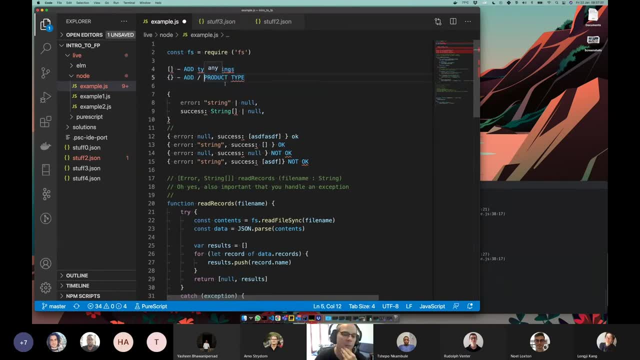 javascript c and c plus plus, etc. javascript c and c plus plus, etc. they all primarily, they all primarily, they all primarily use and in product types there's no use. and in product types there's no use. and in product types there's no natural or type. you may say that. 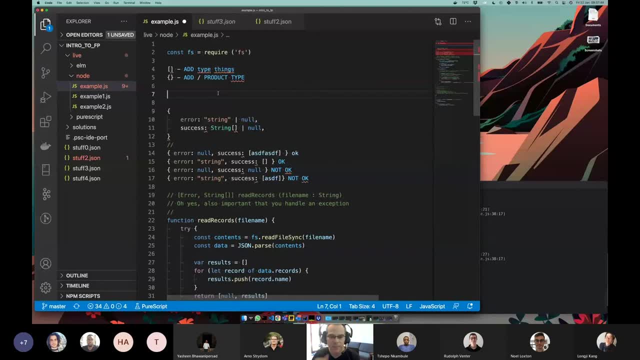 natural or type. you may say that natural or type, you may say that so, so so. there may be, though, so like, so, so so there may be, though, so like, so, so so. there may be, though, so like in um, in um, in um, in in c. you have this, this concept of a. 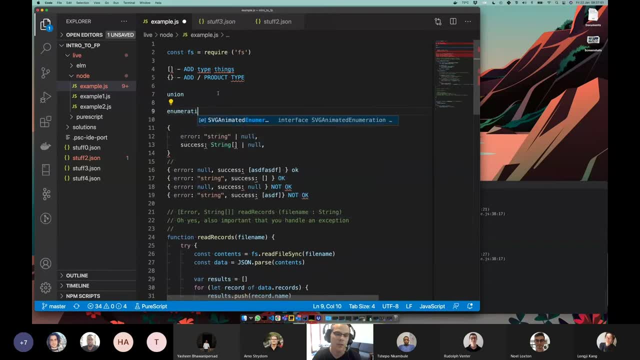 in in in c. you have this, this concept of a in in in c. you have this, this concept of a thing called a union, thing called a union, thing called a union. uh, you have a thing called an. uh, you have a thing called an. uh, you have a thing called an enumeration. 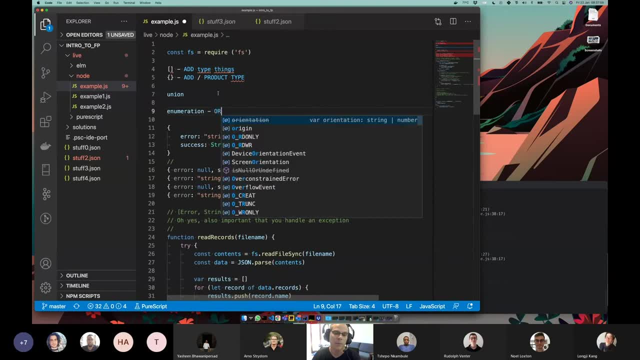 enumeration, enumeration, um, and these things are starting to be um, and these things are starting to be um, and these things are starting to be all types, so enumeration or a union. all types, so enumeration or a union. all types, so enumeration or a union is an all type. where you can, where you 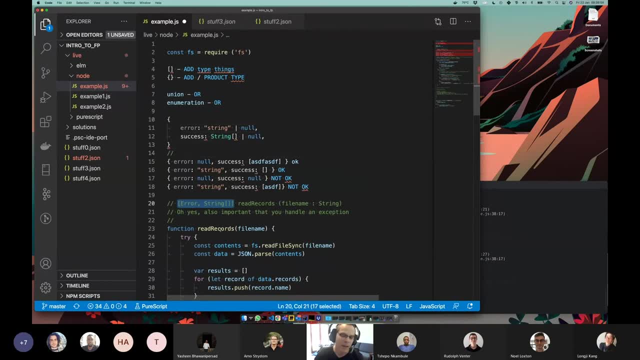 is an all type where you can, where you is an all type where you can, where you can encode here you could. i could say: can encode, here you could. i could say: can encode here you could. i could say: um, somehow in the encoding of this i um, somehow in the encoding of this, i. 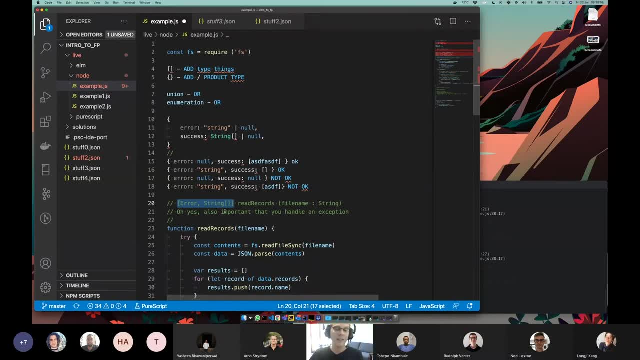 um, somehow in the encoding of this i could say it's an error, could say it's an error, could say it's an error or it's a string, it's not both and it's, or it's a string, it's not both and it's, or it's a string, it's not both and it's not none. so it can't be these two. 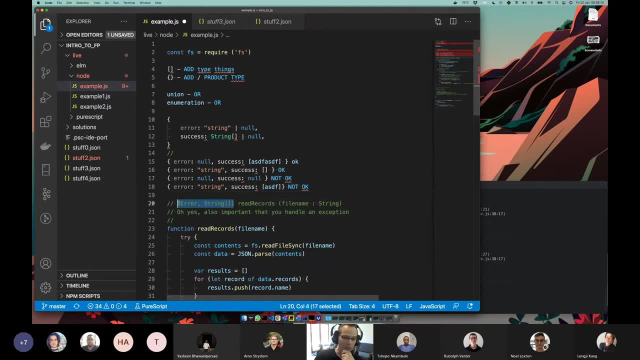 not none. so it can't be these two, not none. so it can't be these two scenarios, meaning that my caller can be scenarios, meaning that my caller can be scenarios. meaning that my caller can be very explicit about, very explicit about, very explicit about um, can explicitly know what my return. um can explicitly know what my return um can explicitly know what my return types are. does that kind of make sense types are? does that kind of make sense types are? does that kind of make sense? so these are all types are also called. so, these are all types are also called. 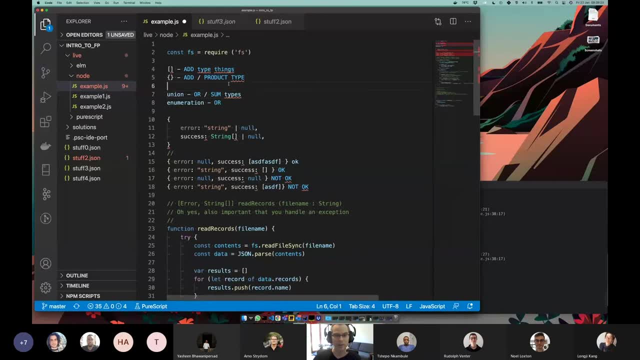 so these are all types, are also called: some types in more mathematical senses, some types in more mathematical senses, some types in more mathematical senses. so you have products. so if you think so, you have products. so if you think so, you have products. so if you think about, like: what does product mean? 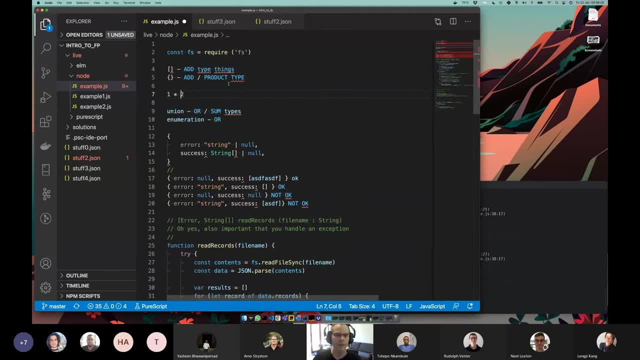 about like what does product mean? about like what does product mean. product means multiply right. product means multiply right. product means multiply, right. um, that's a product, right so product. um, that's a product, right so product. um, that's a product, right so product is one times two and the sum would be: 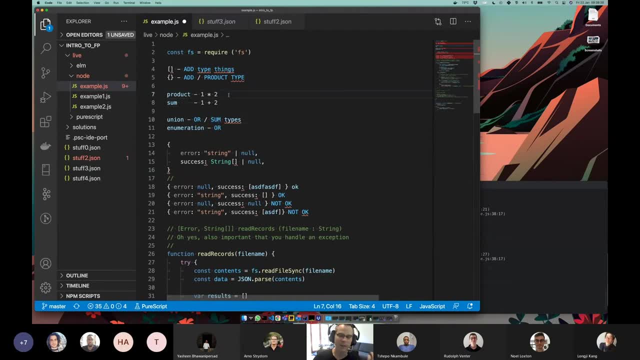 is one times two, and the sum would be: is one times two, and the sum would be one plus two right, and so why are they one plus two right? and so why are they one plus two right? and so why are they called sum and product types and and for. 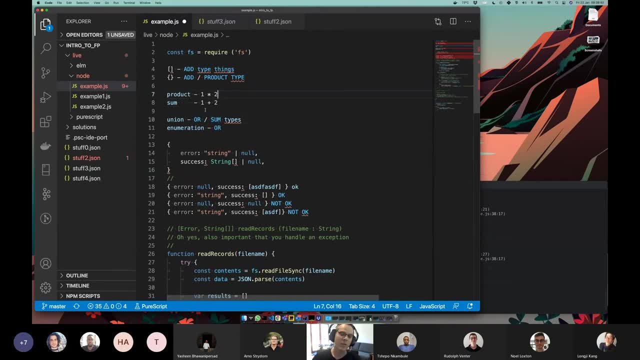 called sum and product types, and and for called sum and product types, and, and. for me it's very simple. it's like let's me it's very simple. it's like let's me it's very simple. it's like let's just work out the, the combinations of 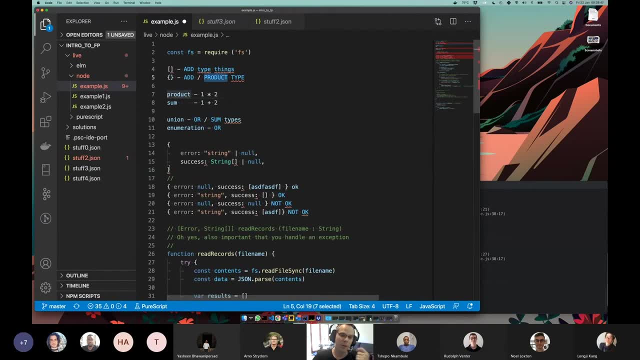 just work out the, the combinations of, just work out the, the combinations of, of um, of um, of um of a product type. so if you look at if of a product type, so if you look at if of a product type, so if you look at, if you look at this, you can see that this 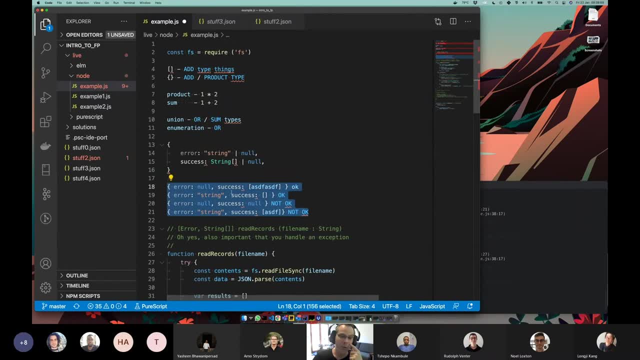 you look at this, you can see that this, you look at this, you can see that this is a permutation. and so how many is a permutation? and so how many is a permutation? and so how many permutations are there? there's kind of permutations are there? there's kind of? 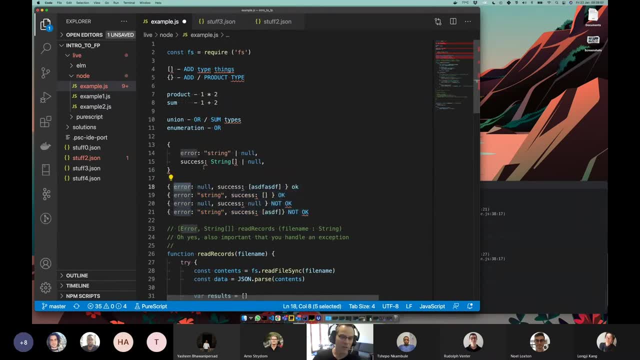 permutations are there. there's kind of four permutations. so it's like there four permutations, so it's like there four permutations. so it's like there were two potential values for error, were two potential values for error, were two potential values for error it's null or string. success has got. 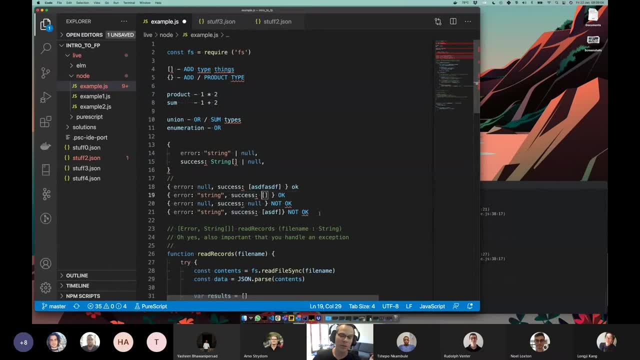 it's null or string success has got. it's null or string success has got either null or an array, so that's two, either null or an array, so that's two. either null or string. success has got two times by two: there are four. times by two, there are four. 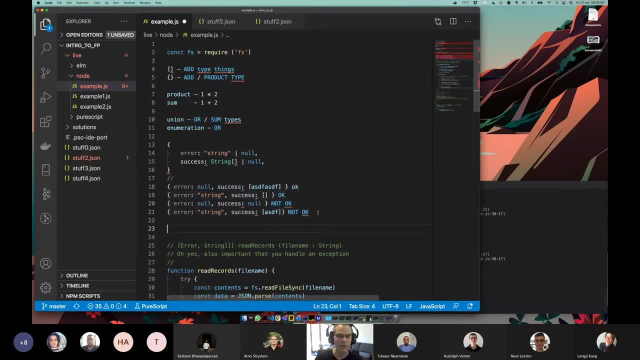 times by two, there are four permutations. what we really wanted was permutations. what we really wanted was permutations. what we really wanted was: we wanted um a. we wanted um a. we wanted um a. some type where we say we only want, some type where we say we only want. 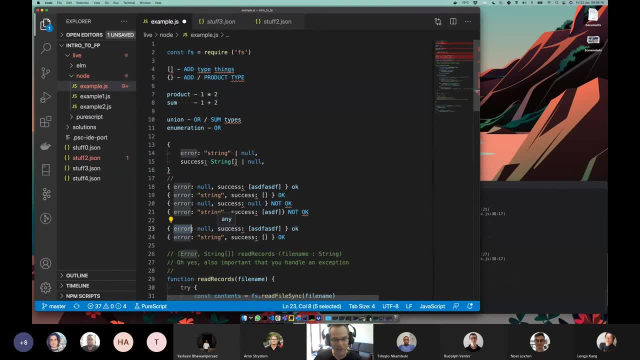 some type where we say: we only want these two, we only want, so we want one, these two, we only want, so we want one, these two, we only want. so we want one permutation plus one permutation, permutation plus one permutation, permutation plus one permutation: meaning we've got two possible states. 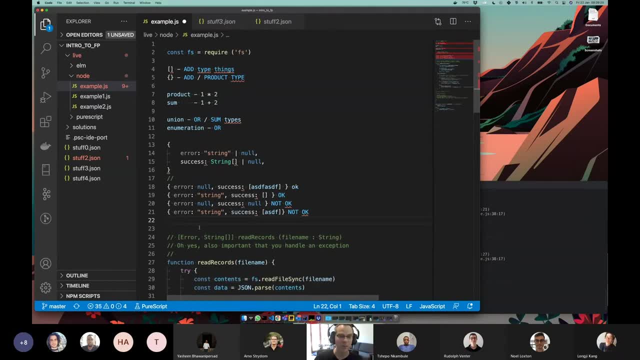 meaning we've got two possible states. meaning we've got two possible states so so often when we and so so often when we and so so often when we. and apologies getting too theoretical, but apologies getting too theoretical, but apologies getting too theoretical, but it's cool to know this kind of stuff to. 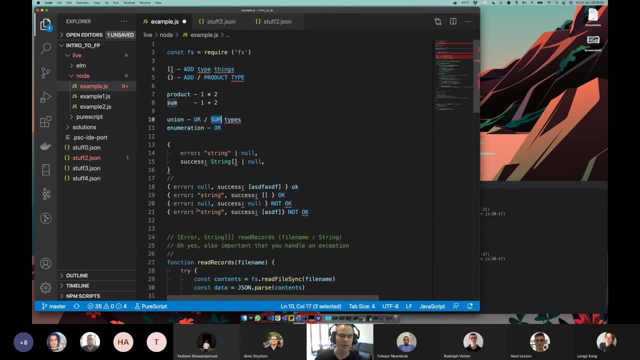 it's cool to know this kind of stuff to. it's cool to know this kind of stuff to look for in a language. look for the look for in a language. look for the look for in a language. look for the concept of what is a sum type. 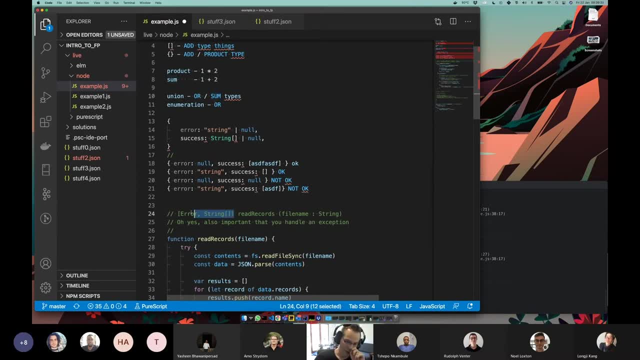 concept of what is a sum type, concept of what is a sum type, um, and that can sometimes give you um, and that can sometimes give you um and that can sometimes give you a good way of writing more explicit, a good way of writing more explicit, a good way of writing more explicit stuff here. so, unfortunately, in 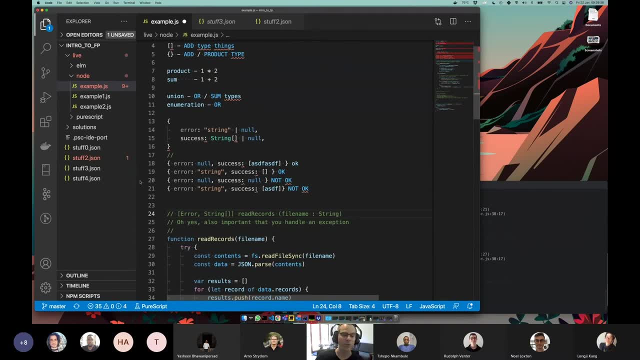 stuff here, so unfortunately, in stuff here, so unfortunately in javascript, there's no such thing really. javascript, there's no such thing really. javascript, there's no such thing really. i mean, you can kind of make up your own. i mean, you can kind of make up your own. 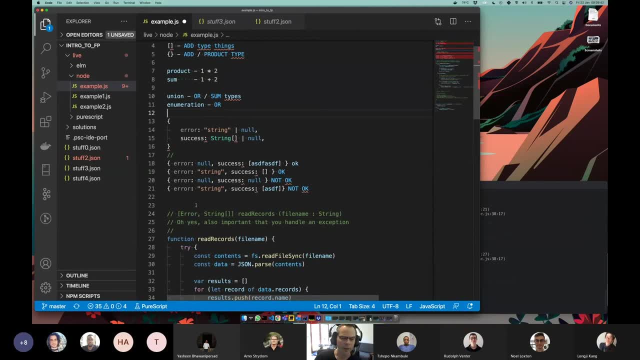 i mean you can kind of make up your own some type. i suppose, um there's no real some type i suppose, um there's no real some type, i suppose, um there's no real native one. so maybe one way of achieving native one. so maybe one way of achieving. 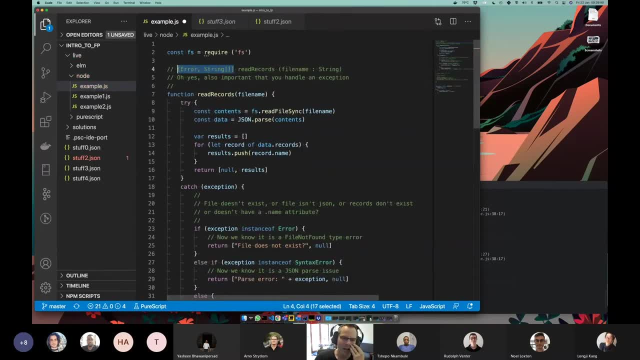 native one. so maybe one way of achieving achieving it, though, is to say well, okay. achieving it, though, is to say well, okay. achieving it, though is to say, well, okay, so our return type here we can't encode, so our return type here we can't encode, so our return type here we can't encode enough into this thing. so is there? 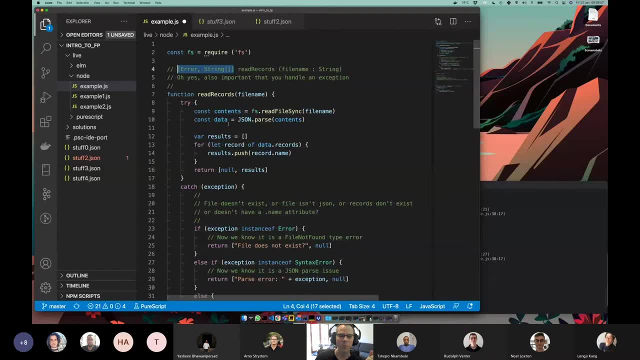 enough into this thing. so is there enough into this thing? so is there another place where we could encode more, another place where we could encode more, another place where we could encode more, more, more, more stuff into this, into this, more, more, more, more stuff into this, into this? 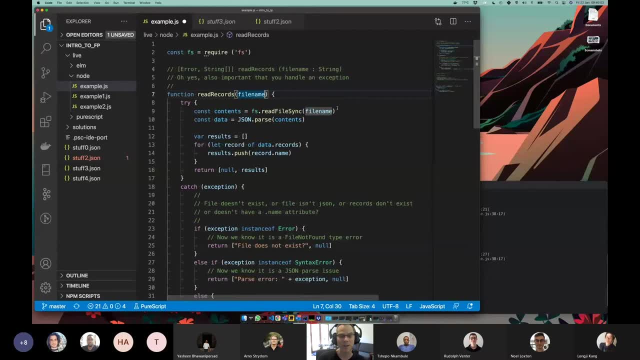 more, more, more stuff into this, into this function, and yes, there is, and so this function, and yes, there is. and so this function, and yes, there is. and so this might be like a little bit surprising, might be like a little bit surprising, might be like a little bit surprising, but because this is um javascript. 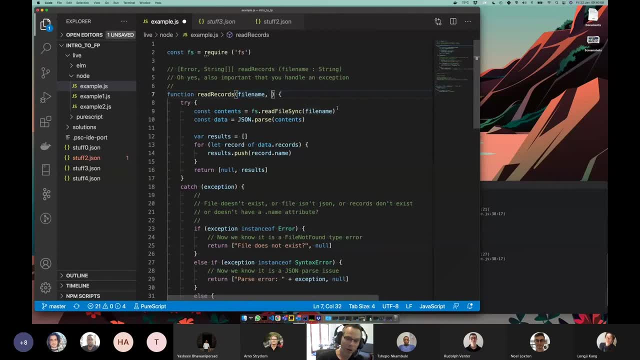 but because this is um javascript, but because this is um javascript, supports, supports, supports um first class functions, we could pass um first class functions. we could pass um first class functions. we could pass a function in here from like a callback, a function in here from like a callback. 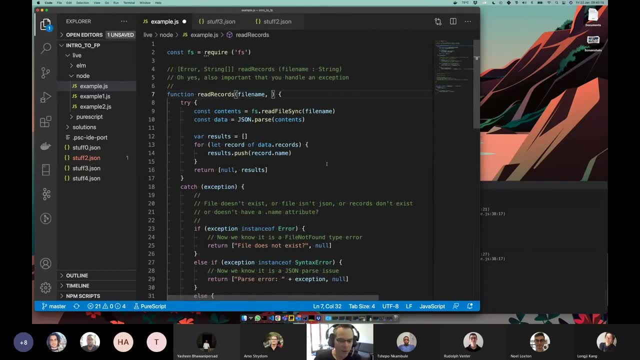 a function in here from like a callback perspective, which would then allow us to perspective, which would then allow us to perspective, which would then allow us to encode a particular thing, and, and so encode a particular thing, and and so encode a particular thing, and, and so what. i'll go through it quickly and 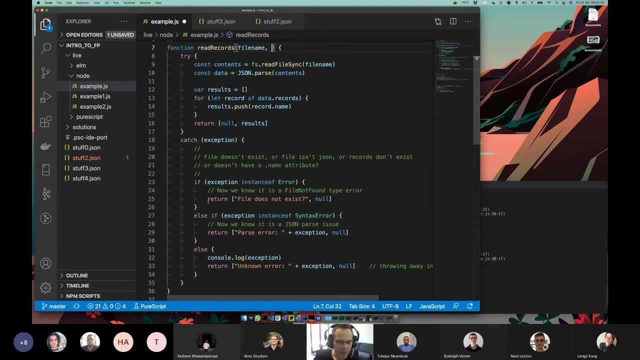 what? i'll go through it quickly, and, and so what? i'll go through it quickly and we'll just quickly implement it. we'll just quickly implement it. we'll just quickly implement it and then explain it later. but and then explain it later, but and then explain it later. but let's do this actually. so what we want to, 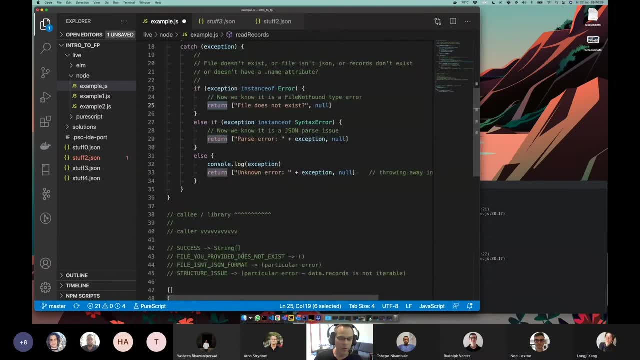 let's do this actually. so what we want to, let's do this actually. so what we want to do, do, do is: if the file doesn't exist, we want to is: if the file doesn't exist, we want to is: if the file doesn't exist, we want to notify this guy down here that his file 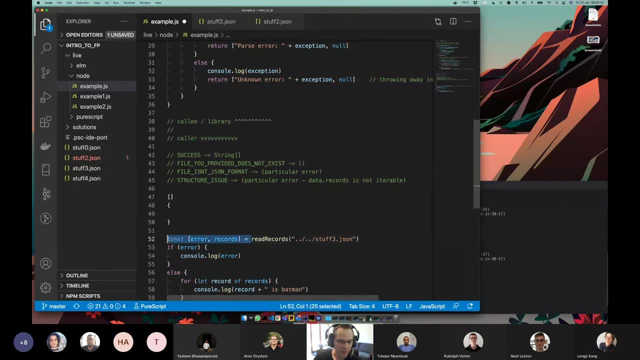 notify this guy down here that his file. notify this guy down here that his file doesn't exist. so effectively we're going doesn't exist. so effectively we're going doesn't exist. so effectively we're going to do it like: let me just rewrite this. to do it like: let me just rewrite this. 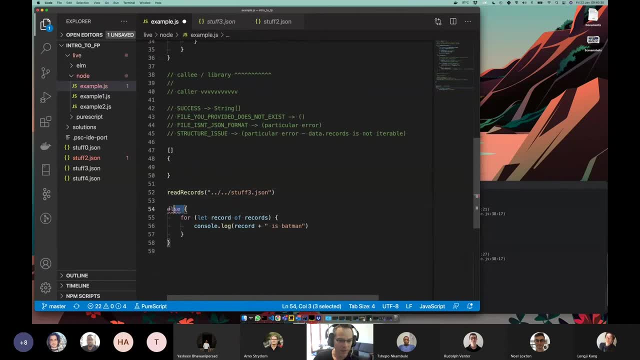 to do it like: let me just rewrite this actually, and then maybe it'll be more actually, and then maybe it'll be more actually, and then maybe it'll be more explicit, explicit, explicit. so we don't like any of this, this is all. so we don't like any of this, this is all. 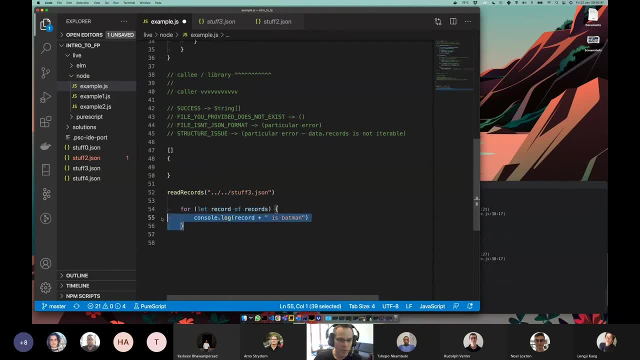 so we don't like any of this. this is all broken. it's not broken, but um broken. it's not broken, but um broken. it's not broken, but um. it's too simple, so effectively what we. it's too simple, so effectively, what we. it's too simple, so effectively, what we want to do. 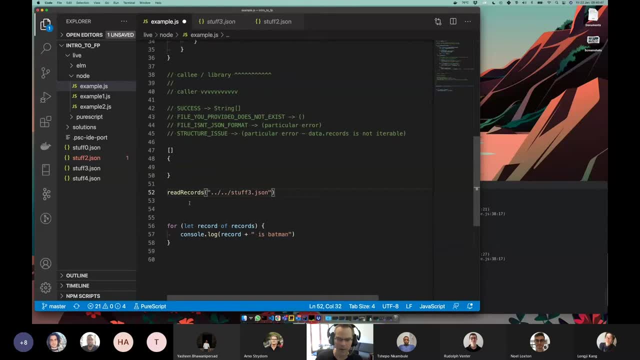 want to do, want to do with our javascript? is we want to say with our javascript? is we want to say with our javascript? is we want to say, yes, we want to give you this, yes, we want to give you this, yes, we want to give you this thingy here? but what we want to know is: 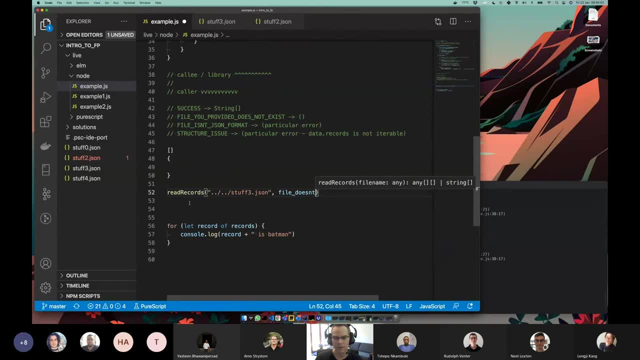 thingy here. but what we want to know is, if the file doesn't, if the file doesn't, if the file doesn't doesn't exist, then and i think we go doesn't exist then, and i think we go doesn't exist then, and i think we go like this: 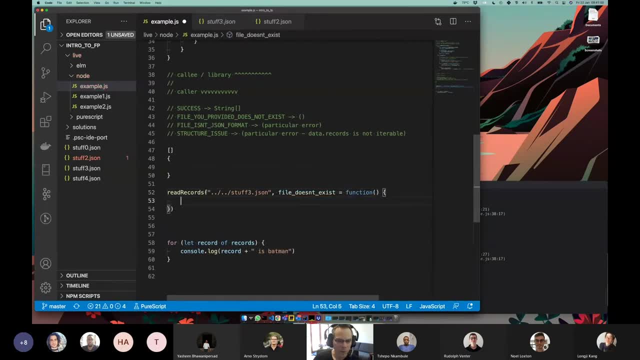 like this, like this: please call this function. so we're, please call this function. so we're please call this function. so we're going to pass callbacks into going to pass callbacks, into going to pass callbacks into our into our read records function. our into our read records function. 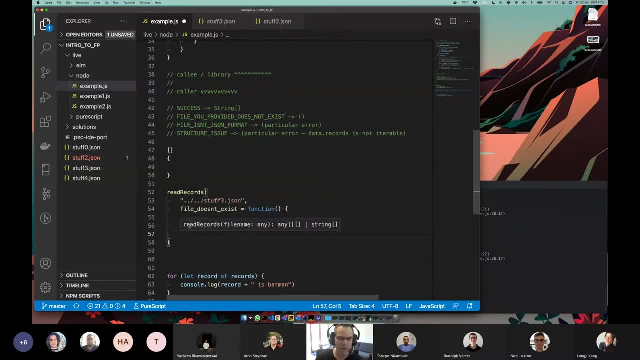 our into our read records function which is going to encode us and give us which is going to encode us and give us which is going to encode us and give us more information about the scenario that more information about the scenario that more information about the scenario that that didn't work pause. 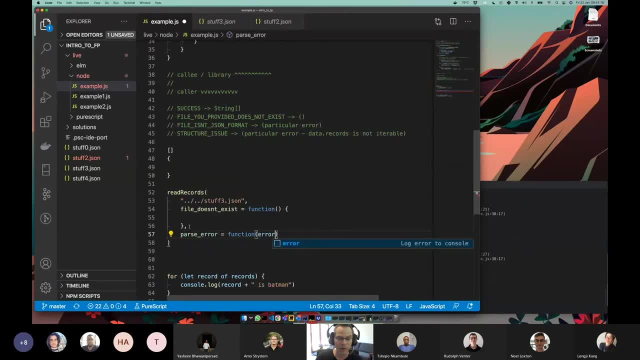 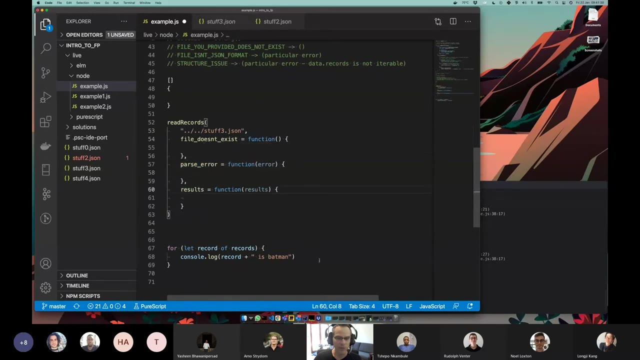 that didn't work. pause that didn't work, pause error equals a function with the or the results is a function with results, with the actual results. so here we can see already like, look, we're kind of forcing the caller to handle the three different situations that could. 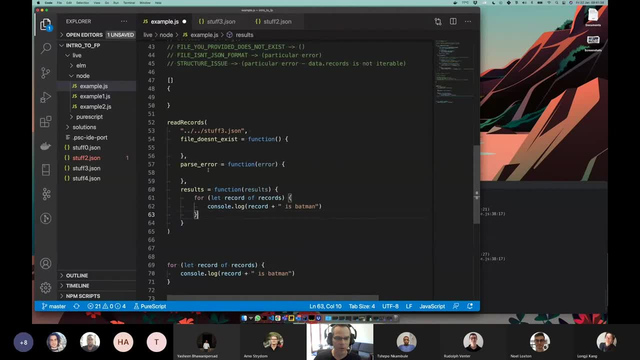 occur. so we know that. when it's results, we want to do that. when it's a pause error- pause error- we want to actually print the error, and when it's a file not found error- file not found- there's- there's nothing like. we have no information given to us other than file not found. 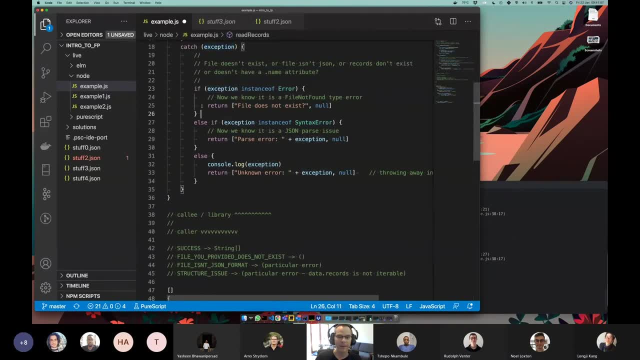 error, whereas up here, if you think about at this point, we actually did have that information, we had the exception, but we didn't plus it onto our string, if you look there, because we didn't really care, like if the file doesn't exist, there's no other information we want to tell the guy, just 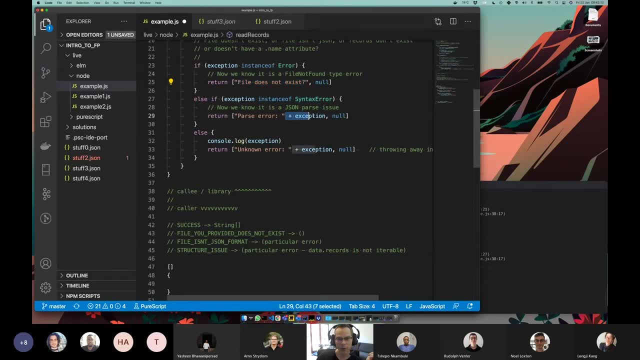 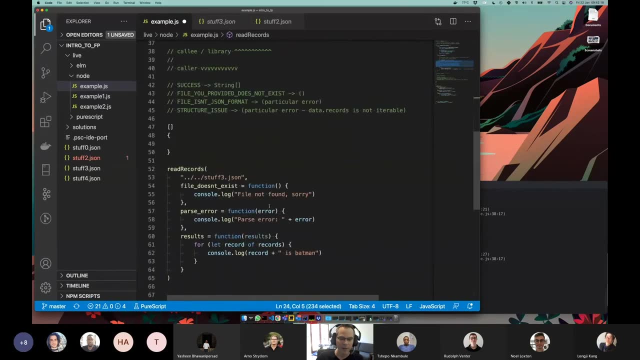 his file doesn't exist. that totally makes sense, whereas if it's a pause error, we want to pass him that particular error so that he can print it out. but but these are two different scenarios, right and? and here we've already encoded them. so we said: file doesn't exist. carries no information, pause error. carries the particular pause issue. 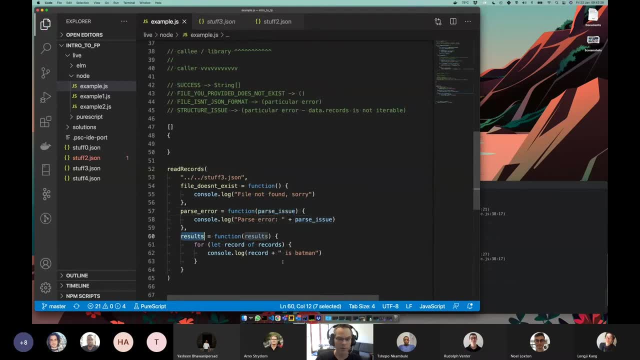 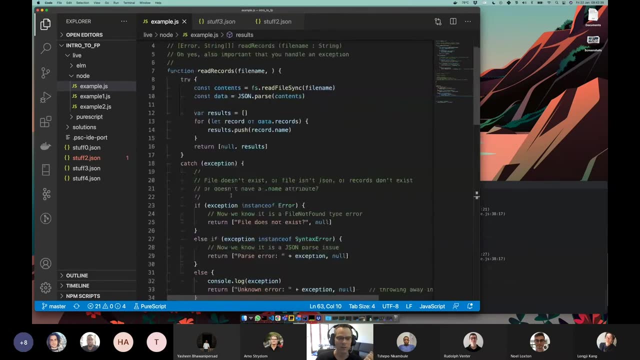 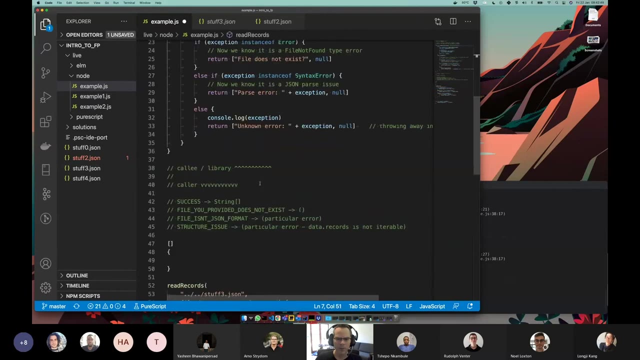 which he can then print, uh, whereas with results he gets a list of string which he can print over here. does that kind of make sense? so we can go ahead quickly and implement this and really what we're saying is we're going to take these extra thingies as parameters. 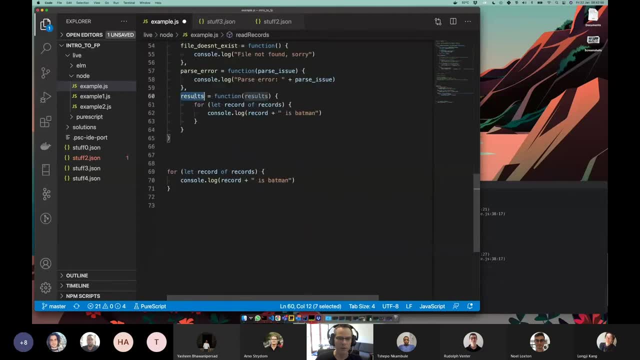 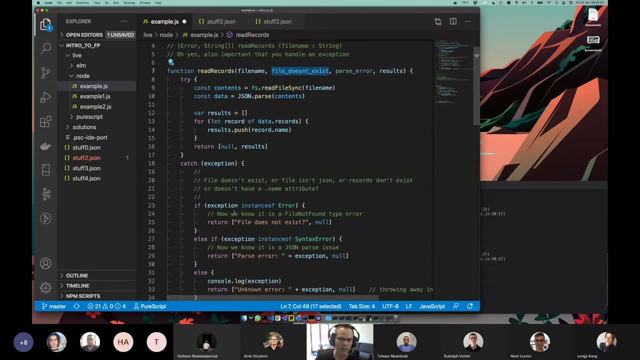 so these are now first class functions. um, if that makes sense and we can say: hey, when we down here in exception land and we know the file doesn't exist, we can just execute that function. file doesn't exist, when it's a pause error, we execute it with that particular message and when there are results, we we don't do this. 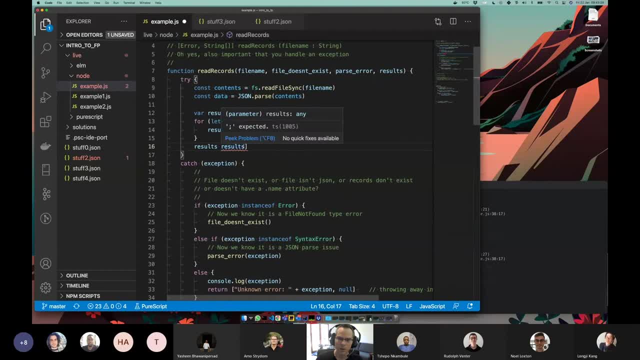 we don't return them, we just return: ah, this is called results, and so is that called results. so let's call this, i would call it prime, but uh, let's call it results. underscore: return those results as a function. that kind of makes sense. oh, and if there's like an unknown type error, that's. there's a third scenario. 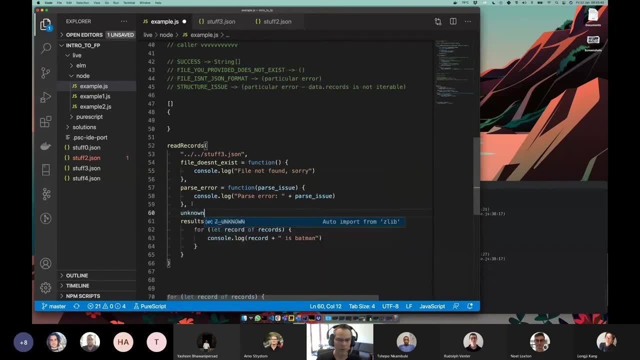 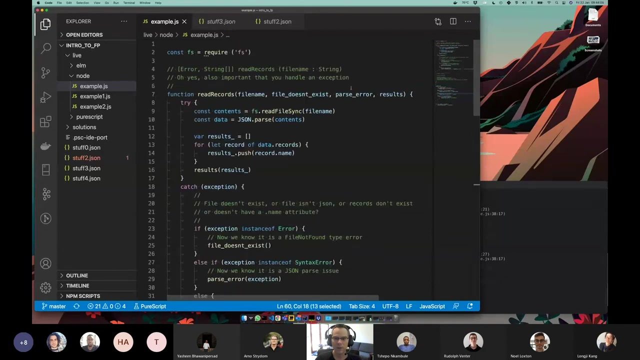 that we're not supporting um, which is an unknown error function and it's like i don't know the actual text of it. yeah, so why not? uh, yeah, the error description, that's fine and it's similar to that one. right, i'll just go unknown with that error. that means we need this guy up here. 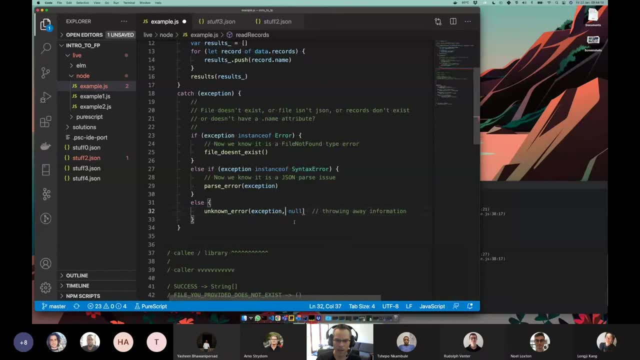 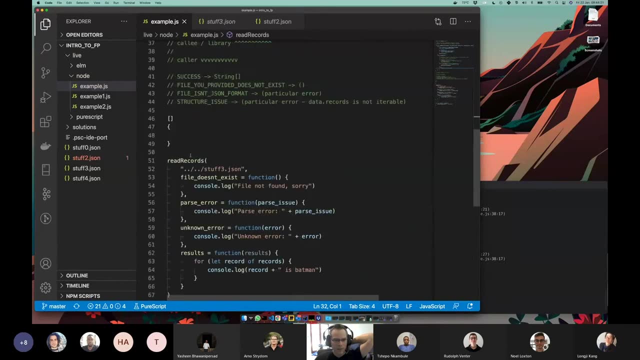 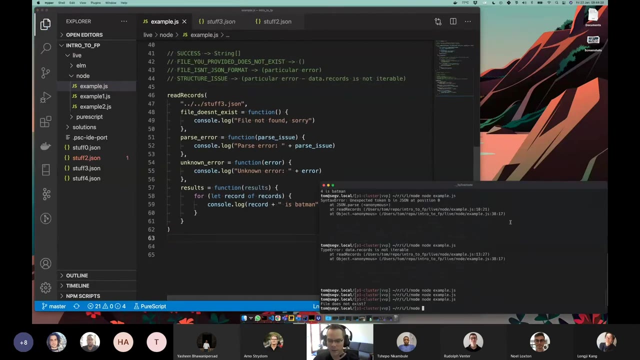 so what do you guys think? look, we've written a better function, haven't we? and i think we've, yeah, look, so we've done it, we've done it nicely. so if it's stuff zero file not found, did i save it. no, why is that stuff is. 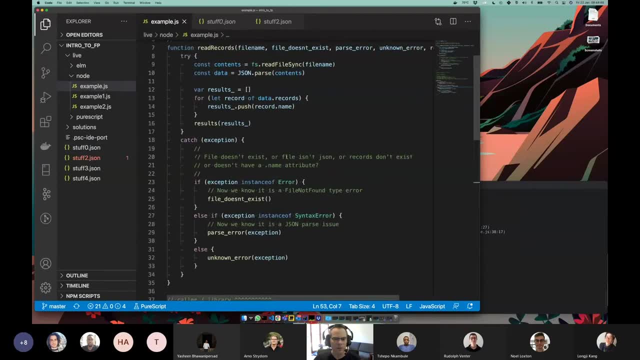 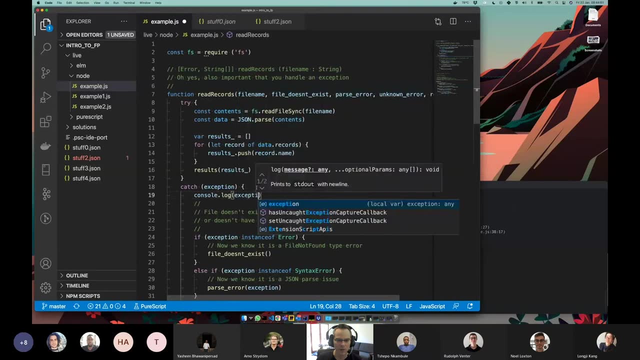 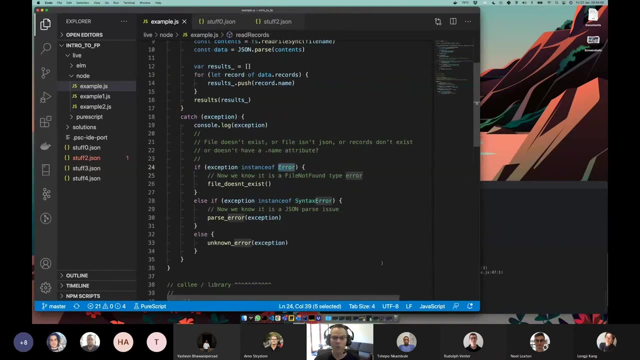 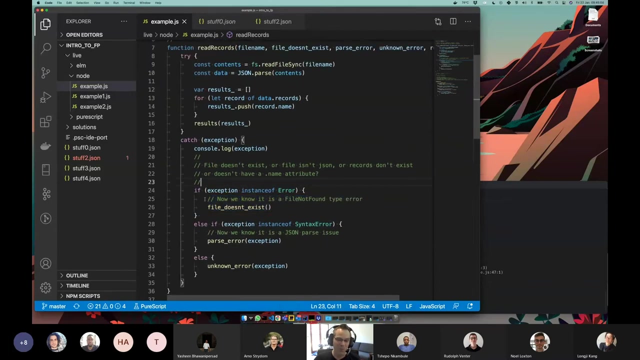 zero, it does work, so we should probably be printing just for debuggy reasons. records is not defined. ah yes, okay, oh so look, records not defined is also of type error, where it's being handled up here. so how irritating is that actually? so, in fact, maybe we. 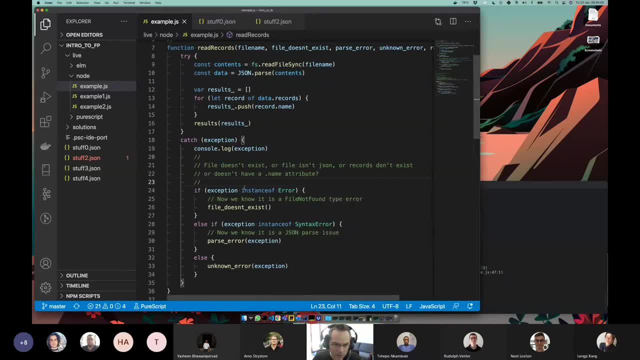 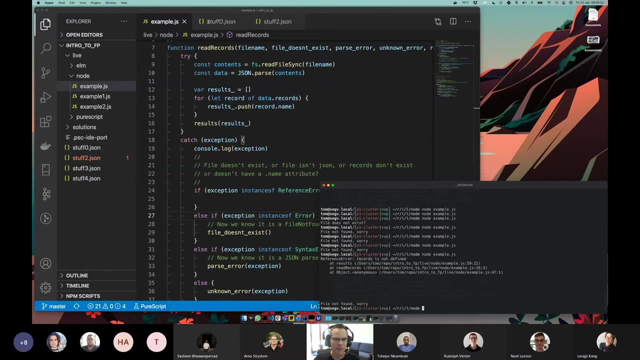 don't even have the. we like i don't even know how you do this, so like maybe we have to go if exception, instance of reference error. now we know, and this would be an else, so now we know records is not defined, which is that scenario? what scenario was that actually? 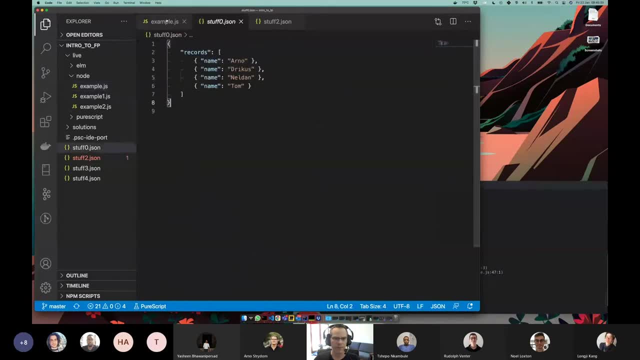 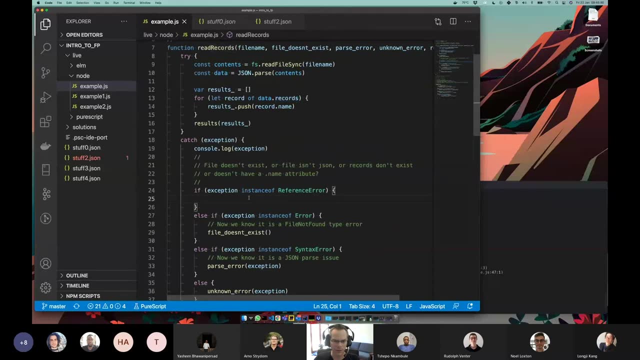 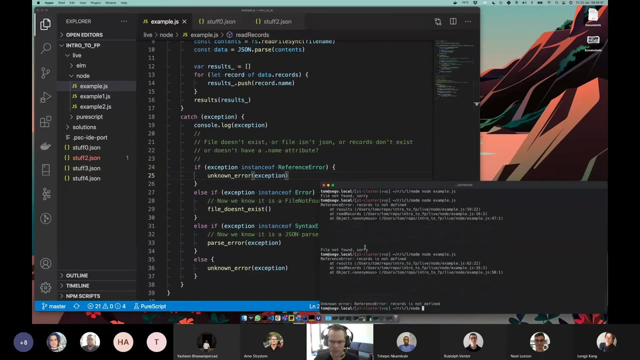 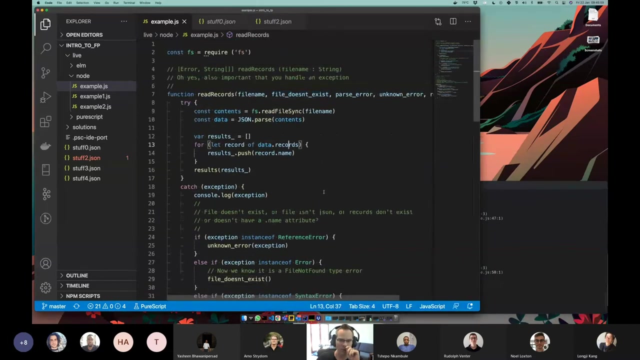 oh, in zero. what did we do with zero? records is not defined. oh, i don't know. let's make this an unknown error. yes, unknown error, fine, okay, well, i don't know. so there's some issue here, right? um, maybe you guys can can see it. uh, can you see it? do we care? records not not defined there. 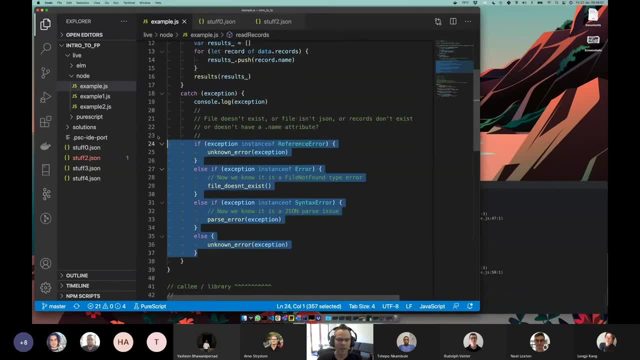 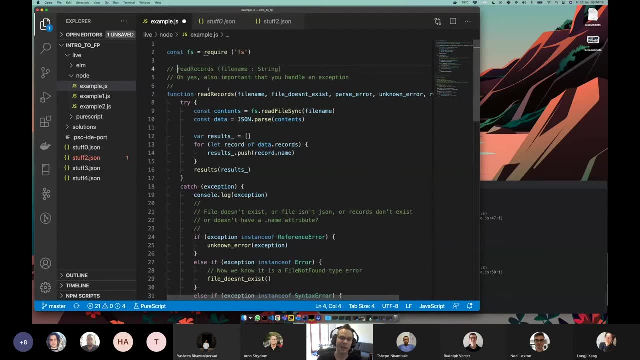 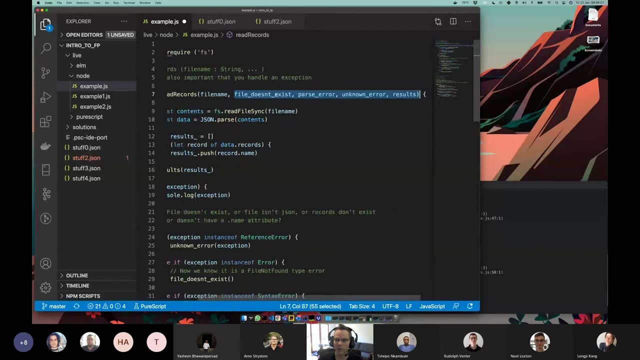 i don't know, i didn't even want to run it actually, but like i wanted to demonstrate the idea of of now. so in fact, now if we look at our signature, we no longer return actually anything, but we now return a whole lot more information up here about the three different scenarios, or the sorry, the. 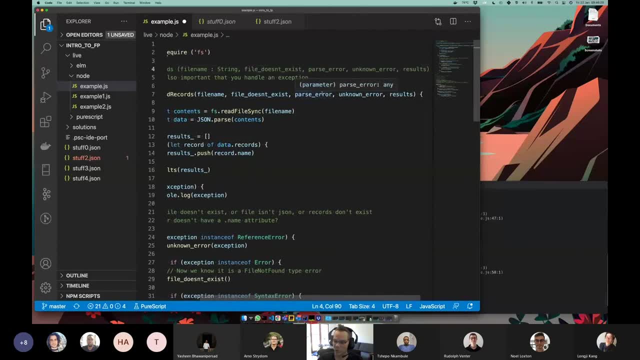 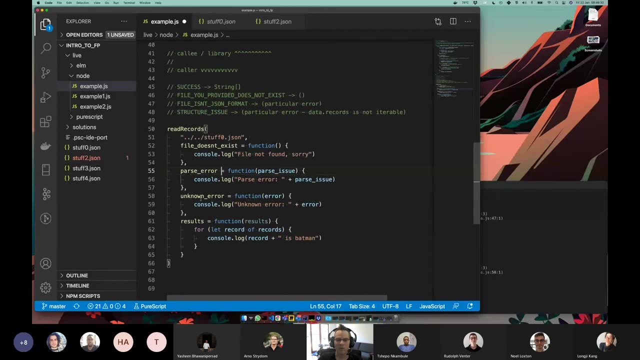 four different scenarios that could occur, which are now actually. if you think about read records, this is actually now become something which does support. it's more like a some type, um, or an or type of function. so So this function, either it executes this part or it does this part, or it does this part. 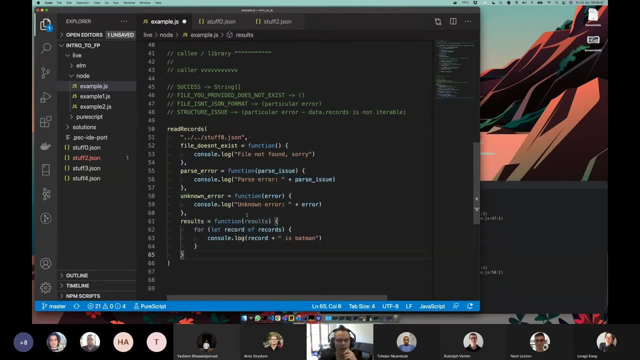 or it does that part right. It's no longer. there's no longer any doubt as to like: sometimes it's a this and sometimes it's a this. do you know what I mean? There's no decision that has to be made by the caller. 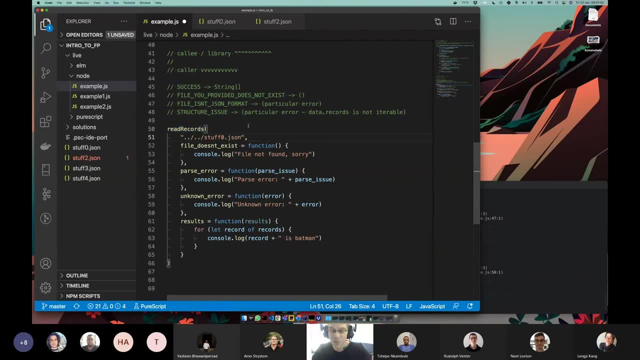 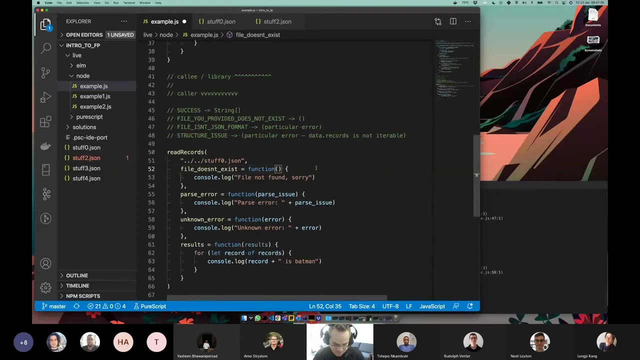 Does anyone have any questions about that? Does this look very foreign? Is this very weird, or does it seem okay? Somebody's unmuted so you can talk. It seems okay. yeah, Okay, yeah, And so you'll see this a lot in JavaScript. 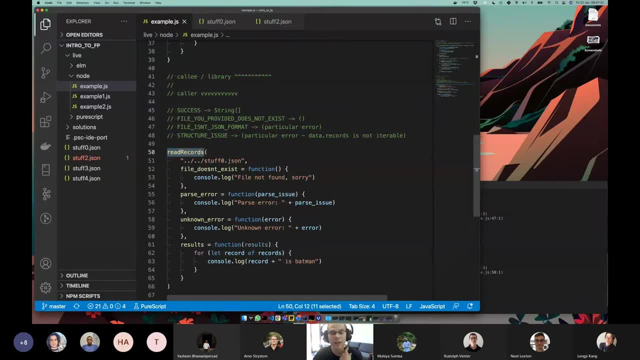 Definitely this kind of idea of passing callbacks into functions in JavaScript. Often it happens around like I want to. you know, like file reading, or I want to do this kind of thing. You know, like file reading, or I want to do this kind of thing. 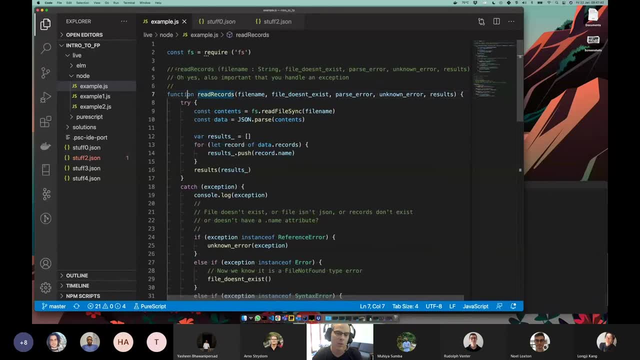 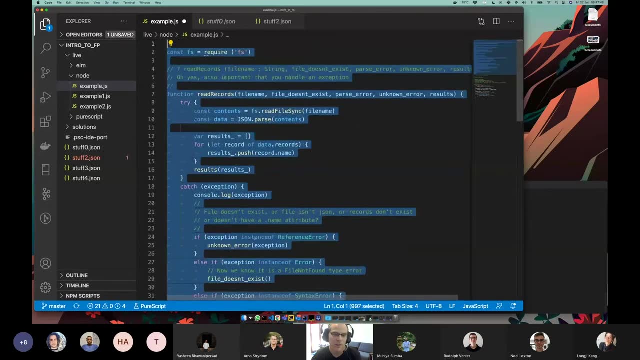 I want to make a request over the network, But often you will see like almost no use of the return value because in fact the return value here is nothing, right? In fact we have no return statement in this function whatsoever, right, There's no word return. 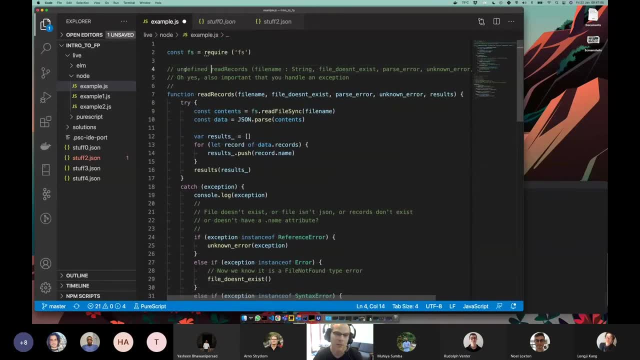 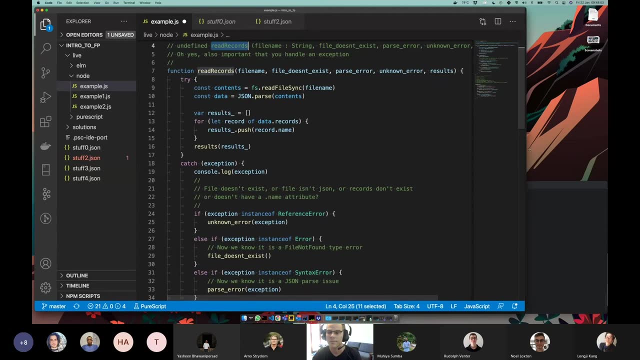 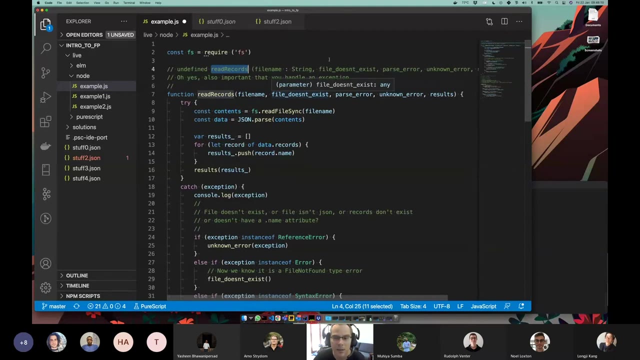 So in fact, we are always returning like undefined. It's like always undefined. So in fact, we've just thrown away the idea that this is a function which returns anything. It's like it's a sum type function, because it will just execute the right chain up here. 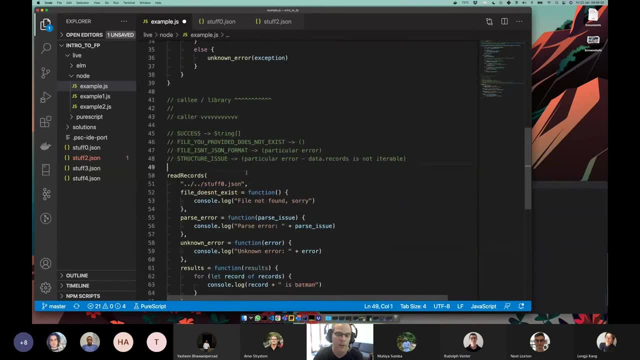 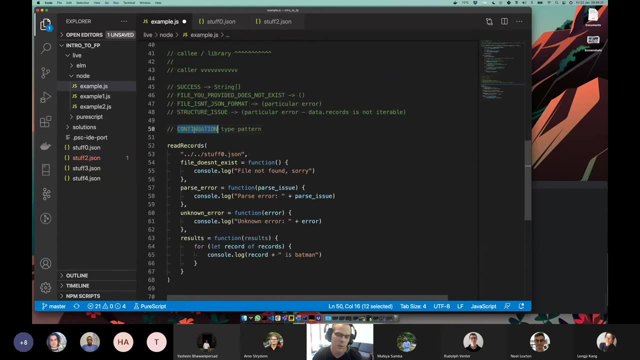 So quite often this kind of pattern, I would often call this like a continuation type pattern, And why it's called a continuation is because I execute a function which then is going to execute a function for me in order to continue the computation that goes. 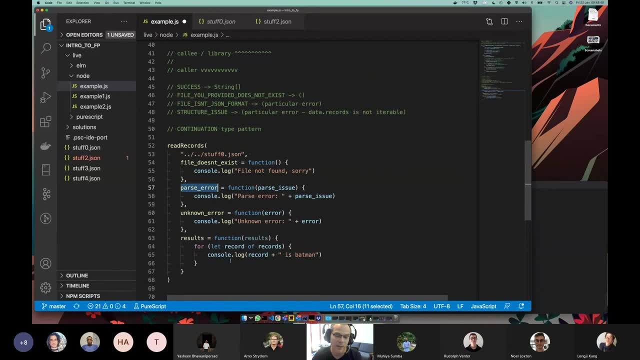 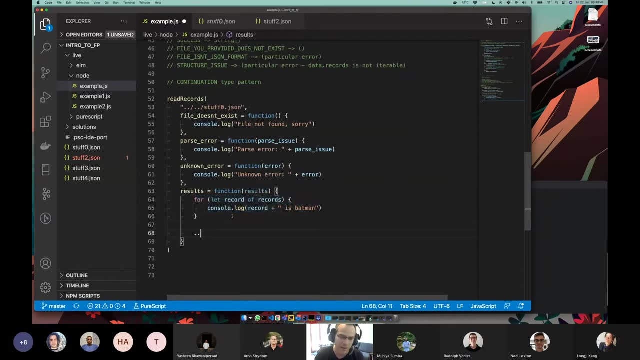 So I'm not. I'm not saying this is perfect, because if you think about it like now, if you're going to do a whole ton of stuff based on what results does, it means like all of your code you know from here on in is like squashed into this little thing. 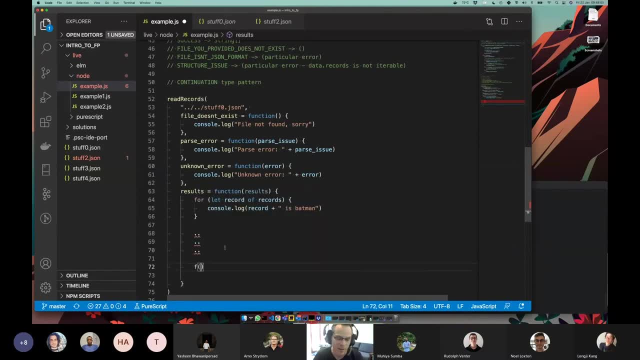 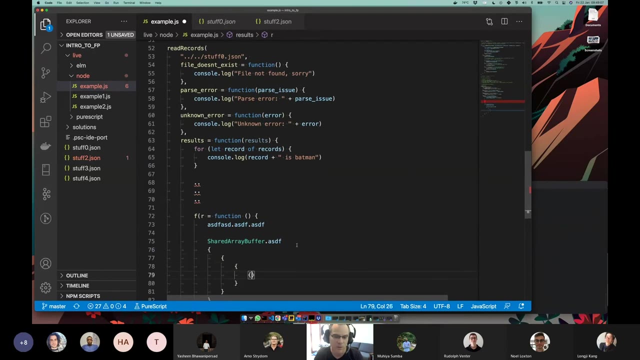 And if you call another function, you know that does something similar and it also takes results, which you know also does more stuff. It's like, oh look, we're starting to nest sort of left to right, Like our code opens and opens, and opens. 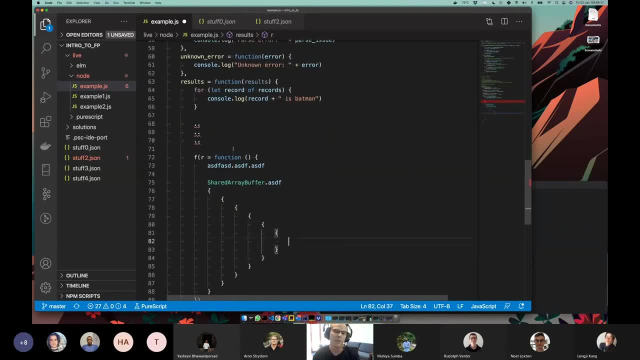 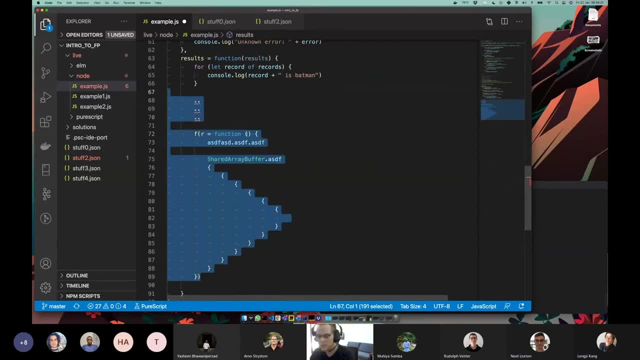 So I've done that very ugly but hopefully it passes it on, And that quite often is called. this kind of idea is called callback hell, which you might have heard about, And if you write enough JavaScript you'll certainly experience callback hell. 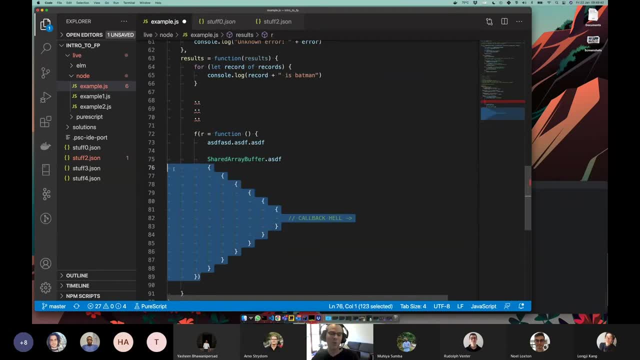 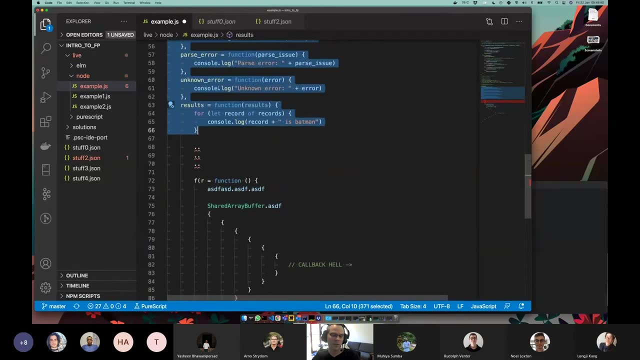 And so there are different techniques in order to manage callback- hell right. So it's a good idea overall, this kind of thing. it's a good idea, but it's not quite as just as simple as this, So to live with this is very hard. 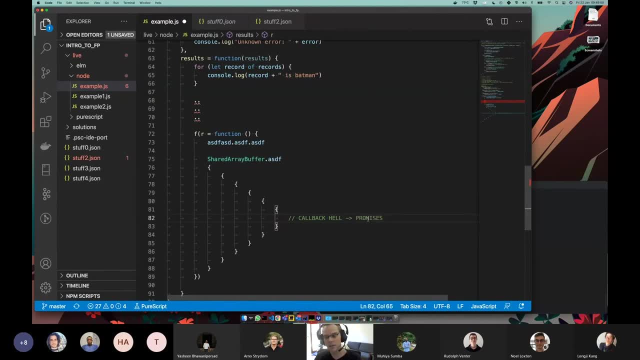 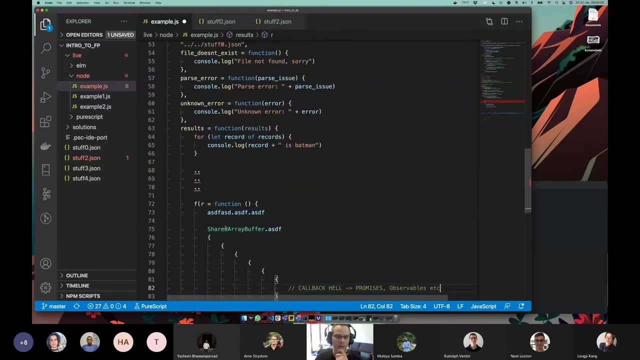 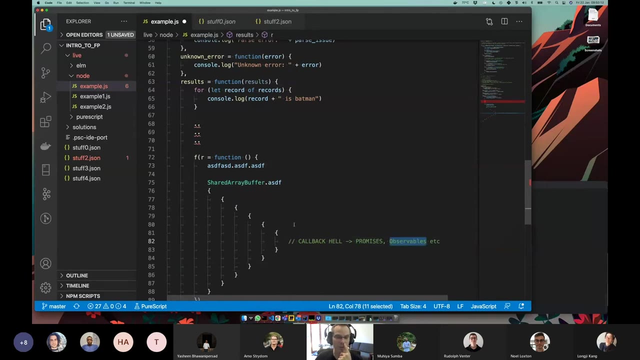 And so things like promises and observables et cetera exist in order to take this very left to right code and turn it back into top to bottom type code. So promises and observables will do that, but I'm not going to get into that kind of stuff. 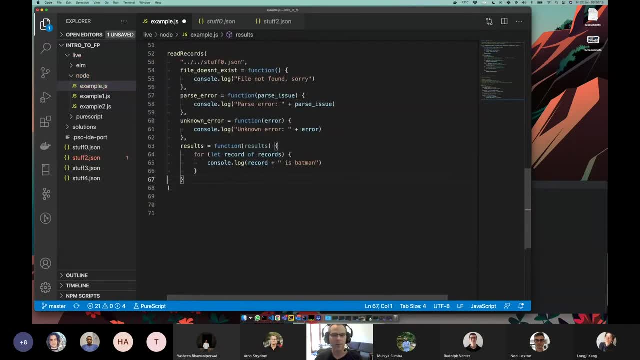 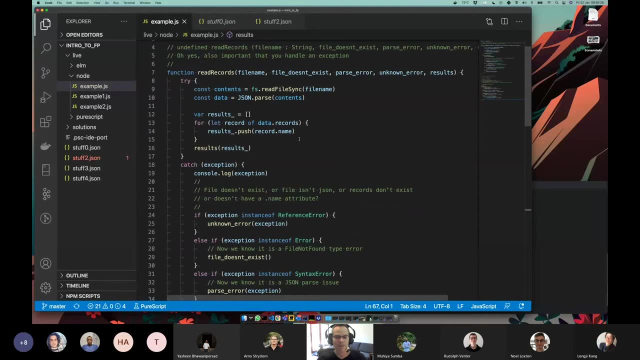 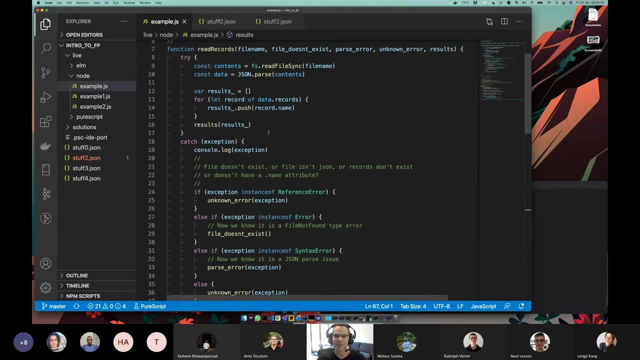 So it's definitely worth getting into that kind of thing. Anything else, Any other questions? Because I think we're done with this example. I think we've butchered it. It's a horrible looking function, though. hey, We happy now. 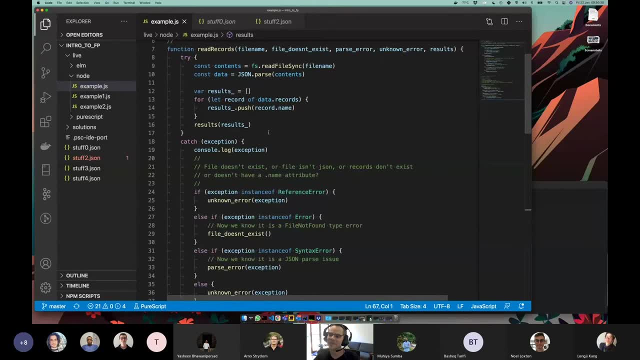 I have a question. Yeah, Is this sort of- I don't know if like, is this something specific to like functional programming or is this just like good practice generally? Yeah, that's a good question. Now, I would say this has got very little. 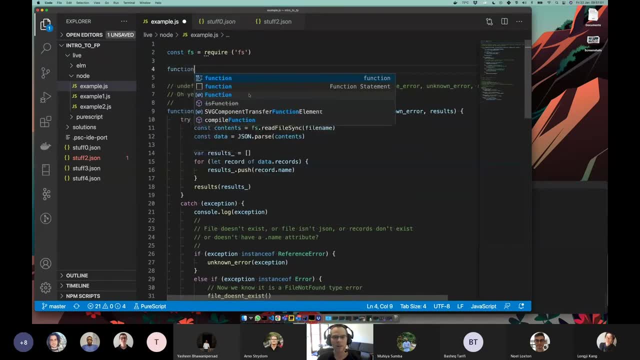 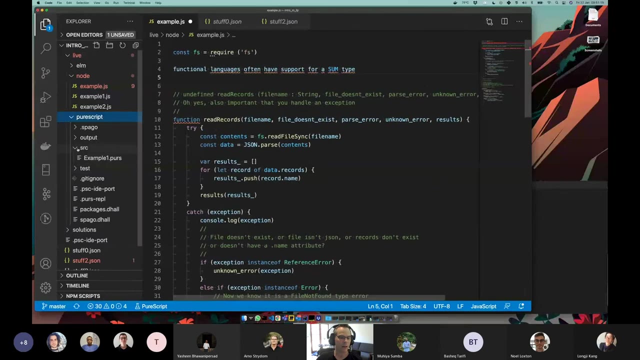 to do with functional programming other than functional programming, functional languages often have support for a summary. So some of the things that I think are the most popular and some of the things that I think are the least popular is the code type. So if you have a problem with a code type, 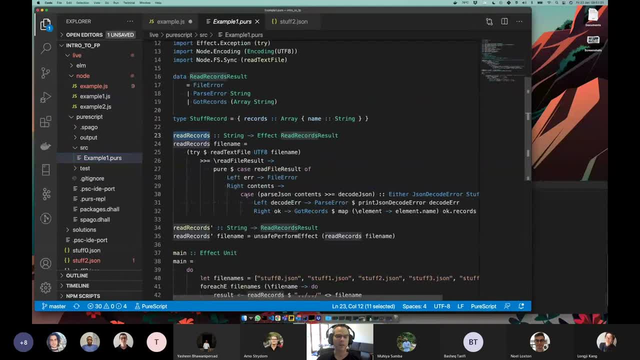 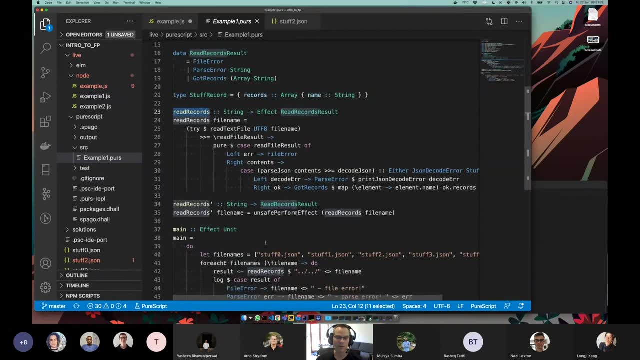 or if you have a problem with some type and okay, so I'll show you an example actually. So I've got this exact thing, I think, written in pure script. So pure script is a pure functional language, and I've written a function called read records. 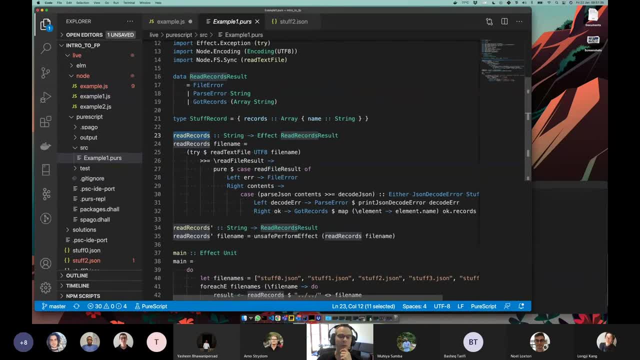 I'm not gonna take you through the syntax. It's very scary version is it does make use of the return type. So if we look at what read records does in pure script, it takes a string and this is what it returns. So you can ignore this thing called. 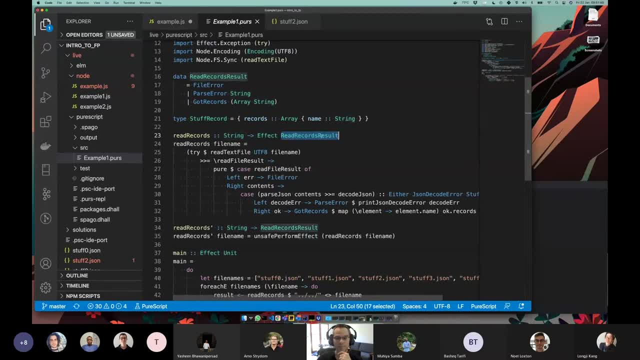 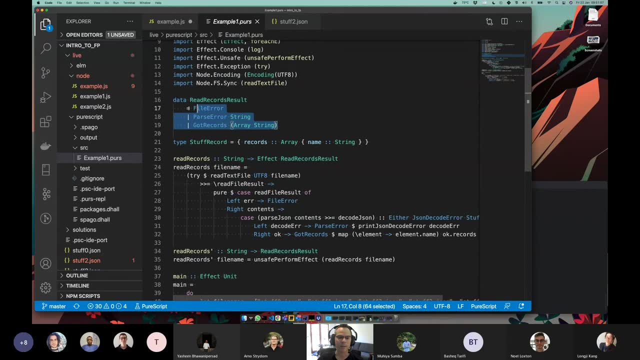 effect takes a string and it returns a read records result. That's its data type, So it's no longer an array of strings or whatever it is. If we look at what is a read records result, we can see it's this thing: It is either a file error or a pause error which carries a string. 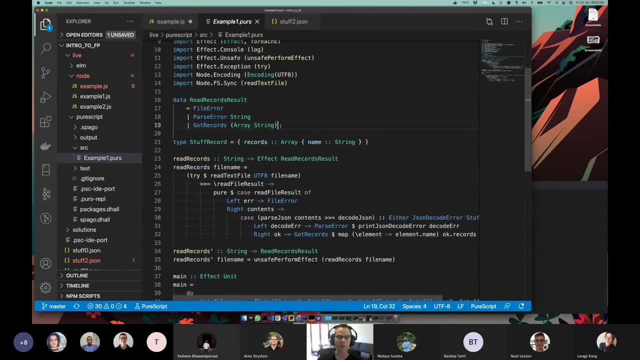 or a got records with an array of strings. So this could be like success, I suppose. In our example I think we called it success. So what pure script does, as a- and it is a particular dialect of a language very much inspired by Haskell- is it has first class support for that. 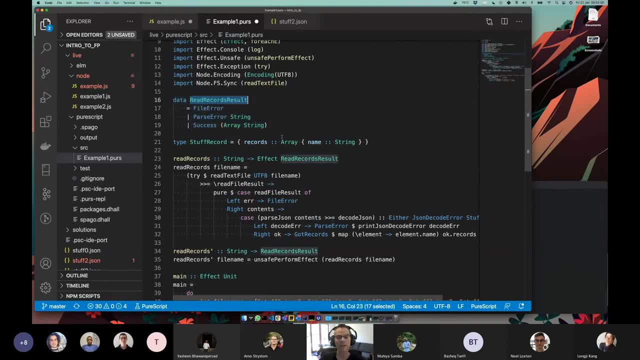 idea of some type. So it says: read records. results could be a file error or a pause error or a success. It can't be All three of them, It certainly cannot be more than one, It has to be exactly one, And in fact. 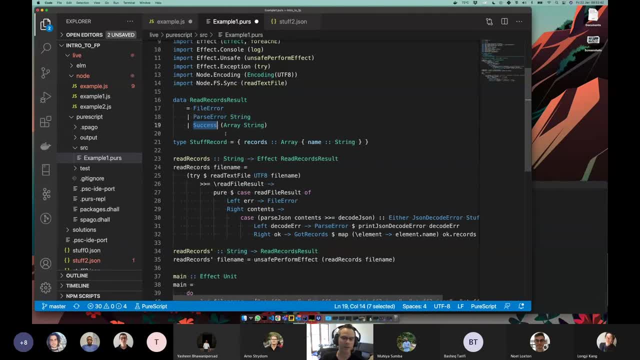 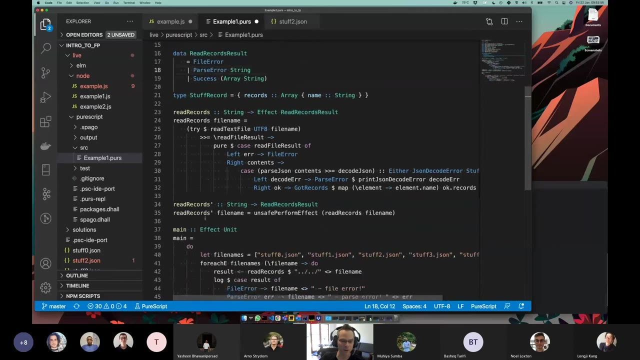 if it's a pause error, it also must carry around a string. If it's a success, it must carry around an array of string. Does that make sense? So these are called constructors of that type. So the cool thing about this is it's very explicit, right, It's very explicit. And so when I call 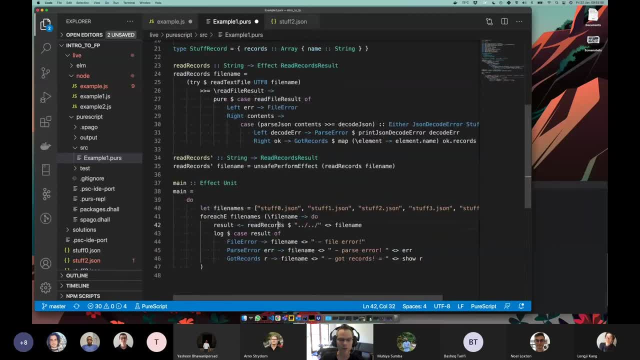 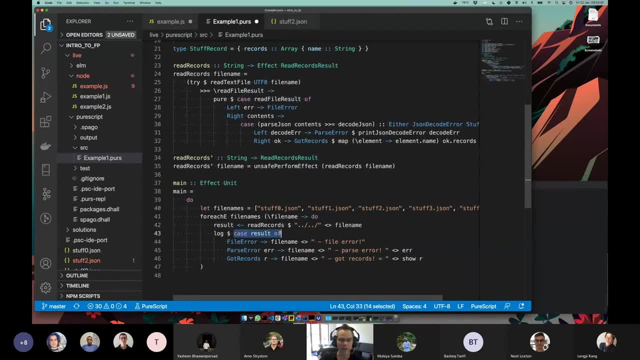 I can't use it because I don't know what type it is. yet I have to do a case match on it and say, oh, it's a file error. Then do this: Oh, it's a pause error. Please set the string that it was. 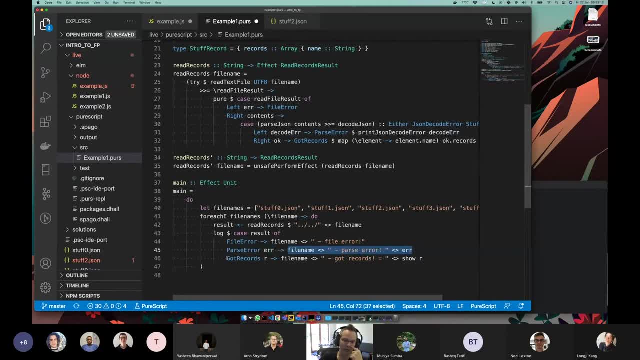 attached to this variable called error and I can do something with it. If it was a got records, I got an R and maybe I want to show those records or whatever it is. So a pure functional language is very often well, certainly like PureScript, and Haskell have very strong support for this. 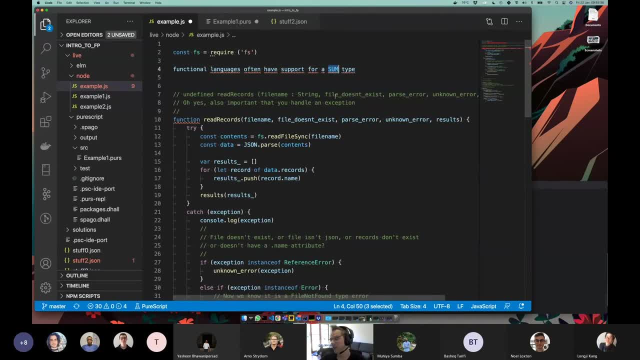 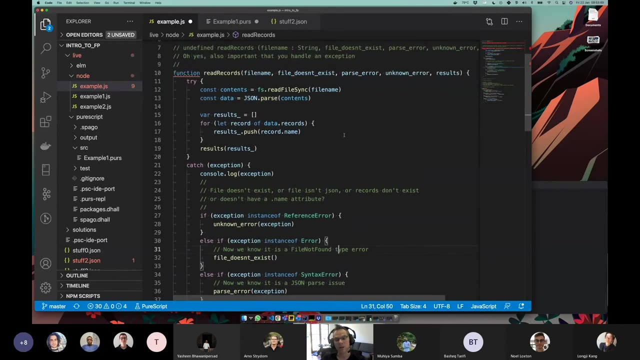 notion of a sum type. I find in a lot of not explicitly functional languages are glaringly missing this kind of idea, this sum type. You can, of course, do it through things like this, but it becomes quite wordy and quite annoying And it's not also a guarantee. So for example here where I catch 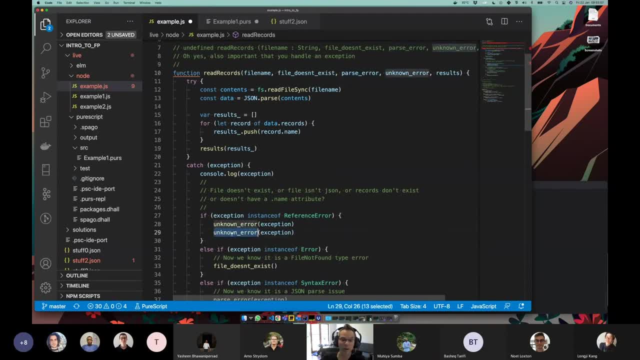 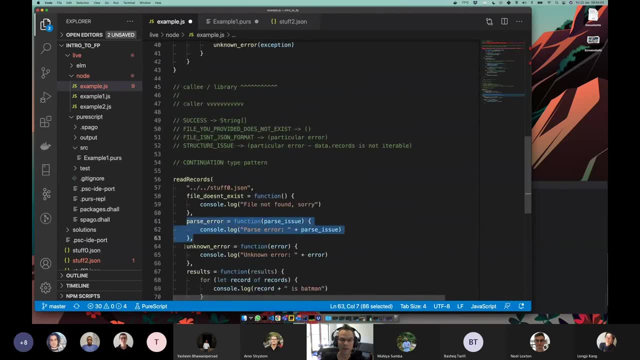 an unknown exception, an unknown error. I could also call pause, error at the same time. right, I could call that, then call that, And what I've done is I've ended up calling this OK's function there And then his error there And it's like: oh, he probably very, you know, he very much didn't. 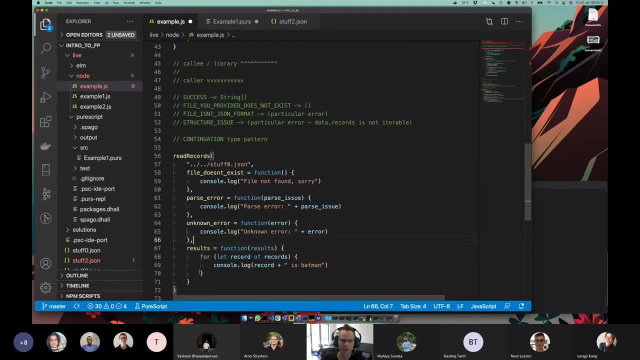 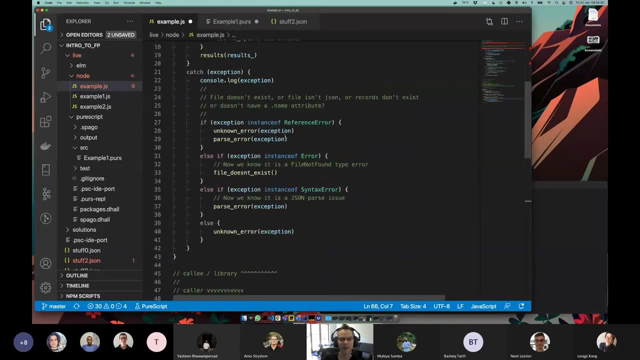 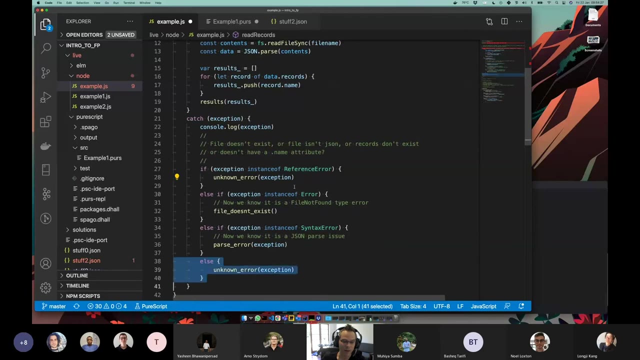 expect me to do that. right, He expects me to call at least one of these things. Not at least one, exactly one. So not zero and not more than, and not two. right, But I'm not prevented from breaking that error up here. In fact, I don't have to call anything. So, in fact, if I had a bug in my code, 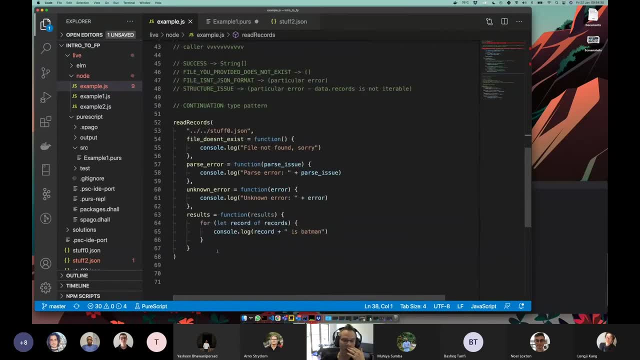 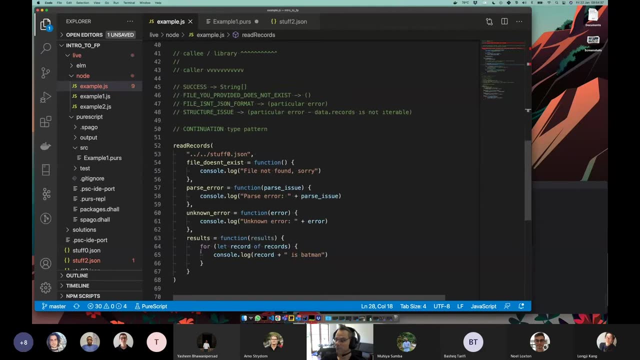 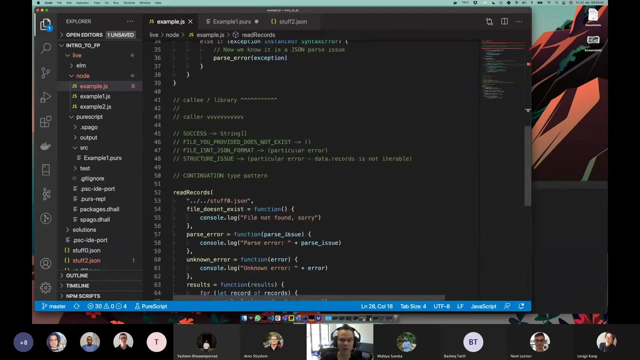 and I left off this else over here. I would end up calling absolutely nothing down here in that scenario And I would leave his program just sitting there, right, It would just be doing nothing, right, And that's a very unexpected state for him to be in, right, That he calls my function. 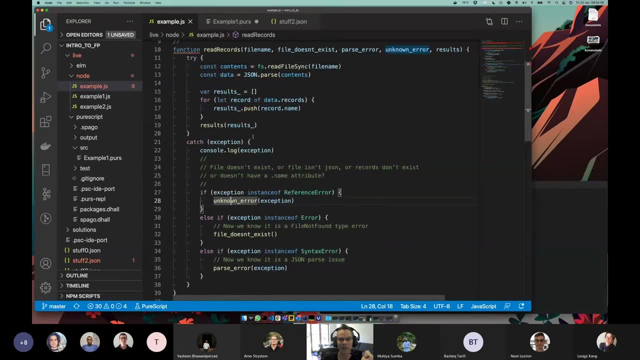 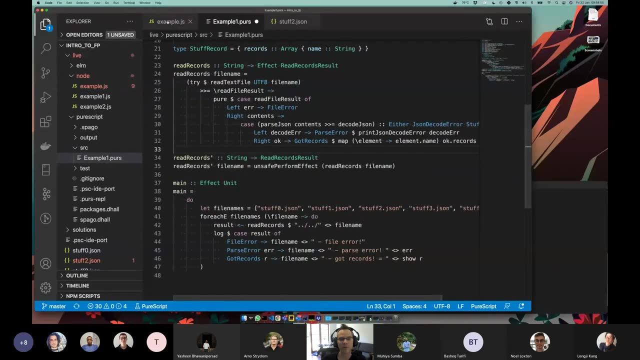 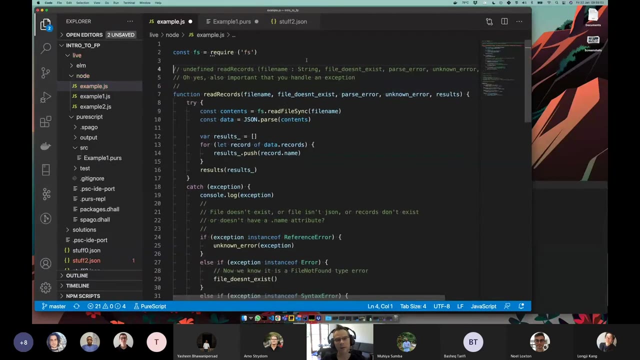 and then suddenly nothing occurs ever again. right, It gets kind of just lost in this, or the program exits or whatever, if that makes sense. So when you ask: is it a pure, is it a functional thing, I would say, the idea of a sum type is certainly something that's popular in functional. 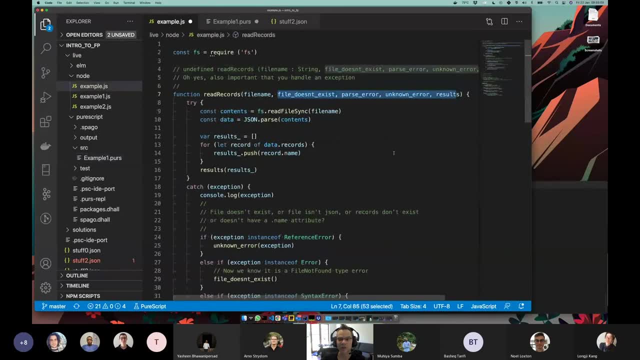 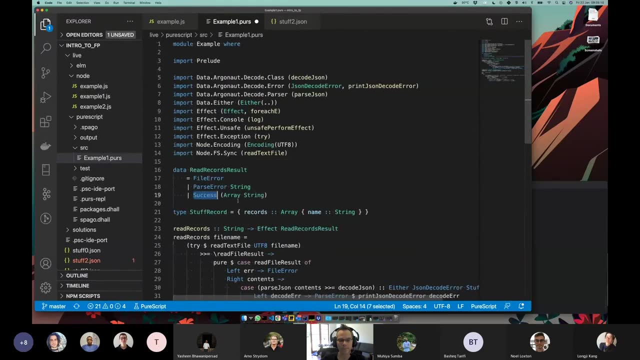 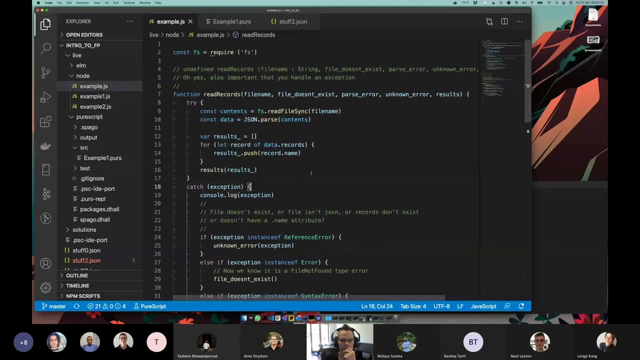 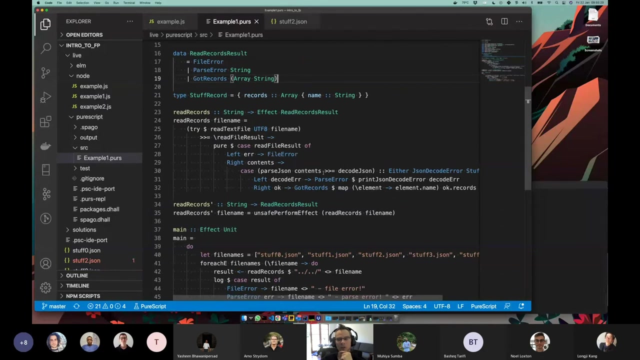 languages, But it doesn't mean that you can't use them in non-functional languages, Like here. I've just demonstrated that we could have a sum type idea, if that makes sense. Yeah, So here it's pretty explicit. Okay, All good, Okay, So what I'm going to do is: yeah, yeah, yeah, shoot. 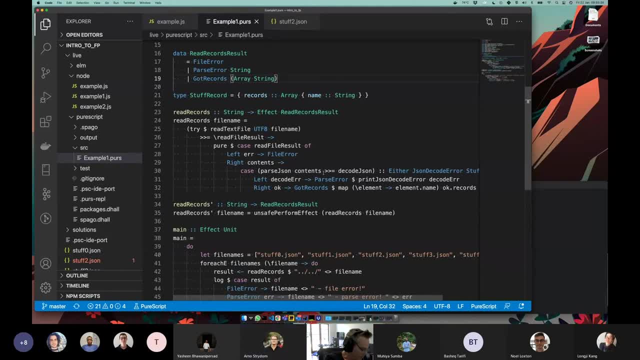 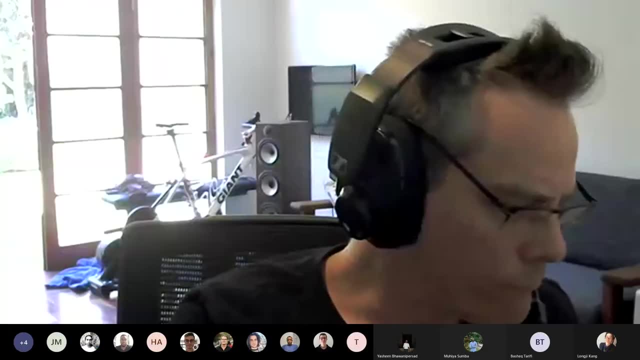 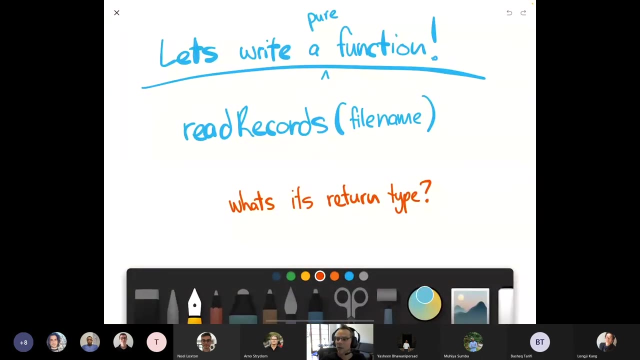 No, no, no, it's all good. Okay, cool. I'm just going to go back to my iPad here. I think we've got 30 minutes and I think, yeah, cool. Hopefully I'm going to stop sharing there. Okay, there we go, Cool. 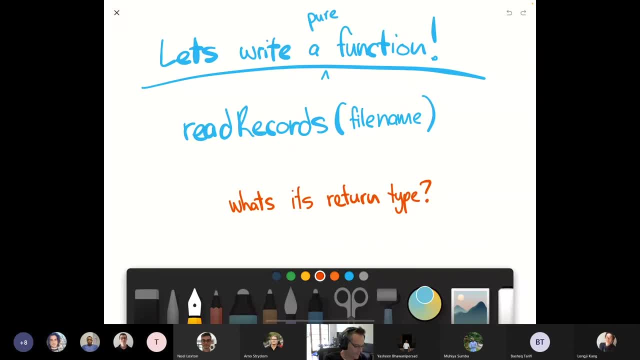 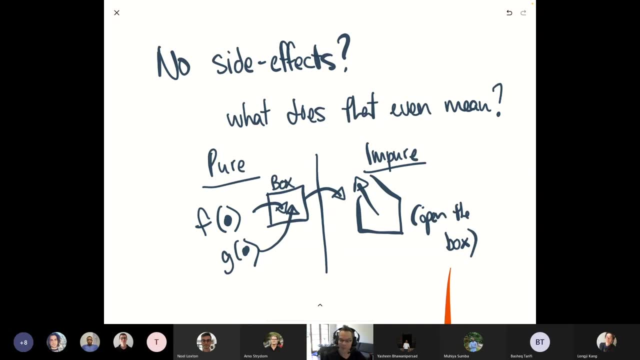 All right, You guys can see that right. Yeah, Yeah, Yeah, Okay. So I know we. so one of the things about functional programming, and maybe I'll talk about this very briefly. I won't give any code examples, but 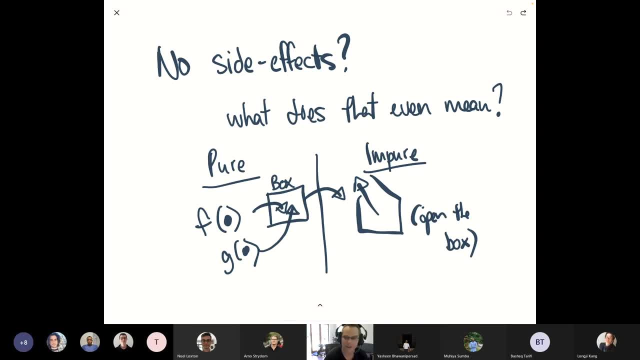 we talked earlier about side effects. Did we talk about side effects? I think so. So I said, I think we talked about this idea of purity in our program right? So in a pure, functional language, we have no ability to create side effects, which means we can't read a file. 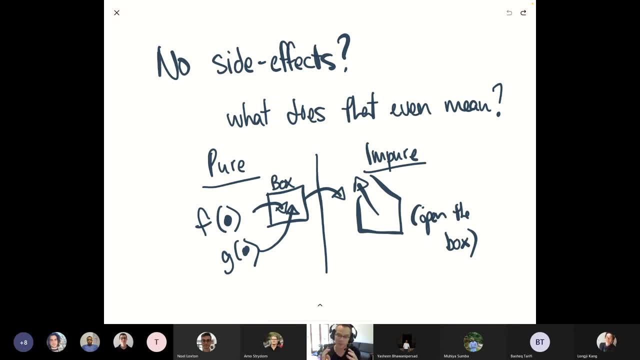 and we can't write to a file, We can't talk to the network, because these are things that are outside of the outside of the purity of our program. right, If we assume that our program is kind of like a mathematical sort of set of, you know, set of expressions or whatever an expression can't 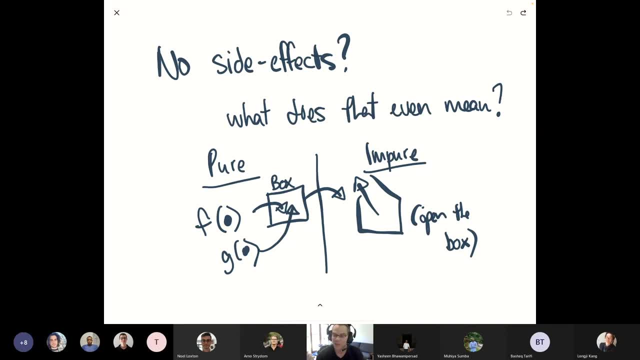 like read a file, because that file might change tomorrow, or it could change the next second or whatever, And we know that when we execute a function with a particular input, it must always give us back that same, the same output for the same input, right? 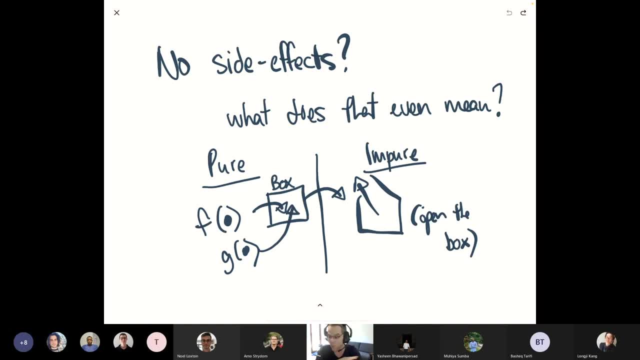 So if I give plus one a one, I expect you to give me a two in all situations, right? It doesn't matter what time of day, what, what like planet I'm on. Plus one plus one equals two, always, right. 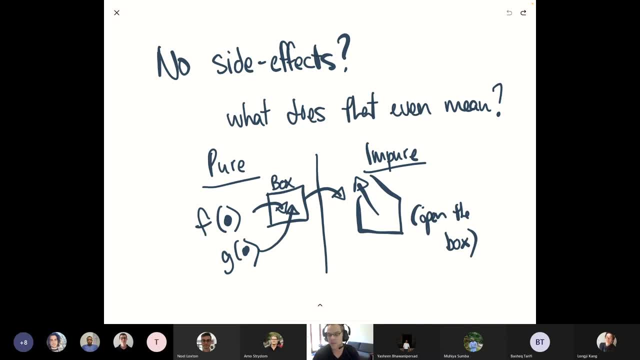 And that's one of the cool properties of pure, Pure means, and so, and when something is pure, you can- you can have some interesting effects, Like, for example, if someone says what is one plus one and I give them the answer two, someone else asks: what is one plus one? 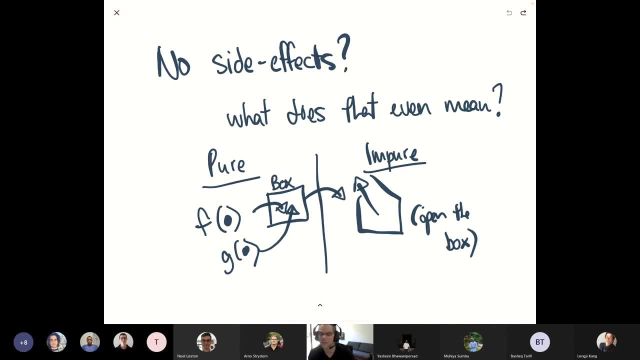 I don't need to recalculate it. I already know it's two because I gave it to someone else earlier. Right, I don't need to recalculate it. So, for example, like calculating pi two, a thousand decimal points, If someone executes that twice, I can just remember, like four, pi 1000,. 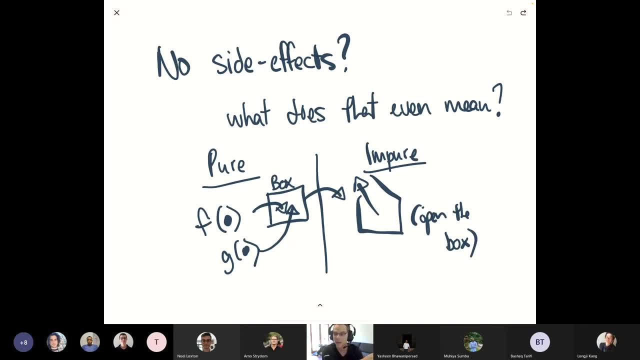 it was this answer. I don't need to go and recalculate pi to get to it again, Right, Um, and because it's a pure function, I know that it's not possible, that it could be different, whereas if I was reading pi like the starting point of pi off of disc. 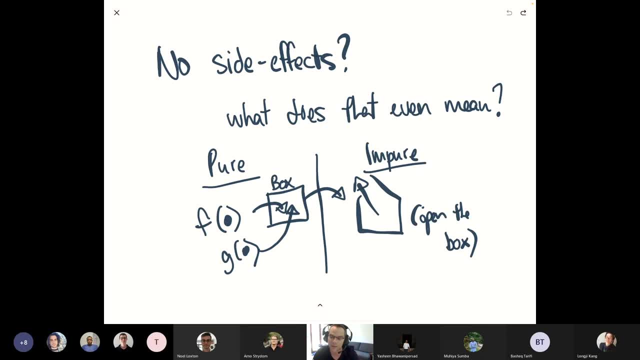 okay, I have no such guarantee that it's still the same in that file right. Some external factor is an input to that function, And so it's not entirely true that something like PureScript or Haskell has no side effects, because it would be pretty useless right to write a program that has no effect on the world. 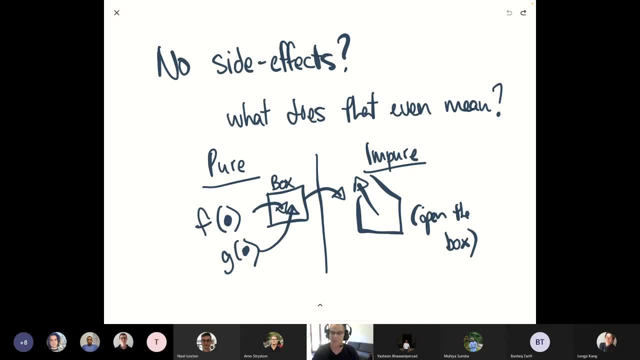 I can't think of one situation where that would be useful, other than maybe I was a mathematician right and I wanted to solve pi right. But even at the end, if I know what the thousandth decimal of pi is, I probably want to print it. 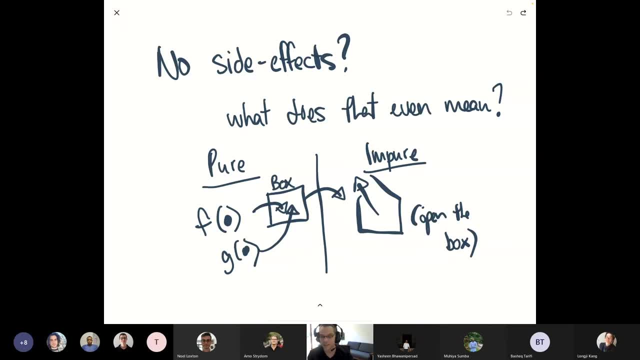 or I want to like show it to the user. And if you're saying showing that to the user is a side effect, like sure that makes it a pretty useless function. that only the program can have the answer and no one else, right? 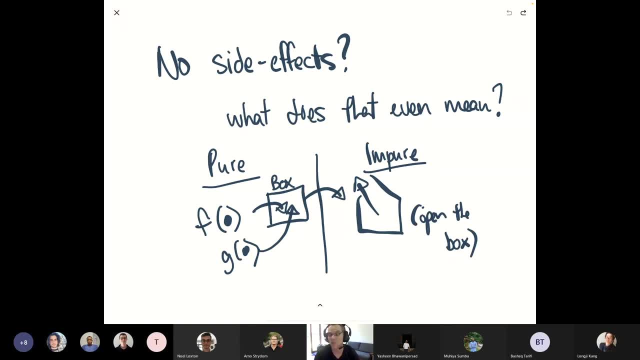 And so, of course, no side effects is not really a thing. What happens in functional languages? they're often just put inside a box, And so you have this pure side of your program and you have this impure side of your program. 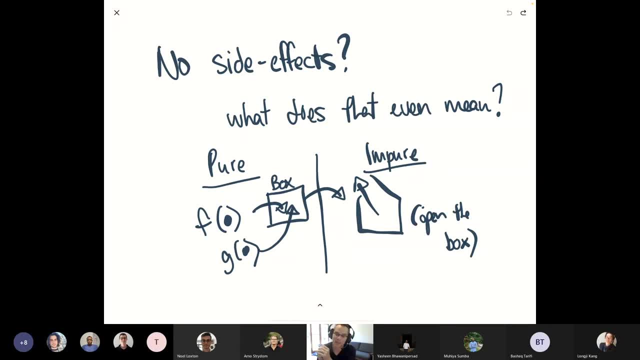 And that impure side is very much. what it does is it's just open the box and it's for like one small situation where effects are going to occur inside this box. And the idea is kind of that what you do on the pure side is you do a whole lot of preparing yourself. 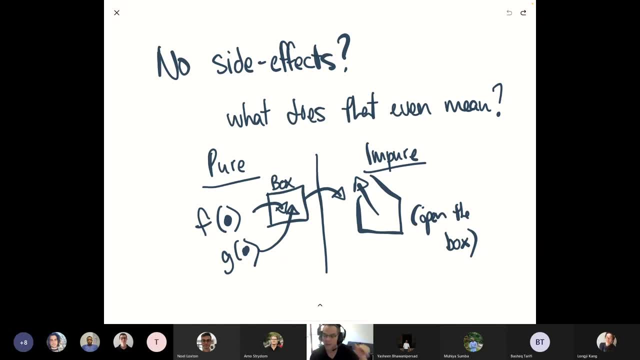 and putting stuff into that box while your program executes. So if you were calculating pi, for example, and you were reading the starting value out of a file- I don't even know how to calculate pi, actually, So maybe a bad example, but like. but say, for example, you needed a starting value that you were then going to like. 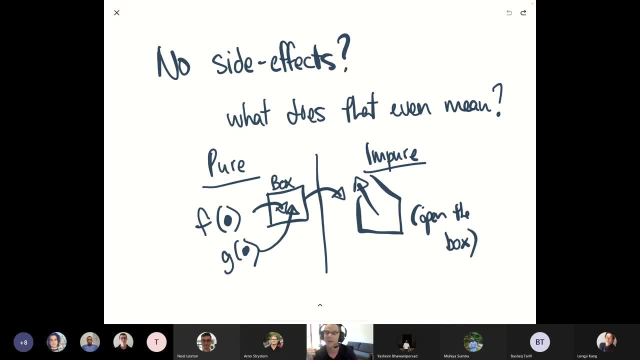 iteratively calculate pi on or something, and you needed that out of a file. What you would do, instead of reading it out of the file in your program, is you would say, hey, my program needs to read this out of the program and it will give me a result. 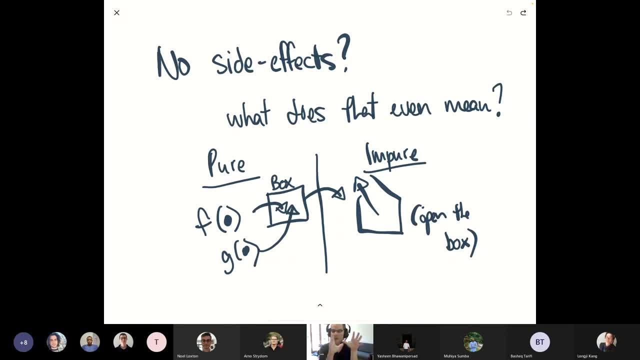 With that result, I intend to do the following. So it's almost like I'm going to wrap it up, almost as like a Is a declaration. So the reading of that value is not something your program can have directly in your code, but it's like you can think about it notionally. 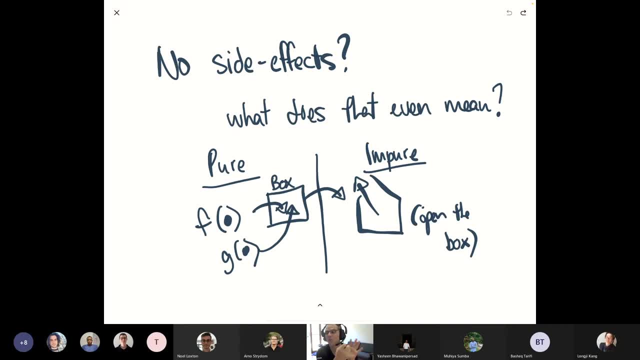 Like if I know that the value is of this type int or this type flow, to whatever it is, or potentially the file doesn't exist. Here's what I should do. Here's the continuation down the different paths, And my program is more about describing what are those paths that it should take. 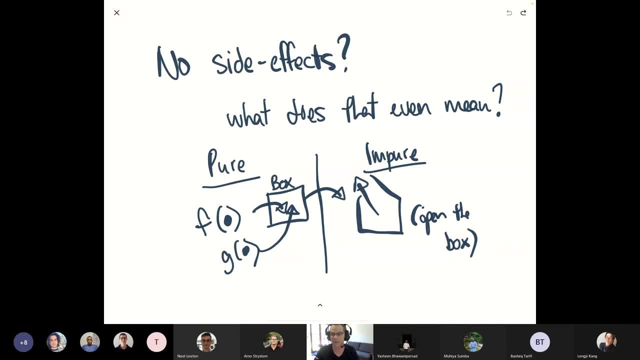 And then when I execute my program, what happens is the kind of like: the runtime sets up that whole set of Expressions all in your pure code, and then it it unlock it, it opens the box and it says: cool, let's go wild, right. 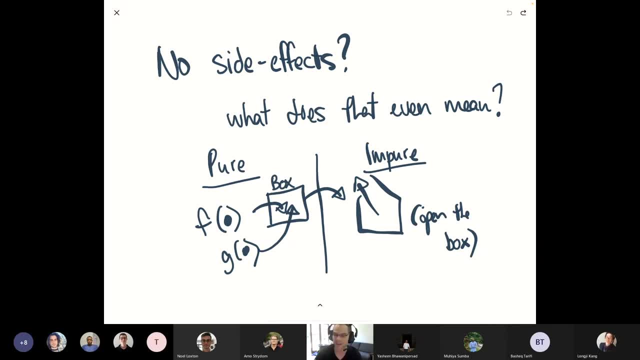 Let's execute it, But it's kind of no longer your code that's running explicitly. It's kind of like if that sort of makes it. I mean, it's like a weird example and we'd have to go into it like into a ton of detail, but it's this idea of putting your, your effects or your impure code inside this box. 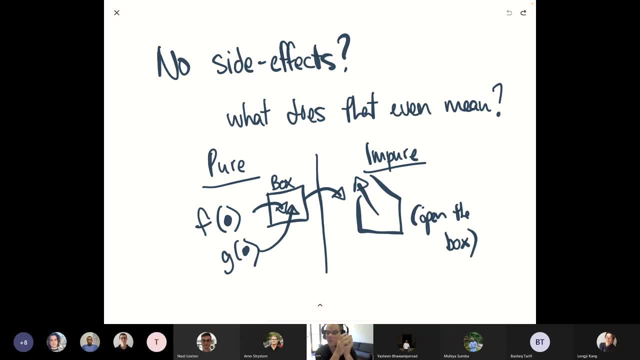 And then you can still reason about the what's in that box. So so you may know that this box, when it's Opened, It may have an integer for me, or it may have an error, And if it does, um, you know, I can add more stuff into that box and say, oh, if it's an error, then I want you to do this. 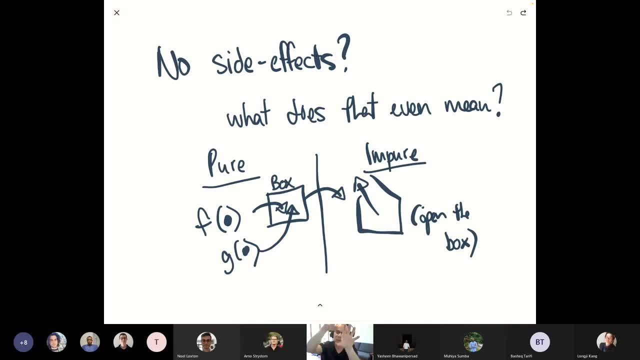 And I put that into the box. And if I get an integer, then do this, And I put that into the box. And if you think about it, that's my code. right, My code is just putting stuff into this box. 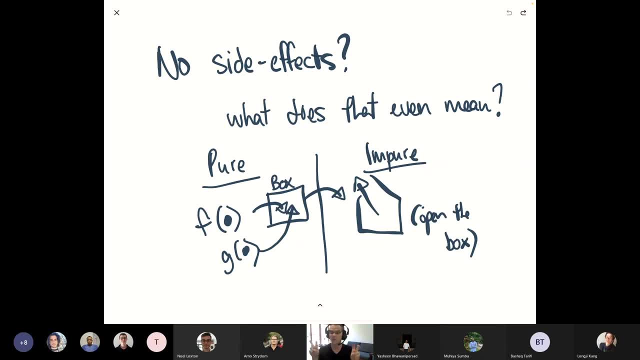 And then at the end I just say, Hey, here's a box. I just returned that back to the the impure side of the program and the impure side goes. cool, I'm going to open the box. Let's hope that it works. 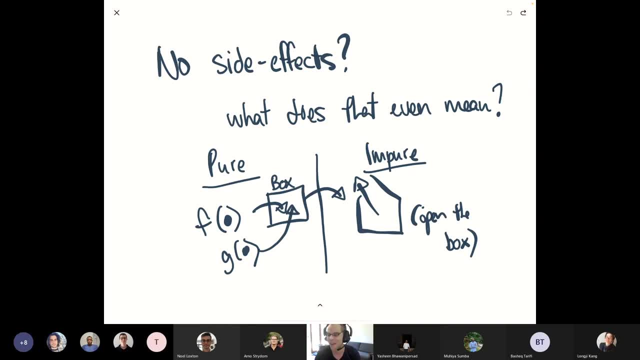 Um, And that's kind of the idea of the way I certainly think about how side effects work. um, in a pure language, is this kind of box concept. And then there's a whole bunch of like really cool ways of describing different kinds of boxes, different ways I can like combine boxes together, uh, et cetera, et cetera, et cetera. 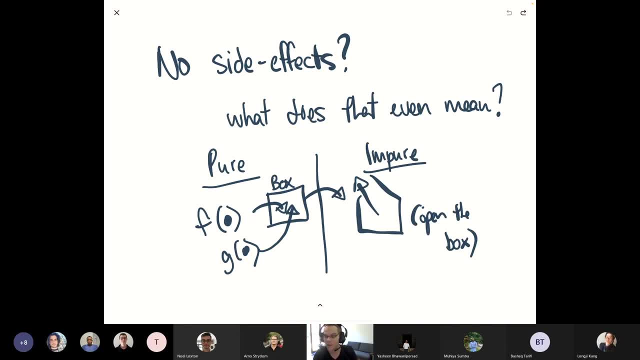 And this takes you into this very exciting world of things like mo uh uh, monads, monoids, functors, applicators, um, et cetera, et cetera. It's like a whole world of things. about what can I say? 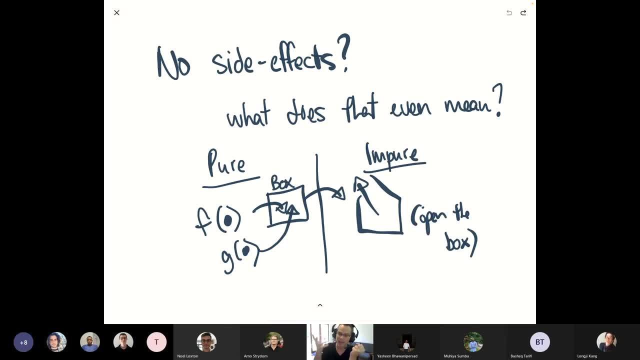 I've got a box and a box. right, I've got a box that opens a file and then a box that displays this thing to the console, displays an integer to a console. These are two boxes. I can't give my program back both boxes. 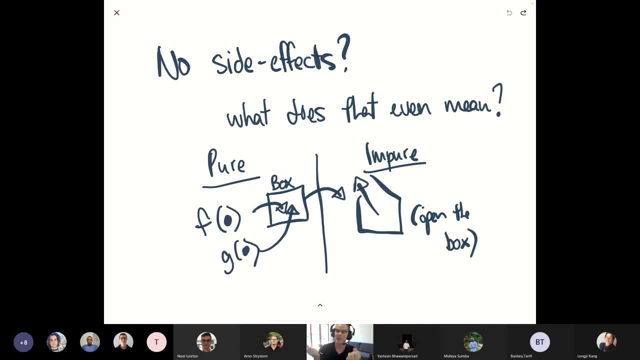 I can only give him one box to open, right, My program can only open one box. I've got a function that can say do this, And when I get the entire of this file I want you to run the, the print, the int function that's inside this box. 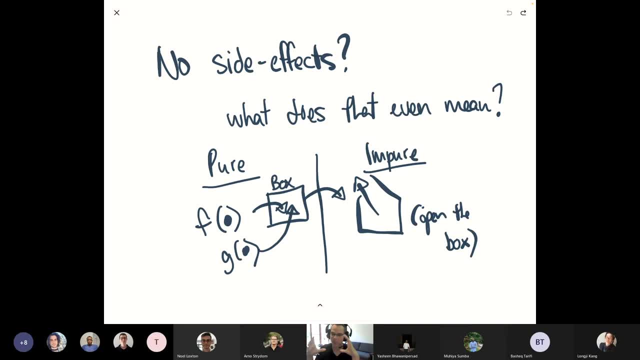 And I can Compose these boxes together to create a new box which is a composition of these two boxes. Do you know what I mean? And I pass that box back to my program. So, like a way of composing boxes together, Does that kind of make sense? 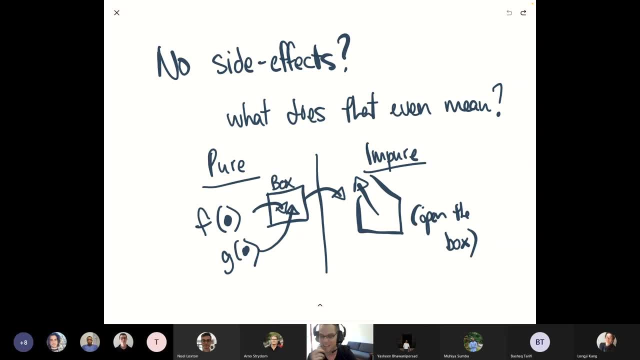 It sounds pretty wacky, but it really is like that, Actually, Any idea. Has anyone ever written any pure functional code? No, you should. Someone has Rudo? Tell us Rudo. Well, no, I mean we've. I think a couple of us have. 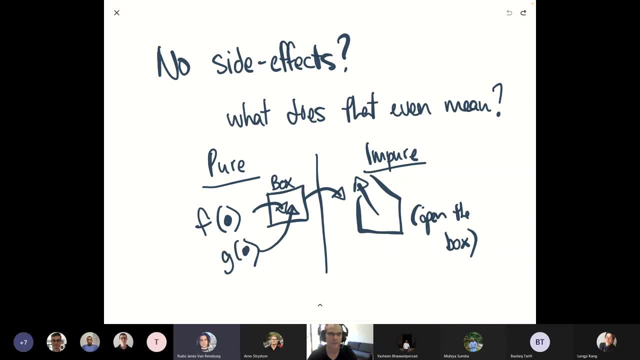 Um, certainly those who did comp sci at the university of Pretoria. we, we did again the basic stuff, but in scheme I guess that is pure functional. Yeah, I think it is. Yeah, Um, my comment is like: yeah, it's for all the um compile optimizations. 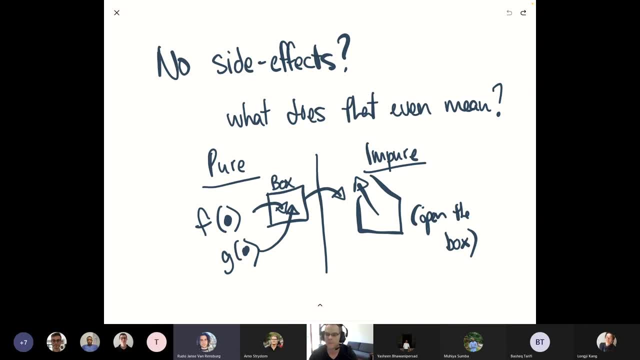 The only real control structures you have are recursion, So I don't know how efficient functional programming really is, but maybe I'll just Have a bias and any. that's my comment. Yeah, Okay, Yeah, Yeah. So it's a very good question. 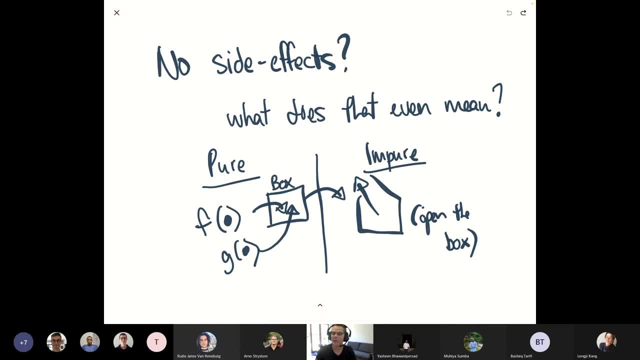 Yeah, That's one of the first things that. so, uh, like like one of the, the, the, the, the sort of initial complaints you may have about functional is like you go, yeah for sure. I have to now describe everything recursively because I can't modify a data structure, so I can't be adding things to an array. 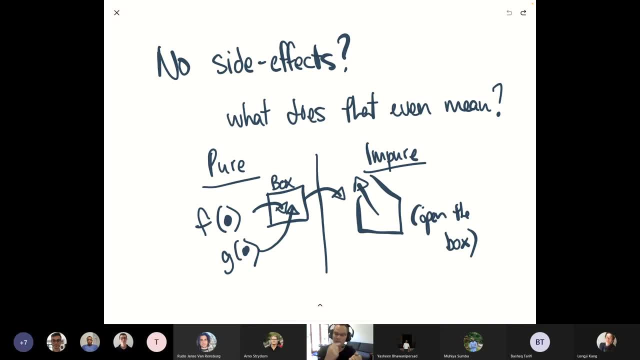 There's. I can't update that, that same array, right? I can't add new elements to an existing array. Of course I can describe a new array based on an old array with an added element, for sure. So I could create. I could create a second array which has got an, an element in addition to all the other elements in the first array. 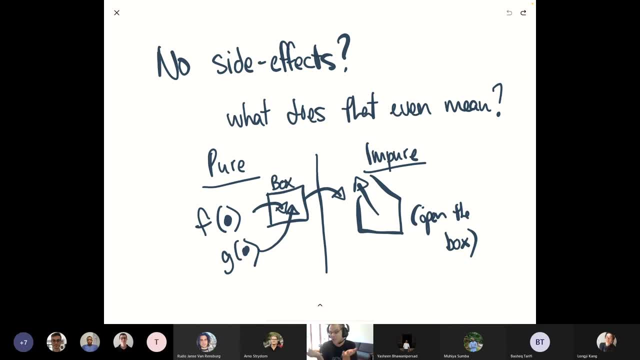 Right, So I can add elements to an array? Sure, They, just the results are different, They're different areas, right? Um, and so your first complaint might be: well, that seems very wasteful and very inefficient. uh, because now I'm copying data structures all over the place. 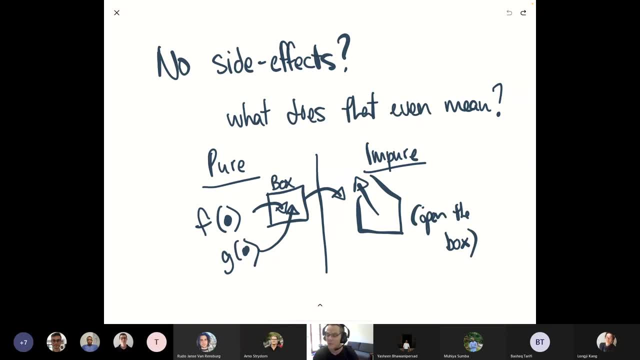 And actually the answer is no, you're wrong, that you don't need to copy them All All over the place. So if you know that your language is pure and that nothing can change within the first array, so when I create the second array I can just add the new element and pointed to the first array because I know that the first array will never change, cannot be changed. 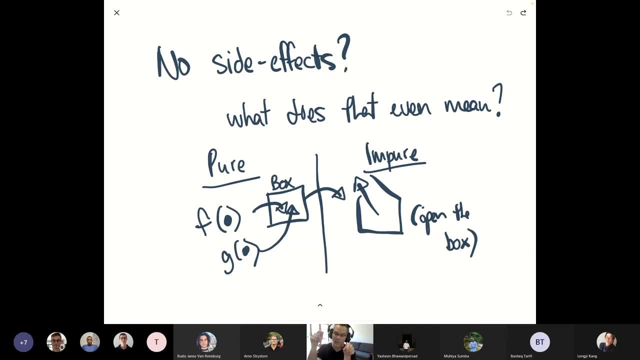 I can be actually be very efficient. All I need to do is just store the new element and appointed to the old array And that way I have a new array which actually happens to incorporate the second array as part of it, And because I know it can't ever change, I can never destroy the first array. 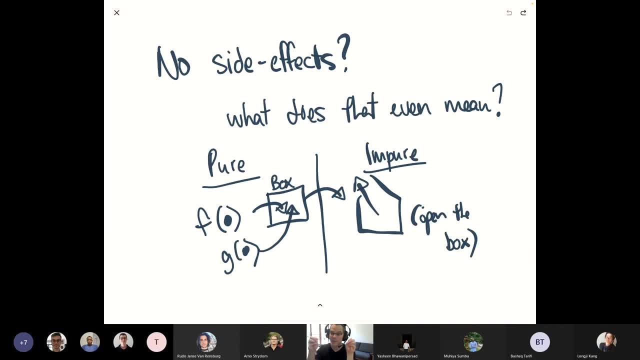 Does that kind of make sense? So, in fact, from an efficiency perspective, um data structures can be very efficient if they are immutable, because you can make assumptions about them like this will never change, So in fact I don't need to make a copy of it. 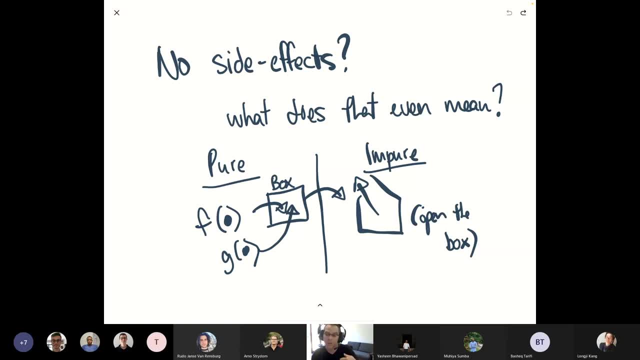 I can just have whatever wants to use it or modify it. just point to the original one. Do you know what I mean? So, uh, that that's often like a miss um uh sort of like naive misunderstanding of immutable data structure that it creates a lot of copies. 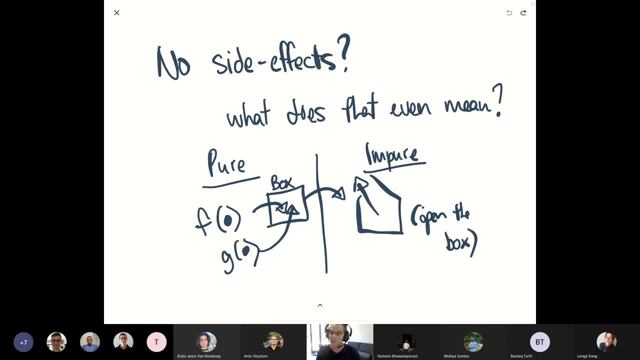 In fact, the answer is It doesn't create a lot of copies because it never needs to, because it it can assume that they never change. So, in fact, you can just reuse stuff which is not necessarily true of an, of um, of a language which has mutable data structure. 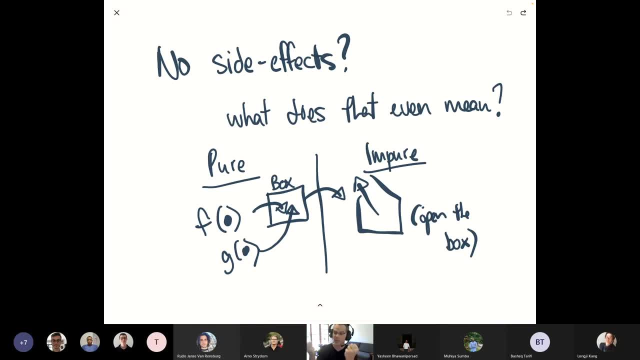 So if, if I had an array and I created a new array with some new elements in it and it just pointed to the original one, if I changed the original one, I would end up changing the subsequent one as well. Right, I would create this dangerous situation of like. 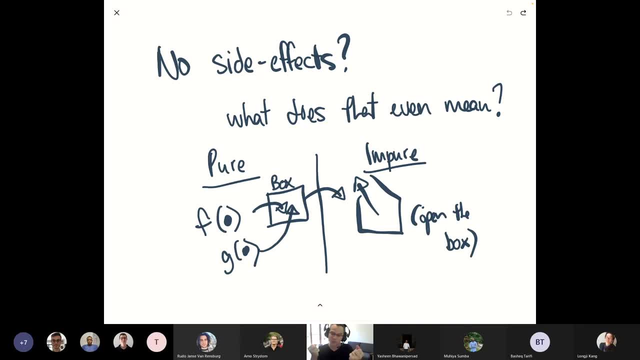 I'm Assuming this is a new array, but it isn't, because when I changed the original one, it ends up changing the second one as well. So in fact, in fact, in that situation I should copy right, I should make a separate copy if I want to defend myself from like weird and wonderful bugs. 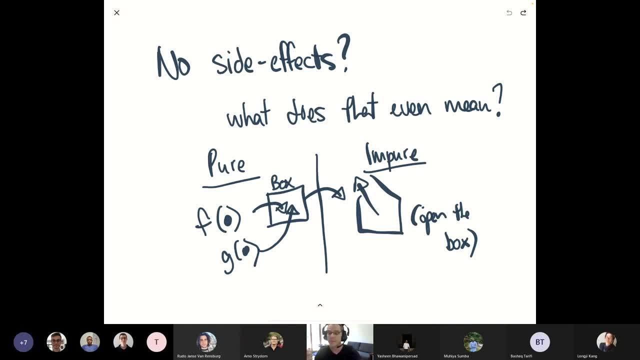 Right, Um, your, your point is around recursion, though, And so recursion, uh, um, you may, you may also think: yes, Okay, So recursion is bad because a function calls itself and therefore puts itself on the stack, of course. 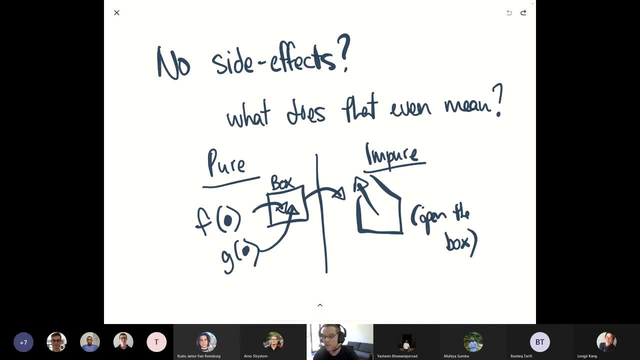 Right, Um, of, of course. So I think that's just an implementation detail. So in in, in, most compilers do do that. Yeah, So a function calling itself would create a new stack frame, copy up its variables, create a new stack frame, copy up its variables, et cetera, et cetera, et cetera, and create a very deep stack. 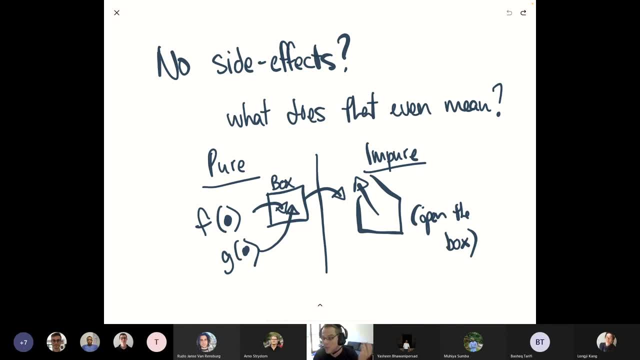 And, of course, we know that a stack is a limited size. So what, uh, what generally most functional languages that I mean out there, I mean other than completely useless ones. what they'll do is they implement something called tail recursion. Yeah, 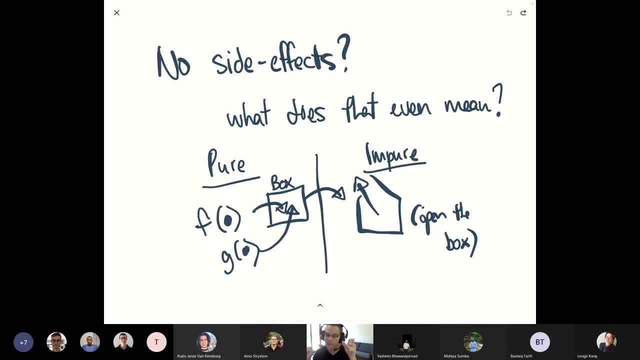 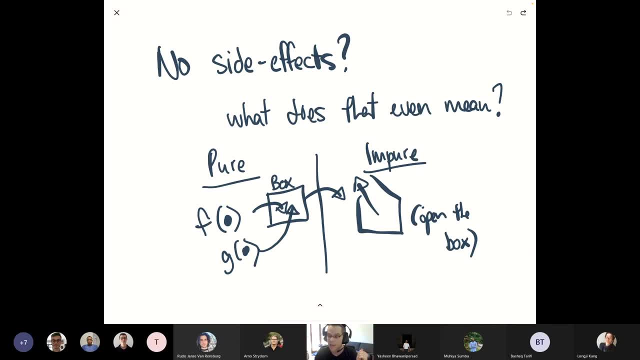 It will just unwind it into a, into a, into a regular ass loop, So it won't make use of the stack in order to run it. But there are some constraints as to how you write that function so that it doesn't make use of the stack. 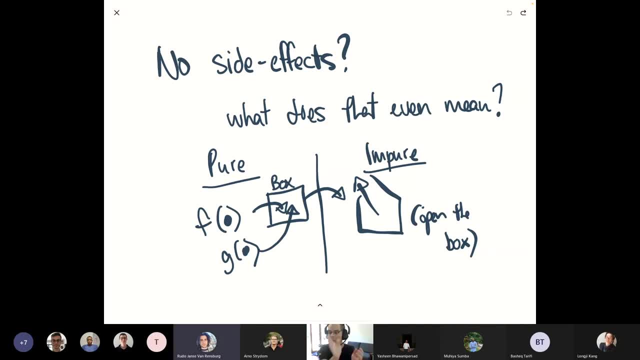 But you can google something called tail recursion that most compilers will use And they'll just unwind it, So they'll, so that you can recursively call it into the infinity, same way that a while loop can run until infinity. but it but it can. it can feel weird and uncomfortable. 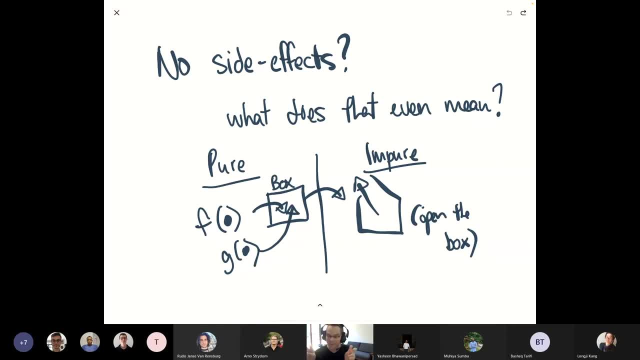 when you, when you sit down and you say, okay, i need to do like a four loopy type thing and i don't have a four loop, so well, i do, but i can't like add results to a thing, so it's like, oh shit, um, now. 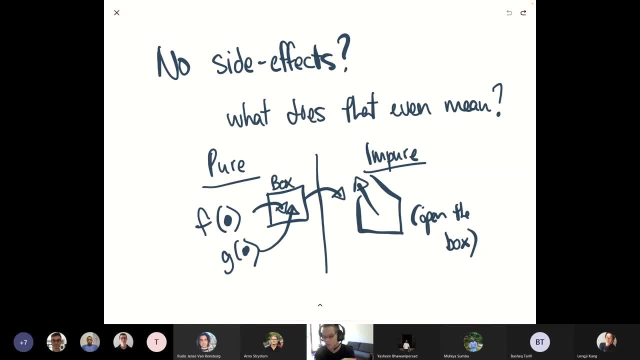 i need to think recursively. absolutely, you do have to think recursively. so when you think about looping through stuff, recursion is the way you do it. yeah, yeah and, and it is probably more tricky than um than regular kind of four loop, modify stuff, for sure, but but i would say that it's one. 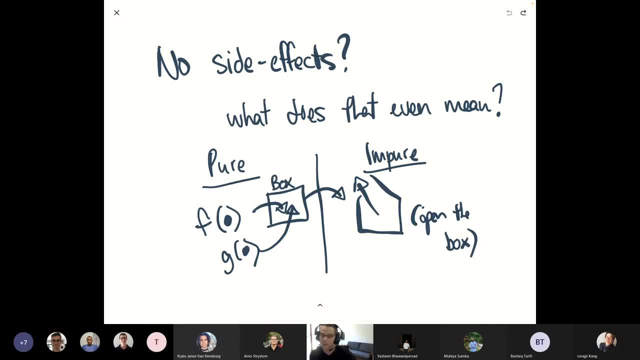 of those comfort things. right. it's like you're comfortable in the four loop world because you've written like hundreds of four loops and maybe thousands and years you've been using four loops. so then when you look at recursion, uh you go: oh, that's weird and it's difficult and my brain 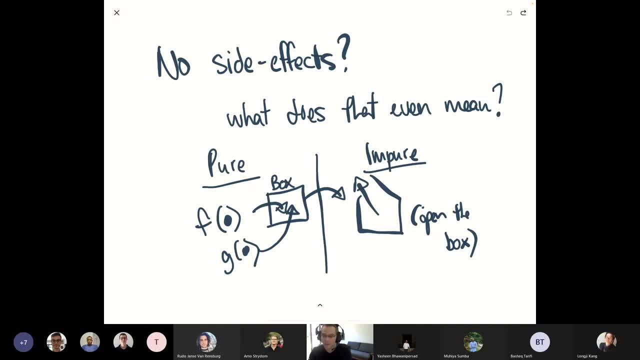 doesn't really understand this, but i would say it's like a practice thing: the more you practice it, the easier it becomes and in fact i think, like most of the- for me certainly- i default to recursion rather than four loops. um, i think i've actually got a. 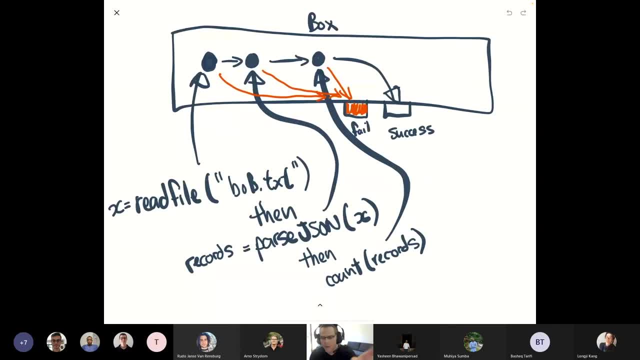 cool example of that. so let's just jump to that actually. oh so this was just a summary of like my boxing idea is, if you, you can kind of see this, this combination of boxing different effects. so in our example, where we had the the kind of like we did that read file thing, then we paused jason. 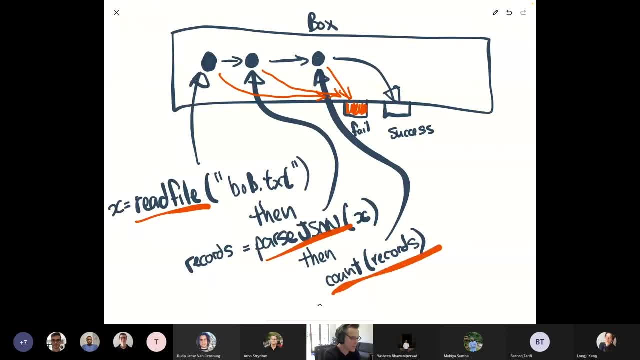 then in this example it like counts them or whatever. those things you can see are just like sort of putting themselves up into the box and so into. and then i pass this box back to the, to the, to the runtime, and i say, hey, my program's done it. unit. 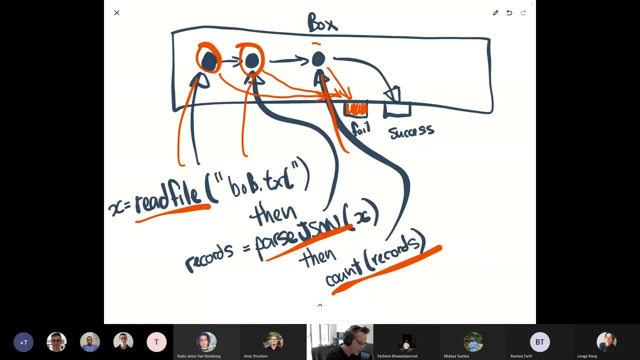 opens the box and then what happens is it will execute that, execute that, execute that, and if there are failure states like i, can also describe how those failure states work. you know what i mean? um, and so i'm not going to get too hung up on that. it's a bit of a weird and wonderful place, um, so i'll. 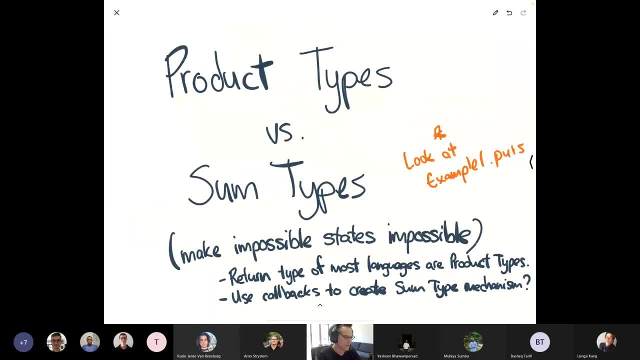 skip that one there, but i wanted to let you guys know that, um, we also have a. we have a bunch of tools that are really good for you, which is if you want to come to the gg tools. we've got a full list of tools and uh. you can go down and look at some of them and have some notes on them in. uh, you can. 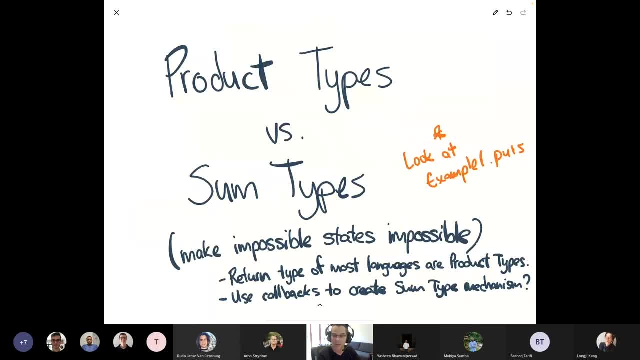 Okay, we talked about products versus some types, And one of the cool ways of thinking about it is, just like these four words here- making impossible states impossible. So I would say to you, when you're looking at your programs and your functions and you're trying to describe them through, like their type, signatures or whatever it is where they are impossible states, try to make them impossible. 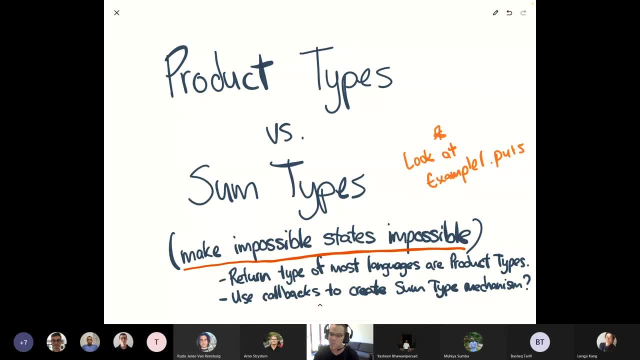 So in your code, try and make sure that those impossible states are explicitly impossible. Do you know what I mean? So that idea of having an error or a list of records, try and make that an impossible state, right? So because it is in your mind, in your perfect world, it is a scenario that you do not want to support, right? 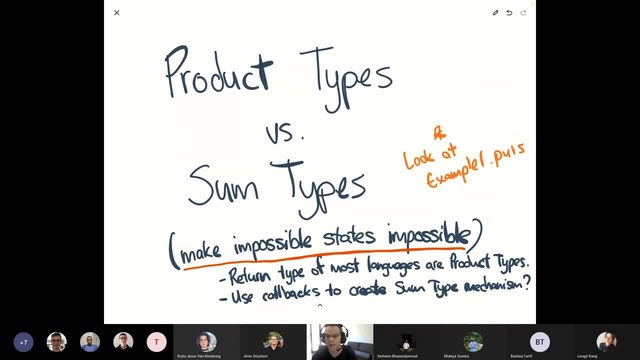 So it's an impossible state. Make sure that your code also makes that explicit. Unfortunately, in a lot of languages you don't have this concept of the sum type. Maybe you do like with an enumeration Or a union in C. 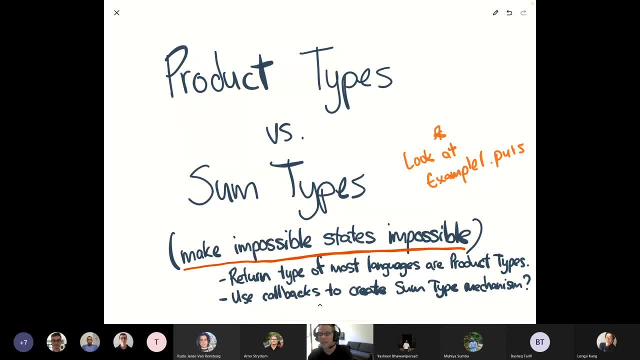 And hopefully you'll never have to deal with one of those. So maybe in other languages you might look for something called a discriminated union or an algebraic data type, an ADT or a sum type or an enumeration kind of similar kinds of things. 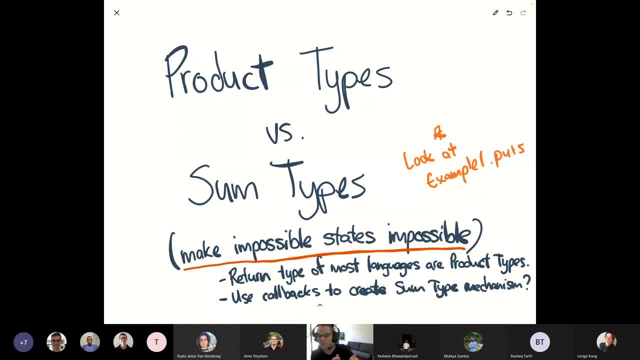 Unfortunately, enumerations don't often carry that extra piece of information that we were looking for. So remember when the enumeration- so for example, our thing- could return An unknown error with an error attached to it, or a result with an array of strings attached to it. 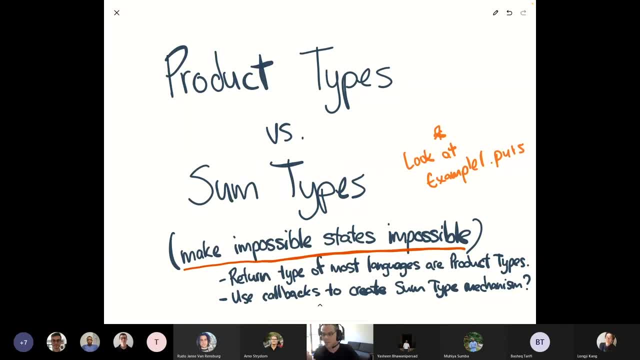 Enumerations don't often support the carrying of that extra little piece of information along with them. I think in some languages, enumerations do do that though, And so that's a good use of enumerations of carrying that extra piece of information, which is pretty cool. 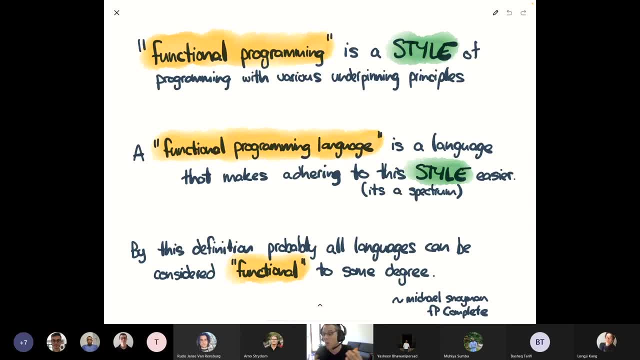 So this is just some blurb about what is functional. So functional programming- And this is a guy called Michael Snoyman. He's a Haskeller, but he's very outspoken in the FP community. So think of functional programming as a style more than like a technical thing. 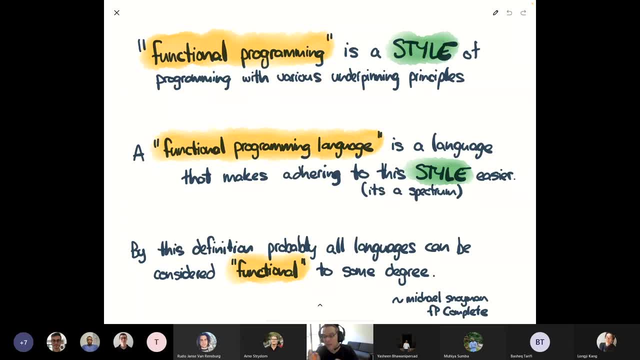 Functional programming is not a language-bound thing. It can be accentuated by particular languages. So certain languages make that style easier to adhere to and others make it a little bit more hard to adhere to. But the style is still a good one. 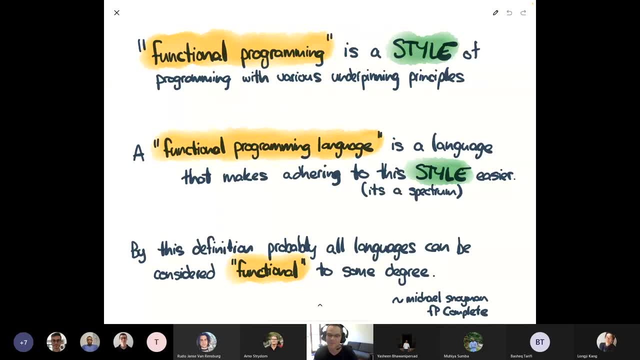 Because it's It's about making your code more explicit, right, Yeah? and so, like, a lot of languages can be considered functional. It's like a spectrum You have this idea of like pure functional languages all the way back to imperative languages that have a lot of functional features in them. 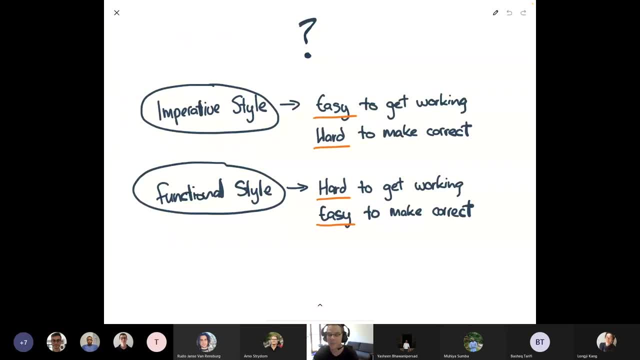 And so I think Yeah, yeah, yeah. So one way I like to think about this and this is just like maybe my own internal model, And like I'm not proposing, I'm not saying guys like write only functional. 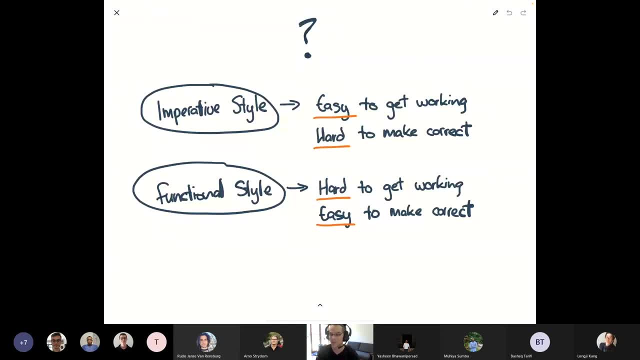 I'm not Like you know. that's completely a personal choice that you have to take on board And it, like, has big like outcomes attached to them, right? But when I think about these two styles, I see them as being trade-offs, right. 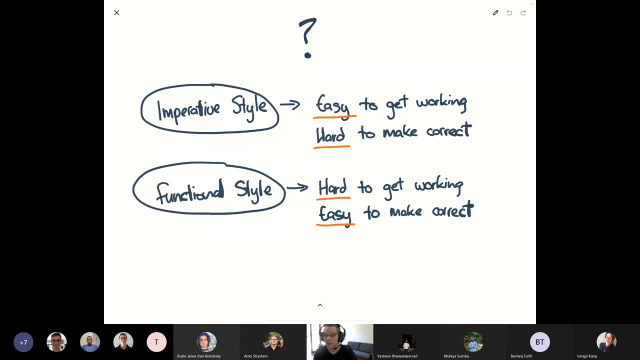 So imperative style. it's very easy to get working Like we saw this right. We had our five-line program earlier. It just worked, And it worked in 99% of the cases, But it's very hard to make it correct. 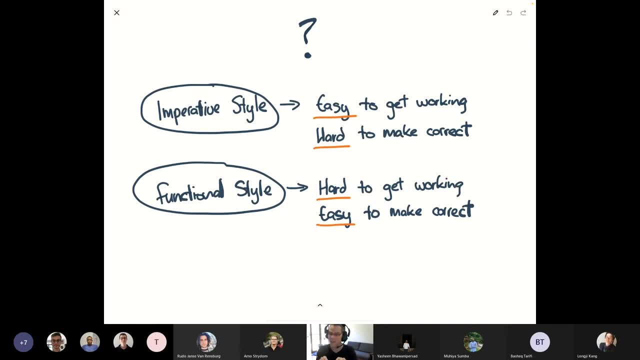 So when I talk about correct, it's like. It's like this thing is explicit about what it does And it handles every error scenario And it makes it explicit to the caller of it right, It doesn't hide, It doesn't throw away information. 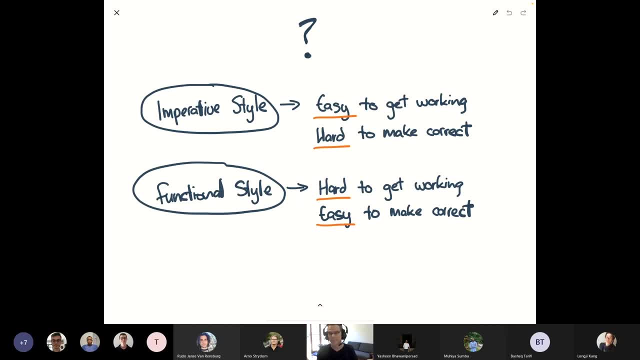 So where we caught an exception and then we just returned empty records, it's like it's not really correct, Like it wasn't. The file didn't have empty records in it. right, It was incorrect. We just We hid that. 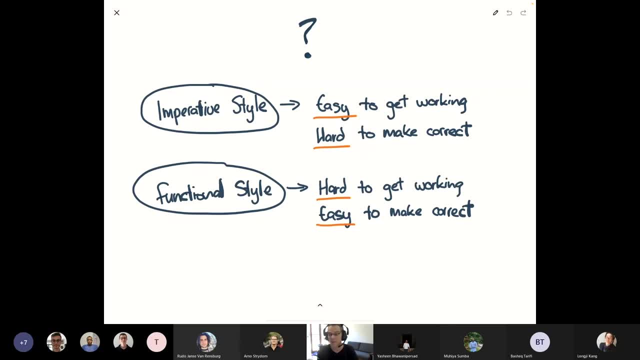 We just like threw it away because we couldn't, We didn't know how to deal with it right. So I would say that it's hard to make Using imperative style, it's hard to make your functions and programs correct, And I'm using like: not correct, not as in working, correct as in correct. 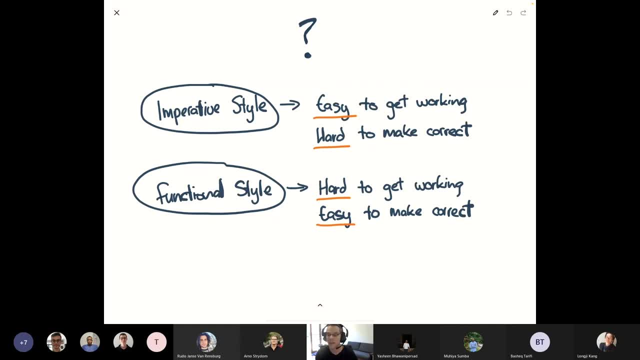 With a more functional style. for sure, it's harder to get working Absolutely And it's because you have to handle and be explicit about what is correct as you do that. But once you've got it working, often it is just correct. 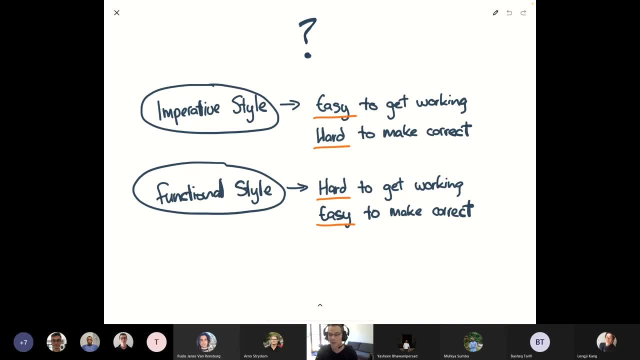 So it's like almost plus naught to go from working to correct very often if that makes sense. So it's kind of like If you're trying to get to correct, going through imperative is going to maybe hurt as much as functional. 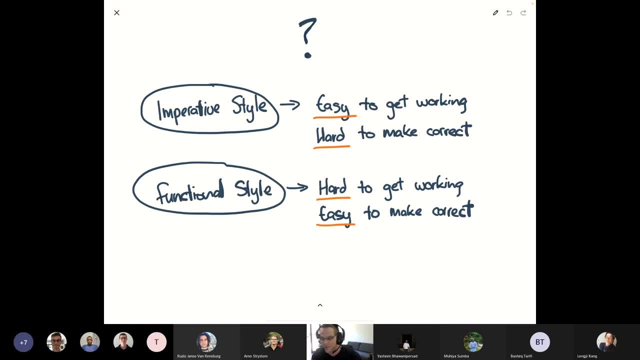 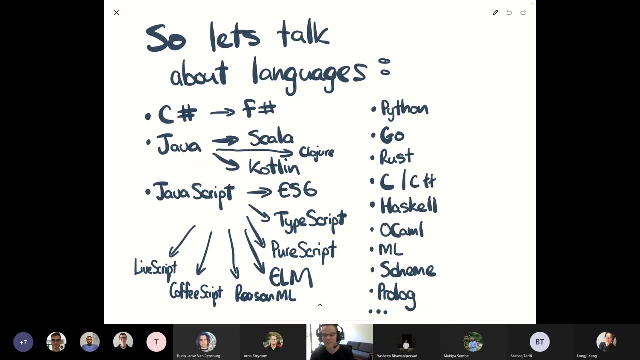 but you'll be at correct by the time you're at working, if that makes sense. Okay, So like I've just quickly put up a bunch of languages, I don't know all of these languages, I know a lot of them And look schema's on there. 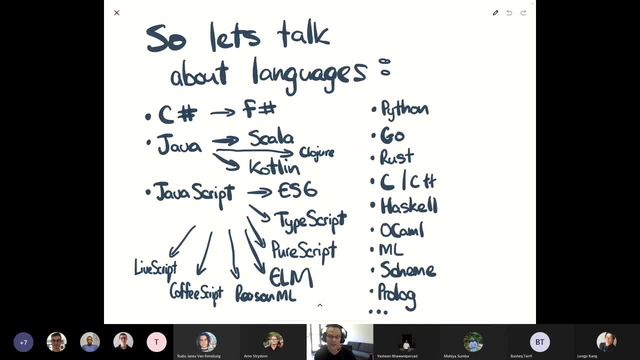 But, like I would say, almost all of these languages to some degree have got the ability to write pretty good functional style code In them. So C-sharp for sure is getting more and more functional over time. In fact there is a language called F-sharp which is not pure functional. 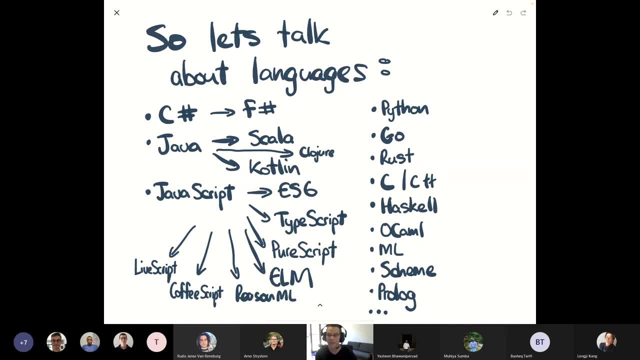 but it's got a whole lot of very interesting things like discriminated unions, ADT. some types stuff like that even into some simpler ideas around side effects and monads and boxing and unboxing and stuff like that, which I think is very cool. 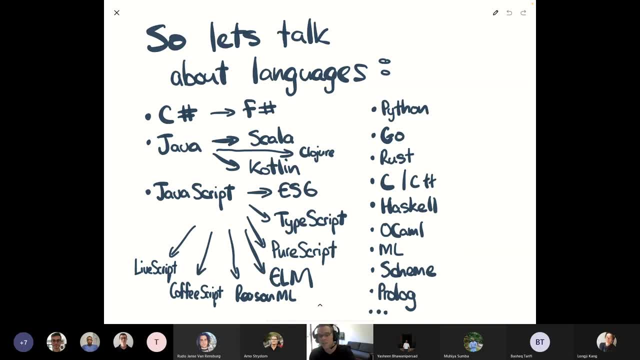 And if you followed C-sharp, So I follow C-sharp. I don't write a lot, I don't use C-sharp, but I definitely follow their release notes whenever there's a new version, Like you're seeing a lot of the new language features coming in there or like functional features actually. 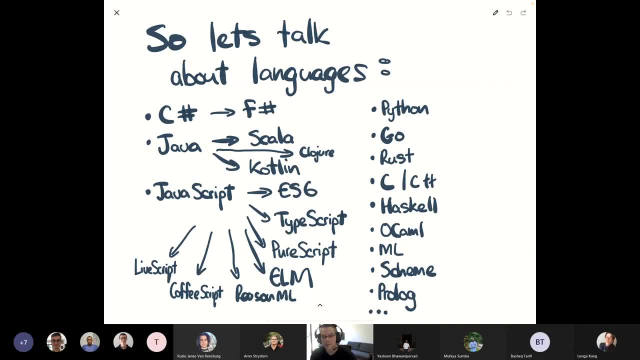 Java for sure is, I would say, in kind of the same boat. It's also trying, it's catching up. but there are some really good, more explicitly functional dialects within the Java ecosystem: Scala for sure, Clojure, Kotlin. 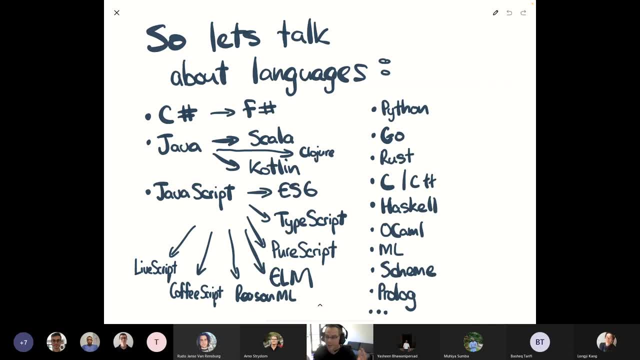 These things have got very much what I would call like they're functional or They're imperative languages. You could choose to go both ways, which is actually really cool. So C-sharp and F-sharp- 100%, You can say like. I feel like writing this little function in an imperative way because I'm comfortable with four loops and stuff. 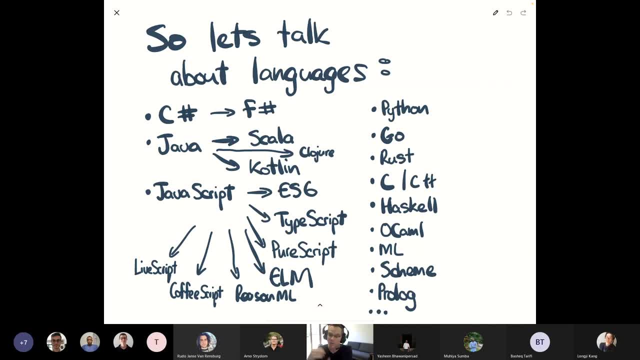 But this other little function here like: ooh, I want to be very explicit and I'm going to return some types out of my function So you can mix and match functional and imperative style very easily in C-sharp, Java and their ecosystem. 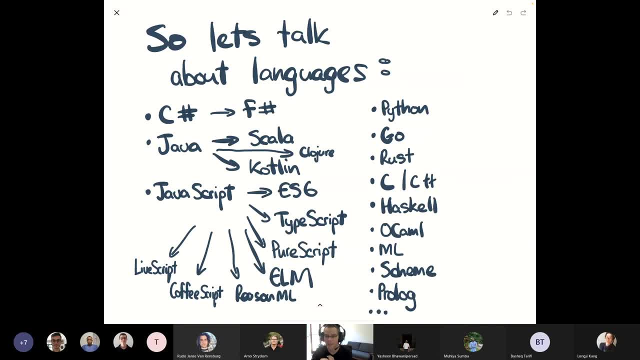 So Scala, Kotlin, Clojure, for sure, JavaScript is like 100% in the same Same situation. In fact, I would say JavaScript is probably a lot more tending towards the functional side And if we specifically look at its like dialects, so the other languages that compile to JavaScript or that are in the same ecosystem, right. 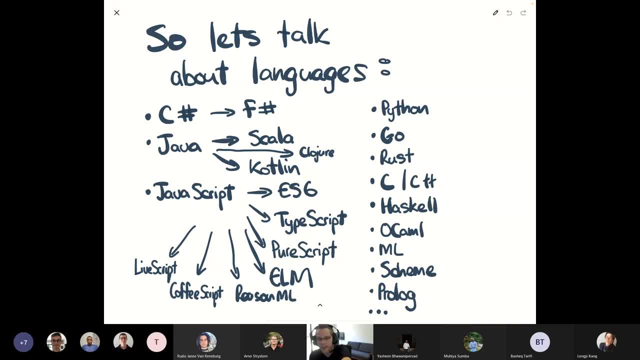 So ES6 is JavaScript right. TypeScript, for sure, is probably accentuates more, like the type system, maybe less accentuation or functional, Although I'd say I'd prefer to use TypeScript over ES6 because it does do some cool stuff. 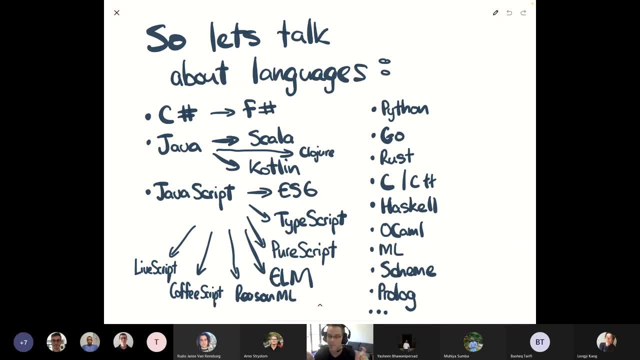 It does do some cool stuff around being more explicit around types, which I really like. I think type systems are good. Functional style is good. PureScript we saw earlier, it's a pure functional language. In fact, it even takes you to that pure side which is like hey, even effects and side effects have got to be put in these boxes and the compiler will enforce that stuff. 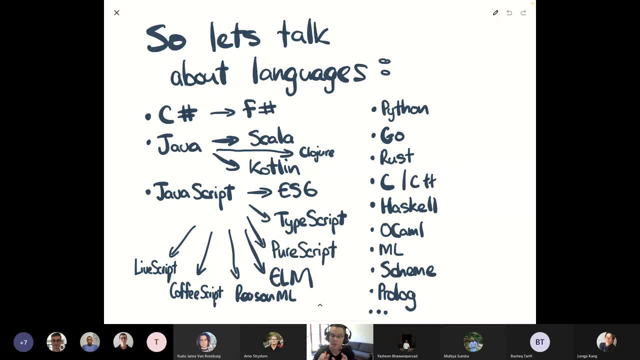 So you can't just have like a consolelog somewhere randomly in your code. You have to put that in the box right. Elm is a very interesting one. I don't know if anyone's ever looked at Elm, but it's a web programming language. 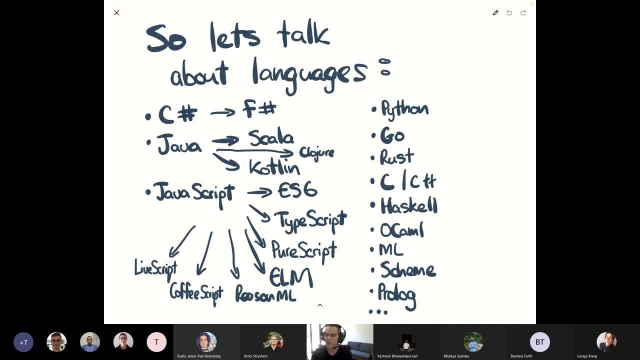 It's a web programming language And I actually I actually have a cool example. I don't think we're going to have time to like go through it, But Elm is super cool as like a toy language to really like build something in a pure functional way and go through the pain and hardship that is associated with it, but in a way that's pretty fun and interesting and it's a very limited language. 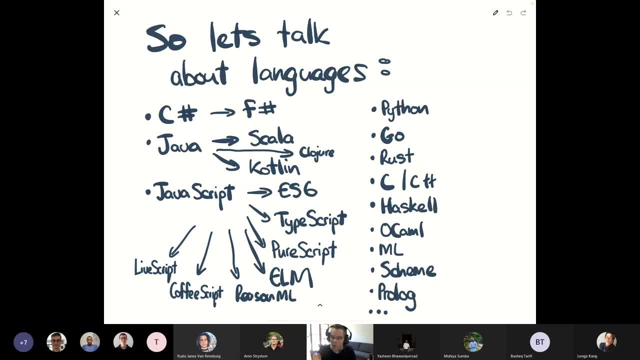 So, like it really takes away like this burden of knowing, like what is a monad and a semigroup and a functor and all this stuff, It literally says, hey, this is all you got. You got these like three tools. 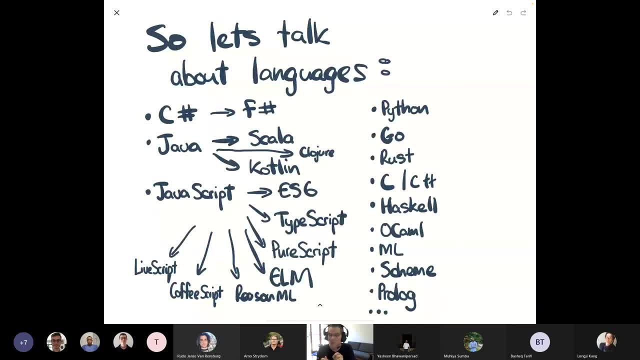 And this is how you're going to build web stuff And try and build web stuff with Elm. I wouldn't like recommend it for, like, big production stuff, but for toy and learning projects. I think Elm is great. It's really really cool to get into. what are ADTs and all that stuff. 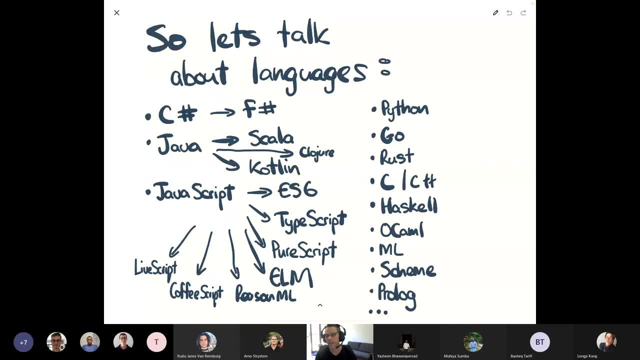 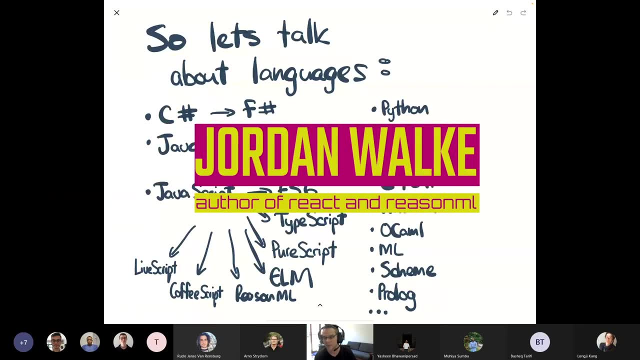 Reason: ML is another very cool one in the JavaScript space and this is by the author of React. So if you guys have used React and React Native- I don't remember the guy's name, but he got very excited about functional. It was about 2016.. 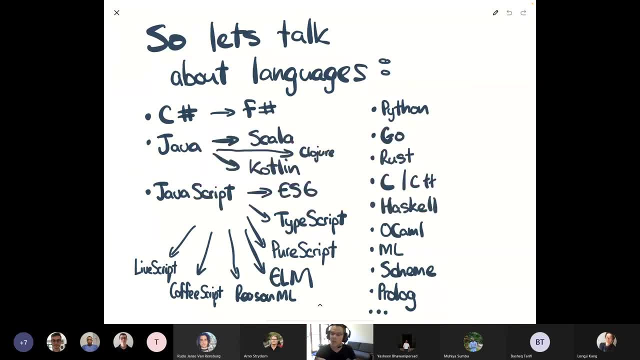 So he built React. He was very inspired by a bunch of things going on, but he wasn't a functional programmer, Not really. While through the journey of building React has realized that actually functional programming is the answer for React and in fact has created his own dialect on top of a language family called ML, called Reason. 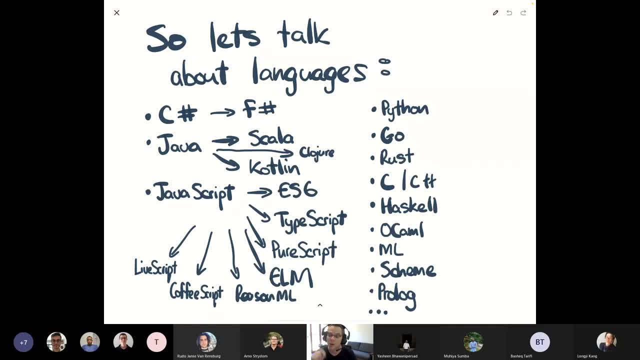 And so ML is Today. if you want to write ML, you'd probably use OCaml. Yeah, so OCaml is like a dialect of ML. ML is a family of languages and Reason. ML is, I suppose, like a stepson of OCaml, but compiles to JavaScript using something called BuckleScript, and it very much accentuates the React. 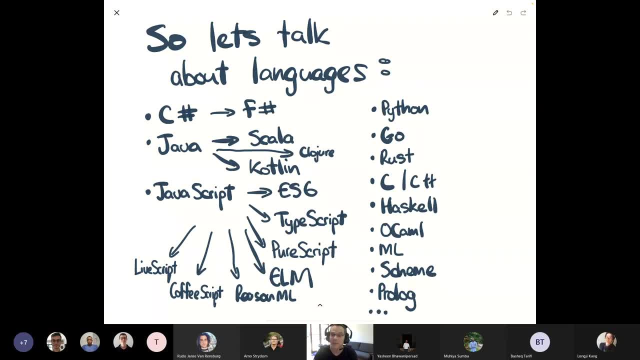 So if you like React and you've been writing React in TypeScript or ECMAScript, you may feel the pull to be pulled into Reason ML And I would say go for it, Go and try it out. Reason, Reason ML. It's a functional slash imperative. 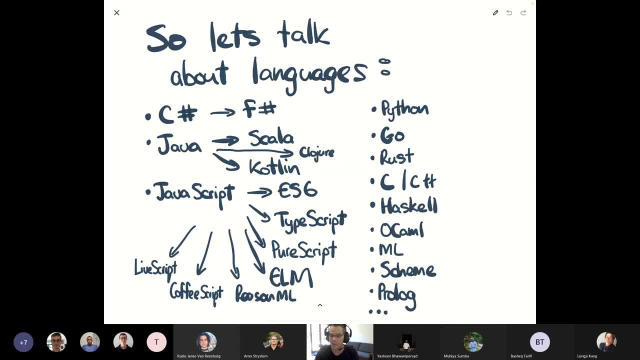 It's not pure, which is really cool. So it's like: easy to pick up, easy to go, easy to be productive. You can write for loops if you want, but you can also be like have the power of ML underneath you. 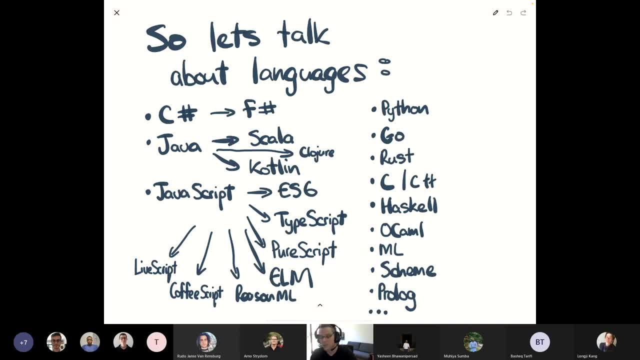 CoffeeScript, LiveScript- those are also, LiveScript being more probably functional. CoffeeScript may be more object-oriented But, like Python, unfortunately doesn't have great pure functional or any functional stuff. It has this concept of a lambda. 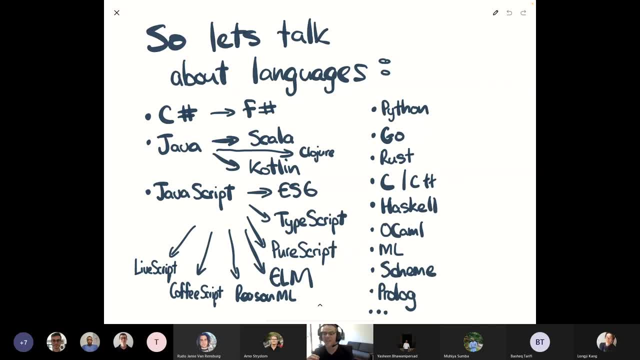 It doesn't really have high-order functions, unfortunately, Like Python really sucks from a functional perspective, I think it's just painful to write functional-style programs in painful It can be, And so you quite often just default back to like imperative style. 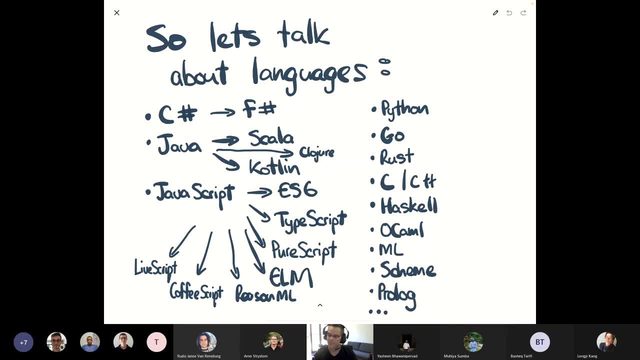 Go, I would say, is almost in the same category as Python. It's very OO. Anyway. it loves mutation, It loves null, It loves returning nils from functions, that kind of stuff. Rust is, I would say, quite close to being an almost pure functional language. 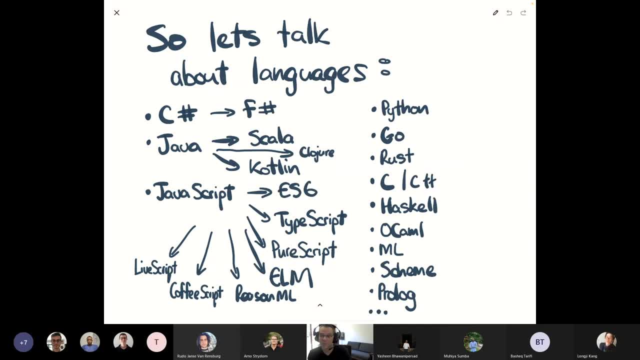 Very functional C and C++. actually it's pretty easy to flip over to a more functional style. Haskell is pure functional. OCaml is functional, very much on that spectrum. It's not pure. ML is the same Scheme? I don't actually know that well. 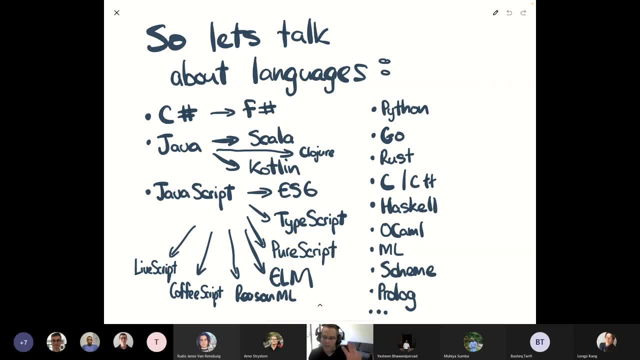 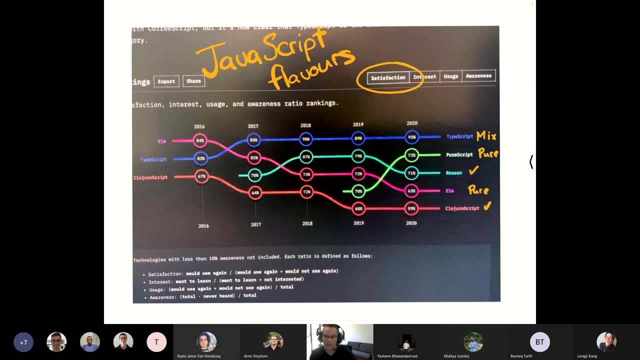 Prolog I think. I actually don't know too well either, other than it's got some other interesting language stuff. So anyway it's like it's available. You can do functional style in almost everything, even Python. 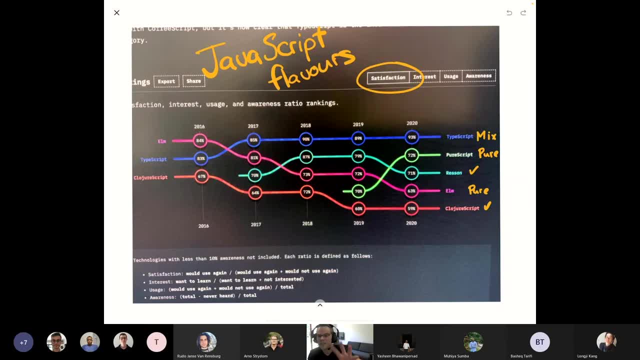 Oh yeah, I found a cool picture here. Actually, it's like this: It's a satisfaction index of people using JavaScript and its various like dialects. It doesn't have all of them, but it's got like, I suppose, the most popular five dialects of JavaScript. 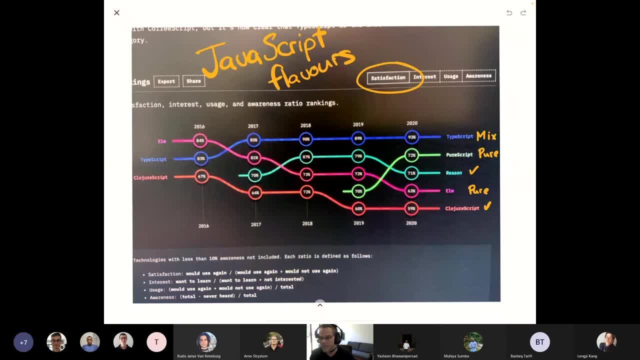 TypeScript 100% at the top. 93% of people are satisfied using it. And TypeScript is a mix of. you can go imperative, you can go functional, you can do both. You can mix them together. Interestingly, PureScript is at number two on that list from a satisfaction perspective. 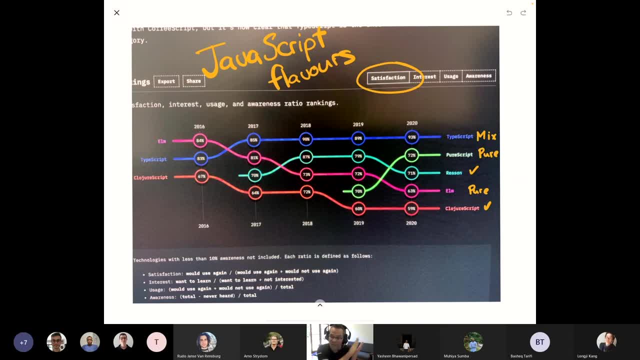 And it is pure functional. So it's not even on that like Spectrum, it's like hardcore, Hardcore, pure. You can't consolelogprint, You have to use those boxes and all that stuff. Reason is on there as well. 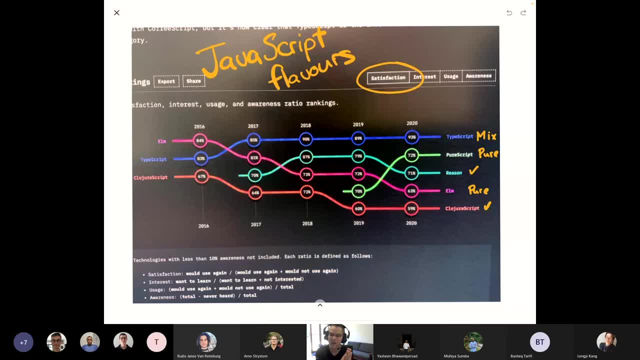 Elm is pure as well. It's also far on the other side of the spectrum And ClojureScript. So it's interesting that of the like five there, I would say four of them are functional, like functional languages. 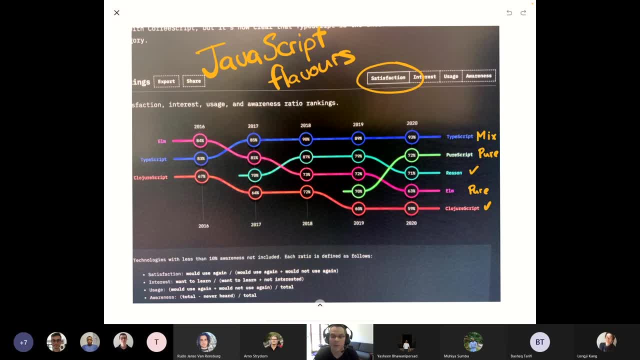 And two of them are at least pure functional languages And you can see there like increases in satisfaction over time. So like be aware of this stuff, man, Functional, Don't run away from it. Ask the hard questions and answer them, and experience these languages and see what they do for you. 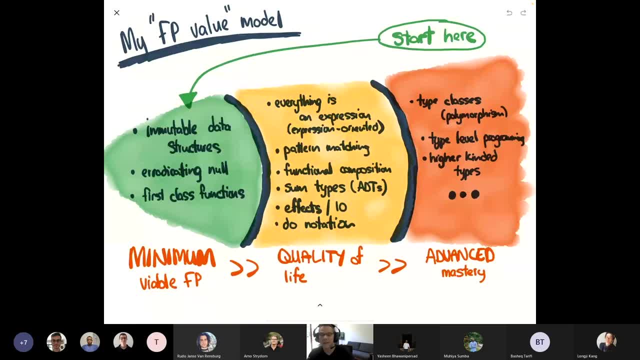 So when I think about functional programming style and it's like my model, for it is like a value model And it's the value to you as an individual right, It's a very big world right. So you've probably, you know, in your past if you've written a lot of code, it's probably been primarily procedural or imperative. 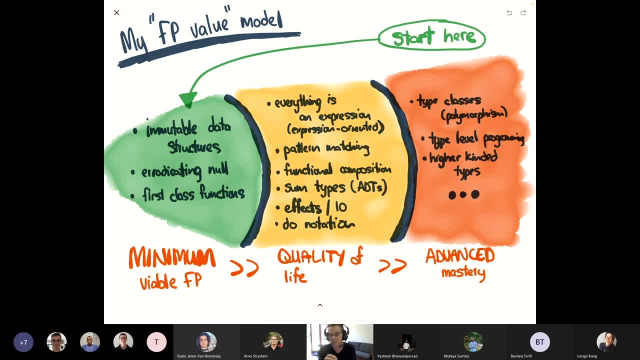 And that's okay, And you've got a lot of value out of it, And that's great. With functional, you might be at the start of your journey, or you might be in the middle or whatever it is, Or maybe you haven't even begun or whatever. 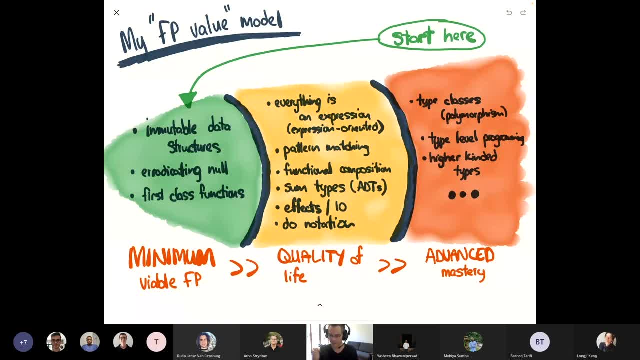 This is how I certainly feel And certainly for me: functional programming style, unlocked value, And so I just put it in these like three sort of like onion rings, The green one, like I call this minimum viable FP. 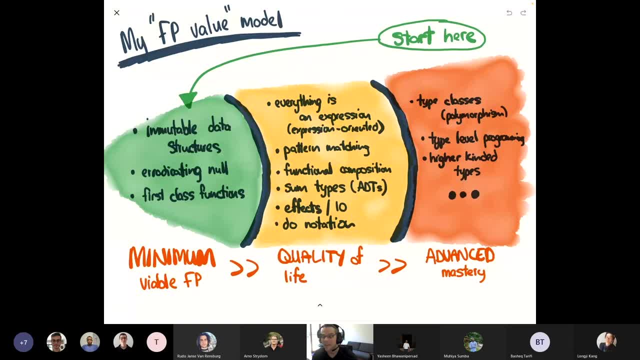 So taking on a style which is like minimum viable, Which is to say, hey, like where I get the opportunity to write this more functional and make this code better, Like I get tons of value actually from doing that, 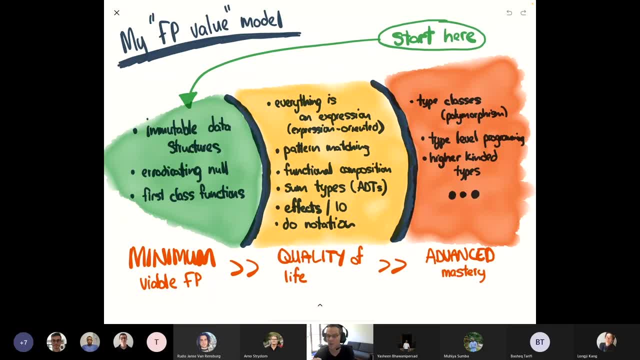 And it doesn't have to be complicated and like hardcore functional type of code. It can just be these simple tricks here, which is like immutable data structures. I really believe this is a strong one. So when you return data to someone or someone passes data to you, it would be nice to have the guarantee that it won't be changed. 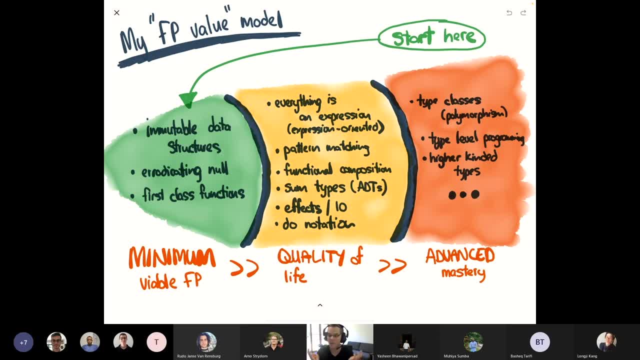 You know what I mean- In the future or whatever right. So like that's a very nice guarantee And I'll. I think there's a little example, maybe later, where we talk about it: Eradicating null. This is like null is such a bad idea everywhere. 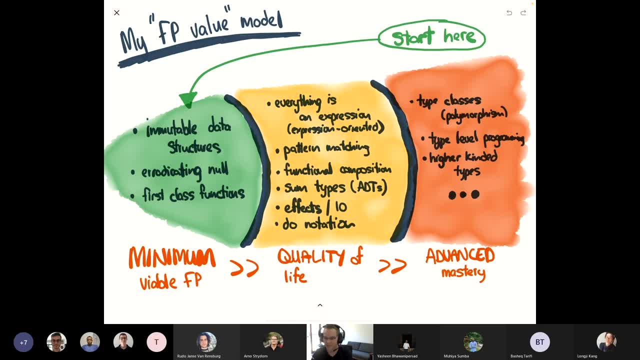 Like there's no good reason to use null ever, ever, ever, ever, ever, ever. Don't use null Ever. Don't return null, Don't accept being returned null. Don't pass null to stuff Like it's a bad idea. 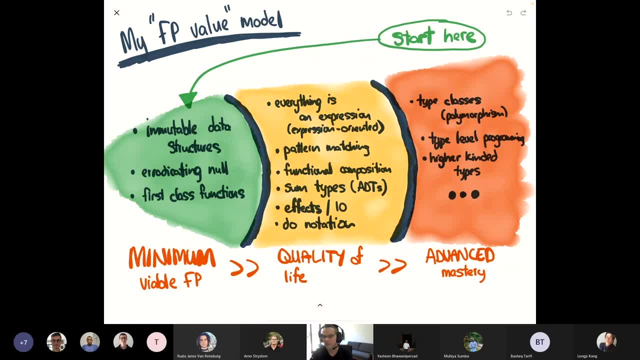 Don't do it. Rather be explicit about what your stuff does. You know what I mean. Either it's a string array or it's an error. What is null? What does that mean If I return null as in the place of the string array? what about the poor guy who goes for each on that thing? 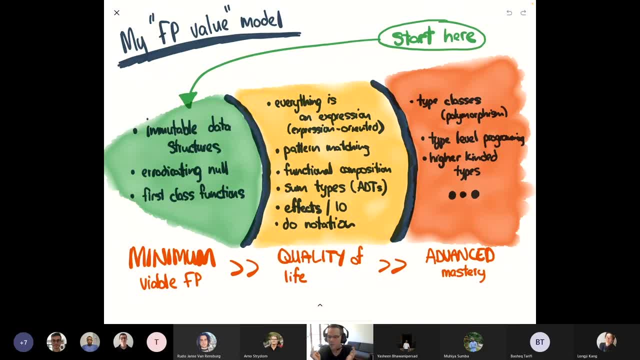 He just blows up Boom. Do you know what I mean? So use null like Null is the absence of. It's a weird one because it's not binary, right? So if you think about, If you think about like, what is null? it adds one more state to everything. 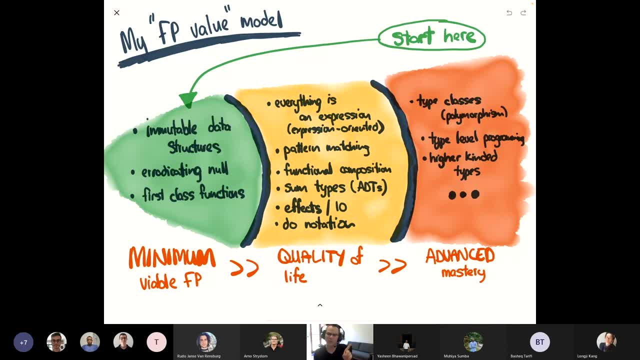 So like, hey, I've got an object or I don't have an object. Then I have this like pointer to an object which could be null. So it's like, oh, there's actually a third state That the object exists. the object doesn't exist, and then my reference to it doesn't point to anything. 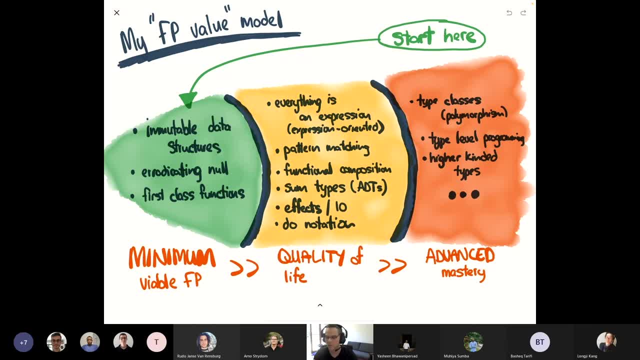 It's like: oh, that's a third state. It's like: it's terrible, Try and reduce it everywhere. It's almost always a problem to have null. First class functions are also really cool And our example earlier of JavaScript where you passed functions into a function and that function executes those functions. those are called first class functions. 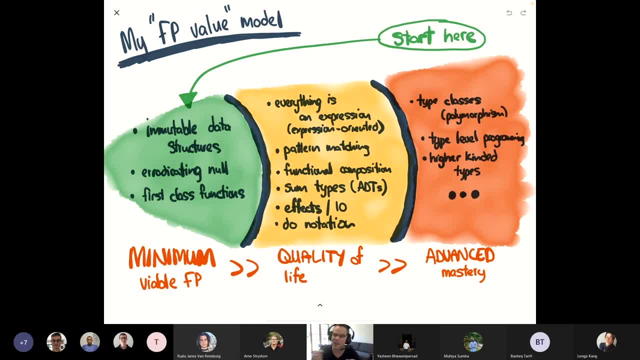 And they're first class because they're passed around, just like any other variable would be passed around or any other value, right? So they're Kind of first class. That's the way to think of them. So often a function like map or filter or whatever those things are quite often first class functions. 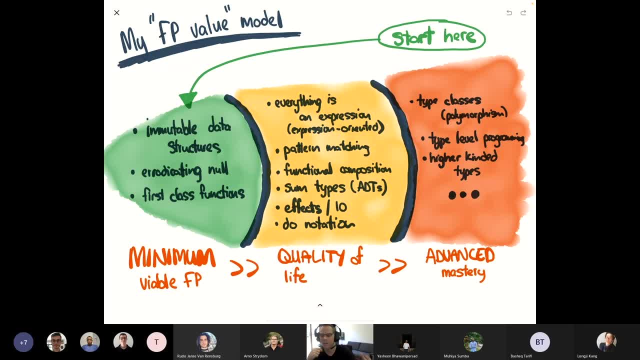 Yeah, Yeah, Yeah. Actually they're higher order functions which take first class functions as arguments. Anyway, first class functions are cool. I think that they're very useful And I don't think that they're difficult And I think they're easy to pick up. 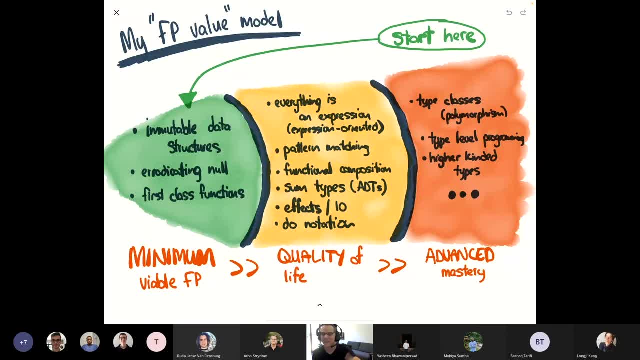 So, like in wave, one minimum viable product, minimum viable FP, like those three things like just do that right And be aware of them right. As you move through the onion layers though, it's like actually there's some cool quality of life stuff that can appear. 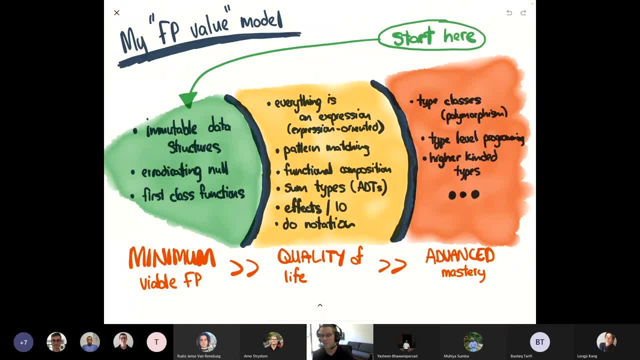 So the more you delve into some of these things, like the concept of everything is an expression- is actually really interesting as well. I don't have a good example here, but like, for example, the if statement in JavaScript unfortunately is not an expression. 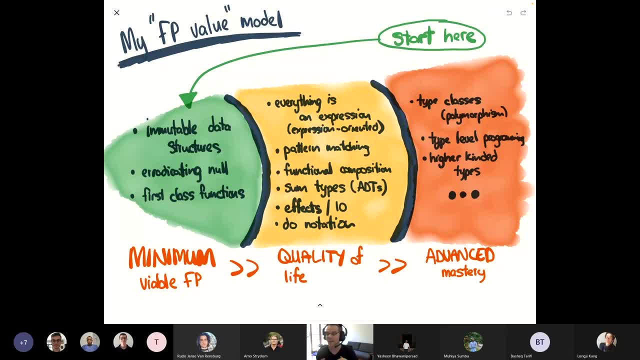 And it's quite sad that it isn't, but it should be if you think about it like a case. a switch statement should be an expression like everything should have a return value, if that makes sense, And the cool thing about that is like things start to compose together, if that makes sense. 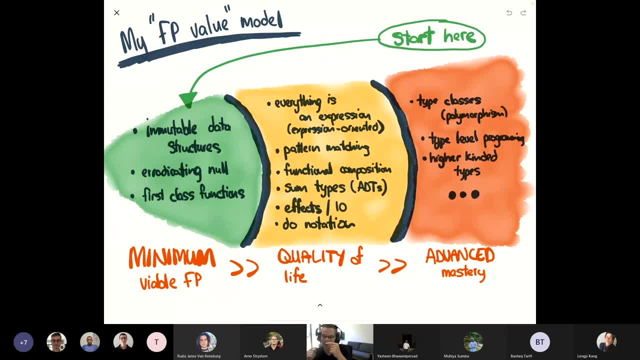 Whereas with when things are statements and they don't, what they're doing is they're intrinsically modifying state of stuff outside of them. if that makes sense, Does that kind of make any sense? No, I could. if we had time, I could give you an example. 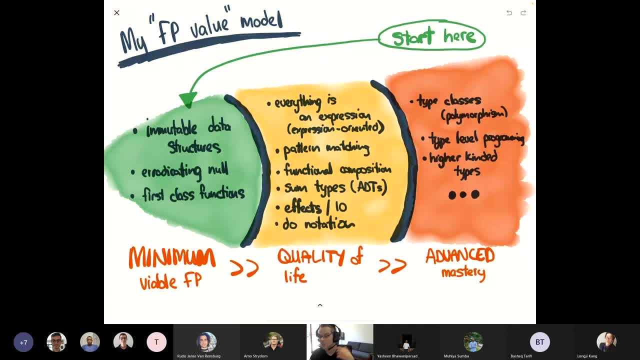 But anyway, everything is. expression is cool, Pattern matching is really cool in a bunch of languages. You should totally look at this stuff And that's. I showed an example when we were handling that ADT and that pure script that we had to do a case match on it. 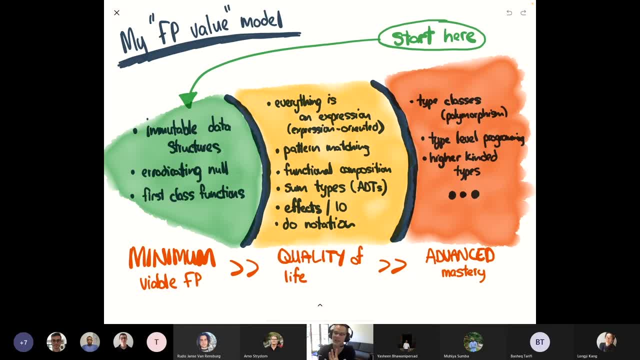 And that's called a pattern match, which then destructures the thing that that particular state is carrying around with it. Hey, it was successful And here's your list of records. That's a pattern match. That's unpacking that for me. 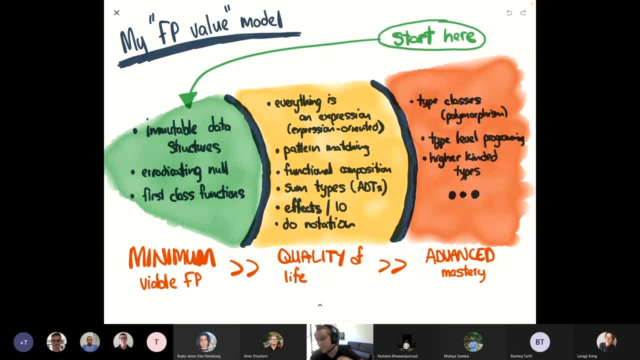 Sometimes there's many other things you could get, And advanced it's almost endless. There's probably like more and more layers as you go through this thing And I would say I'm like I'm like getting into this like third level of stuff. 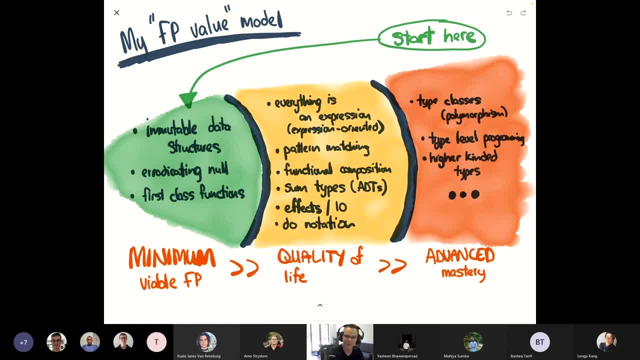 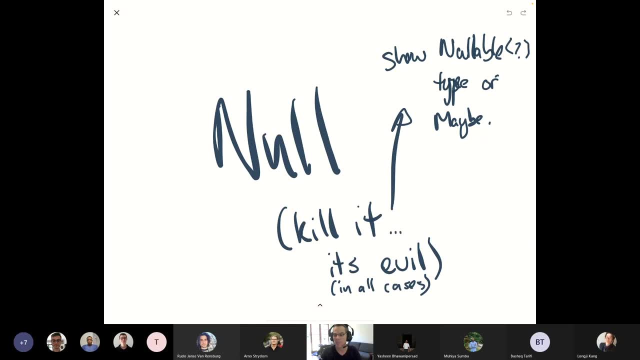 Yeah, null, kill it, This one. I don't want to hear any arguments. Why is that not changing? There we go. So there are, like, other ways to deal with null, Like the idea of the nullable type in. I think it's in C, sharp maybe, or Java. 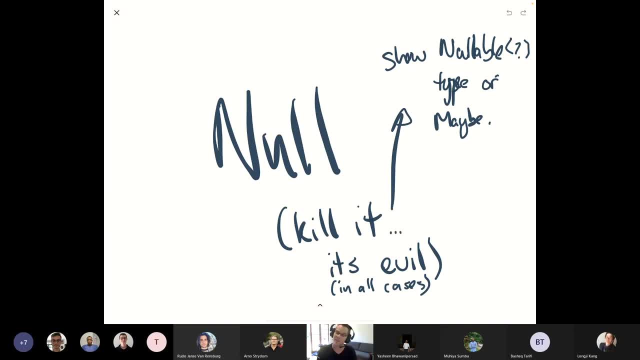 In Scala you would call it like the maybe, type, et cetera, And like that's explicit. Because if I call a function And it returns a nullable string, it's like: oh cool, it could be null or it could be a string. 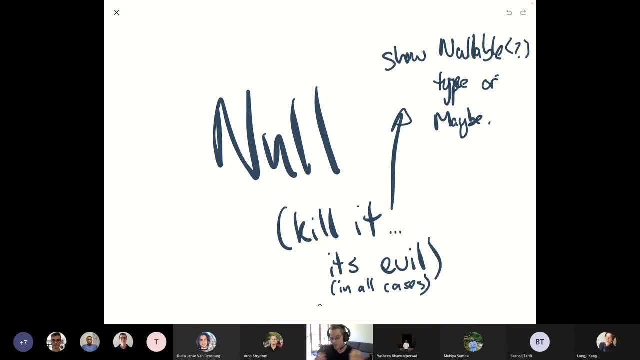 Makes sense to me, right? Whereas if it says, hey, I return a string, And it like turns out that string's null, Then screw you, man, Like you hit me with a null when I wasn't expecting it, Rather wrap it up in this thing called nullable right. 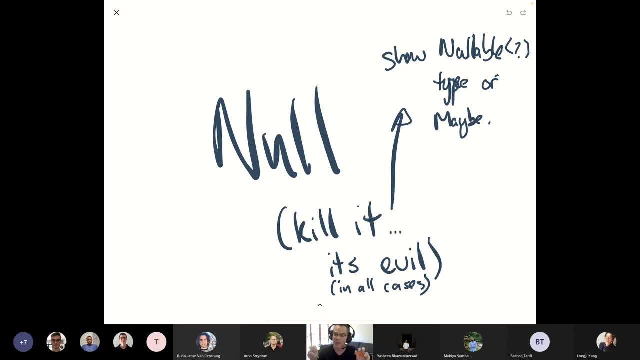 Makes sense, right? A lot of languages are going this way. They're getting rid of null by introducing a generic type called nullable or maybe, or whatever. To wrap it up, to make that code more explicit: Immutable data structures- we talked about it. 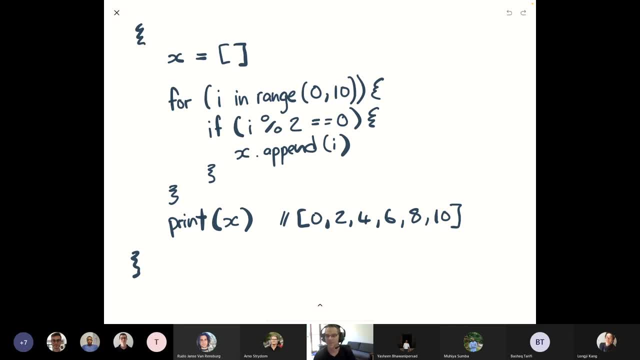 But here's maybe the last example of code around and this is maybe just something to stick in your mind, But when I look at this code, right, And I'll read it with you- It's very easy. So it's in whatever language you choose. 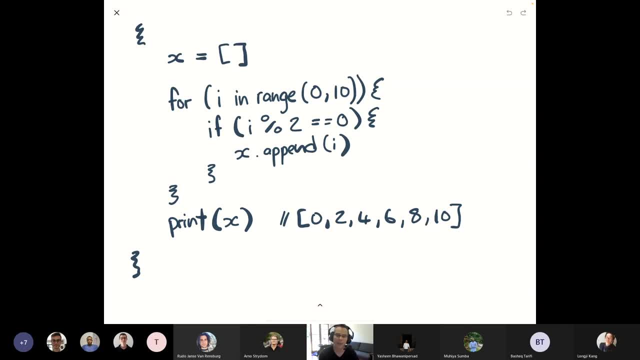 So X equals empty array, right? So X is an empty array. We're happy with that. yes, Then we go through a for loop And this looks Pythony, I suppose Because it's got brackets and stuff, So maybe it isn't. 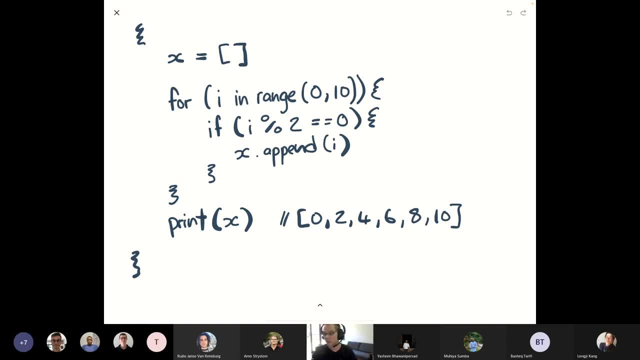 And maybe it's neither So for I in range 0 to 10.. So whether it starts at 0 and ends at 10, who cares, But it goes through a loop of 10 or 11 things. right If I mod 2 equals 0.. 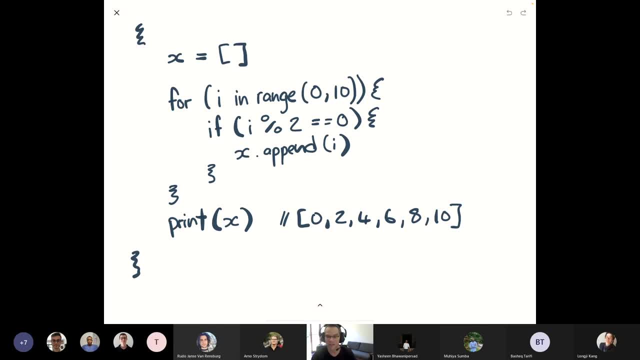 So that's kind of looking like. is it divisible by 2?? If it is divisible by 2, then add I to the array, right, We're comfortable with this right. And then at the end of that we're going to go print whatever is now in X. 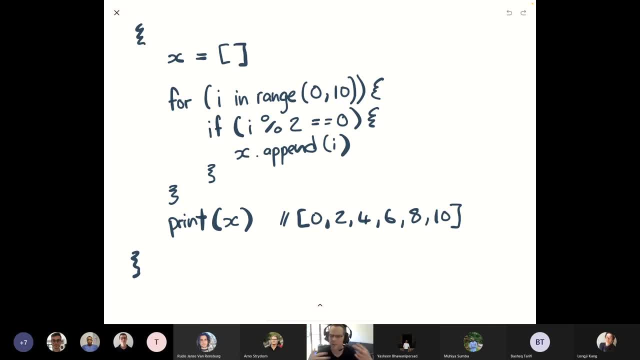 You're happy. So it's kind of like it's the even function. It's like figuring out What are the even numbers in the range 0 to 10? You're happy with that. So my problem with this- and I don't know if you- is like this code sucks man. 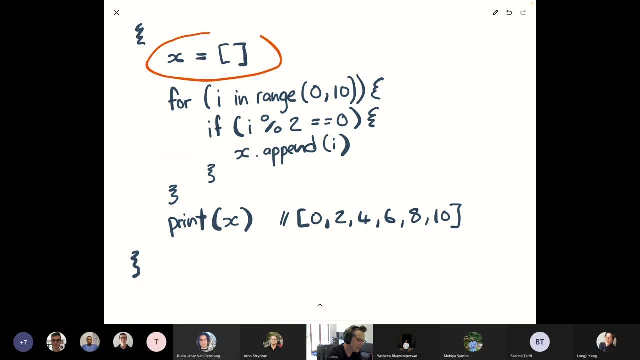 And do you know why it sucks? Because what you said to me here is like: X is an empty array, right? So when I ask you like so, what is X here? I would say, well, it looks like it's an empty array. 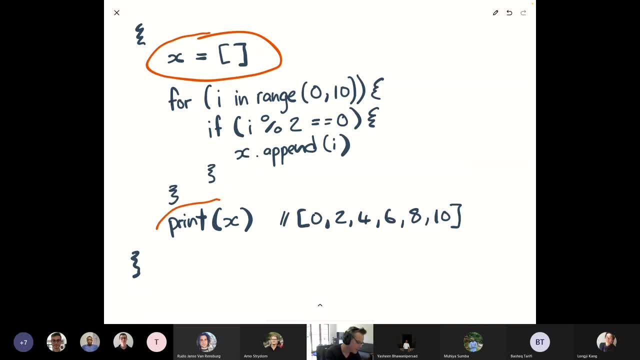 That's what I would say, Right. However, when I down here, it's like, oh shit, it's not an empty array, It's like got stuff in it. So it's like, well, OK, so what actually is X? 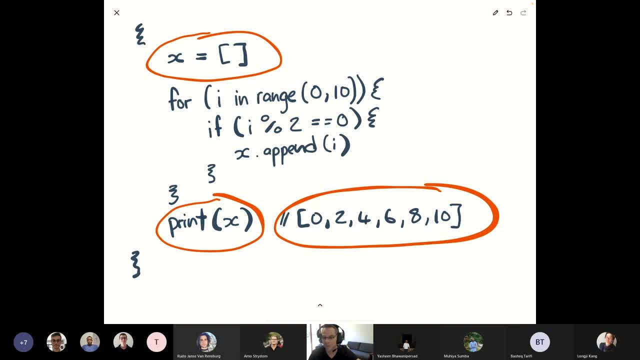 Is X an empty array or is it an array with the even numbers between 0 and 10?? And it's like: well, it depends on the like where you are Right. So if you ask that question and you're something here, it's like who the hell knows. 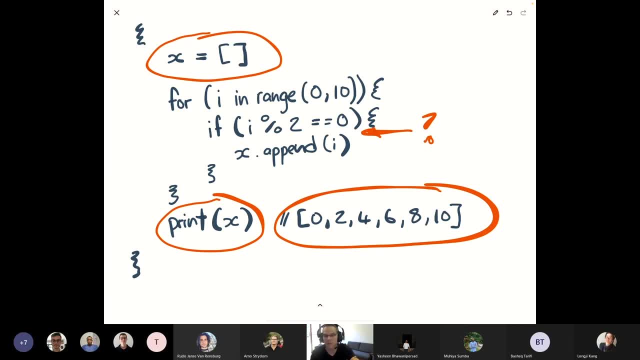 If you ask the question, if you were there, It's like, well, I don't know, it depends on how far, whether you've appended an eye to it or not, or where you are in the for loop or whatever. So it's like actually like this is a big freaking, like lies everywhere here. 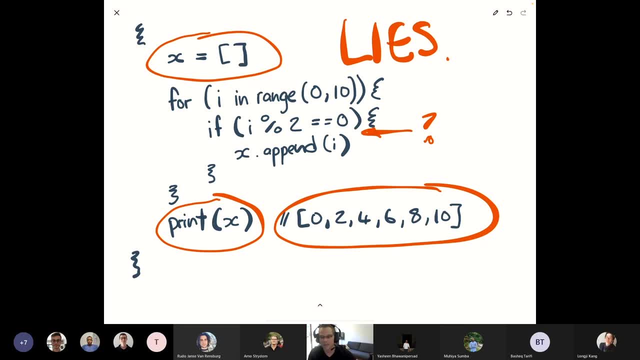 Like this is very, very weird. So when I, when I see X is an empty array and later on I print X and it's like it turns out it's not an empty array, like shit, what's going on here? And it's like I mean I'm, I'm, I'm saying you should ask this. 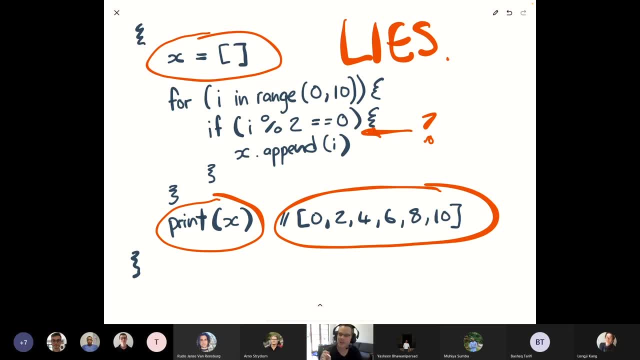 It's like yeah, it's like Why do I? so? it's like no, so it isn't. Sometimes it can be this full array, but it's like you have to have understood and followed its path through this program in order to know what X is. 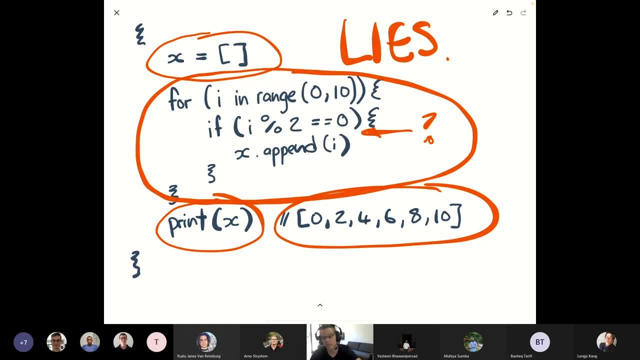 Do you know what I mean? That kind of makes sense. So it's like, oh, it's pretty shitty actually, because it's like in here lies a whole bunch of murky knowledge. So to know anything about X, I must know about the context of where X has ever been or ever been manipulated. 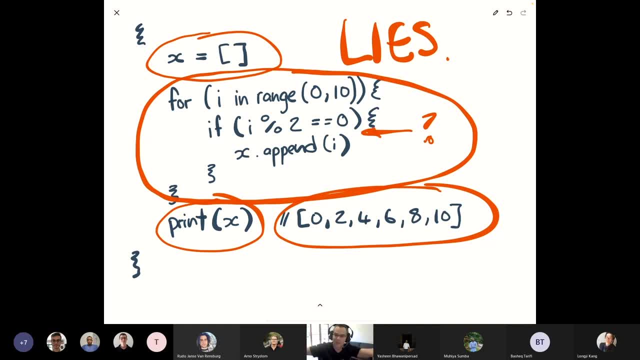 And of course this is like a very stupid example, But take this to like a big you know, take it to the to the extremes where it's like you can know nothing about anything, If, if, you can't, if you can't rely on this statement up here that X is an empty array. 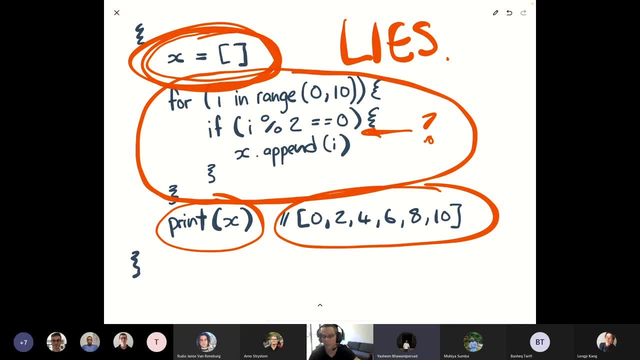 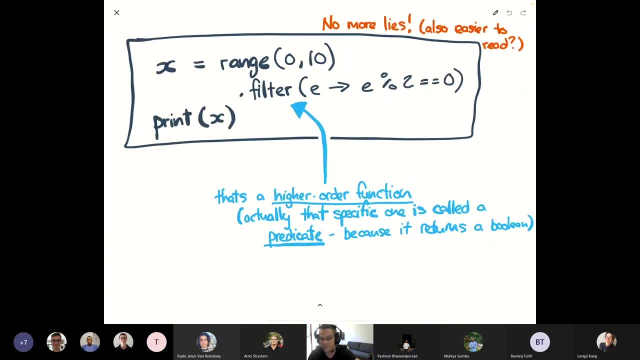 Right. Do you know what I mean? If it can be modified, then it's like: OK, well, all bets are off, always Right? So what's a better way of doing this? So a better way of doing it is to actually make X what he is. 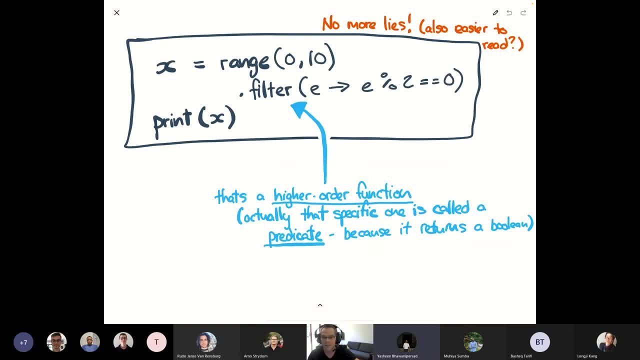 Right, Which is like he is. X is for. So in that range of naught to ten, the list of elements that are filtered for only the ones that are that are even. does that make sense? So look, there's no more lies here. 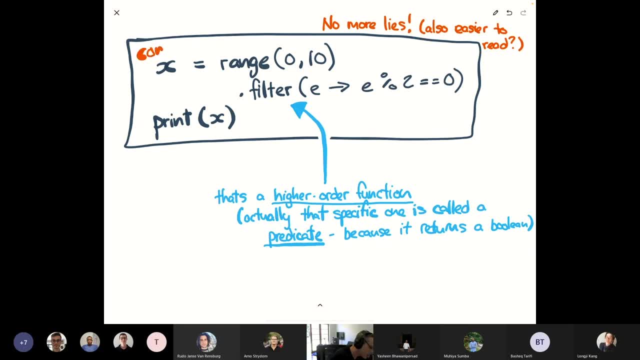 X is this thing, And I can put the word const here, Right, I can say const X if my language- hopefully my compiler or language- supports this thing. So X is always this thing, It's never anything else. So if X is in scope and you are able to print it or do do whatever you want with it, or calculate with it, or 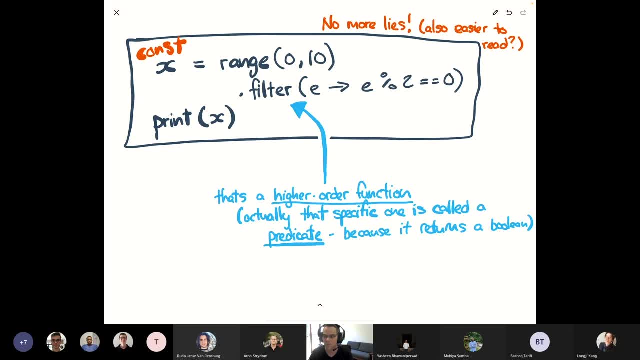 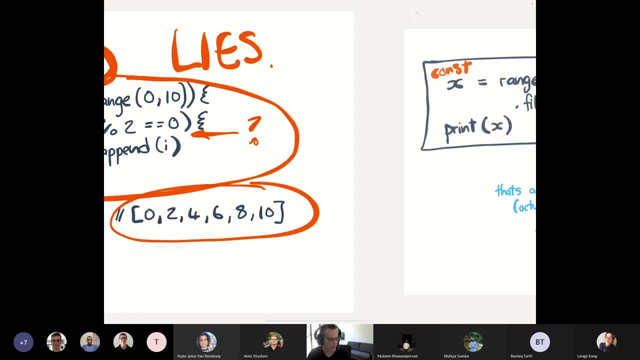 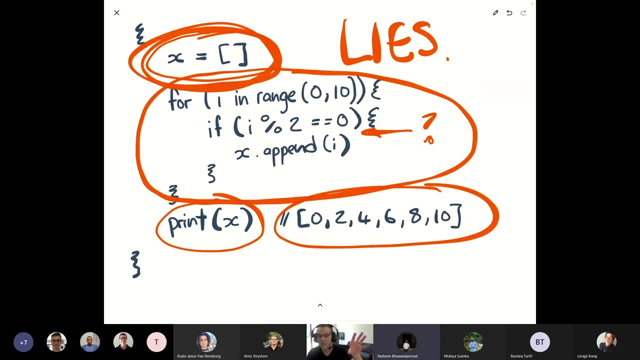 If you can iterate through it, it is this. There's no other state it could possibly be. Does that kind of make sense? So, like this is a better way of describing X Right Rather than this, Do you guys agree? So, so you may be comfortable with this kind of style where it's like: oh, I build up something. 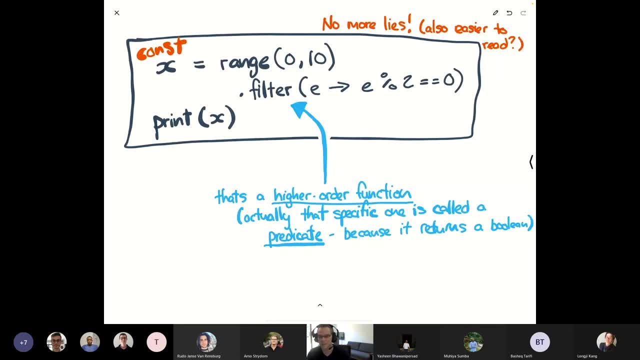 I would say to you: wherever you see this, try to replace it with this, because this is, this is much better, because I can also take X. I could lift this whole piece of code here. I can cut and paste this into anywhere else. 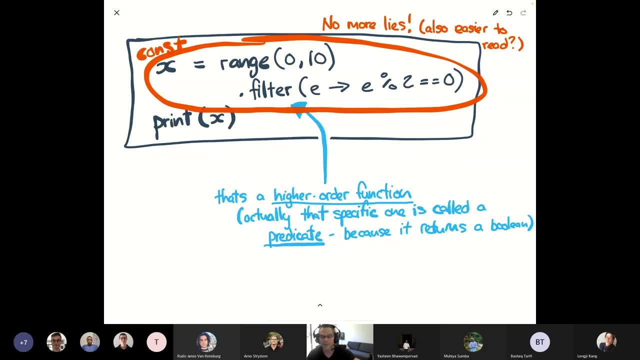 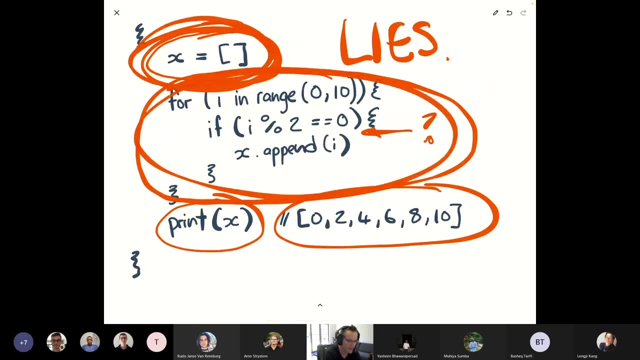 And it's like: yeah, it's good, Like it, X will be this thing. You know what I mean, Whereas I can't cut and paste that there and like it, like this piece of code. If I want to cut and paste that, I also have to know, but I have to cut and paste that piece of code. 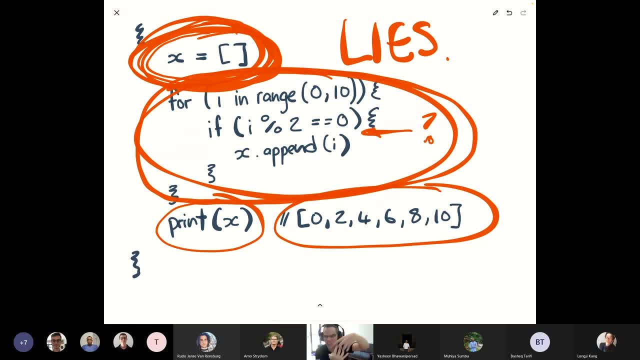 It's all like connected. It's all like that glued together And it's like, actually, the glue is not that explicit, because it's like, well, where does the glue start and end? It's like, oh, it could be anywhere. 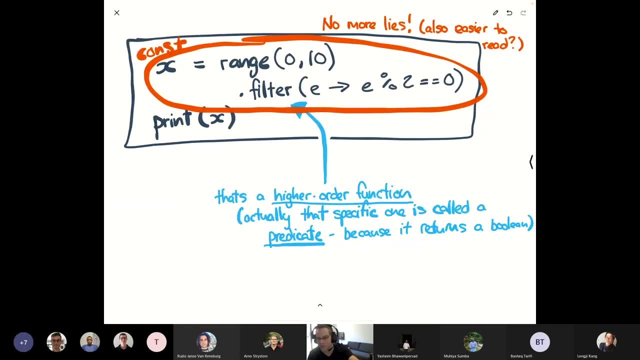 Right, Who knows It could be anywhere. You've got to like file Search, find X where it gets used, who knows? And then you're like try and cut and paste all that together and drop that in, Whereas here this is like totally atomic and beautiful. 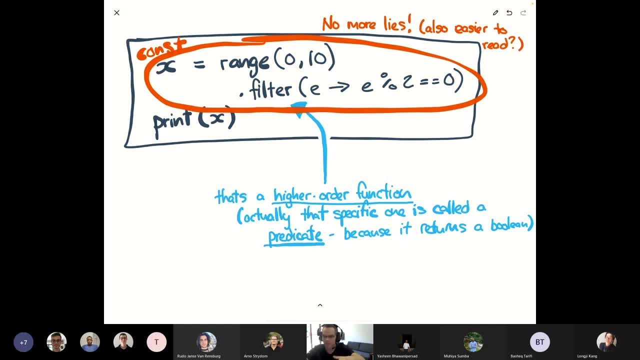 Like one, one line. Of course it could be hundreds of lines of filters and maps and reduces and the whole story, But when I lift it out it's like, yeah, it's complete, Boom, I can drop it in. 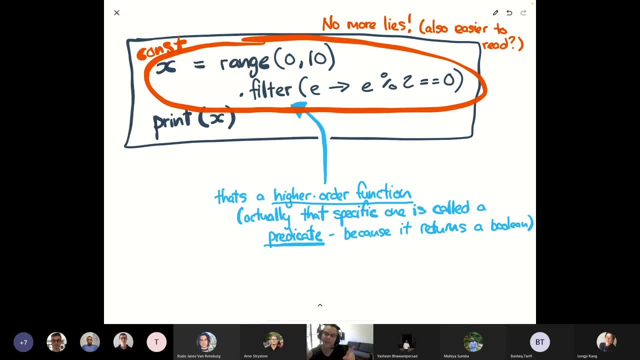 And so to be clear, this thing, filter is a higher order function, So it takes a first class function. I suppose in the scenario of filter that's called a predicate, So it's a function which returns a Boolean. Anyway, there's just good words to throw around and sound clever. 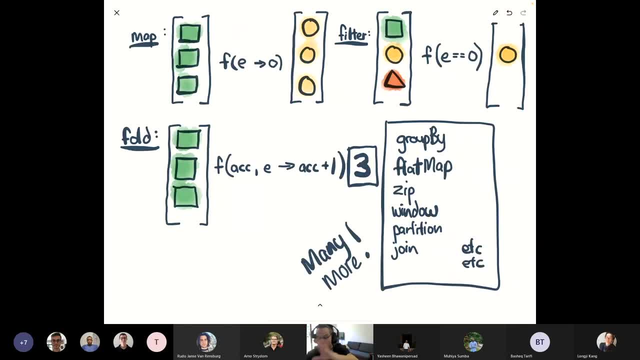 And there's lots of these things, So you can build up these data structures in most languages. I would pick almost any language and say you can do this in any language, Like there is support for this. So you figure out what are the. what does map do? 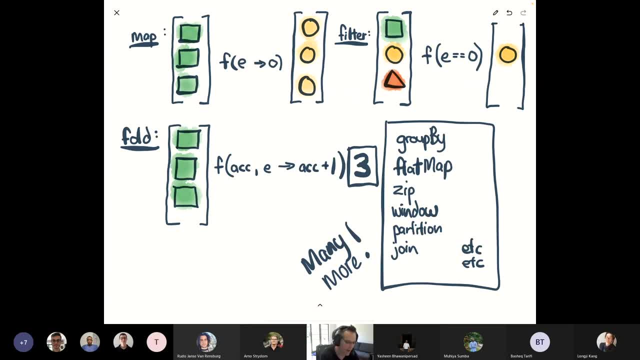 What is filter, do What is fold, do What is, and then I've listed a bunch of group by flat map, zip window, partition, join all these things. These are these things to build data structures In an expression, the type of way in order for you to like, set them to a constant, you know, without you having to iteratively build up data structures. 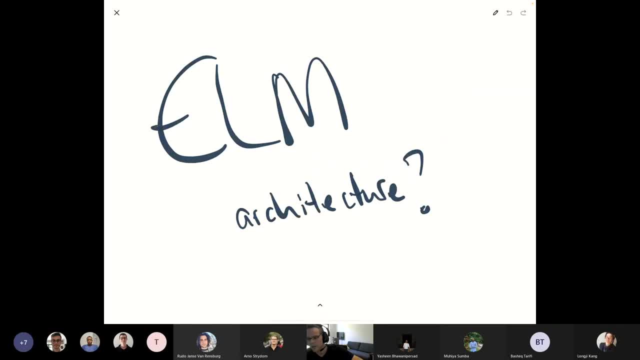 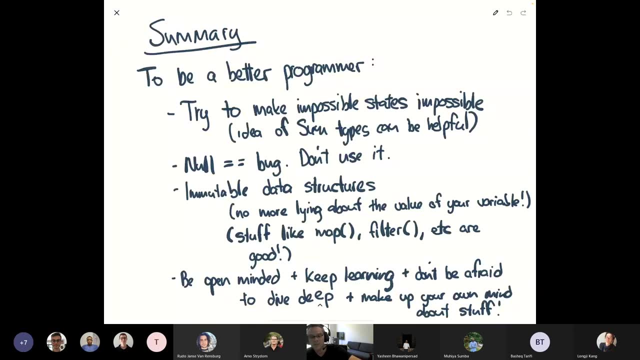 That makes sense. First class functions. Yes, Elm, We don't have time. Sorry, Elm looks like this. Maybe we could do something on Elm in the future. It's very cool. You should play with Elm. Try it, Okay. 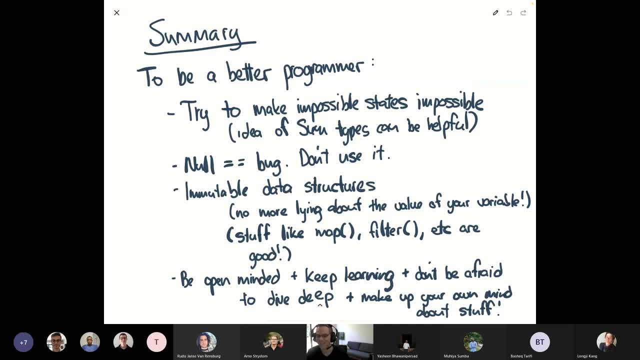 So here's my summary: To be a better programmer. Well, one of the ways to be a better program- I think there's many ways- right, And try to make impossible states. impossible Like this is cool, Actually. you should look at this. 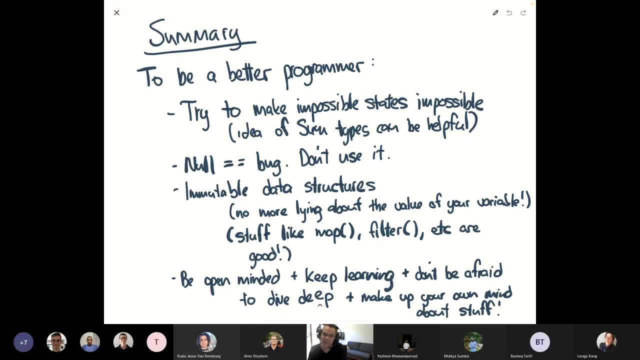 Whenever you write a function, be explicit about like: what are the states that can be, so that the poor guy who's calling your function- even if it's you, you, the poor guy, you tomorrow- who's just woken up and going, Oh, I don't know what this function does? 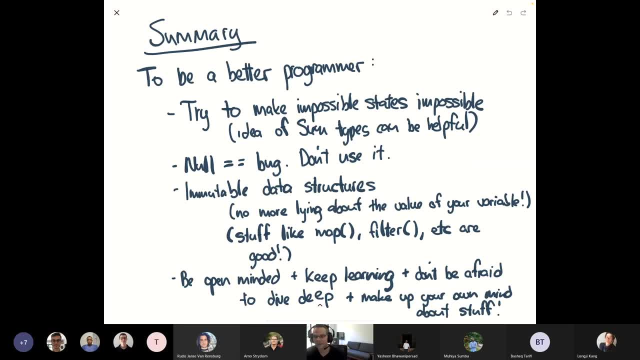 It's like: make his life easier, make the future You, um uh, make his life easier, right, Future You, uh. idea of some types is very beneficial there. Uh, now there's a bug. I would say in almost all cases, like, don't use it. 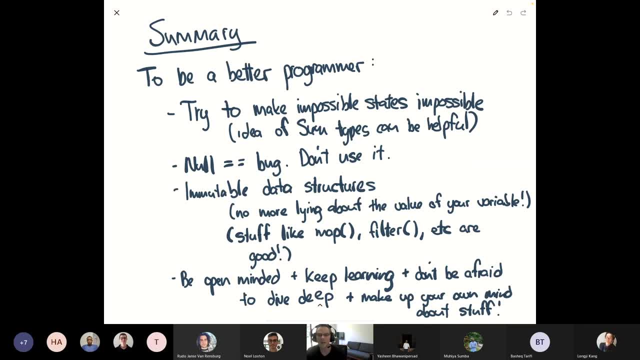 Don't use it. Immutable data structures- definitely worth thinking about. um try not to make put too many lies in your code, So we go: X equals empty array And later on it turns out it isn't like that's a lie. 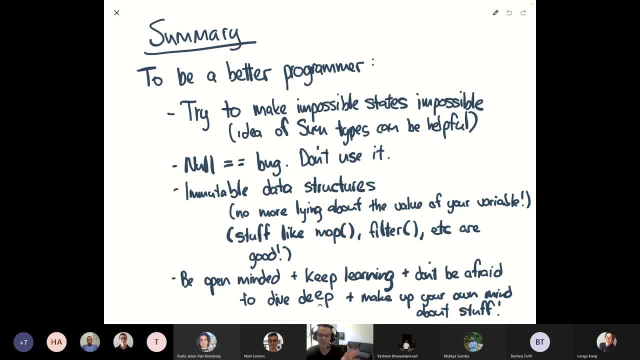 Um and so ideas like const and things like that. sometimes the compiler can help you say: Hey look, you're lying, You're making X, something else. Um, those, those are good, Like it used to. at least default to those things, right. 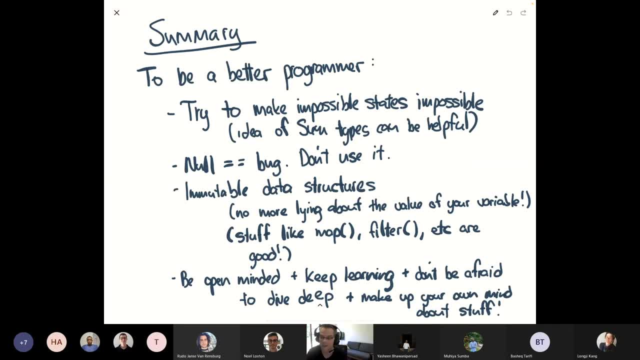 And then make your lies more explicit. So where you do end up having to lie, it's like: Oh, I'm lying here because you know there was a scenario, Don't make all your code. Your code lies, Um. and then the last one is like: be open-minded to these things, like, and, freaking, go and check these things. 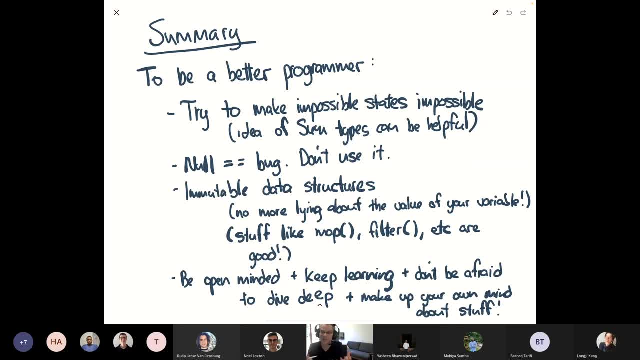 Right. So when, when? um, because you can have this like initial. you know you can choose to respond to new stuff in two different ways. The first one is: go, Oh, it's horrible, And I'm going to like it's evil for some reason. 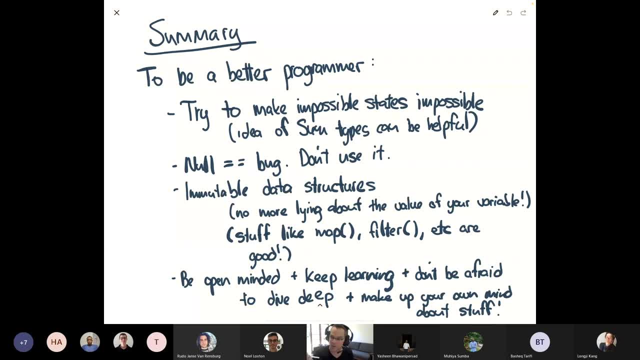 And I'm not going to look at it, or it's like: Ooh, it's new and uncomfortable. There must be something interesting. Let me go and like, look at it Right. So like try to be more of the latter. 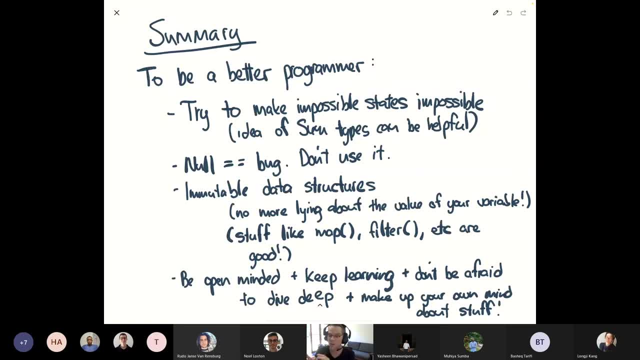 So when you see something New and uncomfortable, go, Oh, there's something interesting, I can learn from this, rather than go, Ooh, no, this, like this, like hurts my worldview somehow and like, Ooh, it's going to make me feel stupid or whatever. 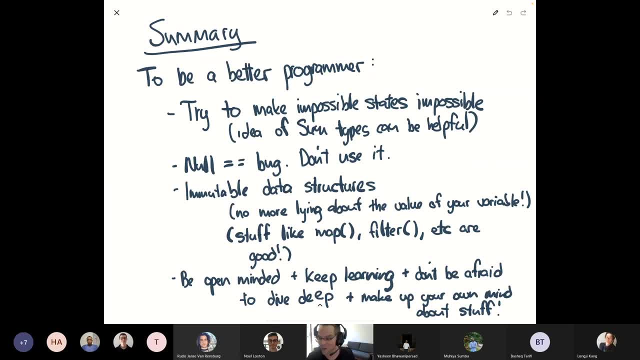 Like no, no things that make you feel stupid or good, because it gives you good opportunities to go and learn about them Right, And make you smarter. Right, You, you must run at the the opportunities to make you smarter, rather than go. no, I'm already smart. 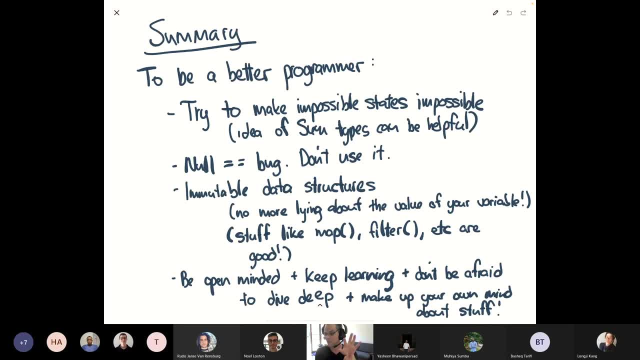 And like: no, I don't want to look at, um, look at this like strange and uncomfortable stuff that people are talking about, because then you will become Uh like. I think that first, first response is: like: you will become a COBOL programmer. 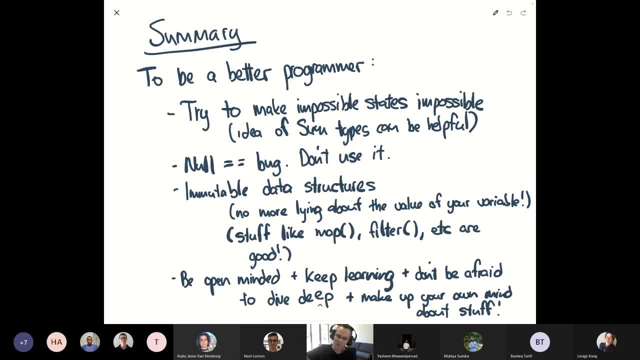 That's what COBOL programmers did. They said, Oh, COBOL is the best. Like, Oh, this new stuff, No, I'm not looking at it. Oh, this new AWS cloud stuff. Oh, what's this? quantum computing? 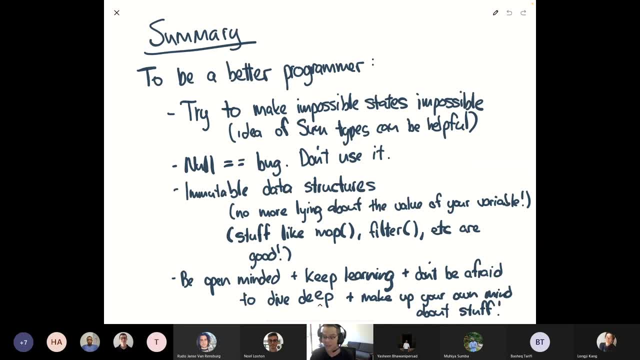 What's this? like I'm not doing it, I'm good at this one thing And like, no, that's actually not the career that you picked, You, you, you didn't pick a career in programming in a language. You picked a career in continuous learning, if that makes sense. 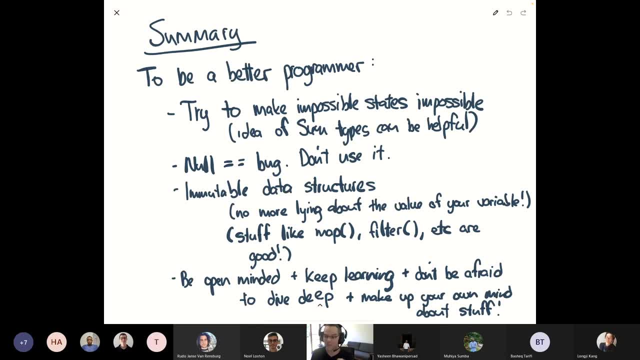 Um and so what must you do as a continuous learner? Go and find, Find the things you don't know about and go and learn those things. Do you know what I mean? Like that's. that's the whole, that's the end. 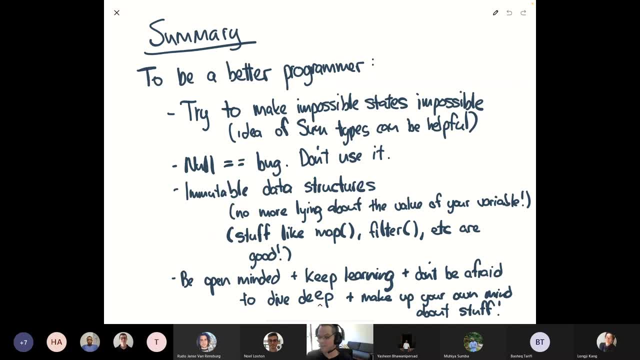 Make like an, apply those things all the time, and then you will be a happy person. If you choose option one, I think you will be deeply unhappy, actually, And like maybe it's the wrong career, I don't know, Um, but I know it isn't because we've, like you know, we've spoken to all of you guys. 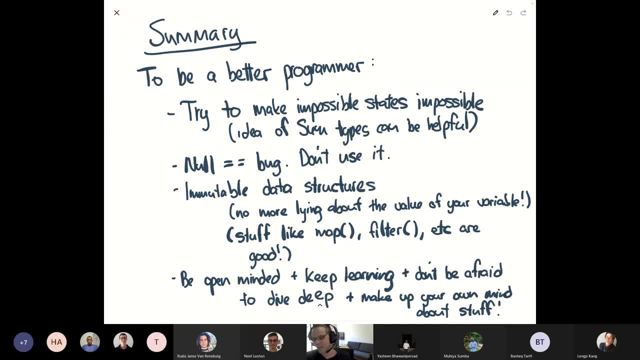 You're all smart, continuous learners, You know. those are the kinds of people we, we we kind of hire and attract, Right, And so make up your own mind about stuff. Yeah, that's important, Um, And that's me, guys. 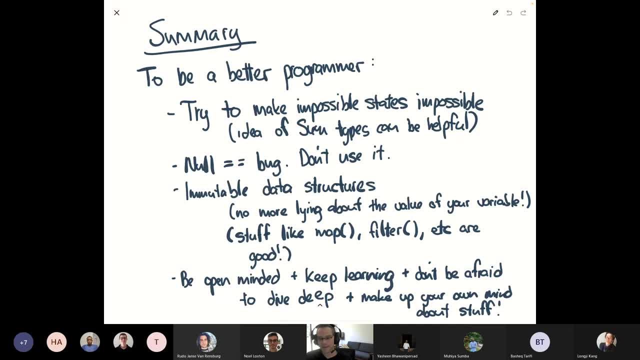 Uh, sorry I've run out of time, but does anyone have any questions about anything? Uh, how's it, Tom? I have a question. Um, are there restrictions on what you can do with functional programming? It's like any program can be turned into a functional program, or are there some things you actually can't do in functional programming, with functional programming? 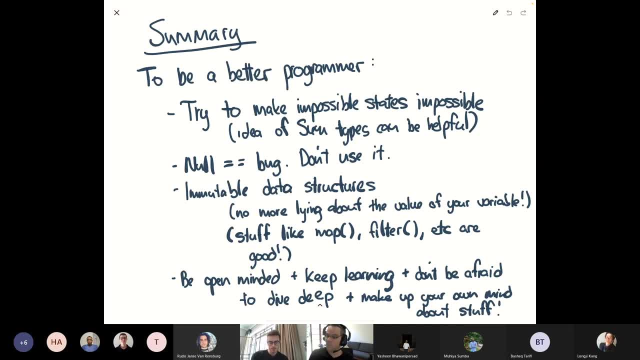 Uh, no, no, I would say anything that can be done in a program can be done In a functional way. whether how much like pain you have to go through in order to achieve it is like, up to you to make you know that assessment. but uh, there's no limitations, so that they're you know it's touring complete right. 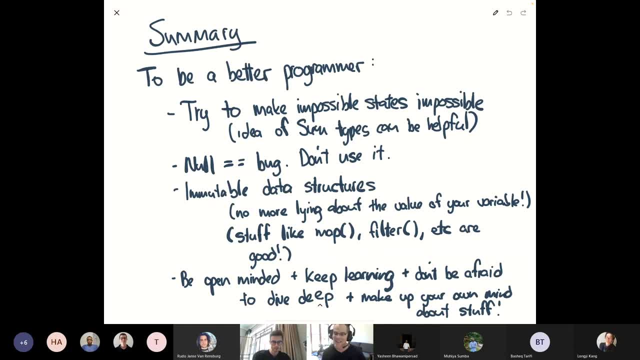 And we know what touring complete means. Hopefully, if you didn't study computer science is like um, you know they can be done. I I would say like there there's a whole domain of problems which are probably more suited to a functional style versus a imperative style, but um, 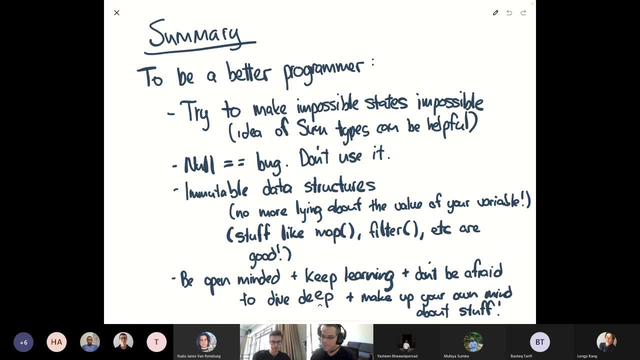 I would say no, there's no limitations, No, no technical ones, No. And what would be the best way to start? just like getting, just be getting your hands dirty going and trying to write code. I would say I mean if, if you're, if, if you're keen to dive into, like, into that world of pure and what is pure, and then so it comes down to like your personal preference. 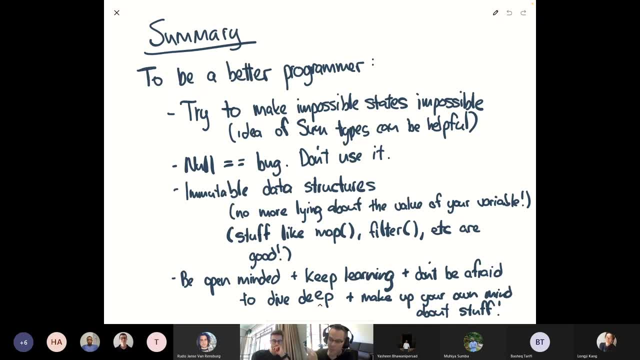 If you want to dive into pure and then figure out how you make your way back to productivity, then I would jump into Elm. honestly, go and have a look at Elm or pure script. I'd say pure script is like like it's. there's some scary shit in there, but I think you can be Elm. Elm is like constrained enough, but it's not. it's not a general purpose language either. 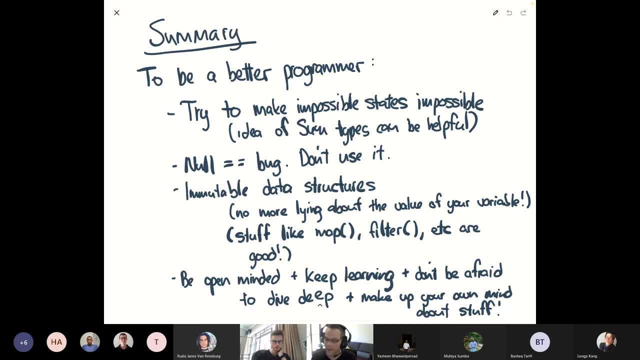 It's only for web programming, So you can only build web apps using Elm. You can't run like a command line script and like read records out of adjacent. It doesn't have any of that stuff, So it's only for building web applications, which is really cool. 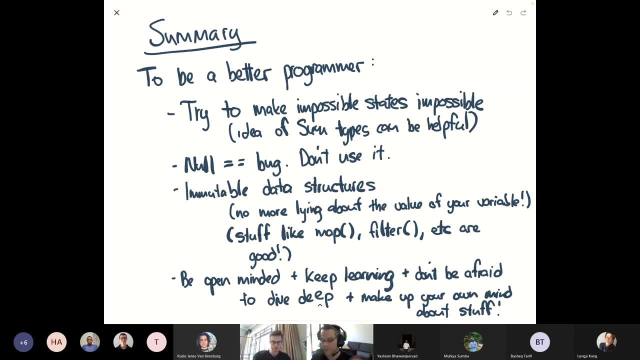 So it's like, in that limited sphere, Elm is beautiful because it's really stripped Self down to what is useful in that domain And I think it's very easy to reason about Um. the other option is like: if you prefer to be less uncomfortable, then it's like: well, take the language that you like- C-sharp, if um, Java, whatever, uh, JavaScript- and then move your way into, into, into, like, using more high order functions, using more immutable data structures, that kind of stuff. 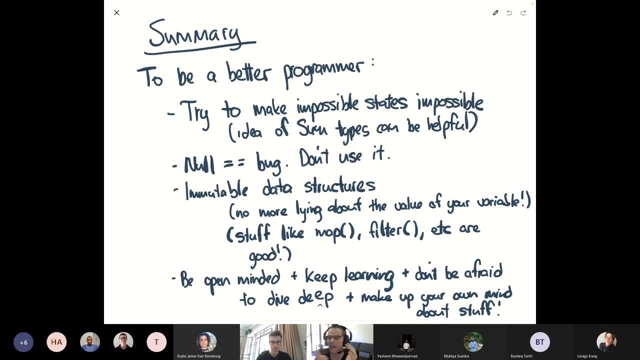 And maybe you're like. so it's like, which way do you come across the bridge? Because at the end of the day, you probably want to be stronger across both of those things. So it's like, if you want to dive headfirst, go for Elm man. go check out Elm. uh, you could check out pure script um Haskell. those things will teach you a ton. but you may go down like a rabbit hole of yours. 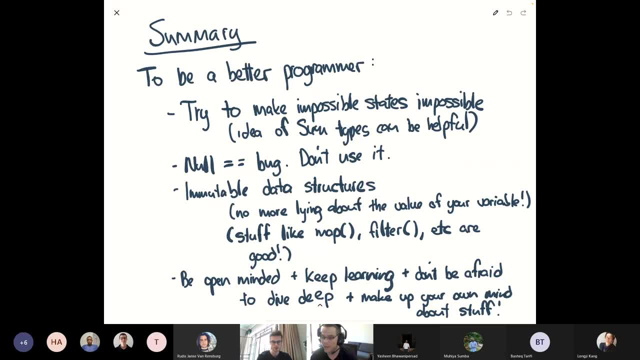 So when I started with Haskell it was probably 2015.. Um, so I knew F-sharp pretty well And I wrote a bunch of Scala in like the early 2010s. That was really my first introduction to like what is really like functional like. what are the functional ideas F-sharp? 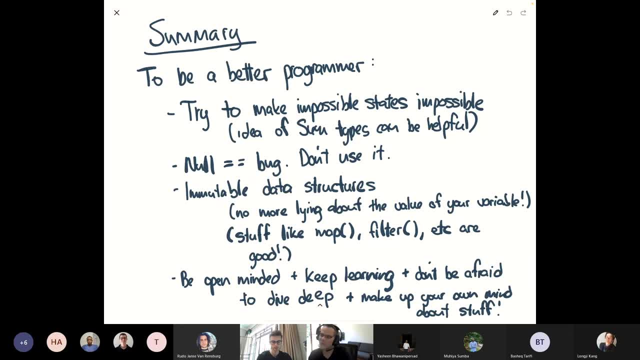 And it was really cool. um, which I think is an ML, or is it? I think it's an ML derivative, So I really enjoy that ML idea. So maybe Reason is also a good, a good uh, Reason, ML is a good language to pick up. 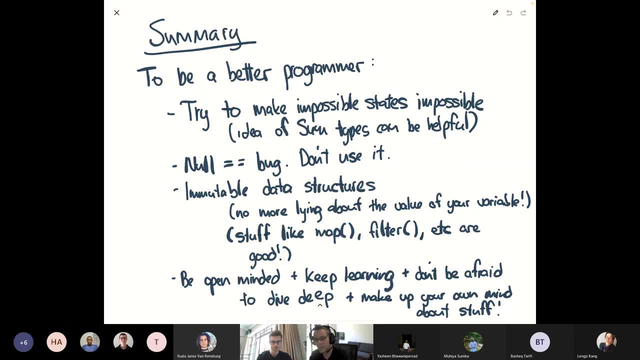 Um, but then I- I just like got into Haskell in 2015 and I just found it like it was far too much. It was like, oh shit, Okay, I gave myself a few weeks to learn this language. you know evenings- and it turns out I need actually like months. 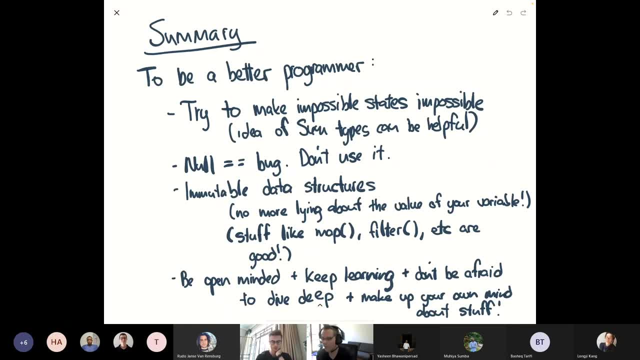 Um, and slowly, from 2015.. I put it away for like a long time, picked it up again, put it away. picked it up, put it away And I'd say today like I probably I still would not comfortably write Haskell, but, um, I'm finding pure script to be an- uh, potentially like a more productive version of of Haskell, but it's like it's taken years to become comfortable.